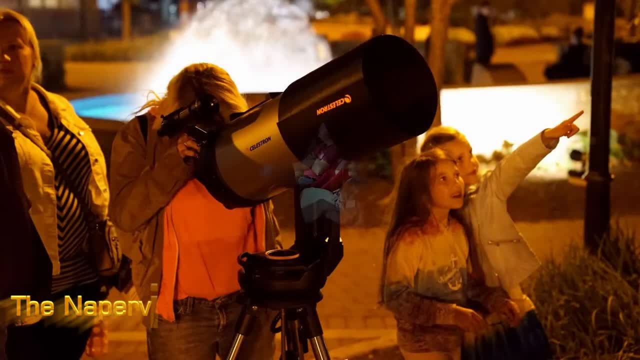 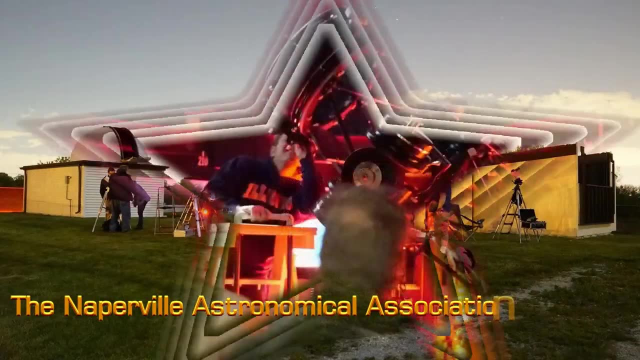 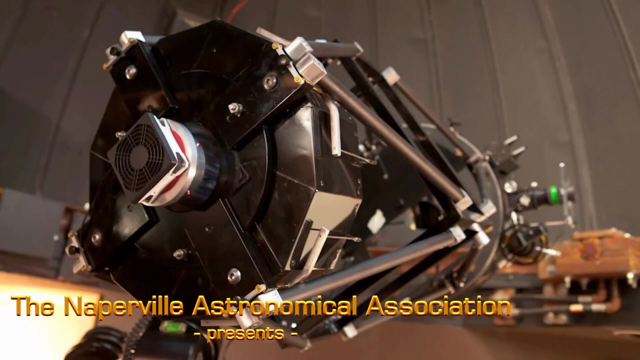 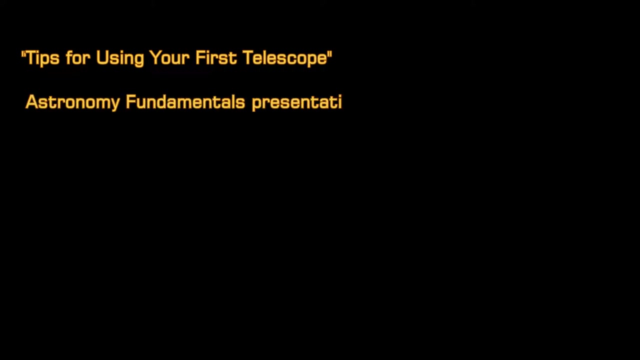 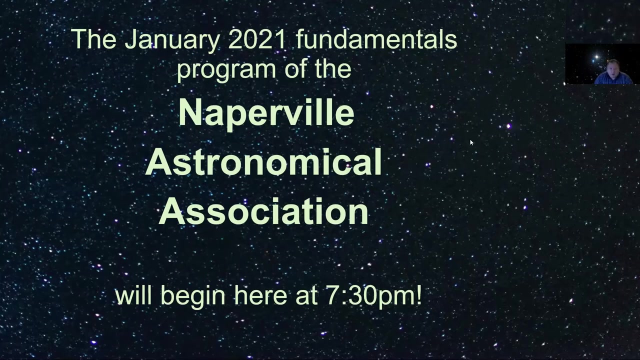 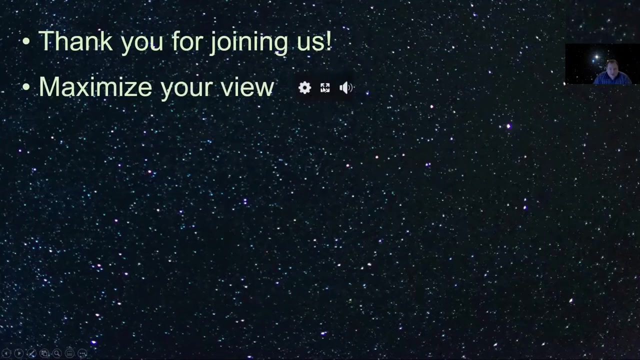 Thank you for watching. Hello, Thank you for joining us tonight for January 2021. Fundamentals Program of the Naperville Astronomical Association. Just a quick reminder: you can maximize your view by clicking the little maximize button in the corner. Make sure the audio is how you want it. 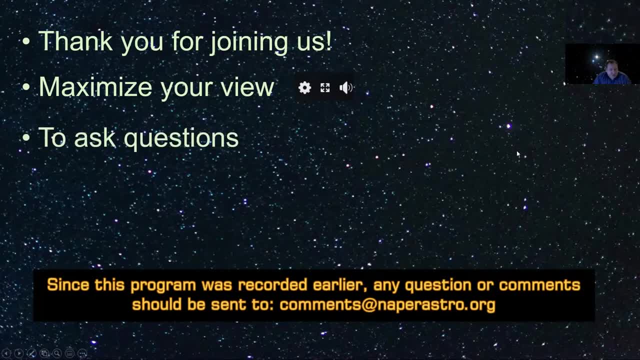 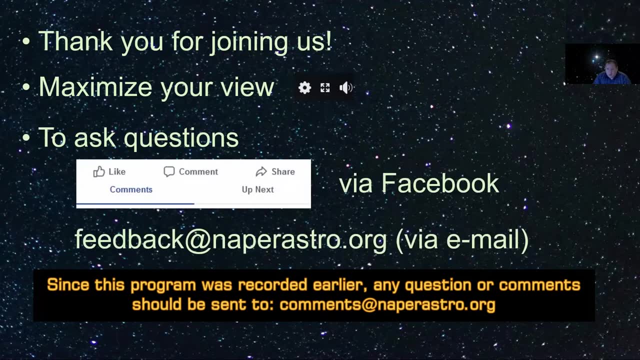 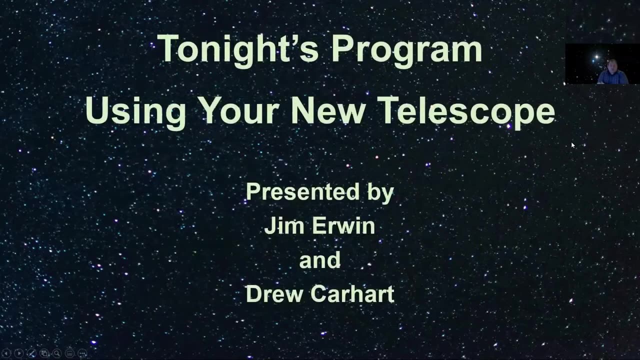 To ask questions. You can ask your questions on Facebook Or you can email us at feedback at naperoastroorg and we will see those questions and we'll try to answer those live. So tonight's program is about using your new telescope. You know it's it's shortly after Christmas time, so we're assuming that some people maybe got a either family present or 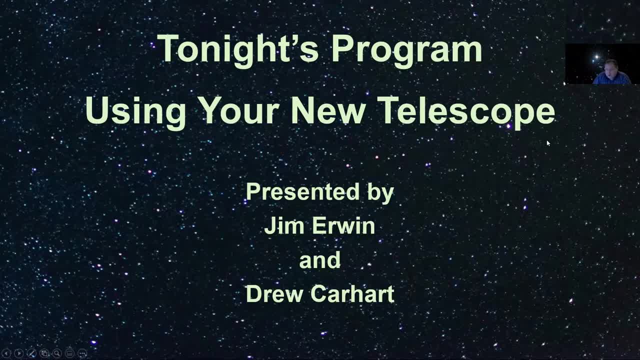 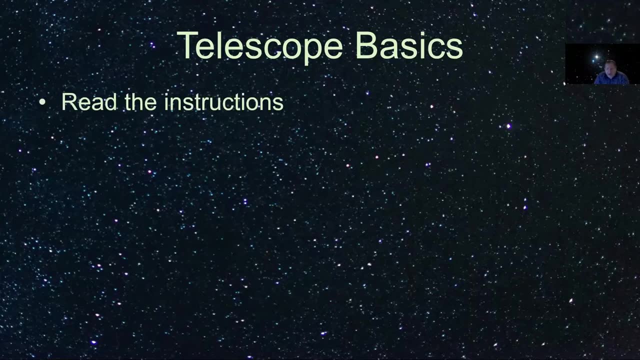 Or somebody got a new telescope for Christmas and you might not know how to use that very well, so hopefully we can demonstrate tonight a few techniques on on how to use your new telescope. So some telescope basics. Try to read the instructions if you can. I'm not necessarily an instructions guide, but 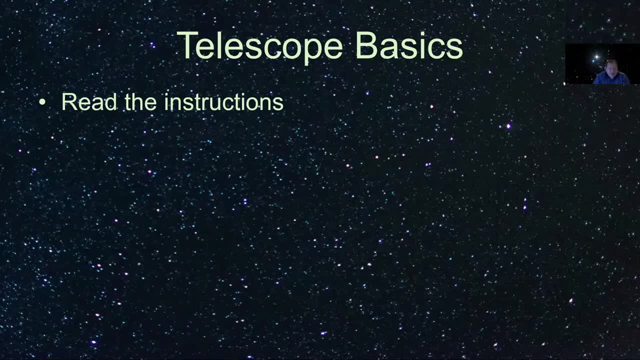 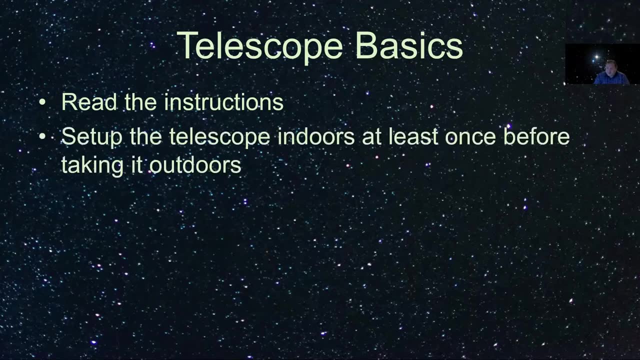 It really will help. if you can, can sit back and take an hour and try to read those instructions. You should set up your telescope inside at least one time before you set up outside. it's- it's cold outside right now anyway, So you know it's. it's a good thing to set it up indoors because 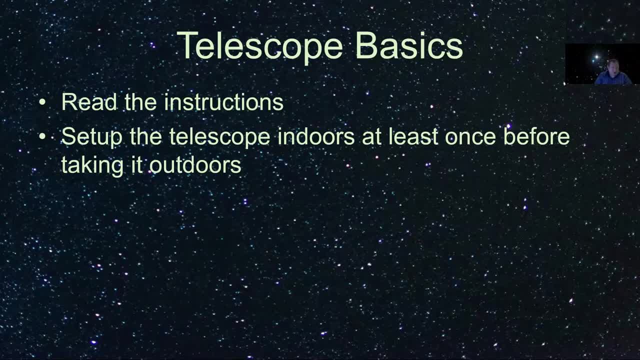 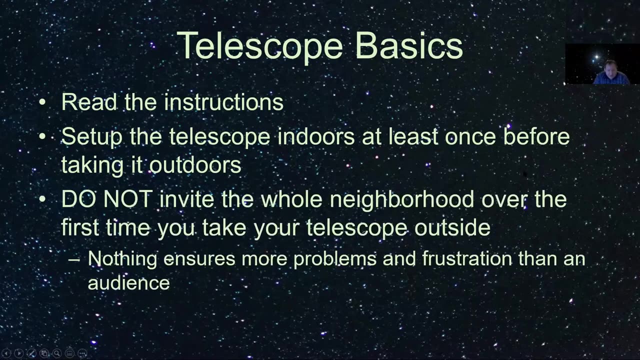 When you do it outside, you might drop a little screw or drop something that you know you're going to. you're going to regret it falling into the grass and you're not being able to find it. Another really important thing is do not Invite the whole neighborhood over the first time you take your telescope outside. 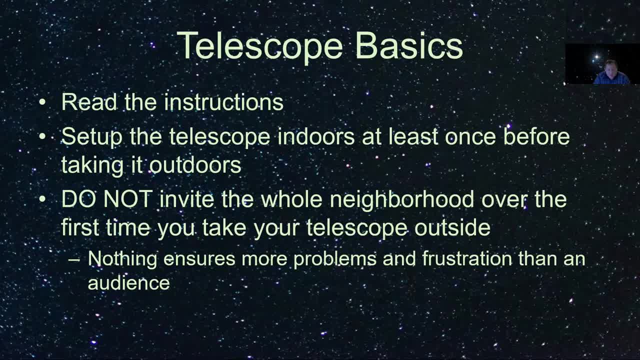 Nothing, nothing ensures that you're going to have more problems than then a crowd standing there watching you. So use it. use it yourself At least once, maybe twice, maybe five times, until you get the hang of it. And then, once you get the hang of it, then you can start inviting people to to look, because 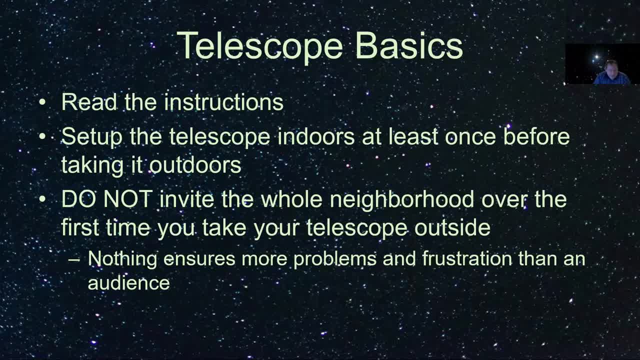 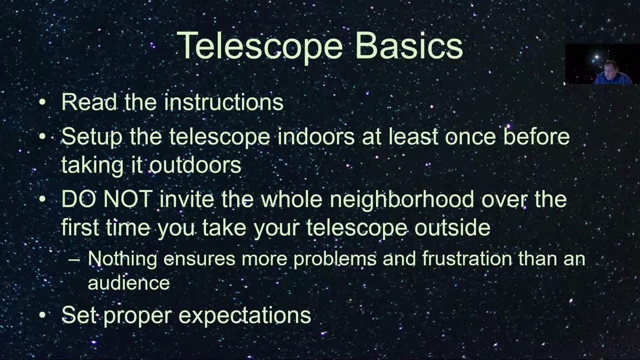 You'd be surprised how many people set it up in the backyard for the first time or take it on vacation up you know where it's really dark and don't know how to use it. Another thing: you need to set proper expectations. So today you know you can Google anything on the internet and 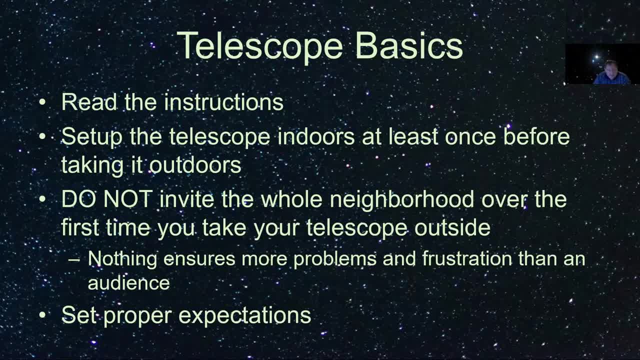 You know you can find the Hubble Hubble views of galaxies and nebula and star clusters. You know you can find the Hubble Hubble views of galaxies and nebula and star clusters. You know you can find the Hubble Hubble views of galaxies and nebula and star clusters. 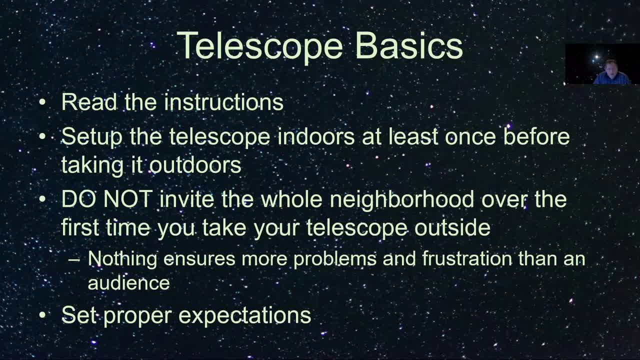 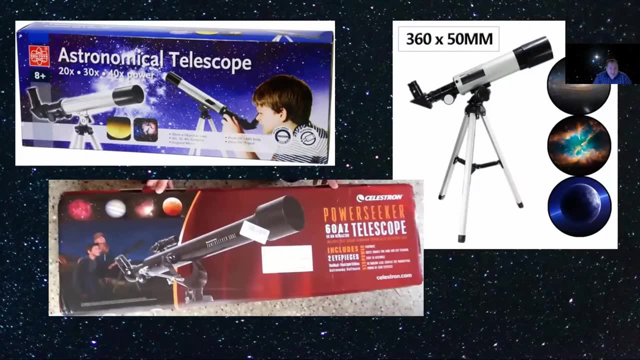 And they all look beautiful And that's not what you're going to see through your telescope in your backyard. So you need to, you need to kind of understand the, the views you're going to get. So these are a couple couple telescope boxes, and the one on the upper right is a is an ad for Walmart for telescope. they they show right on the box: Look at these beautiful things you're going to see and 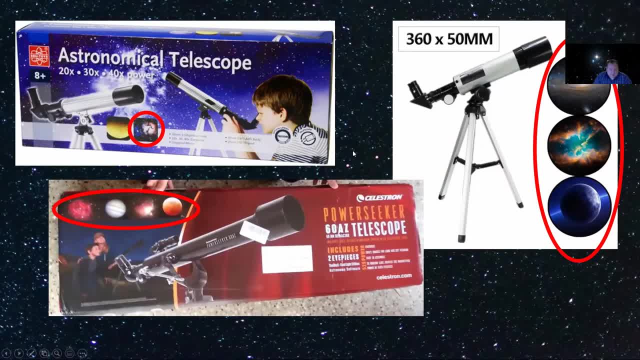 And the prettier the picture, the You know the faker the telescope has. I guess, Because You know to to see. this is the Andromeda galaxy up here in the corner. That's even in the darkest skies with the biggest telescope, It's not going to look that, not going to look that pretty. 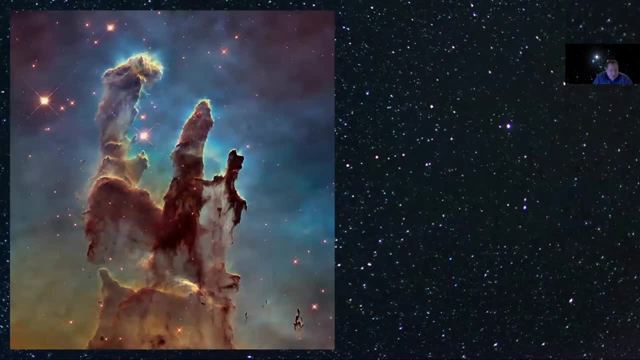 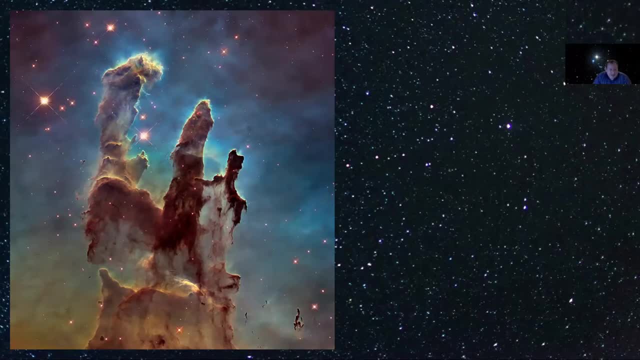 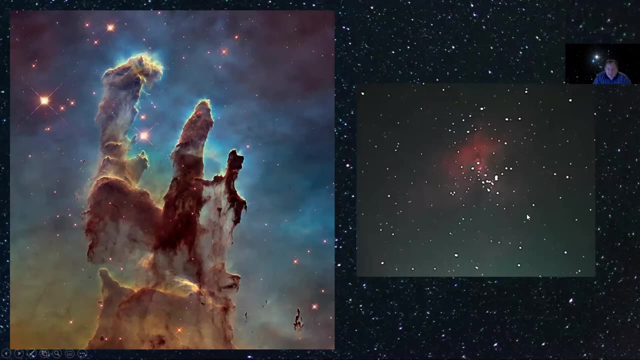 So, again, this is a Hubble image of what's called the Pillars of Crete. So again, this is a Hubble image of what's called the Pillars of Crete. This is located inside the Eagle nebula. So this is the Hubble image, And this is probably more along the lines of what what you would see through your telescope. 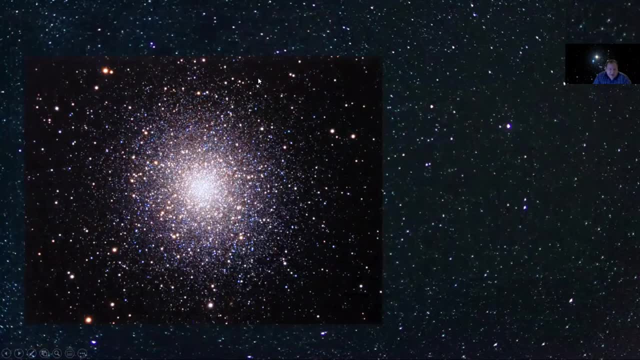 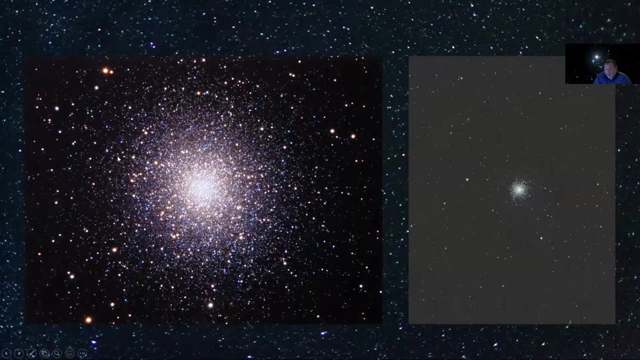 This is a M 13, the star cluster in the constellation Hercules. just a beautiful star cluster. It's probably gonna look a little more like that in your telescope. So we're going to look at some of the. So we're going to look at some of the. 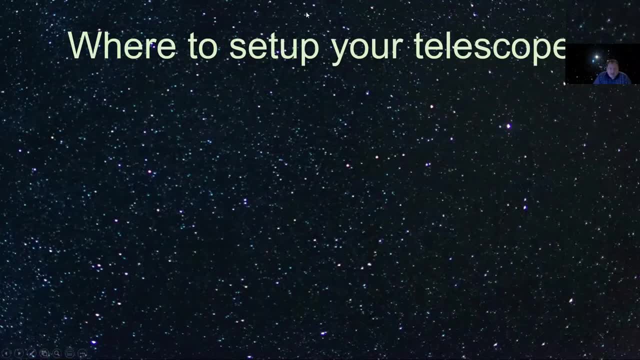 to set up your telescope. the first thing, uh, you, you want to be outdoors. um, i know it's cold out right now, but, uh, you don't want to try to use your telescope through the window. it's, you're going to get glare, it's, it's just not going to work very well whenever you're adding extra glass. 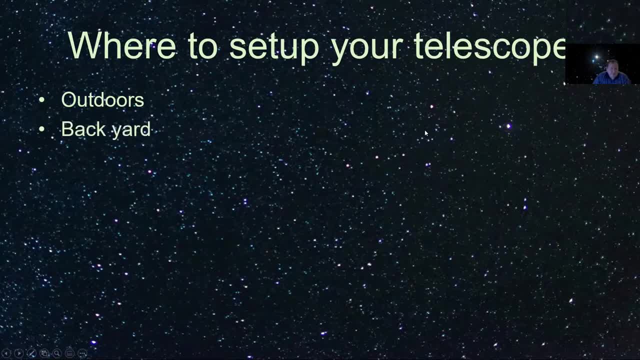 it's not going to do well. so you really do need to take it outside if you can set it up in the in your backyard, like in the darkest part of your backyard, that where you can see the most sky. so if the only area of your backyard that's dark is right under a tree, that's not gonna, that's not. 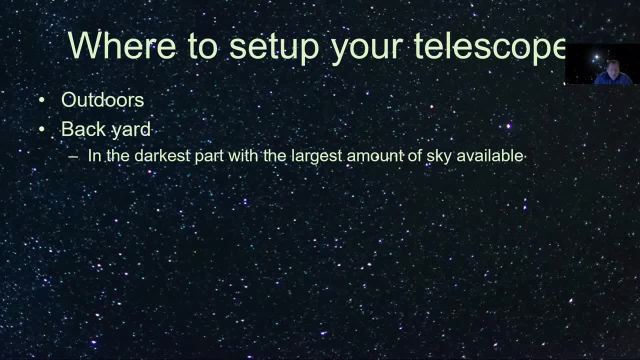 going to do you any good. so, um, you know you need sky to look at. so, uh, you know, pick, pick the place as best you can. but, uh, um, if you can avoid any kind of outdoor lights, do that. avoid surfaces that vibrate. decks are notorious. they're just going to shake every time you. 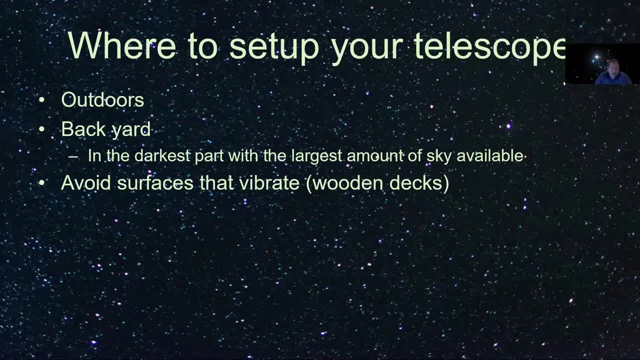 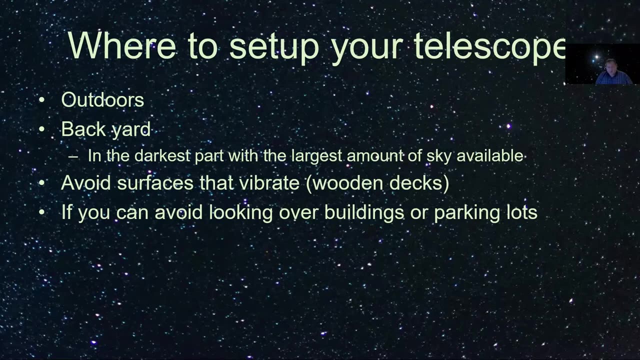 you, you take a step or move the telescope, it's going to vibrate. um so try not to set up on a wood deck if you can avoid looking over the top of buildings or parking lots, these things, uh, the the heat during the day from the sun will kind of soak into these things. 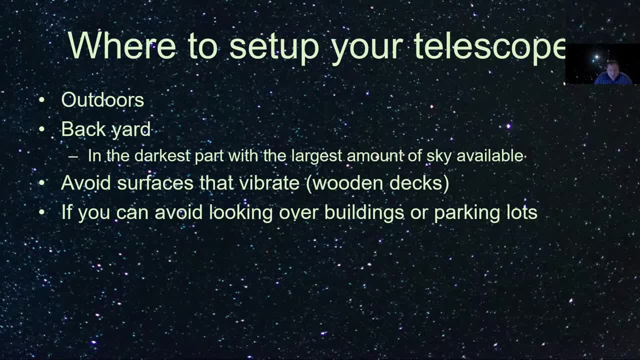 and at night the heat waves will still come off of these things. so you'll, you'll get kind of a wavy um view. the whatever you're looking at. it's going to back up a little bit else around a little bit because of these heat waves. 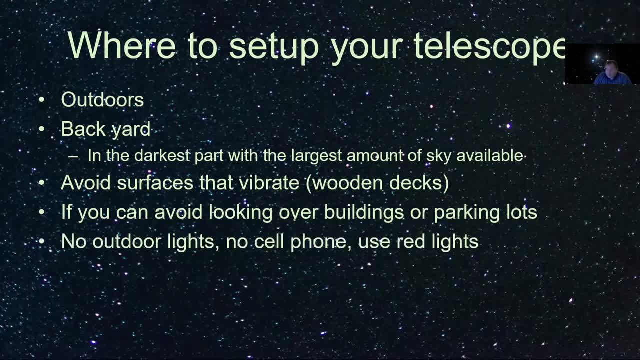 try to shut off all the outdoor lights that you can. don't look at your cell phone um use red lights. you want your eyes, your pupils, to get dark, adapted so the the best thing i can kind of say about this is, if you wake up in the middle of night and you go to the bathroom, you can, you can walk to the 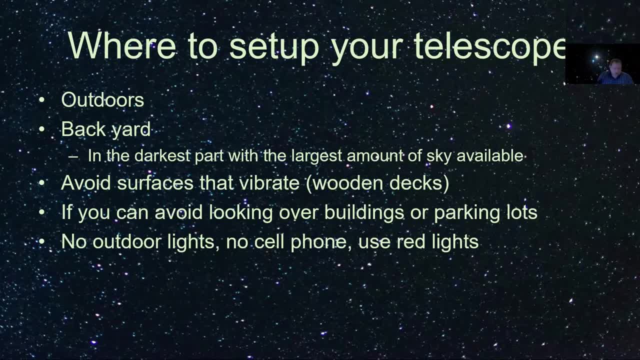 bathroom. just fine with no lights on, but you turn on that bathroom light after you use the bathroom, you shut it off. you're going to be in the middle of the night and you're going to be in the middle of the night. you're bumping into everything on the way back to your, to your bedroom. so when, when your eyes are, 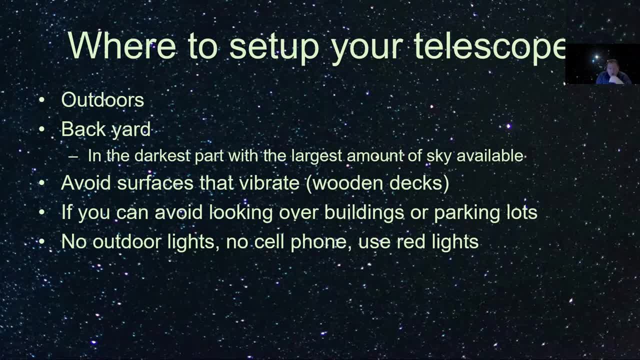 dark, adapted you can, you really can see very well in the dark, but as soon as you you get any kind of white light, your pupils are going to shrink and you're not going to be able to see as much. and uh, one other thing: a place you can set up your telescope if, if you're a member of the 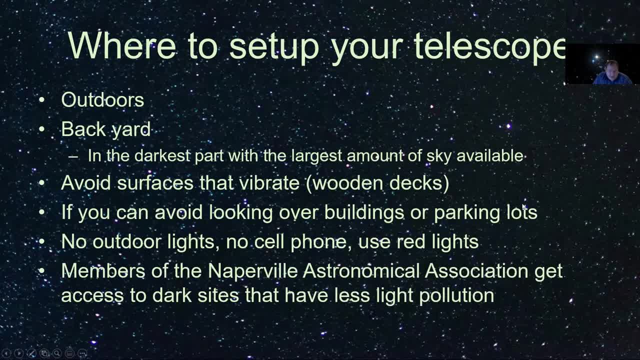 naperville astronomical association, you get access to our dark sites that have uh less light pollution than you can see in the dark. so if you're a member of the naperville astronomical association, you can set up your telescope. if if you're a member of the naperville astronomical association, or maybe a 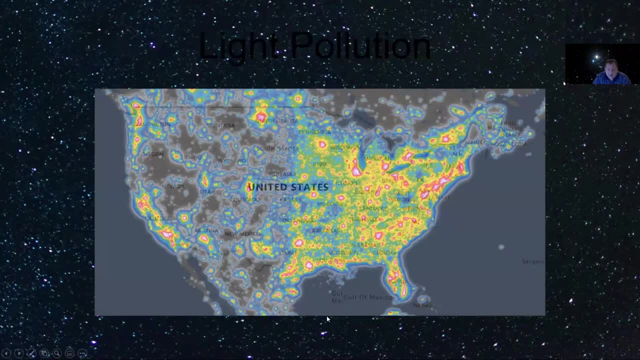 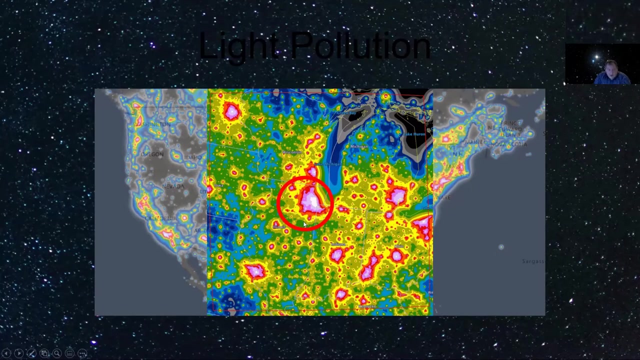 ор you, the more things you can see. The closer you are to white, the less of the sky you're going to be able to see because of light pollution. So it's difficult to see a lot of things from this area just because there's so much light pollution. 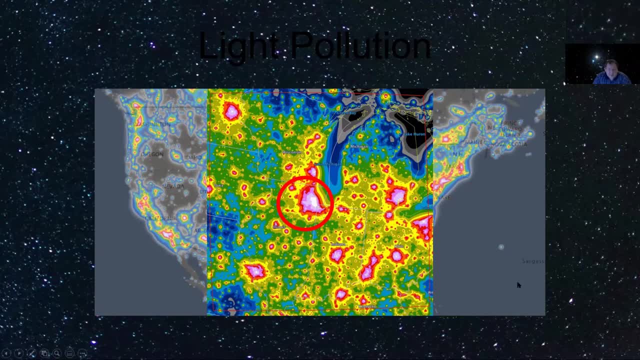 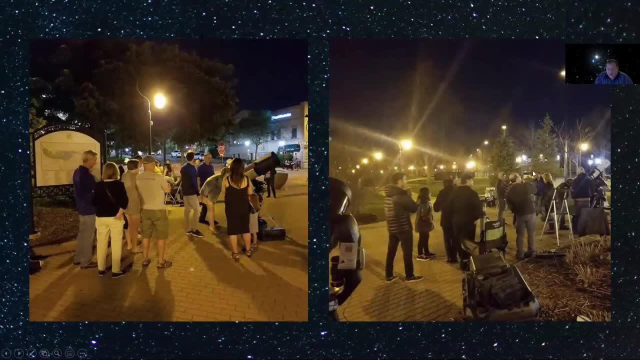 coming from Chicago and coming from the cities around this area. And having said all that, the Naperville Astronomical Association sets up on the downtown Naperville Riverwalk with lights, everywhere Buildings are lit up so you you can view it during the, you know, with with a lot of light pollution, but if you 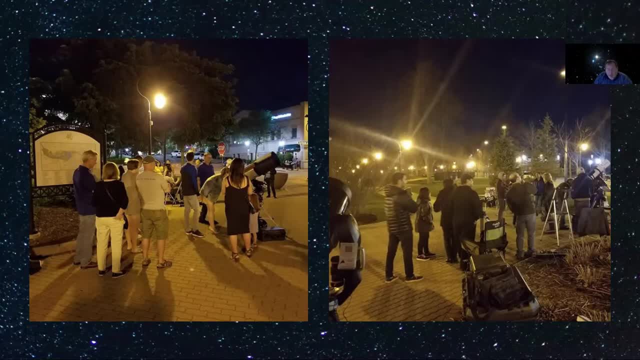 can avoid it, it's, it's better. Typically, what we look at is more of solar system objects, or some of the brighter objects, So some of the things you can still see with with the lights being as bright as they are, but if you want to see dimmer, 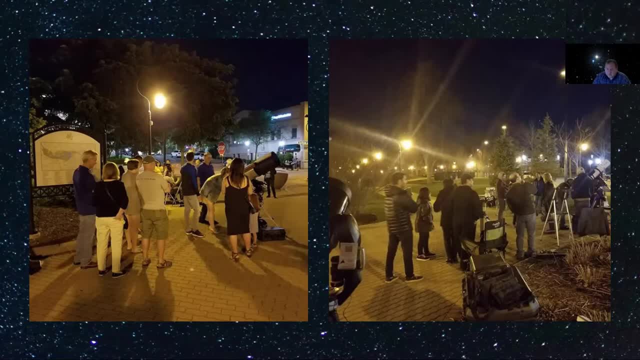 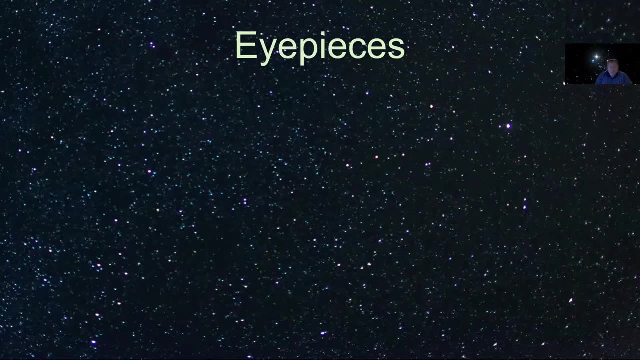 objects you need to get under darker skies. Okay, so you got your new telescope. It probably came with an eyepiece, and maybe you've decided to buy your own eyepieces. There's really three different kinds of eyepieces out there. There's two-inch eyepieces. Now for this. 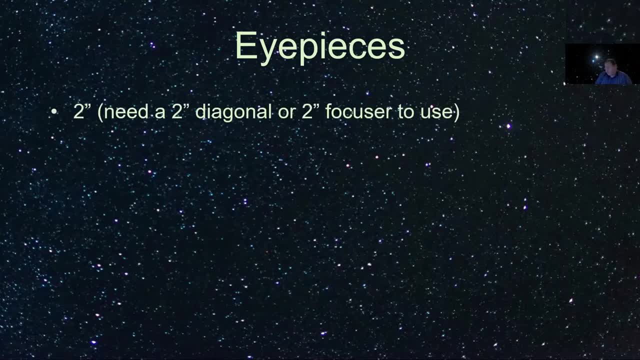 you would need a two-inch diagonal or it'd need to go into a two-inch focuser to use. Probably most of the telescopes that the beginners have don't have a two-inch eyepiece. An inch and a quarter. this is the kind of the standard, An inch and a quarter will. 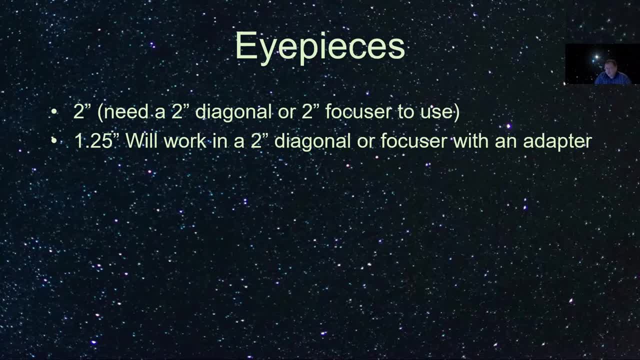 work in a two-inch diagonal or focuser, but you need an adapter and then it usually comes with it. And then there's these older .965 eyepieces. You really don't see these anymore. You might see it if you're looking for stuff on. 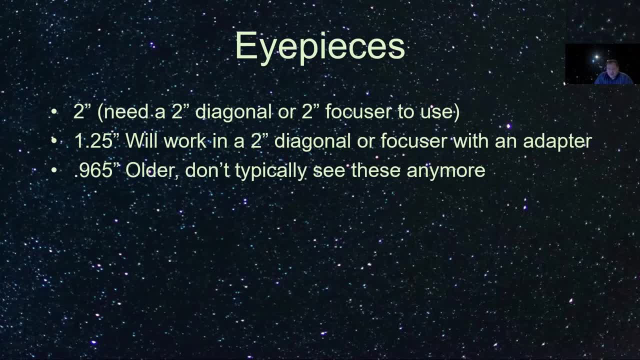 eBay. I would say: just avoid that if you can, because it's there are adapters for those. but you want to go with inch and a quarter or two inch eyepieces? Okay, so this is the most important thing to remember about eyepieces. if 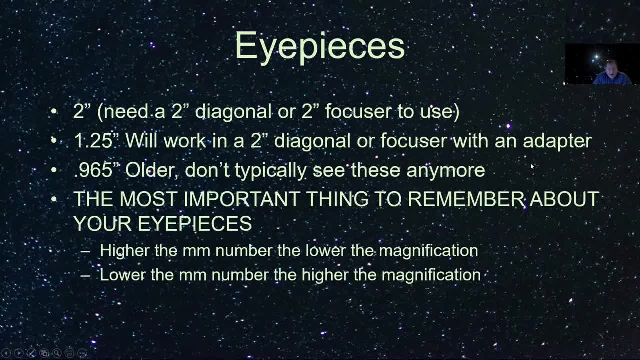 you're a beginner is the higher the millimeter number, the lower the magnification is. and the lower the millimeter number, the higher the magnification. So if you have a 25 millimeter eyepiece, it's lower magnification than your 6 millimeter eyepiece. Now, this is important because 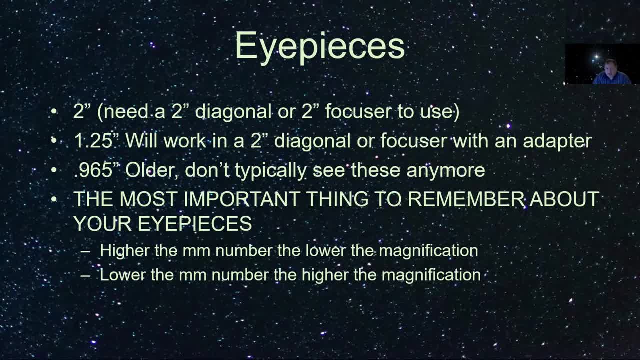 I'm going to show you a little bit of what that magnification is in a later slide. but just remember this: The higher the millimeter number, the lower the magnification. The lower the millimeter number, the higher the magnification. So 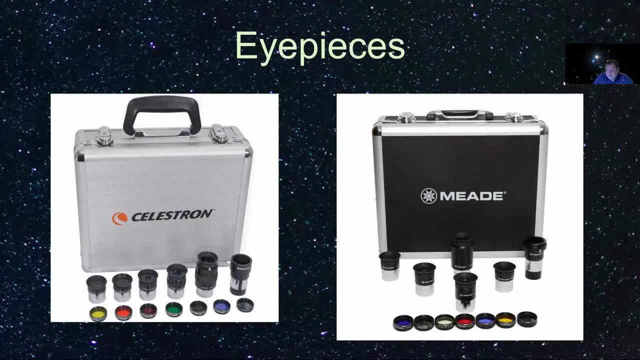 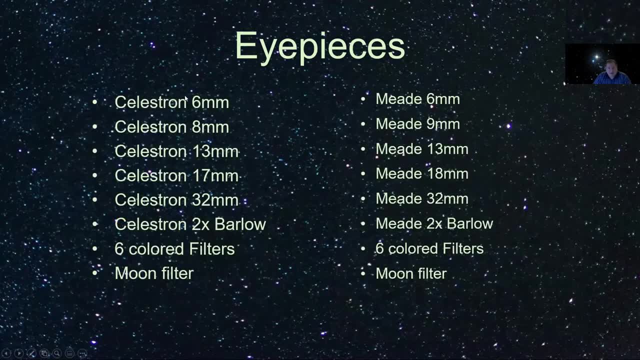 these are two common eyepiece kits that a lot of people get. if they get a new telescope They go out and buy these kits. They come. Celestron is a 6 millimeter 8,, 13,, 17,, 32 millimeter 8.. 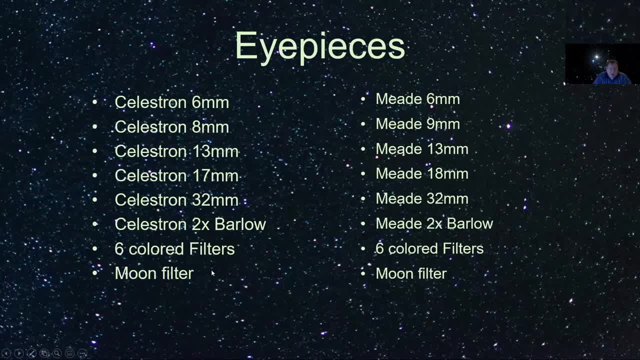 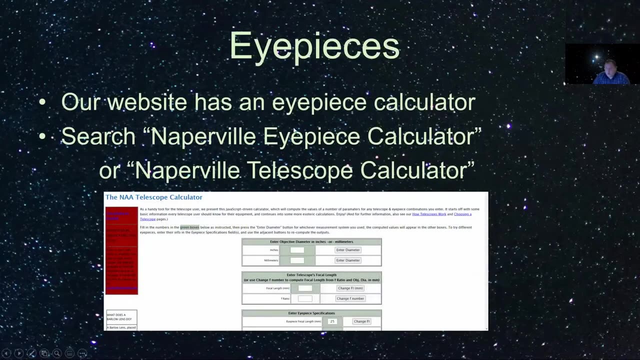 A 2X bar low, six color filters and a m frosting and the feeds a very similar. It's got a 9 millimeter and a 18 millimeter instead of the 8 and the 17.. Our website actually has this eyepiece calculator, so if you google or search, 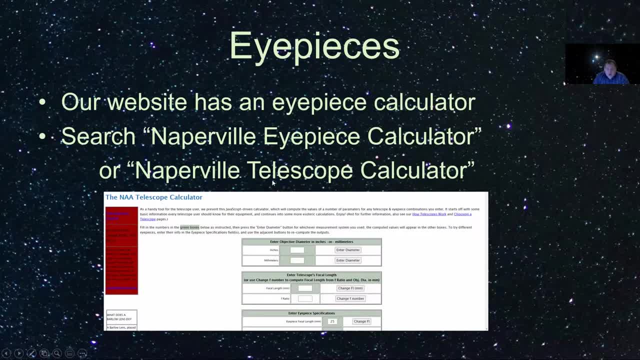 for the term Naperville eyepiece calculator, Naperville telescope calculator, you'll find this site site and you can put in the parameters of your telescope and put in the parameters of an eyepiece that you might be thinking of purchasing and it'll. 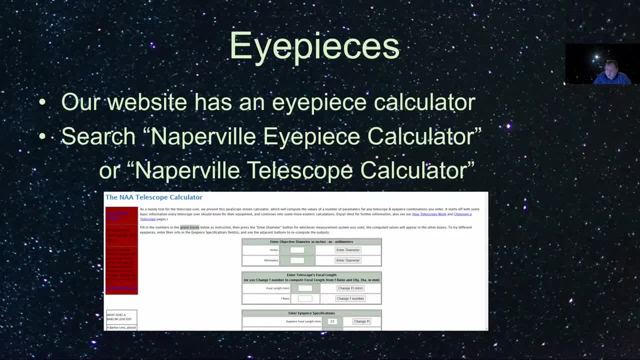 it'll kind of kick out some numbers that tell you whether or not that eyepiece would be a good investment. There's it'll tell you the the power of the eyepiece. so if it's too powerful, if it's if it's magnifying the object too much, it might. 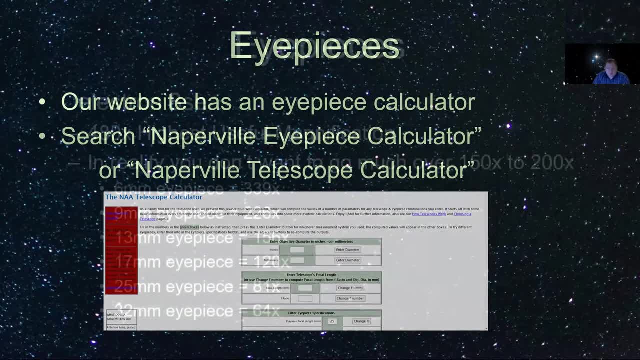 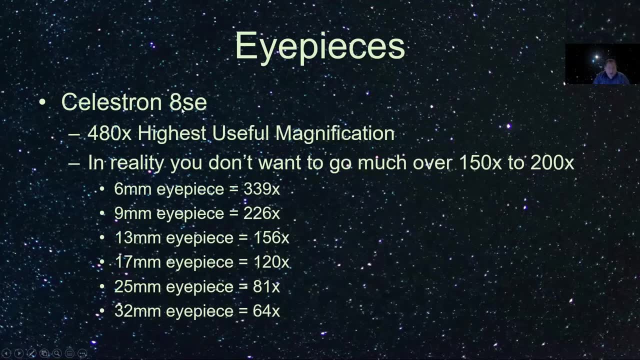 be, might not work very well for your telescope. So the Celestron 8SE is kind of a common telescope that some people buy, so I calculated the magnification for for these eyepieces. Now the the website for the Celestron 8SE says: 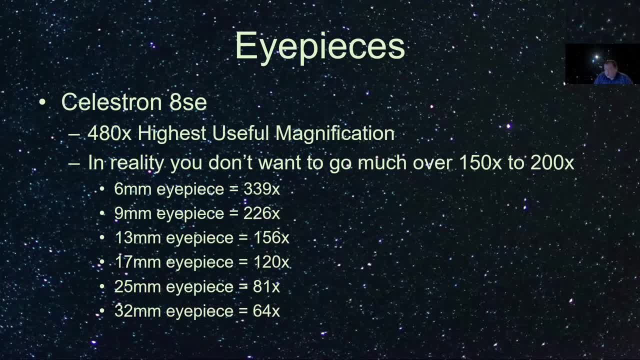 that 480 power is the the highest useful magnification That is, in absolutely perfect conditions, The the best nightly of the year you might have, you know, be able to get 480 magnification once. the whole time you use this telescope. So in reality most people try to keep it. 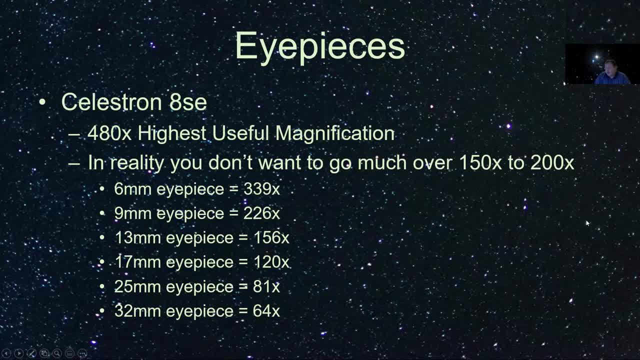 around 150 to 200 power. You know, once you start getting over that the objects dim quite a bit, and this is this is more of the sweet spot- to not exceed this. So, as you can see here, like, a six millimeter eyepiece is going to be 339. 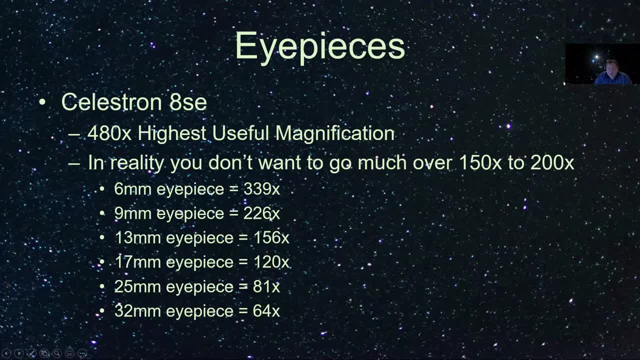 power. So you can see here that the Celestron 8SE is going to be 339 power. So you can see here like a six millimeter eyepiece is going to be 339 power and a nine millimeter eyepiece is going to be 226 power. So both those eyepieces. 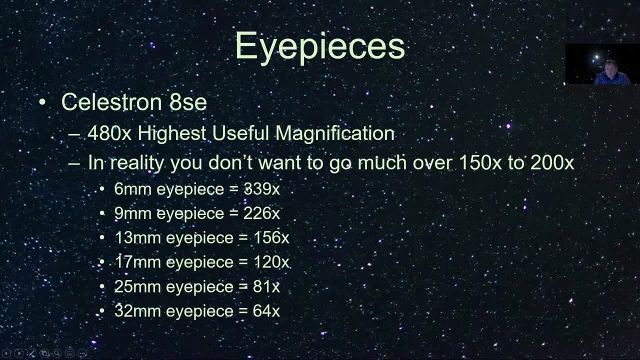 might be on on an average night a little too much for this particular telescope. So that's why that eyepiece calculator can kind of help you. So if you bought that kit that has these eyepieces in it, there might be two eyepieces that you 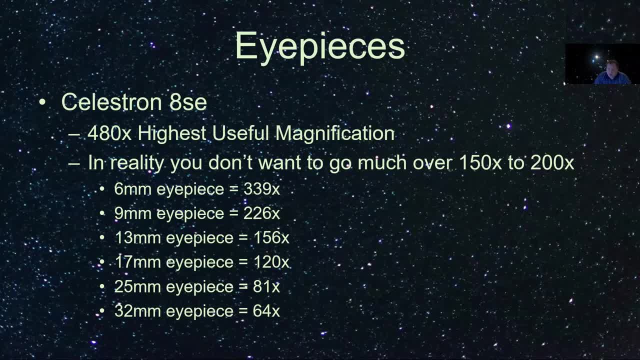 don't even use. So you know, it might be more beneficial to to buy eyepieces individually, to use that telescope, that calculator to figure out what what the best eyepiece to use is, instead of buying the kit. The kits are nice, but there's, there's parts on the kit that will 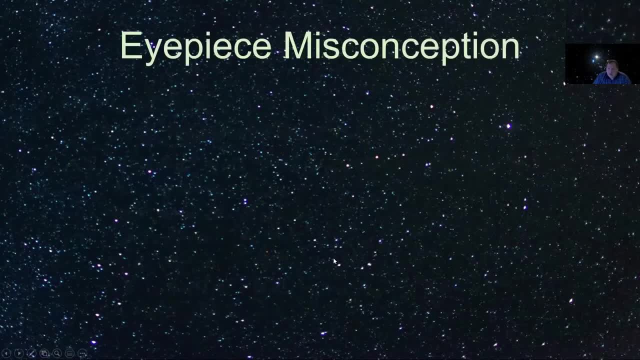 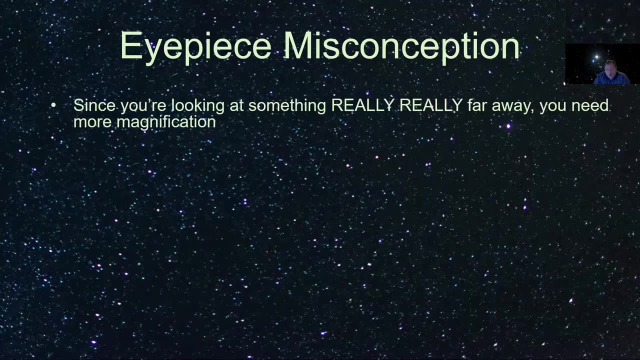 probably go unused. A big misconception on eyepieces is: since you're looking at something that's really really far away, you need to magnify that more. So you're looking at a galaxy, that's that's, you know, two million light-years away. you must have to magnify that. you know a lot just to see that. and the reality is. 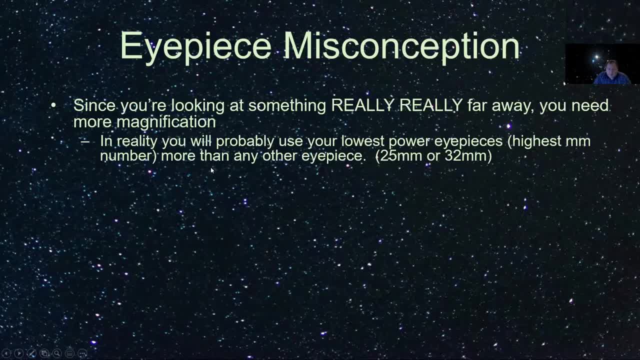 that's. that's not true at all. If you have like a 25 millimeter or 32 millimeter eyepiece- the 25 is what typically comes with your telescope- you'll probably use those two eyepieces more than you'll use your low-power. 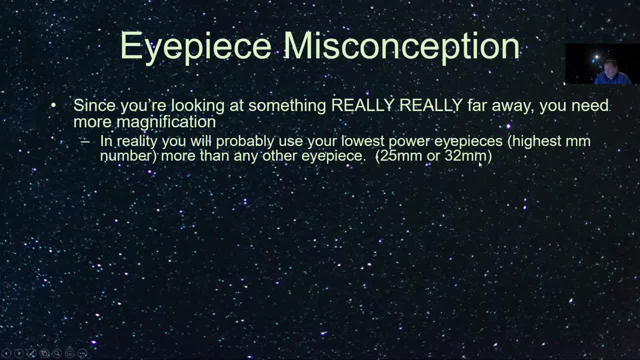 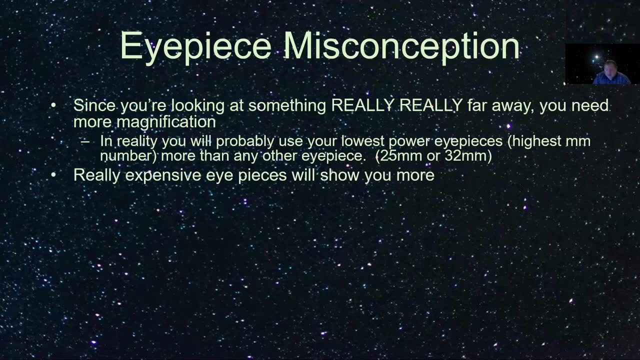 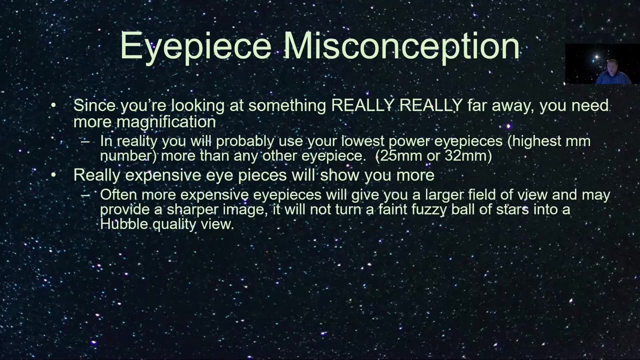 eyepieces. So if you're buying eyepieces separately, you know really focus on kind of a higher magnification, because you'll probably get more use out of that. Another misconception is that very expensive eyepieces are going to show you more Often. the more expensive eyepieces will give you a larger field. 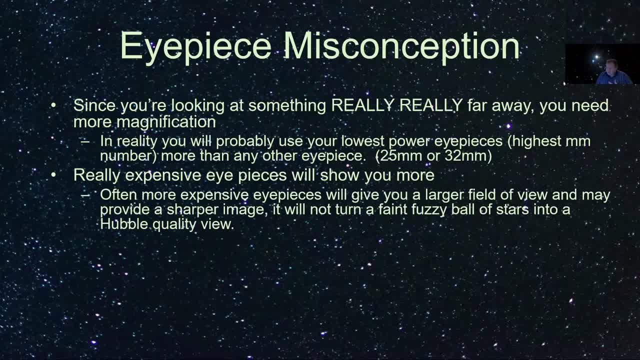 of view or might provide a little sharper image. It's, it's deep down, it's better glass. it's, it's, you know, it's not something that's mass-produced in a way, that's, you know, in a cheap way. So these things will look a little bit better. but if you were looking through, 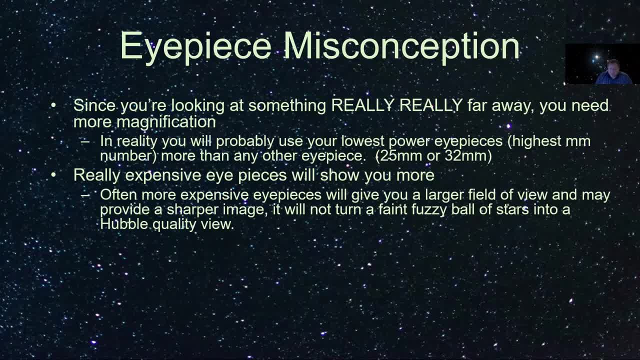 your telescope and you see something and it's. you're just barely able to see it. it's kind of a little fuzzy ball of stars. if you go out and buy a $500 eyepiece, it's not going to be 500 times better. it's good, you know you're. 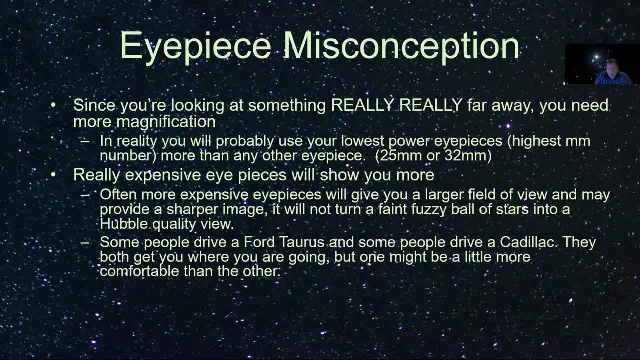 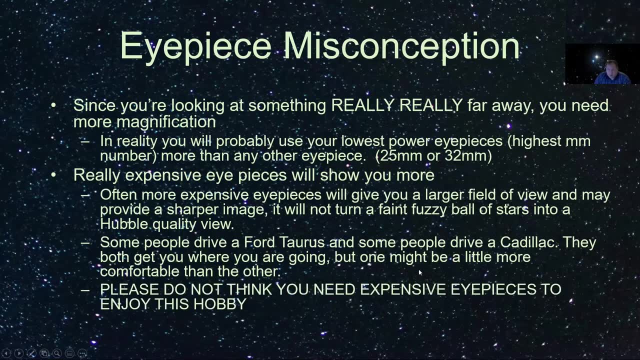 probably not going to notice the difference that that much deep down. So you know, think of it as some people drive a Ford Taurus and some people drive a Cadillac and they both can get you where you're going, but one might have a little more leg room and be a little more comfortable to drive. So do 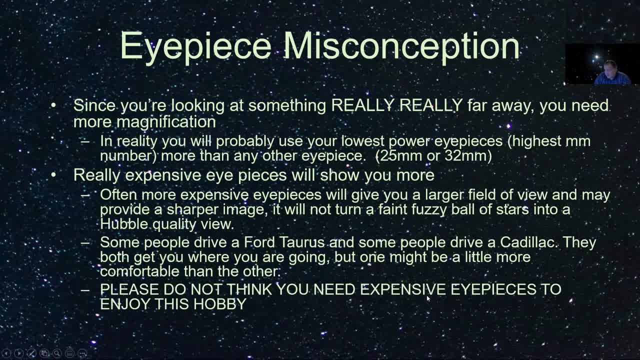 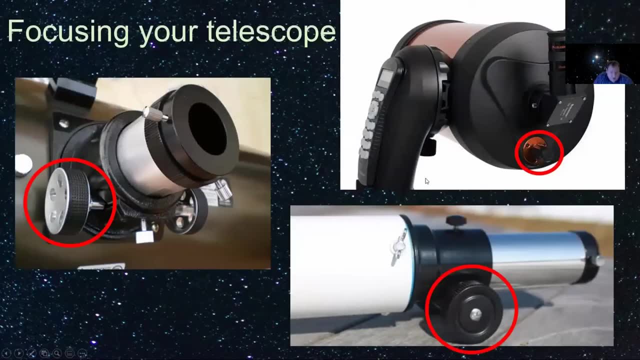 not think that you need to buy expensive eyepieces to enjoy this hobby. The eyepiece, the 25 millimeter eyepiece that comes with your telescope, will probably do the most of the heavy lifting that you need Focusing your telescope there. 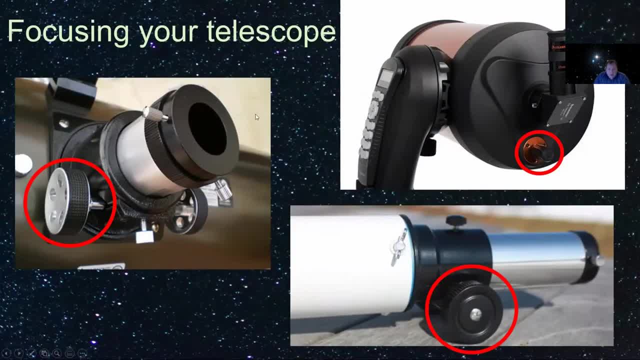 are. it's either going to be a knob or a wheel. so then the top, top right is a smith-cassegrain And it's got a focusing knob and that actually adjusts the internal mirror and moves that mirror around The bottom bottom. most telescope is a refractor and 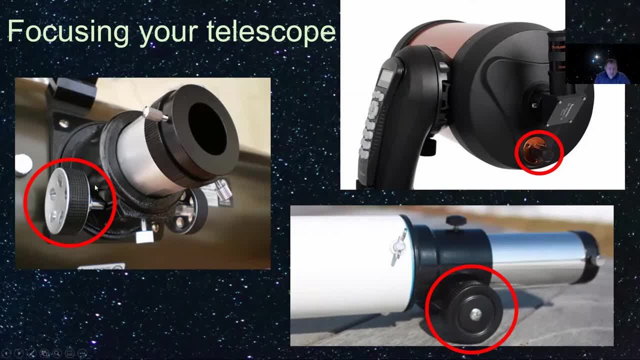 that's actually going to move the eyepiece in and out. and the same with the Dobsonian on the left. it's going to move the eyepiece in and out And as you move that and get your the object into focus, that's focusing right on your, your. 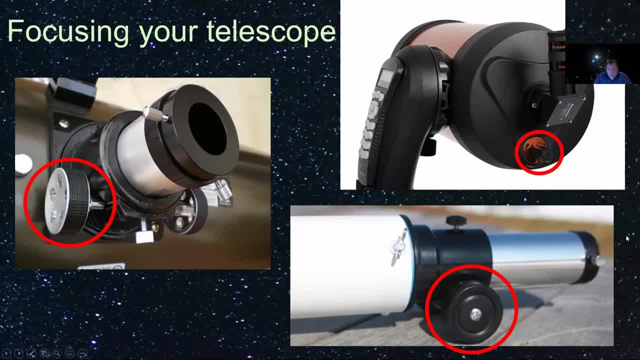 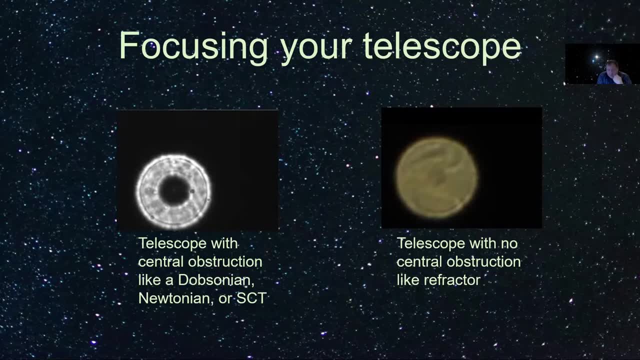 pupil to give you the most optimal view. So when your telescopes not in focus, it's going to look like one of these two things probably, if it's way out of focus. So the one on the left would be from a telescope that has a central obstruction, like a Dobsonian or 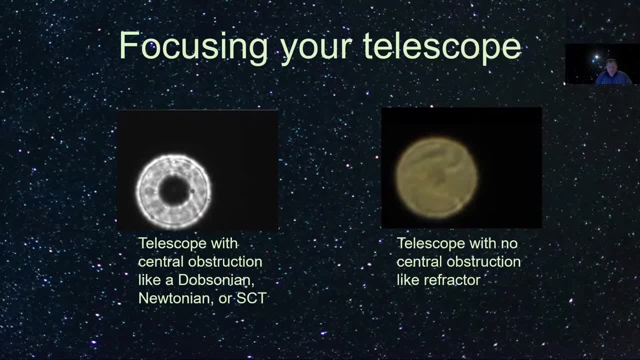 Newtonian or smith-cassegrain, It's going to look like a doughnut. The one on the right is going to look like a- you know, a plate And when you're focusing you turn that focusing knob. if the object gets, if this doughnut gets bigger, you're going. 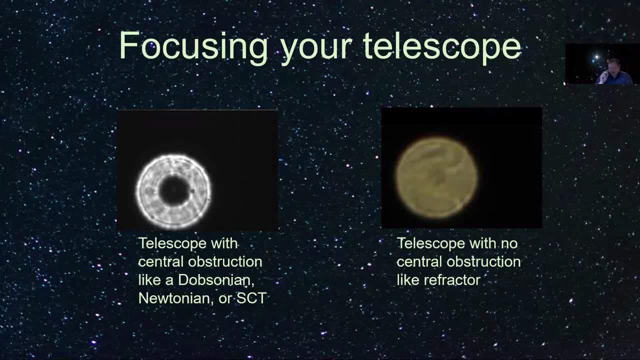 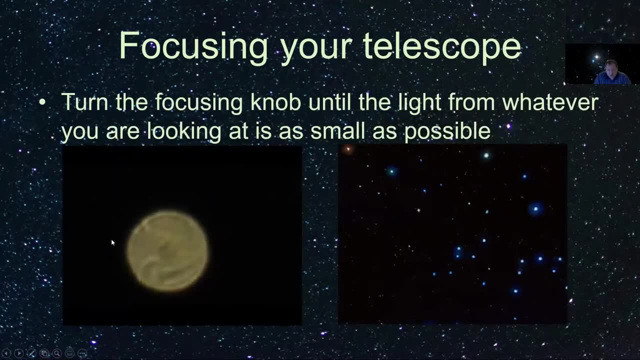 in the wrong direction. So you want to keep focusing until this gets as small as possible. So, again, you're going to take this, this larger disk, and you're going to turn that into a kind of more of a pinpoint star, and that's how you know you're. you're really 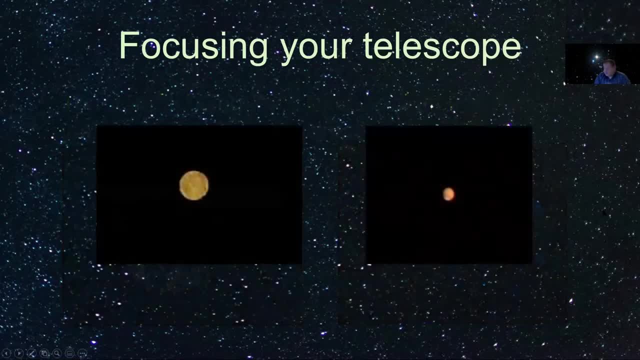 in focus And everybody's eyes are different too, I should point out. So you might focus for you and then you let somebody else look through it and it might be a little bit blurry for them, So they might have to focus themselves. So, like the planet Mars, Mars is really tough to see most of. 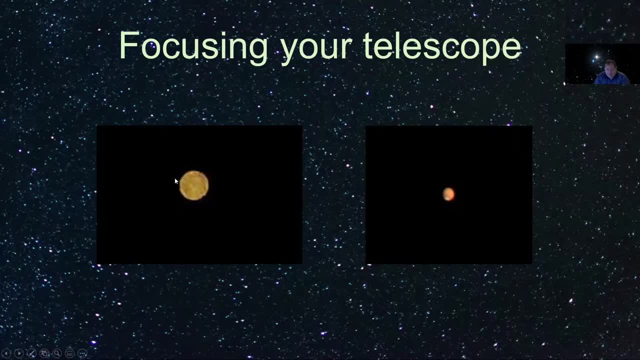 the time Tough to see detail, But if you have a big, you know a great big Mars, that's probably not Mars. Mars is going to be really tiny and in most telescopes But it's going to have kind of more defined edges. The an unfocused 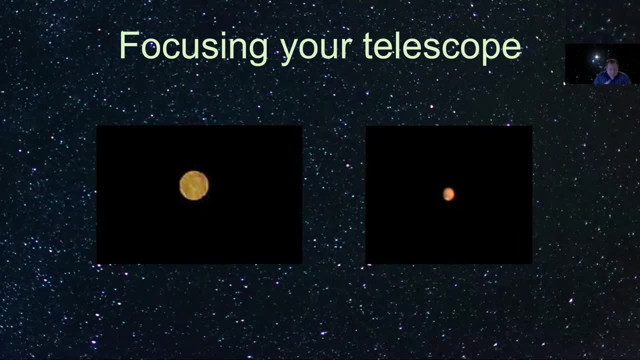 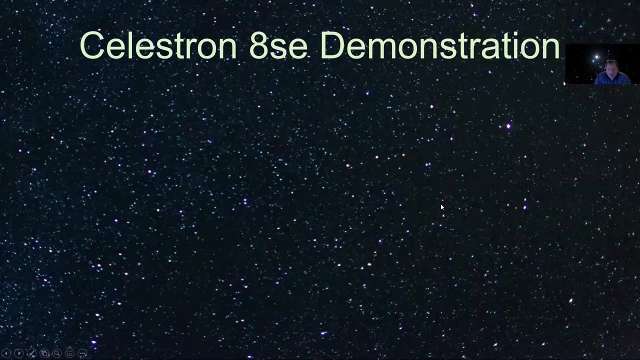 image will be more like a kind of an amoeba, that's, you know, jumbling around the telescope. Okay, so now I actually have a video, and this is me setting up a Celestron 8SC telescope. I'm going to set it all the way up to the point where I align it on 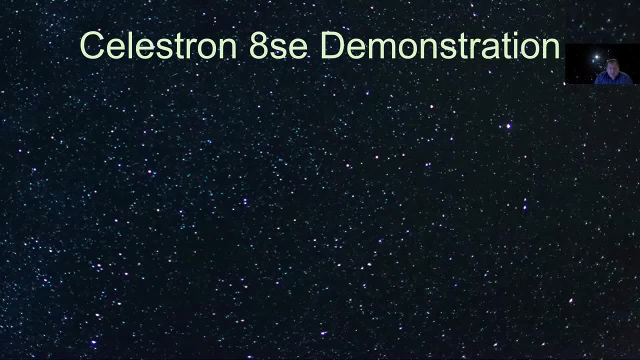 the planet Jupiter And hopefully this will help anybody that has this type of telescope to align it for the first time. These videos will be available on our Facebook page and on our YouTube page later on. So if you're, if you do have an 8SC telescope, you can watch this a few times if you, if you need some. 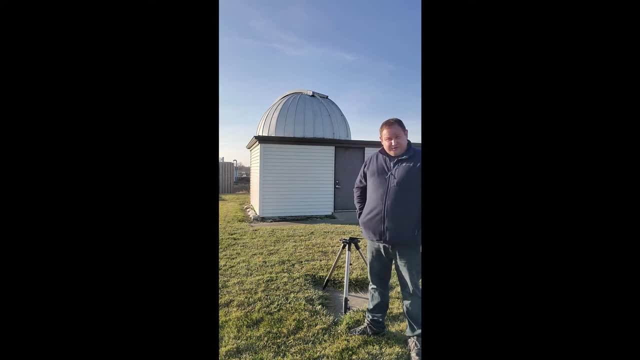 some help getting set up. Hi, I'm Jim from the Naperville Astronomical Association And I'm going to show you today how to set up your Celestron Nexstar telescope. So here we have the mount. The first thing I would suggest is: you want to get? 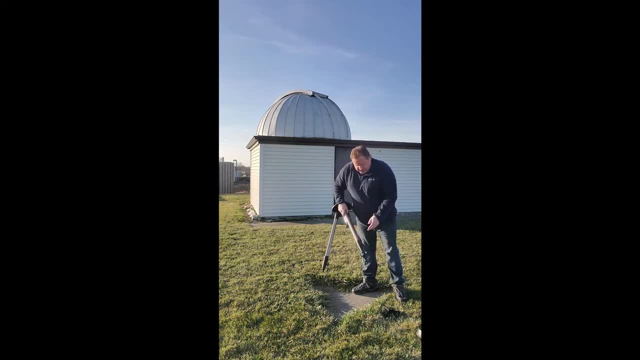 get the telescope to a comfortable height. So I'm going to- I'm going to take all the legs out, probably about halfway out. It's good for my height. You also have to think about who else is going to be looking at the telescope. If you're going to have kids, you might want it a little bit shorter. 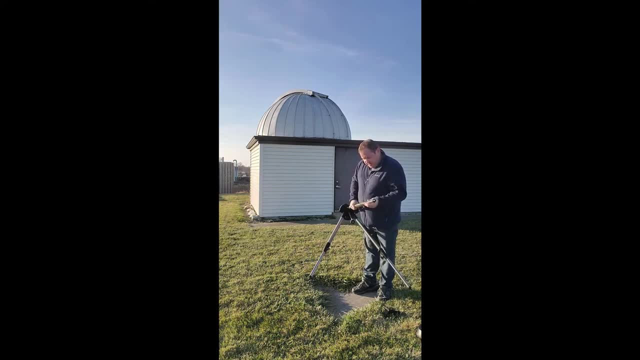 or want to have a step stool, But I'm just going to eyeball these about halfway out. I'm going to set it up here. When you set it up, you want to set it up on something that's that's very sturdy, Something like a deck would be. 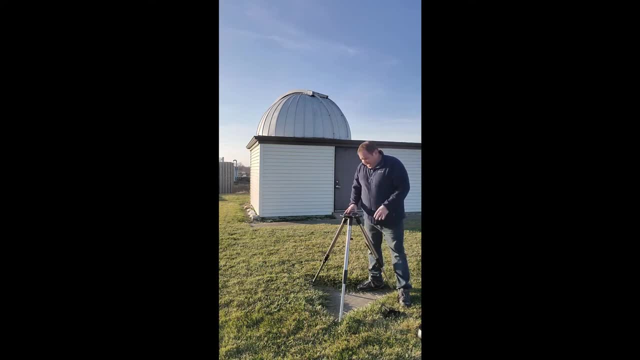 too wobbly, The ground is good, or if there's a cement pad, that would be good. And then your telescope comes with this little bubble level And I'm going to show you how we get this level. So the bubble level is a simple concept, but 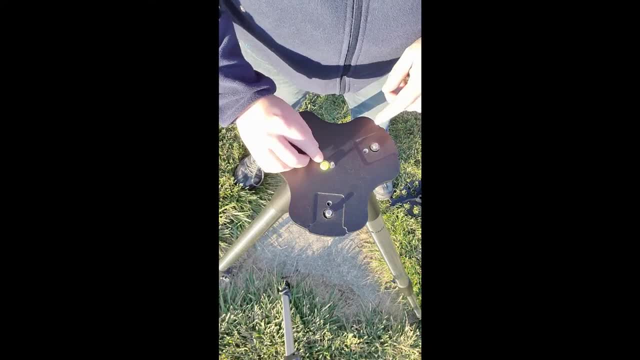 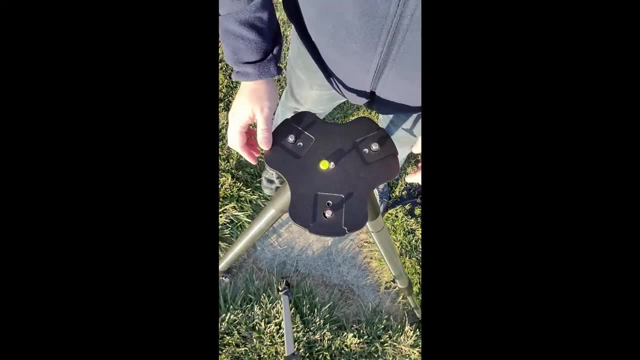 when you have three legs it makes it a little bit difficult. So you have this little little bubble in the center and you want that to be as perfectly in the center as possible. So you set it down on your tripod As you lift a leg. 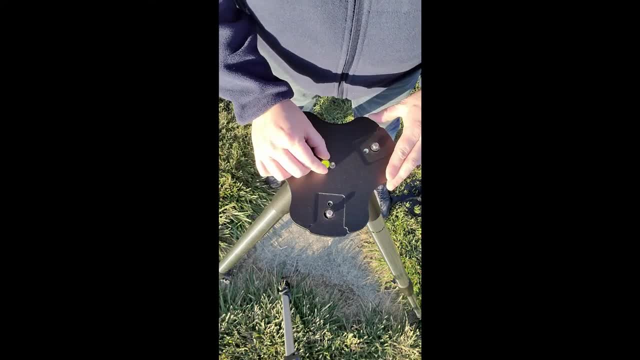 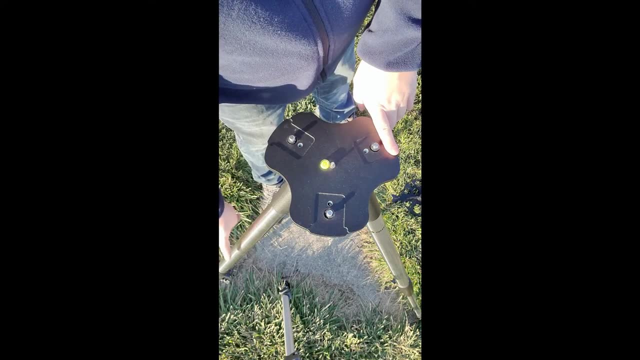 the bubble will go towards that leg. So the way I have it placed right now, it needs to go this way, which, of course, is in between two legs. So what I'm going to do is I'm going to lower this leg a little bit and see if I can get that. 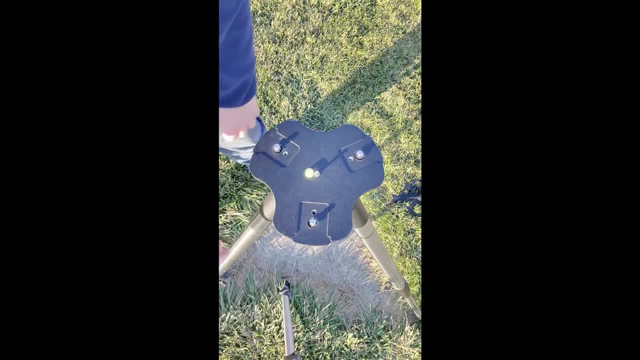 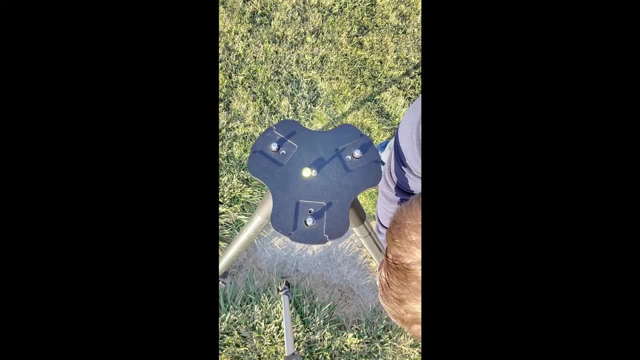 bubble to go more to the center. That's fairly good. I'm going to raise this side just a little bit And I think that's a pretty good. I'm not going to pull the bubble level off yet because I need to put the 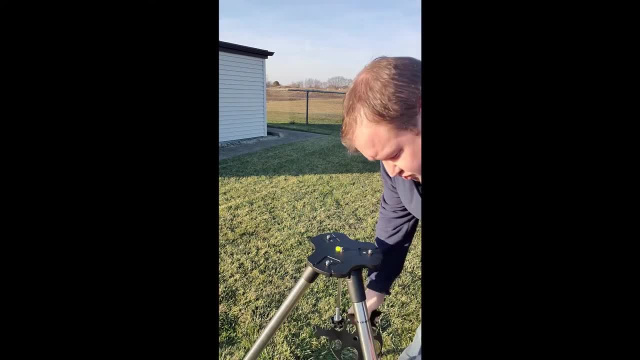 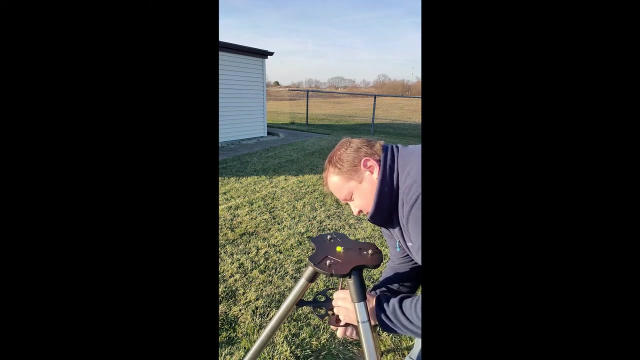 the eyepiece tray on. Now this also acts to keep the legs out at the same distance. So as I do this, it might actually kick the telescope out a little bit, and which would force me to re-level it. Okay, so in my case it didn't change the level at all, so that's pretty good. So I'm. 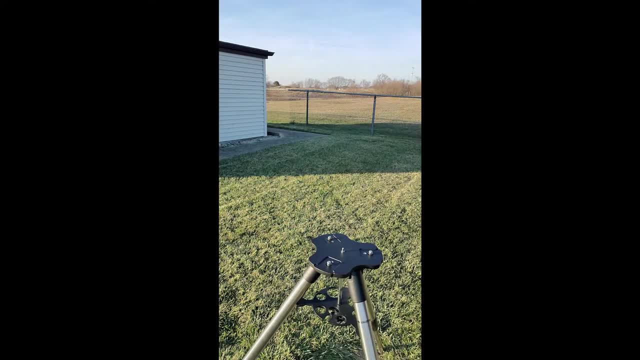 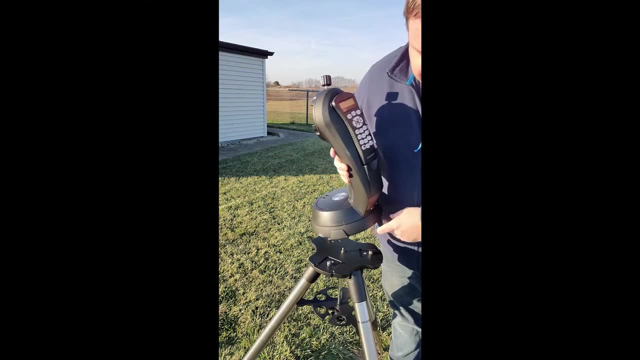 going to put this back in my pocket or in my eyepiece case and we'll move on to the next step. Okay, now we're going to be placing this on. This is all the gears and motors that that help track this, The easy way to figure out how this goes. 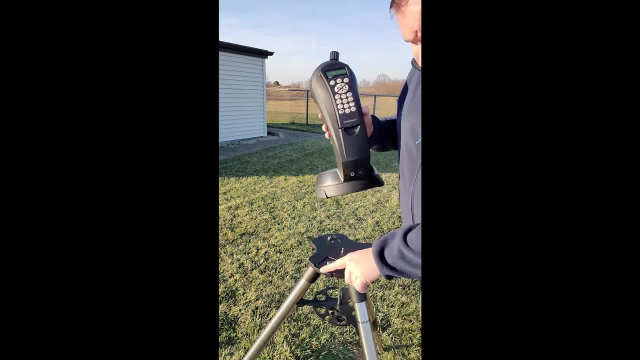 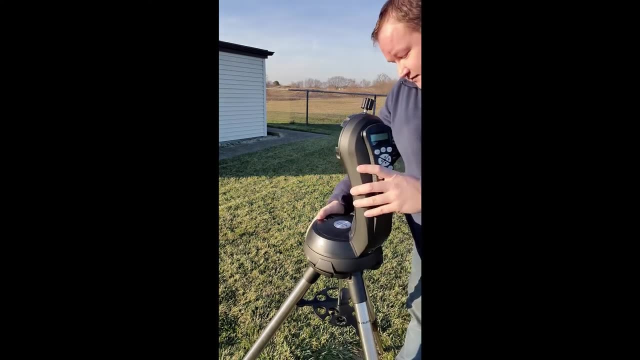 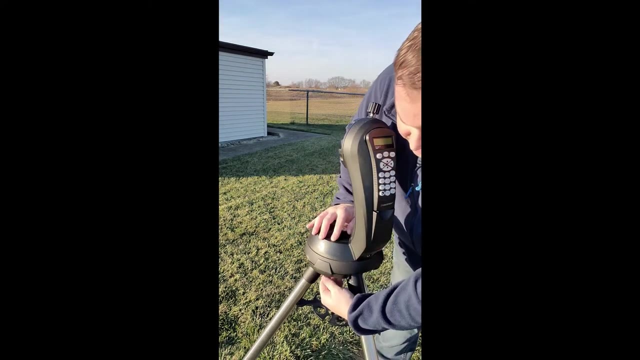 it's got these little bumps that come out, and those bumps would be in line with little bumps on the on the mount. So, as I put that on, you want to be careful not to drop this. but there's a little pin and once it snaps in place you'll feel it. And then you have three sets of screws You want to. 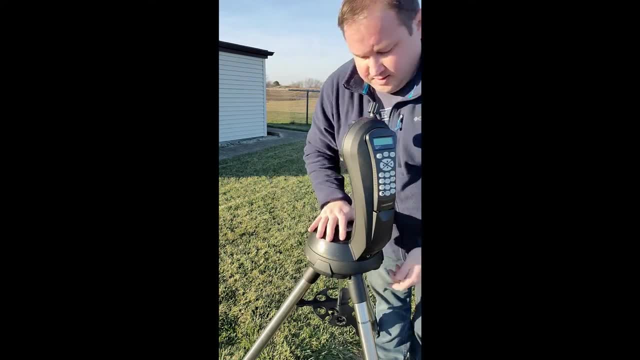 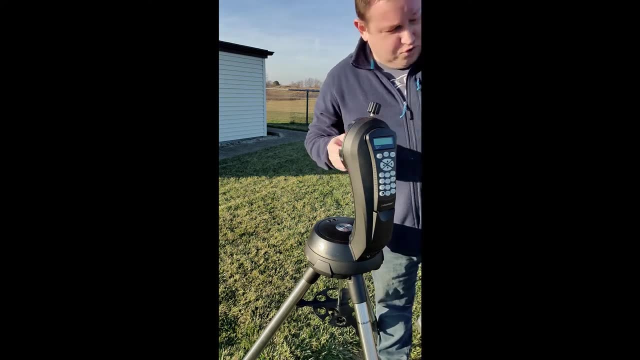 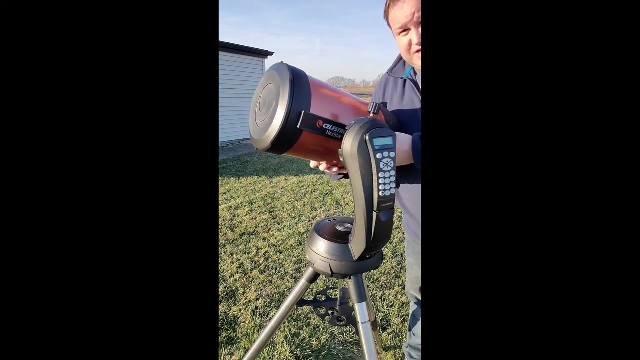 screw those on completely, Okay, and then now I'm going to put the OTA on the optical tube. So this, you need to be very careful. This is an 8SE, So this is an eight inch. You want to get a good, good grip on it, Get it. 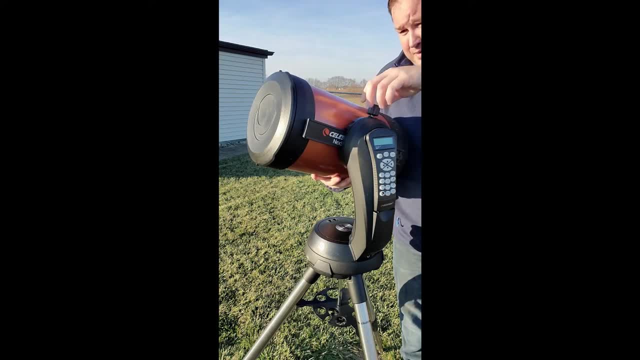 about in the middle and then tighten this knob on top and really make sure that it's in all the way before you let go, Because if you let go this is going to bounce off the ground and there's mirrors and glass and stuff in there. that's not going to work right afterwards. 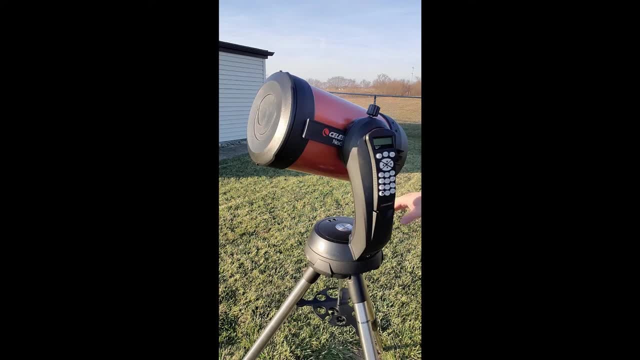 So there's four different ways to power the Celestar Nexstar telescope. There's batteries that you can put in here. You can use an actual power adapter which would plug in down here. There are kind of these older style battery tanks. This uses a nickel cadmium battery, So the bad thing about these is if you run it below. 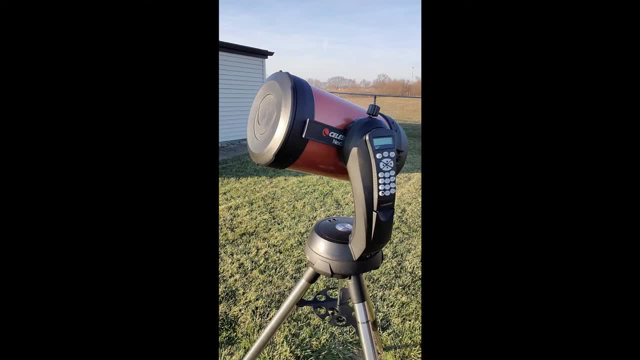 50%, it's not. it kind of isn't good for the battery. things that have come out are these power tanks that use lithium-ion batteries. You can run these completely dead. They can recharge like over 2,000 times and they actually run pretty well. So 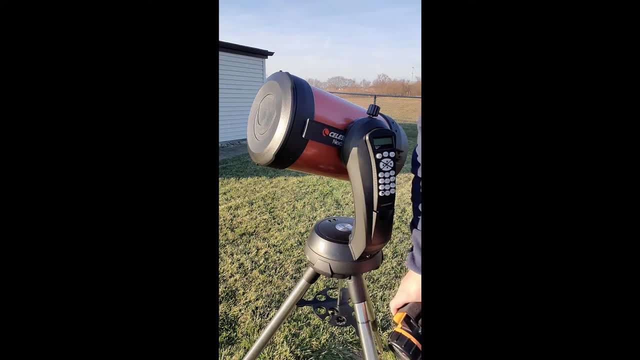 lately I've been preferring this, but if I'm doing it in my backyard I'll just use the power brick. The bad thing about the batteries is if you have batteries in it, it will default to the batteries first. So if you forget to take the batteries out and you try running it off of a different power, 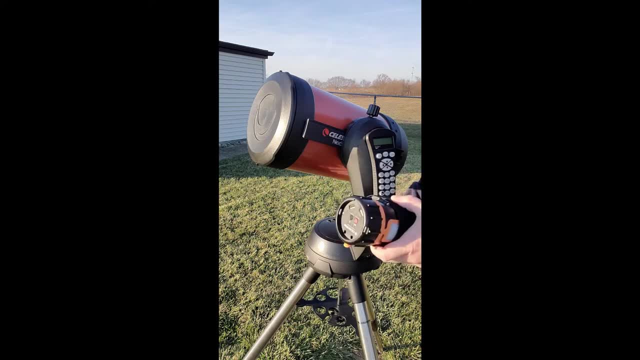 if these batteries go dead, your telescope goes dead, It's not going to automatically use a secondary power source, It's always going to try to use the batteries first. So most people that I know in the astronomy club don't really like the batteries. They're. 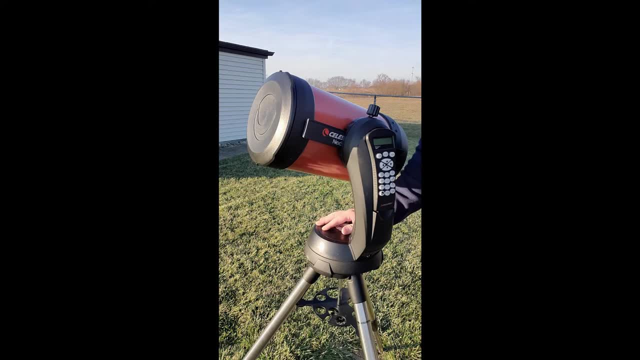 a little too finicky. So if you can help it, either plug it in with your power brick or get it out. It doesn't have to be a Celestron power tank. There's other power tanks you can buy, but typically people use some kind of power tank to power these. 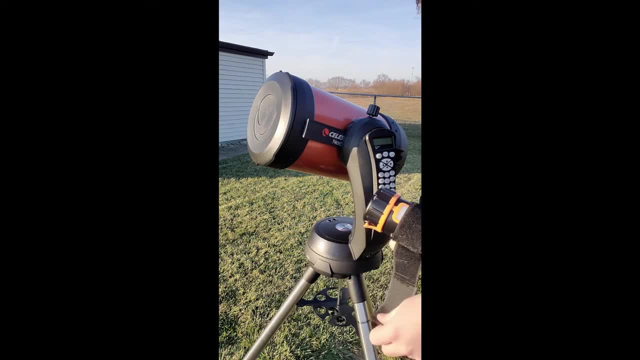 Okay, so I'm going to go ahead and use this power tank here. The nice thing about this is it's got a little wedge to wedge it onto your tripod leg and it's got some Velcro to wrap around it to keep that on your leg, And then I'll kind of tuck it a little bit to the side. This will use. 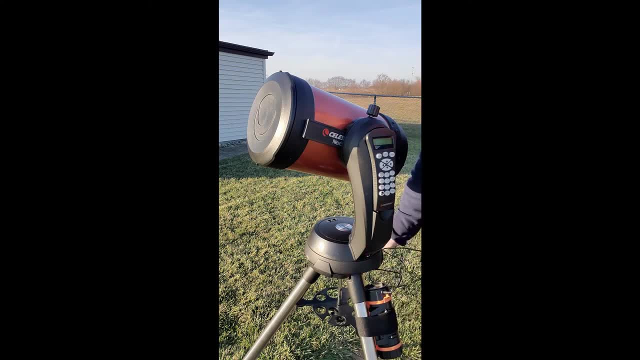 the power will go here, and then the power will go up here, And then I try to tuck the cables away, so nobody's going to kind of get stuck on them or triple them. Okay, so once this is ready, I do have to turn the power on on this power tank. Now, this one requires me to push the on button. two: 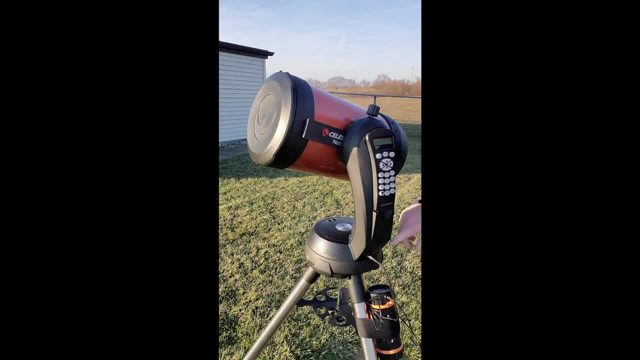 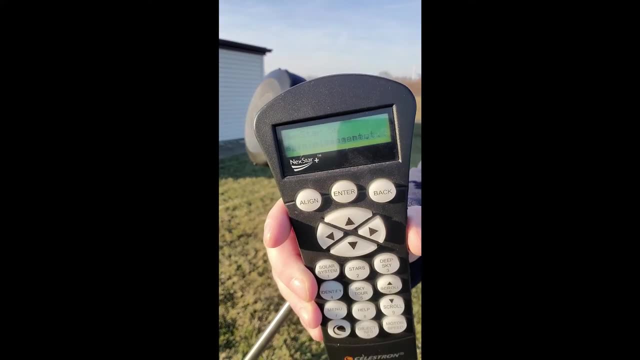 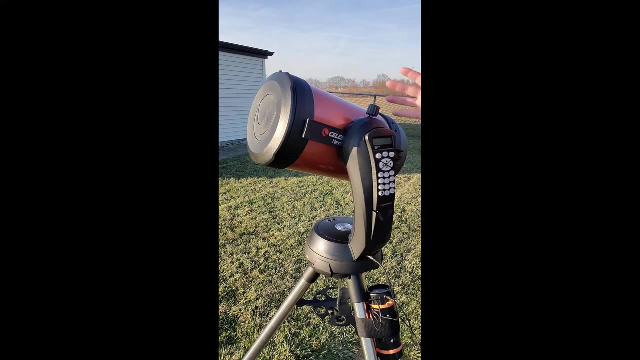 times. I don't know why they designed it that way, but once that's on, we can power on the telescope and the hand is now booting up. A really big, important step that you want to do before you start using this telescope at night is you want to align your finder Now. 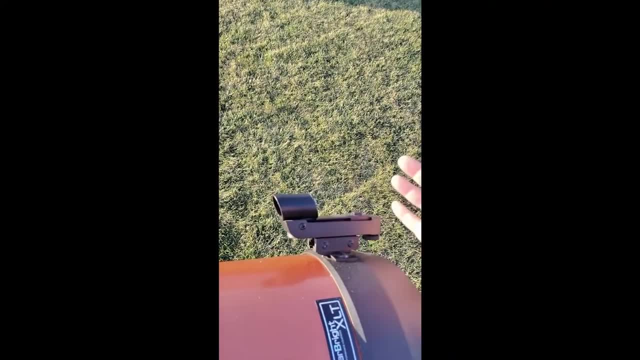 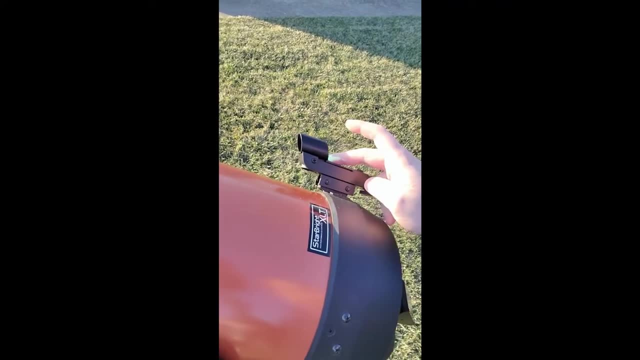 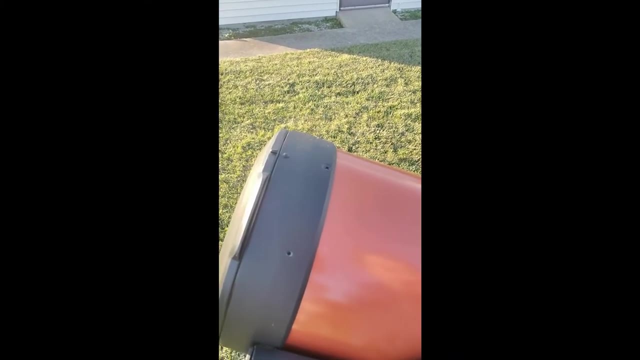 there's different kinds of finders. I'll go over that a little bit later, but the default finder that comes with this is called a red dot finder, and the concept here is: we want this and the telescope to be looking at the same thing. By default, they're not going to look at the same thing, because if 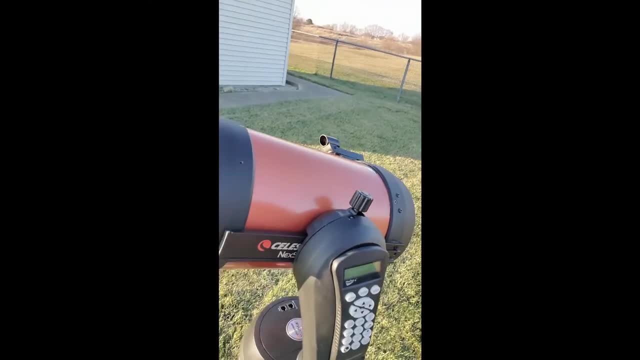 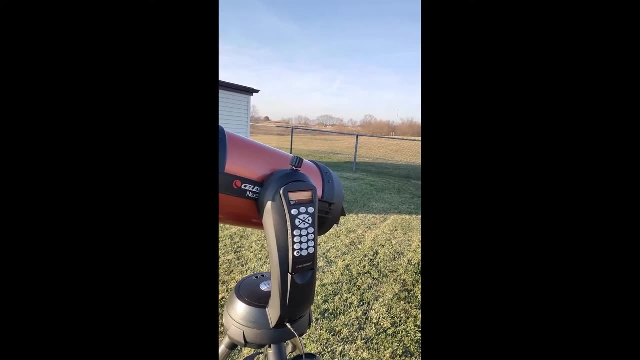 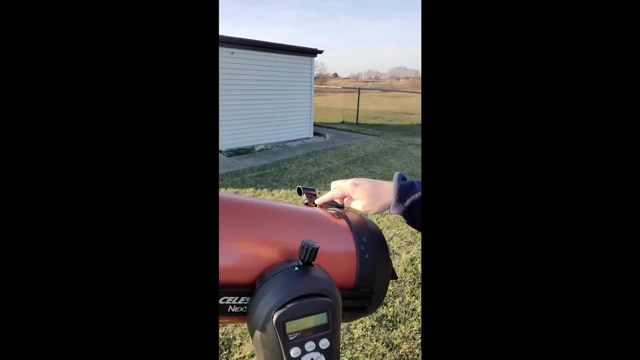 the screws are tightened slightly different, it gets off. So what we're going to want to do is point the telescope to something off in the distance, and then we'll try to get the telescope looking at that thing, and then we will try to get the finder looking at that same thing, and then we'll 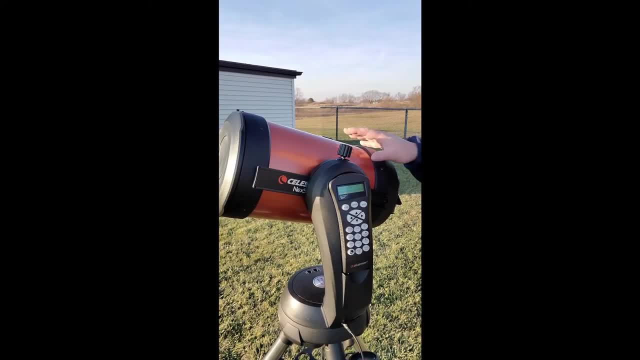 know that the telescope and the finder are aligned. This is a very, very, very important step. If you do not do this, you can point the finder at the moon and if the moon's off to the side, that, you'll never find it in the telescope. So this is a very important. 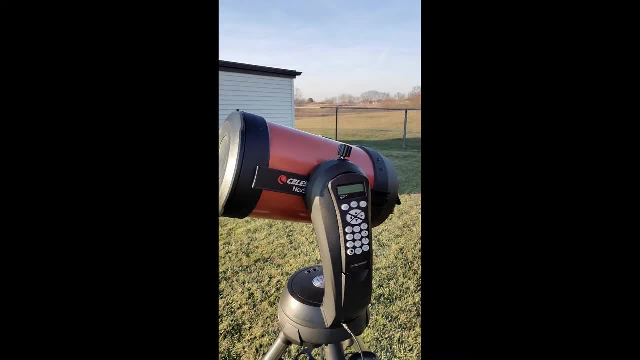 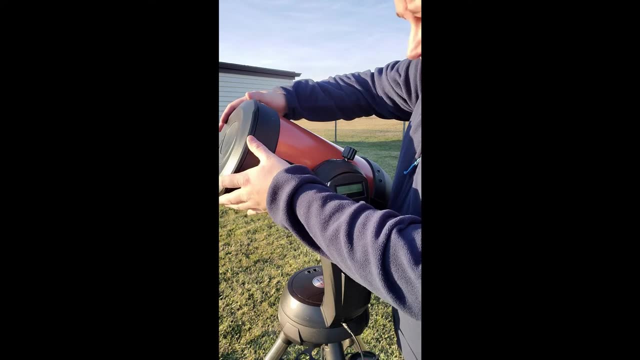 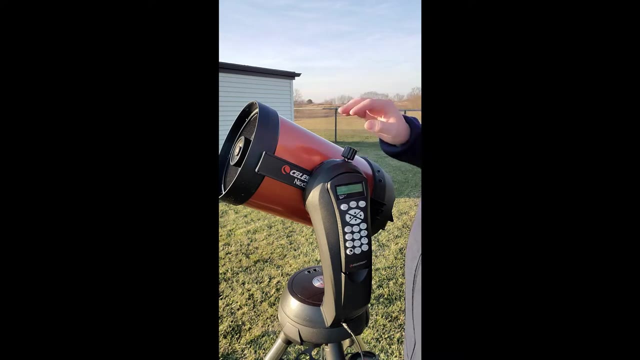 step, and a lot of people don't do this step when they get these telescopes out of the box. So before we move the telescope to align the finder, we want to make sure we take the cap off. You'd be surprised how many people go out some night and have trouble and can't figure out what's. 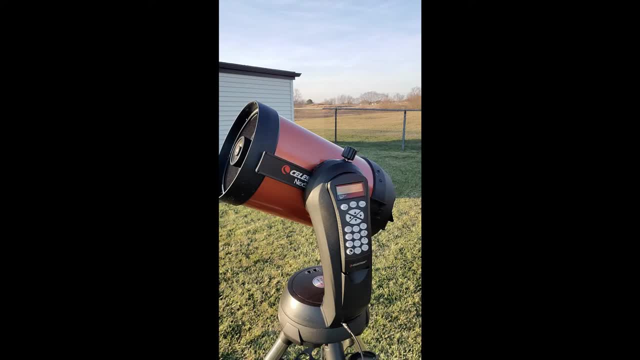 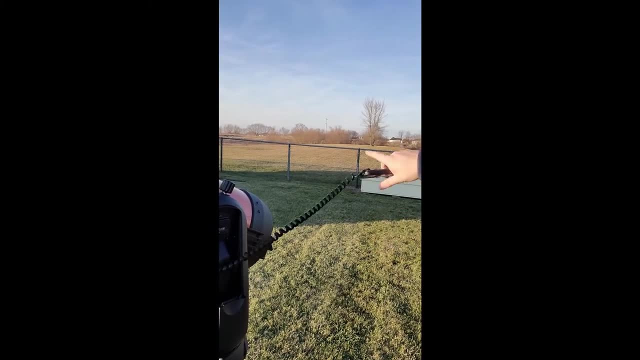 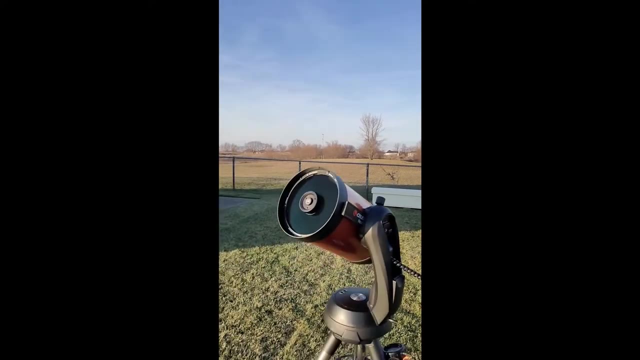 wrong with their telescope and they forget to leave the finder, They forget to leave the telescope it and leave this on. So a good place that we can go is to this electrical pole off in the distance. So what I'm going to do is, using the hand controller, I'm going to turn the 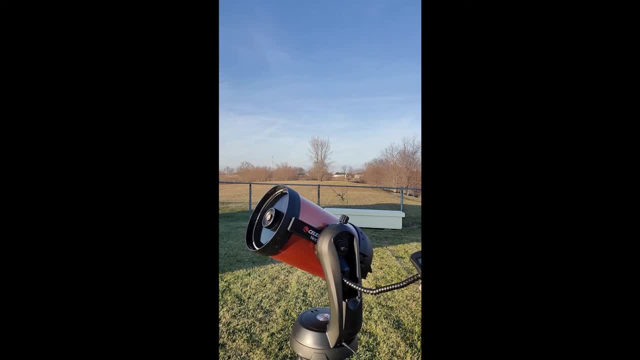 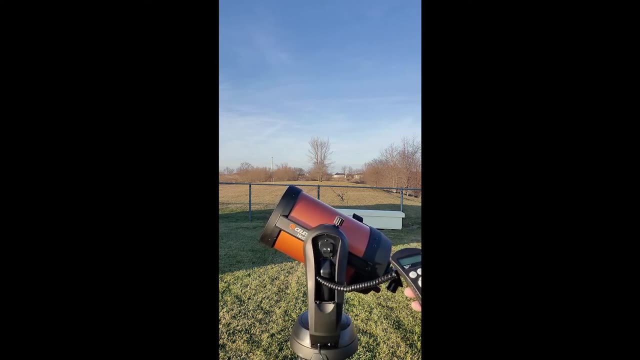 telescope around and point at the very top of that pole. You probably want to do this during the daytime hours. It's a little trickier to align this at night. It can be done, but it's a little bit trickier. But what I'll do is I'll try to get it in a general area. 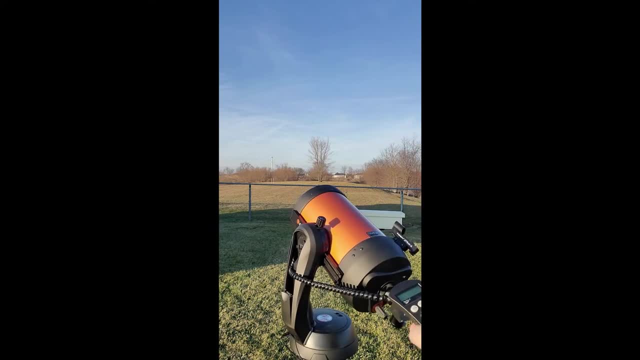 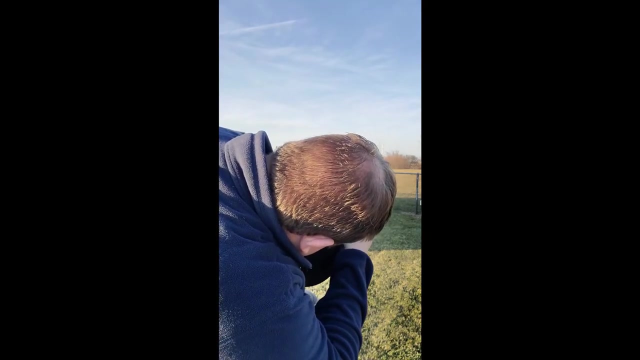 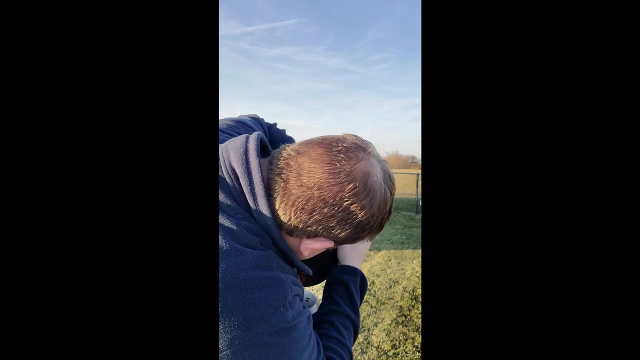 I'll go down to the trees, kind of scan back and forth, until I see the power line or until I see the tower, and then I'll work my way up. So here I go. Oh, it's actually very close to begin with, But by changing these two things, 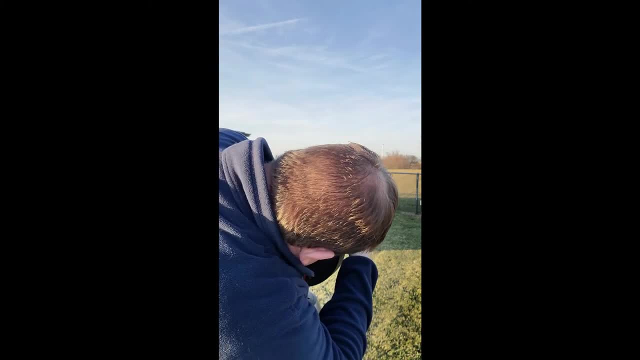 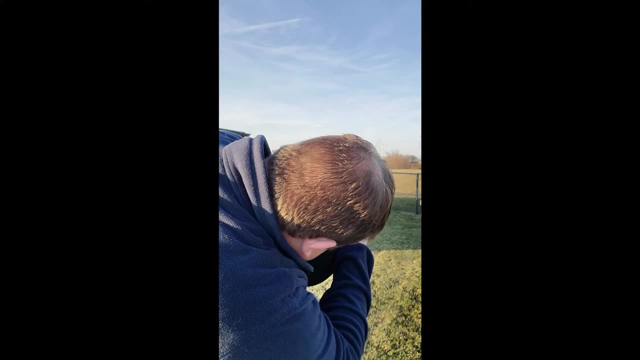 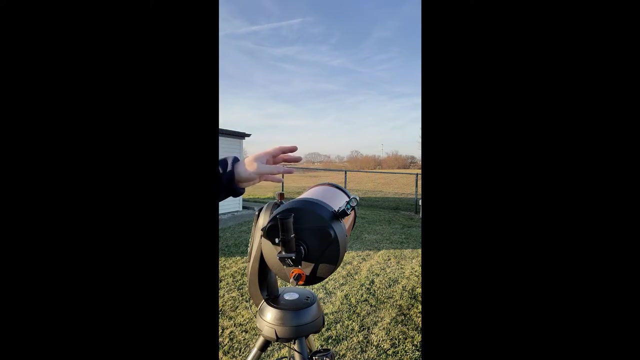 oh my, I find it was a little loose. By changing these two things, I'm going to get it to be the very, very top of the tower. If I look here, I'm still at the very top of the tower. So now this and this are pointed at the same thing. I cannot stress how important that. 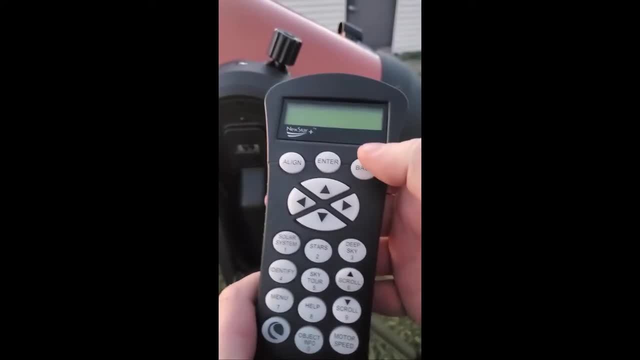 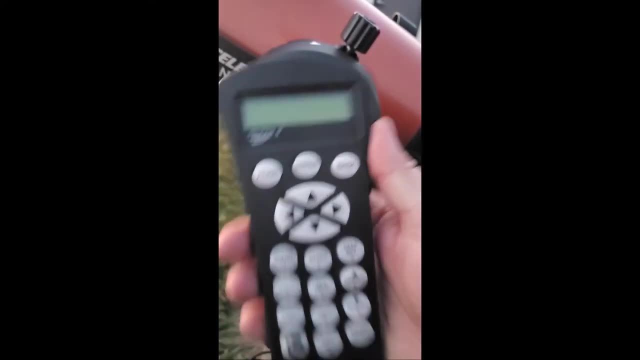 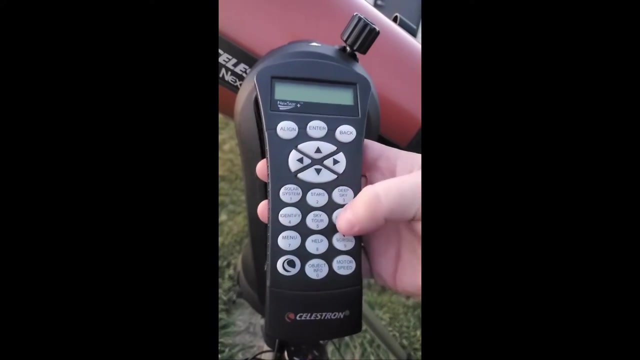 is over some of the aspects of the Nexstar telescope hand controller. I don't know why Celestron likes to change these up every once in a while, So depending on when you bought your telescope, some of the buttons might be a little bit different. They rename things. 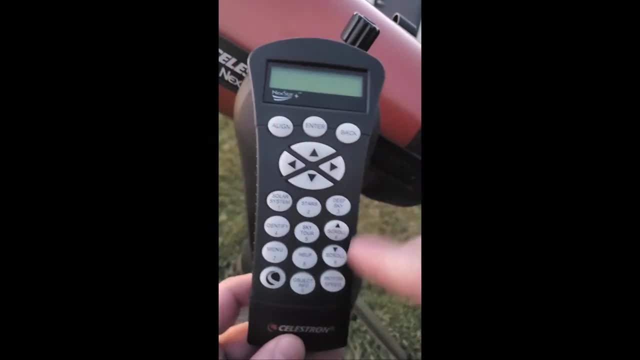 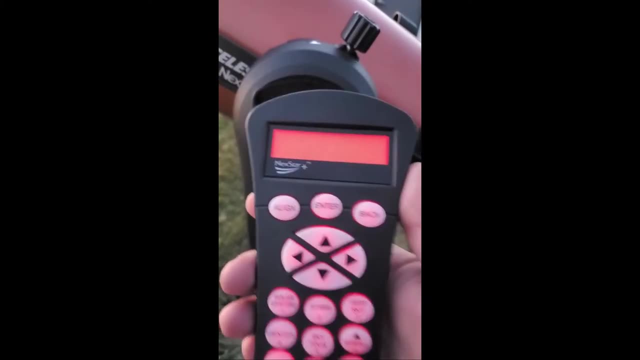 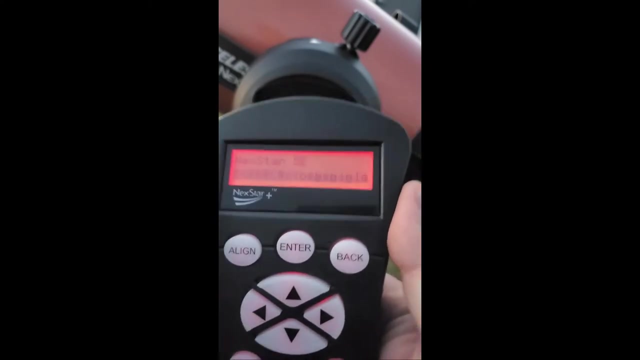 renumber things. So just because I'm showing you this, I'm not going to do that. I'm just showing you this way. Read the button. Don't pay attention to what numbers I'm telling you to do. As we turn it on, it starts up. The whole brain of the telescope is in this. 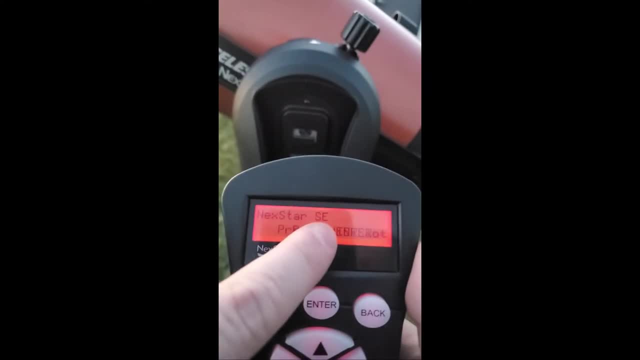 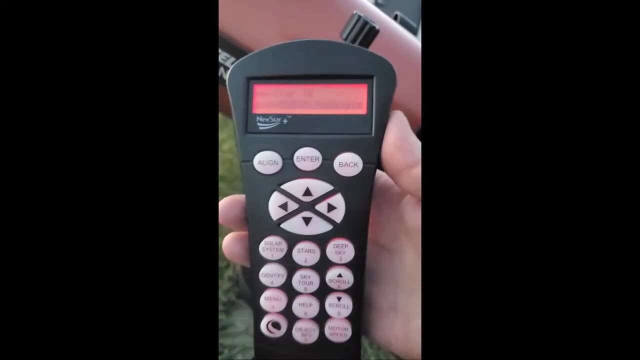 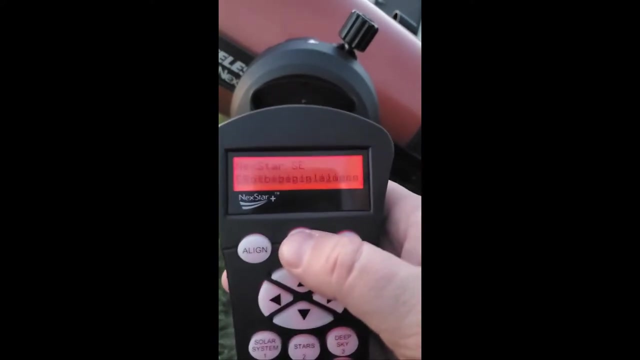 hand controller. So this is the Nexstar SE That stands for second edition. If you have a Nexstar Evolution, these will be very similar but maybe slightly different. The first thing it tells you to do is press enter to begin your alignment. We're going. 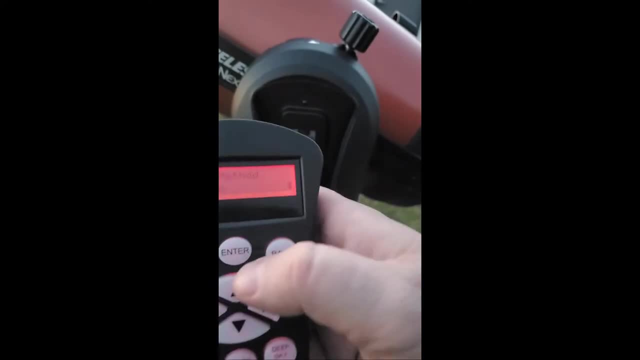 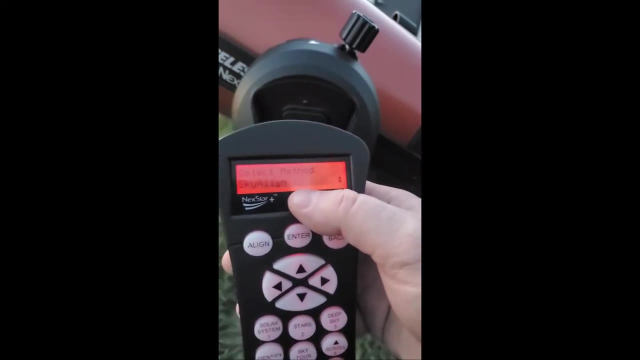 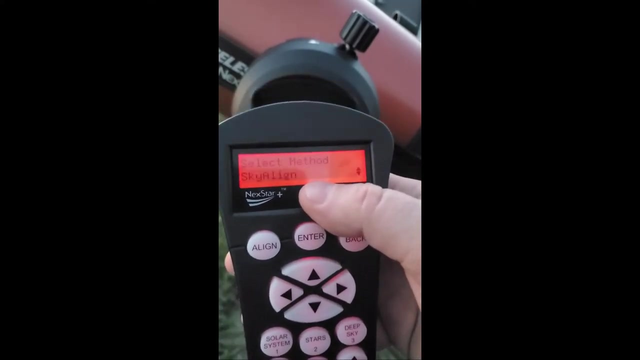 to push enter. It's going to ask you what kind of alignment you'd like. So sky align is supposed to let you pick any three bright objects, any three bright stars. They could be stars, They could be planets, It doesn't, it doesn't care, And the hand controller is. 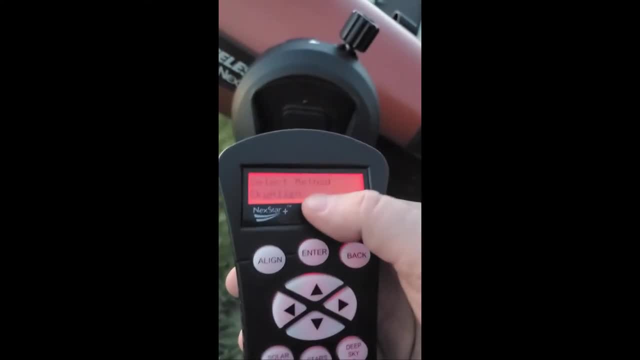 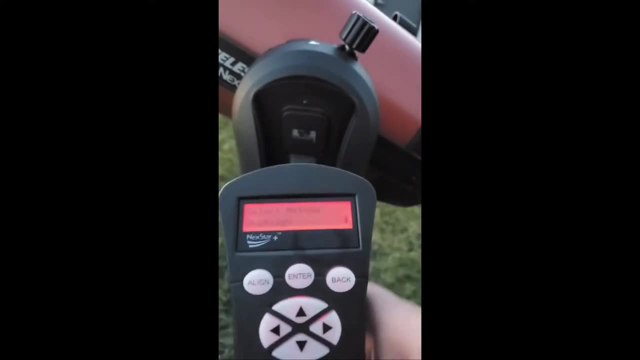 going to try to figure out where you are based on those three objects. I haven't had much luck with this personally. It fails a lot on me, So I haven't really tried it that much anymore, but certainly you can try it. There's some methods that I like a little bit more. 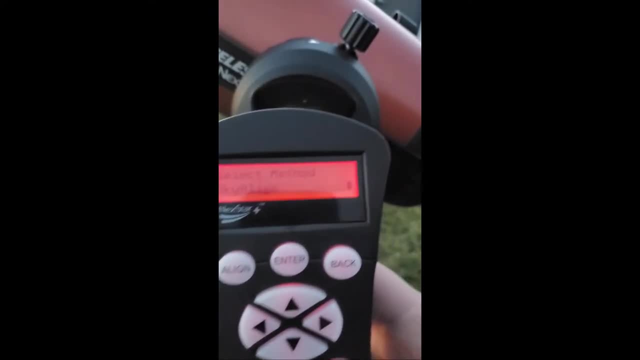 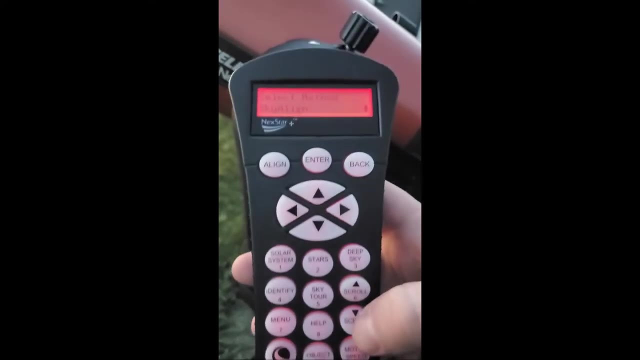 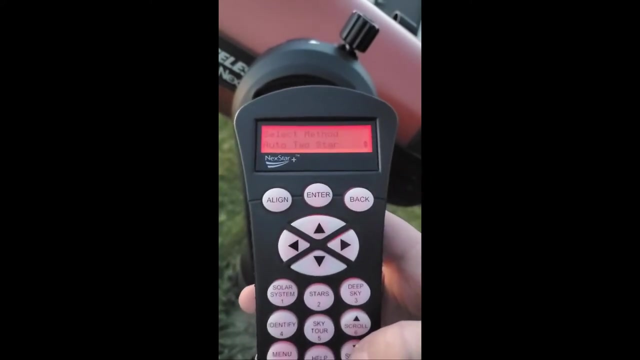 When it's when the, when it first gets dark, the only thing you can see in the night sky are the planets. So if you hit your, so these up and down arrows here are, is what's going to let you change. So auto two star. this is actually an alignment I like the most. 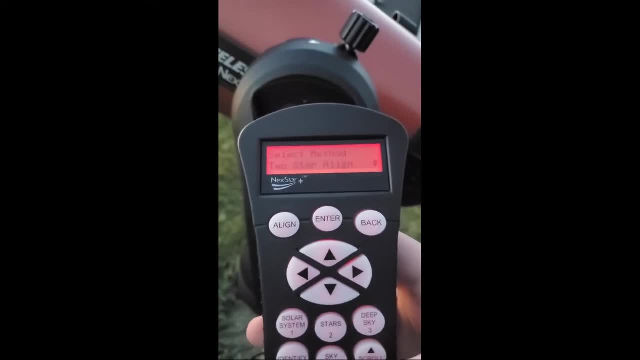 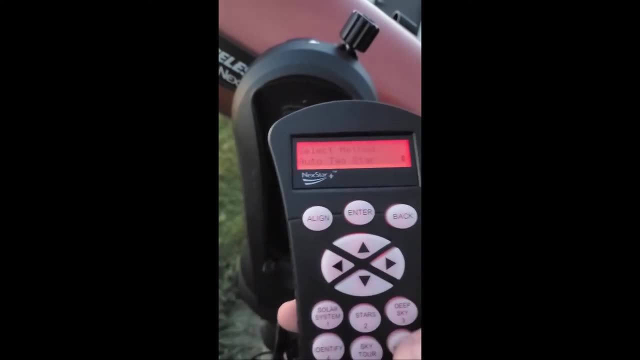 We can't do that until it gets a little bit darker, So we can go down two star line. Now this is different. So auto two star lets you pick the first star and then you tell it the second star and the telescope will get close to the second star, Close enough that you 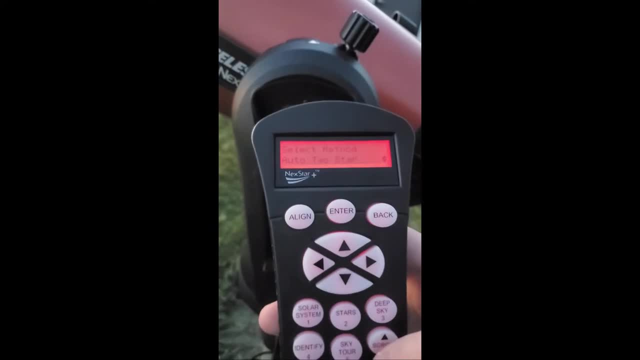 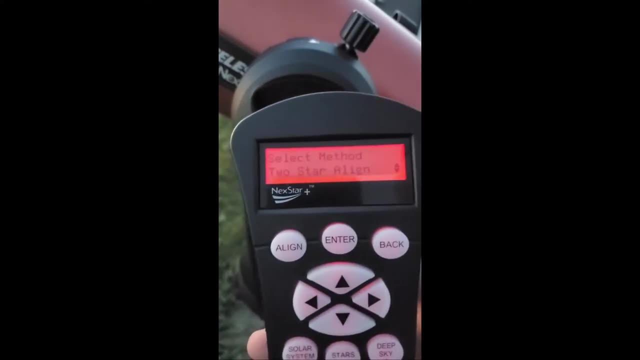 can probably figure out. you know, if you're looking in the sky you think: oh okay, there's only one bright star that's close. So that has to be the second star, Two star. you have to know the two stars that you're pointing at, So you tell it. 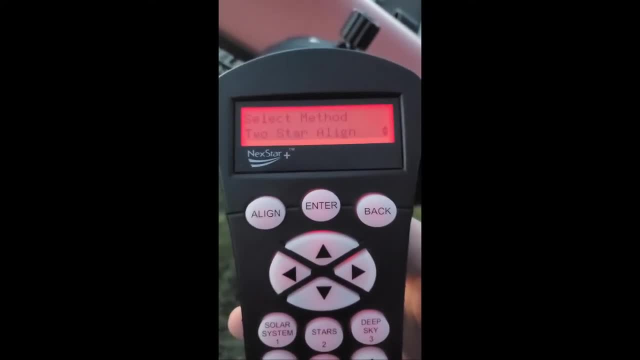 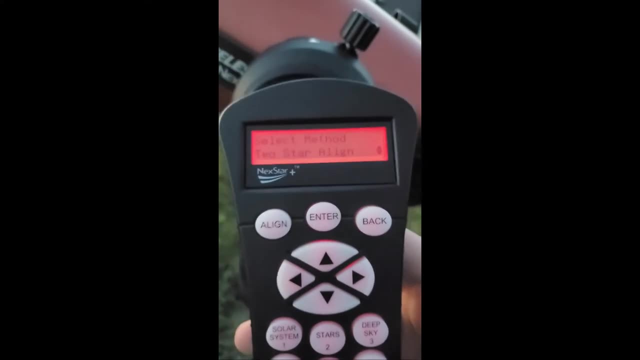 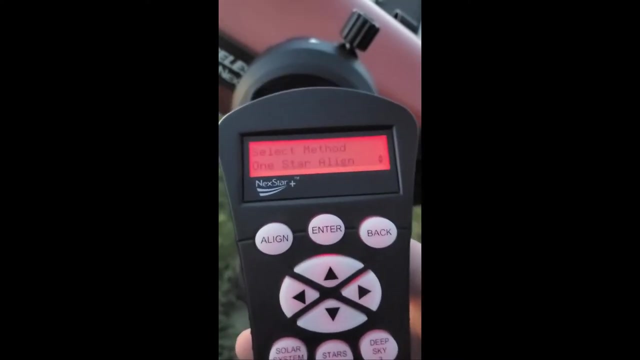 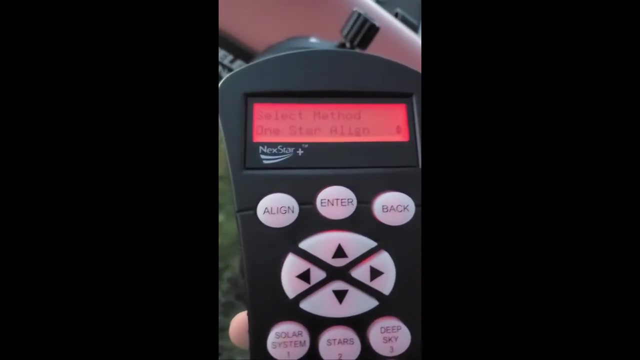 You want Vega and you tell it, you want Altair, And those are the two. those are the two stars that you, you do, but you have to drive the telescope to do that One star line. Typically, the accuracy of this isn't that great because it's only putting one point in the sky And 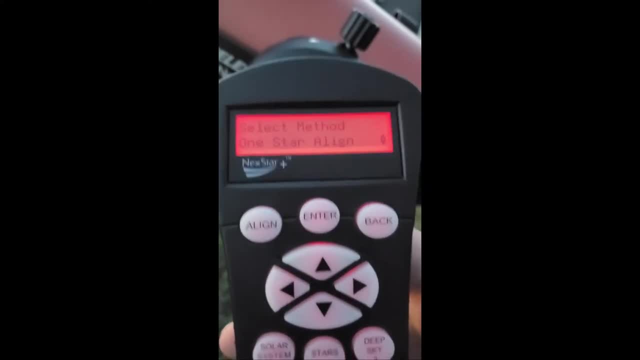 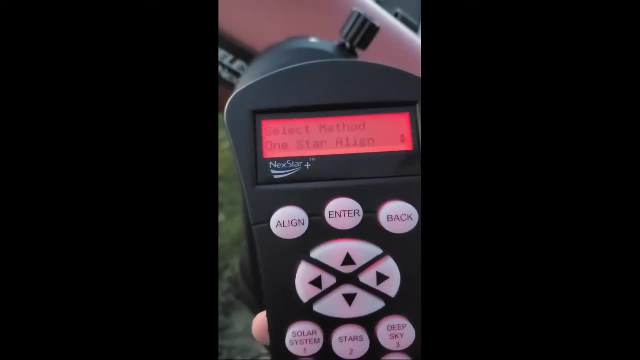 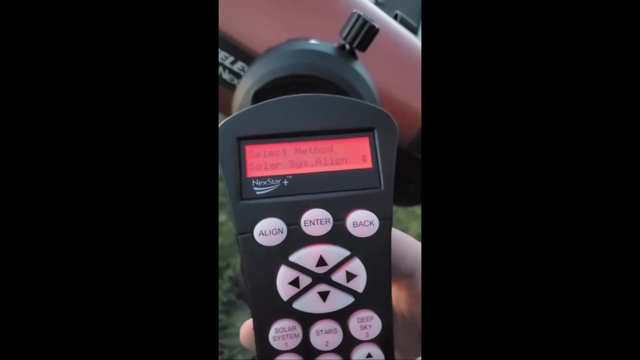 and when. if your telescope's not perfectly level, if things aren't perfect, it just it's. it'll get you something in a pinch, but I wouldn't recommend this one. Solar system align is one you can do when there's only you know, you can only see the moon, You can. 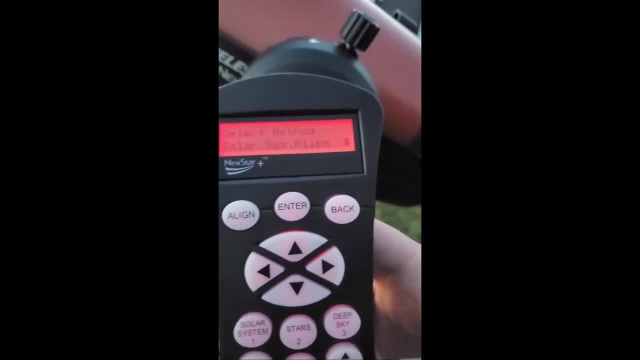 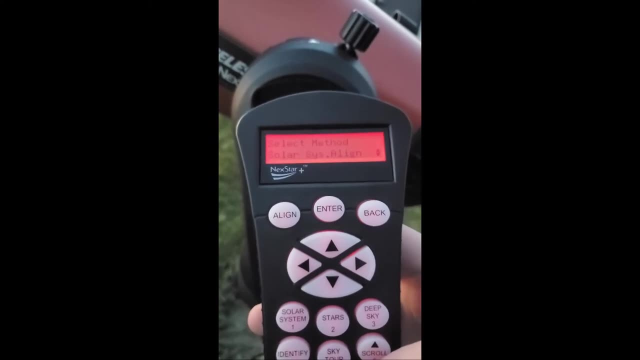 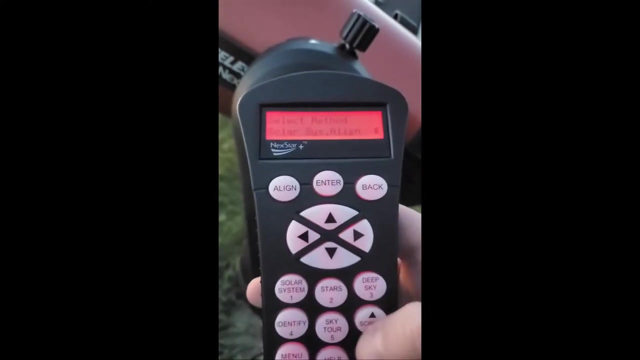 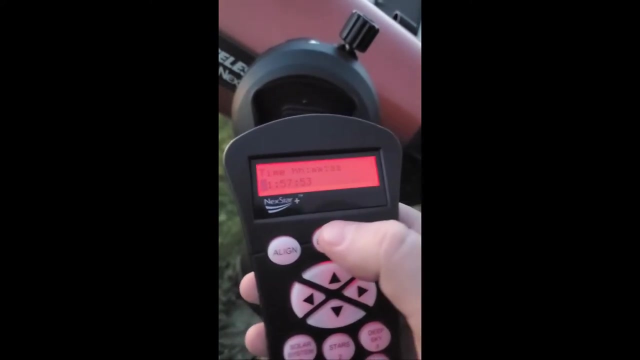 only see Jupiter or Saturn or Venus or Mars. This is actually a good one. This is the one we're going to do right now, Cause I can see it's just getting dark enough that I can see Jupiter, So I'm going to push enter to select solar system align. Now. this is very important. 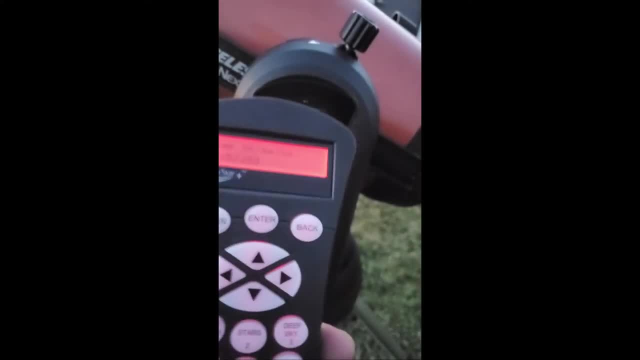 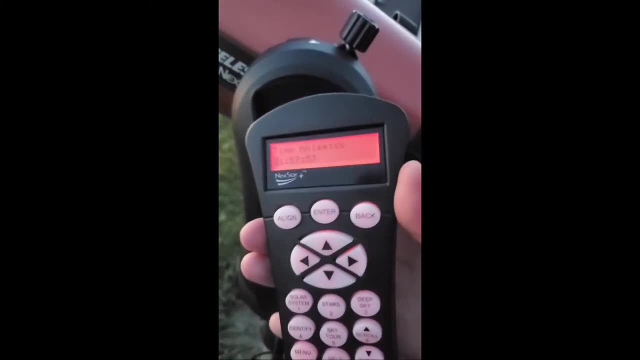 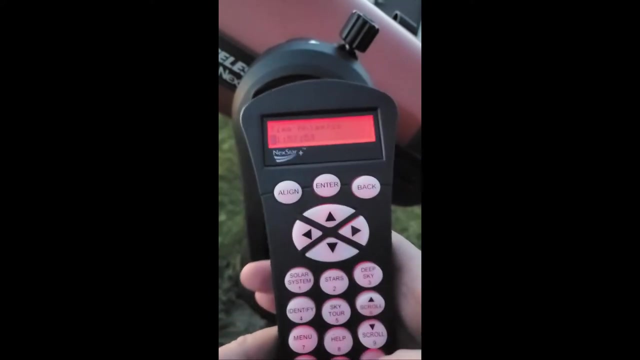 So this is the time Now. some models have a built-in GPS or you can buy an add-on GPS to these. that will get the time and date for you. But if you don't have it, you need to look that up. So right now it is 4- 45.. We need to do it in military time. 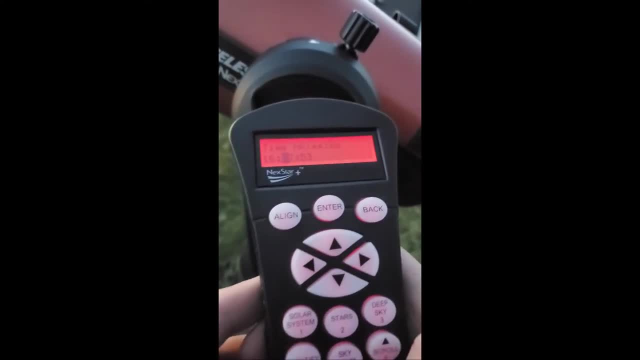 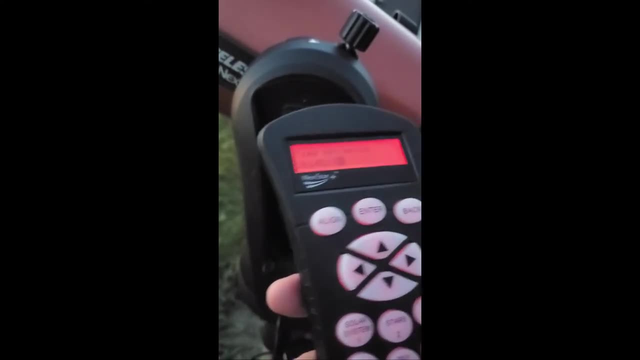 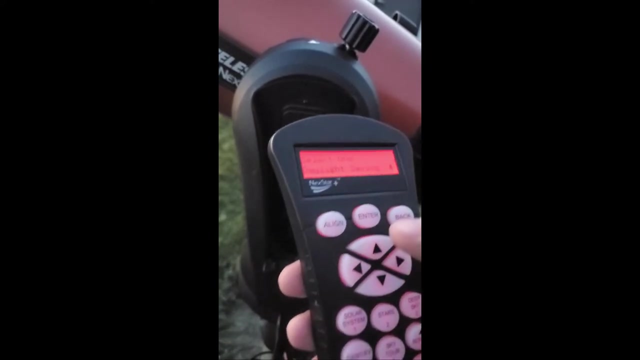 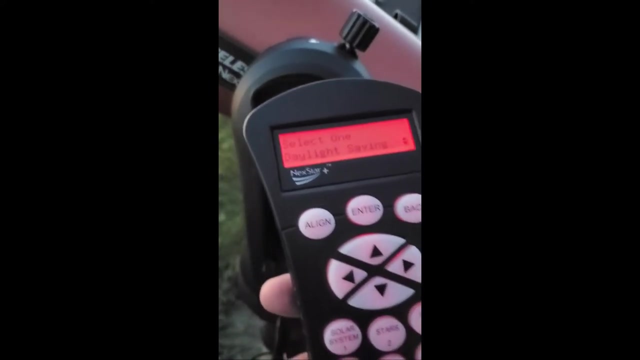 So that would be 16- 45.. The seconds really don't matter that much. I usually put it like at 30 seconds and then I'm going to hit enter Daylight savings- extremely important Winter time. you are not in daylight savings anymore, You were in standard time. So that ends in. 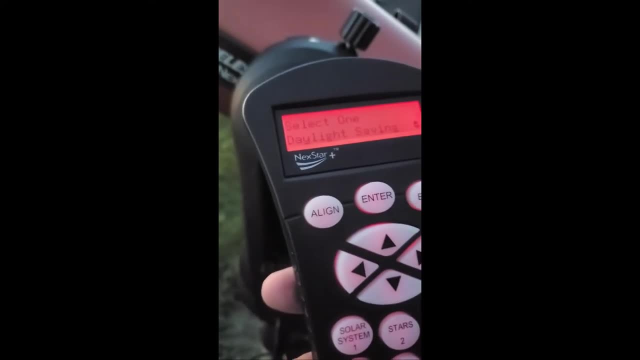 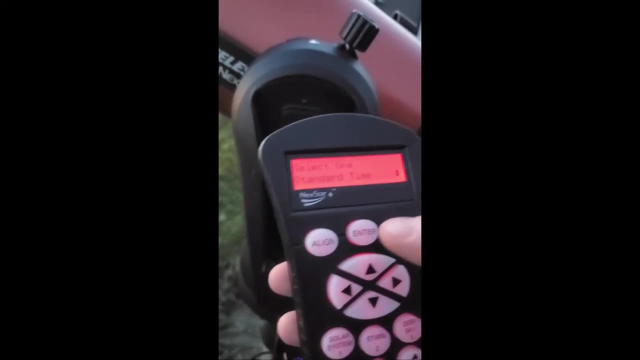 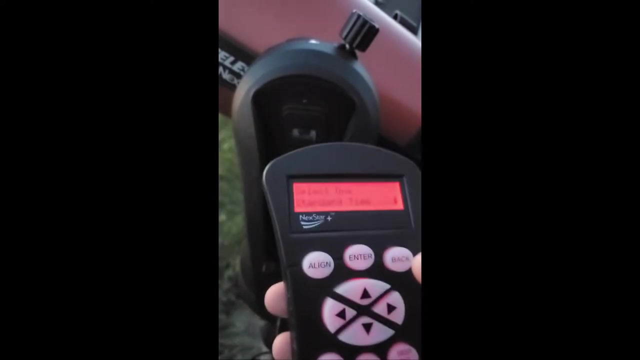 2020.. That was like the first first Sunday in November, So I'm going to change that. I'm going to change this to standard time. If you do this wrong, you're everything's going to be off by an hour. So, if you think that the if the telescope thinks that the moon should be in a 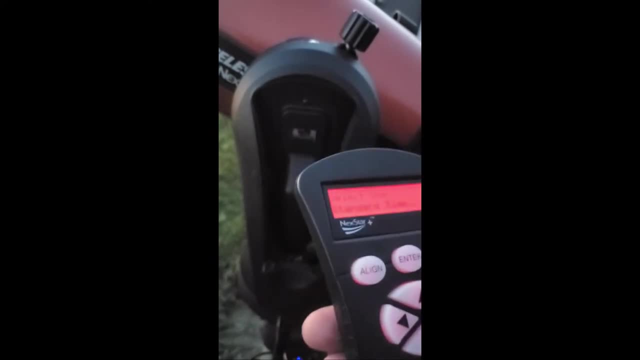 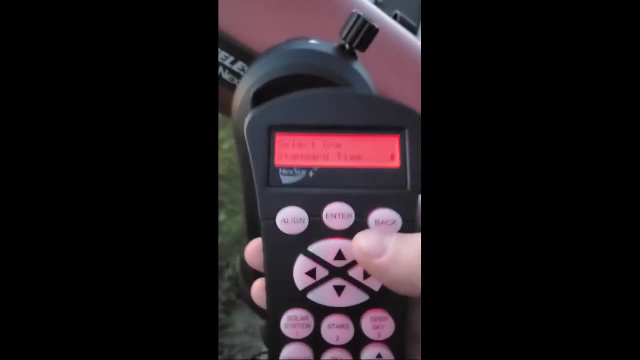 certain position. when it crosses the meridian, the moon stops rising and starts setting, And if you're off by an hour, it's not going to track properly. So this is pretty important, or this is a very important thing that a lot of people get wrong. 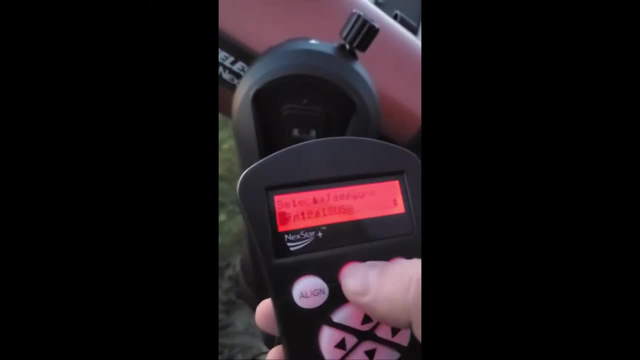 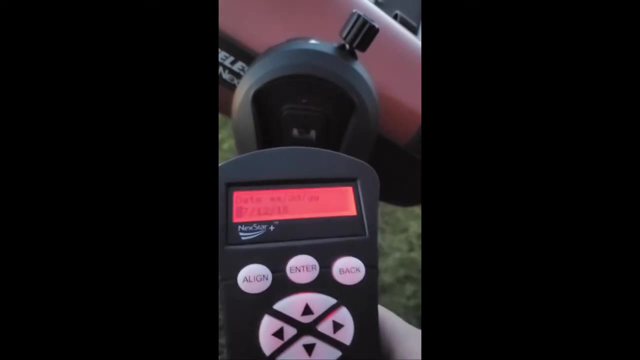 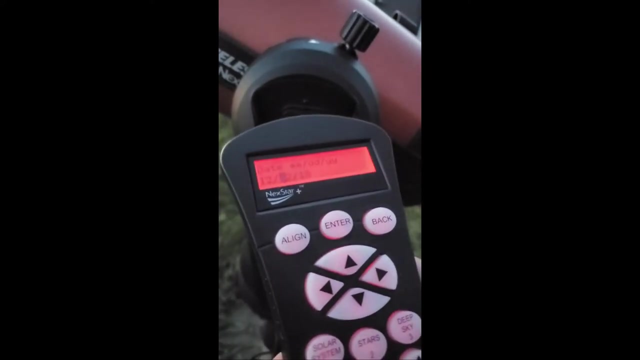 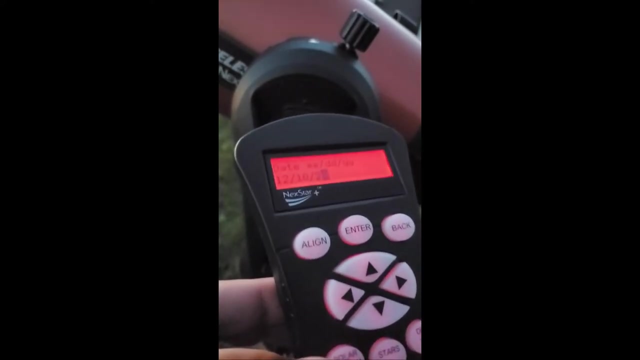 Um central USA, that's where we're located, and the date So, um, typically it remembers the last date and time that you used, So today is 12, uh, what's the date? 12, 10 of 20.. 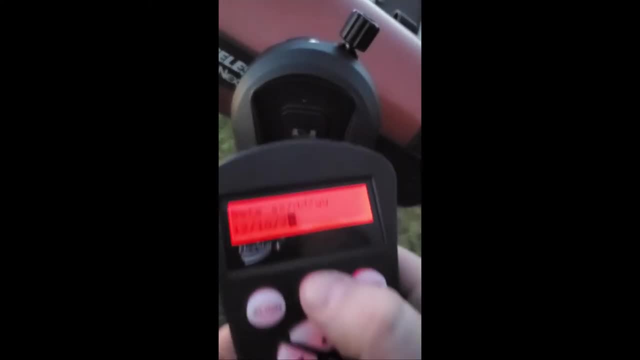 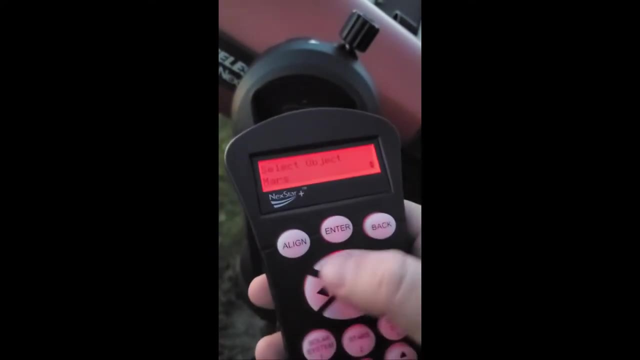 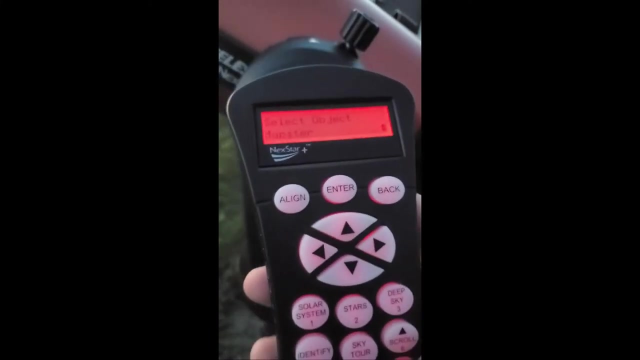 And then we're going to hit enter on that. So it says: select the object. So we're going to select Jupiter again. These control the telescope. When you have to arrow up and down, you need to use these. So I'm going to arrow to Jupiter and it says: 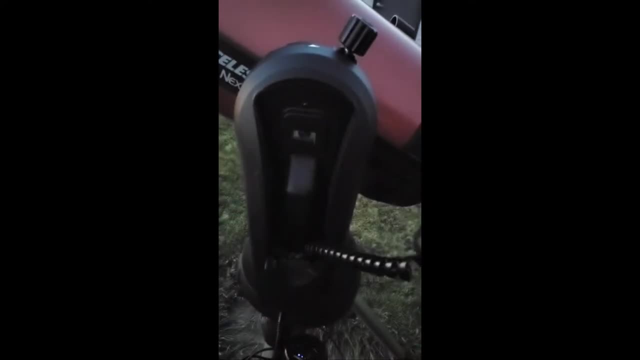 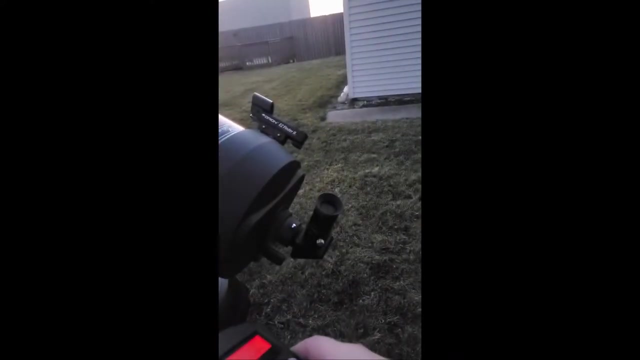 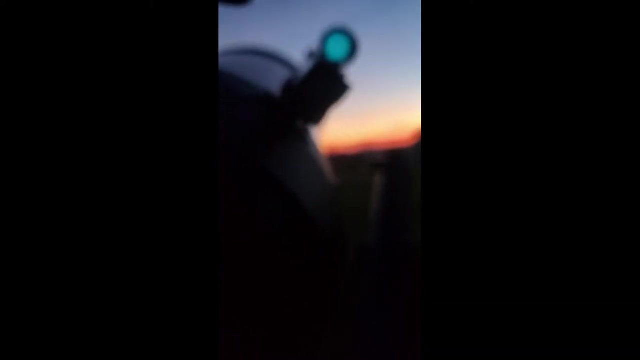 use the directional button- So that's these- to get Jupiter in our finder, which is this. So I saw Jupiter a second ago and now I don't see it. Sorry, see it okay. so this is going to be almost impossible for me to show you, but here I have. 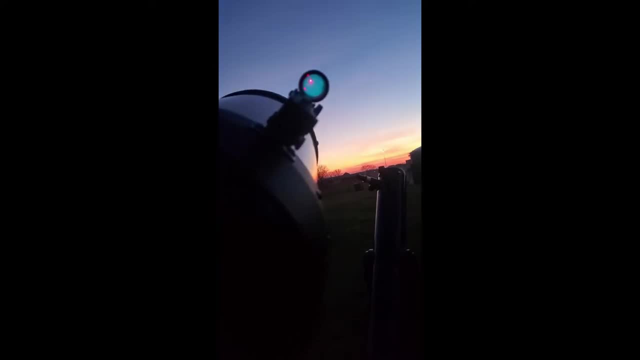 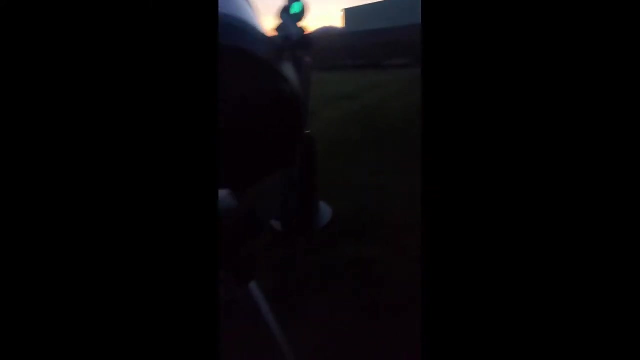 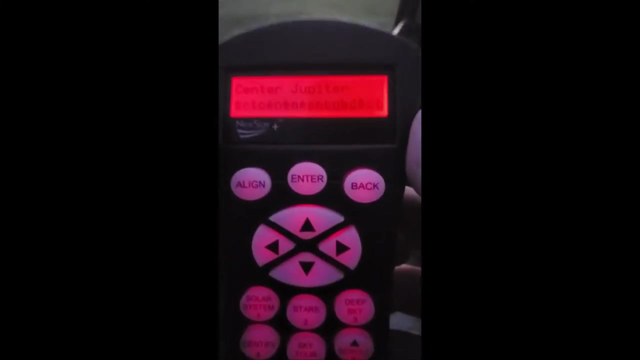 my red dot finder on and if I get that right in the center and you can't see it in the sky, but I promise you that that there's a little glowing dot in the sky which is Jupiter. so I have my red dot finder on Jupiter and what the hand controller asked me is to Center Jupiter in the finder, which 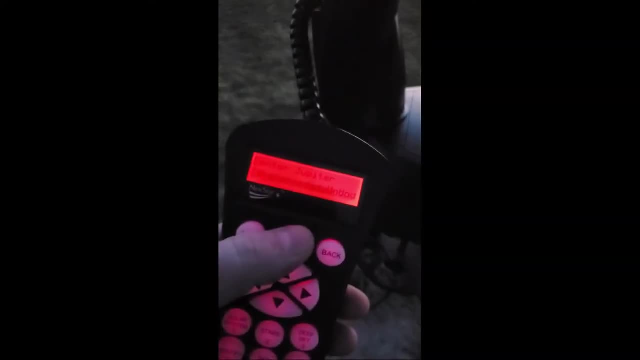 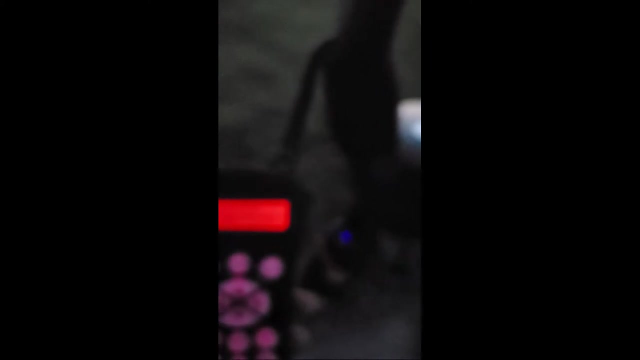 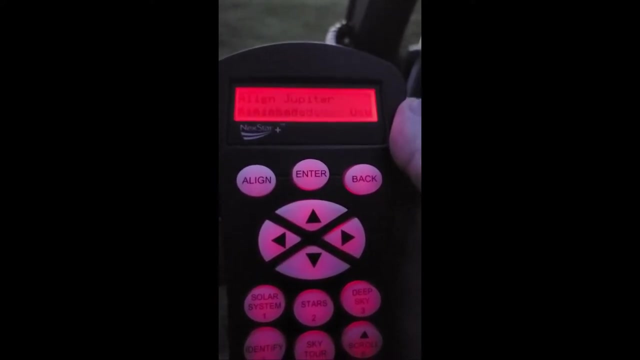 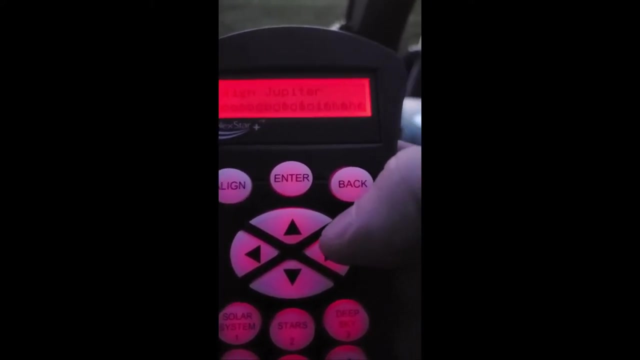 I have done so. once I've done that, I'm going to hit enter Jupiter's in the finder and then what it tells me to do, if I can get this to come in, is align Jupiter. so use my buttons to align Jupiter to line object in the eyepiece. so what? 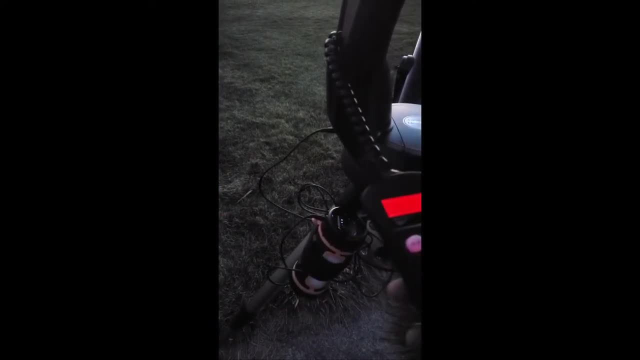 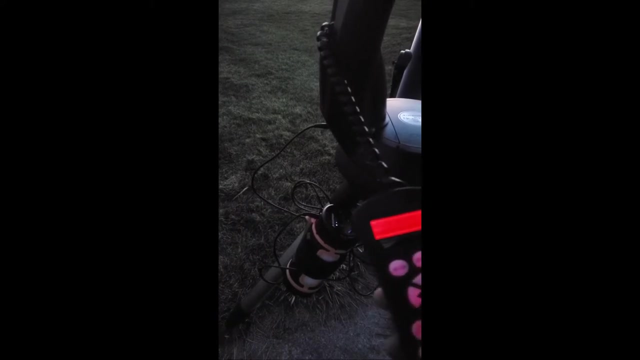 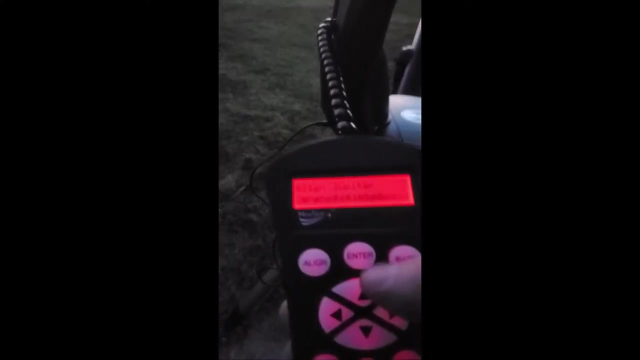 it's telling me to do is get it, get the object in the very center of the eyepiece. this is kind of one of those. do your best. they sell special eyepieces that have crosshair, that have reticles in it so you can know that you're getting it in the exact center. but for the most part this is just the solar. 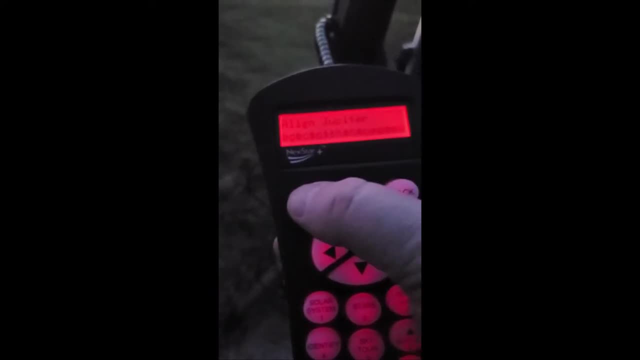 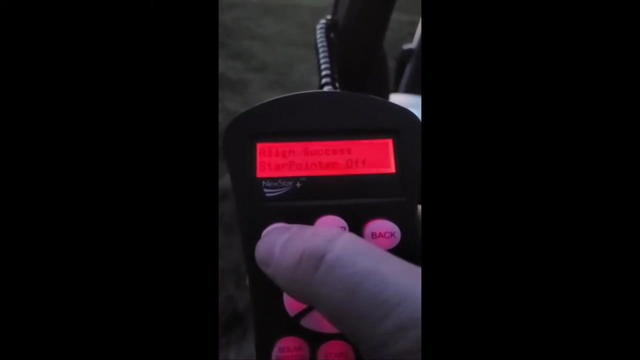 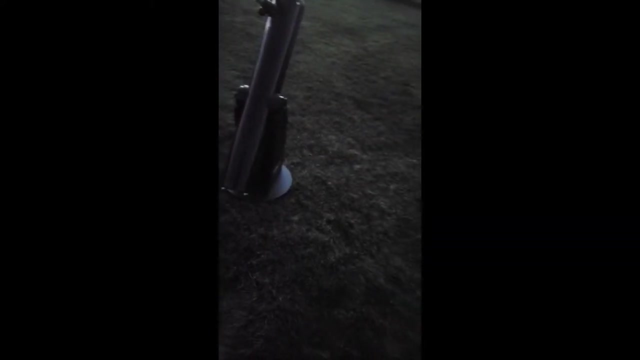 system alignment. so it's not that big deal. anyway, once we do that we're going to hit a line. so earlier when we got it in our finder we hit enter. when we get it in our eyepiece we hit a line. now it says star pointer off. so it's telling us to turn our finder off. so the they actually know. 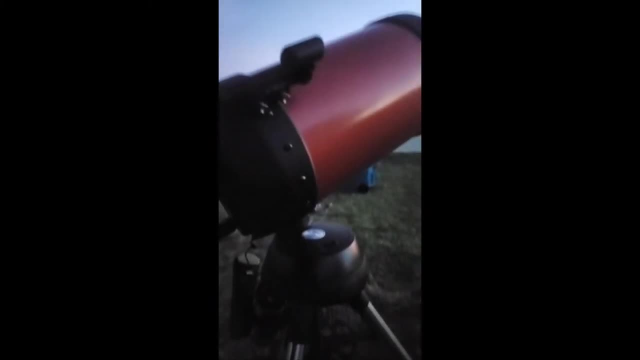 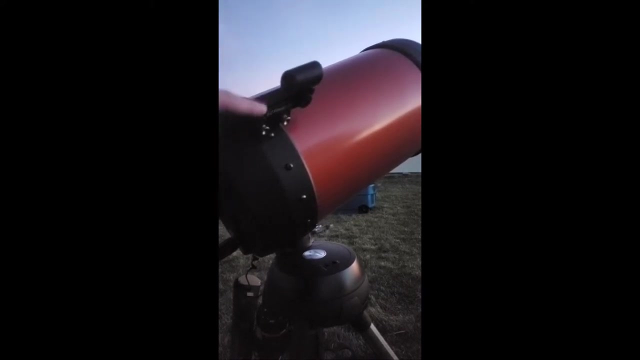 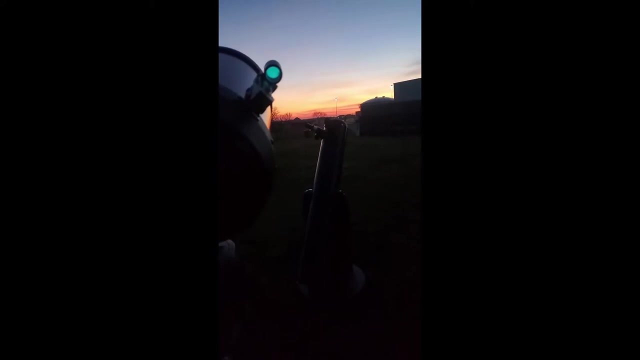 that you're going to forget and leave this on. so they tell you to turn it off. you're gonna forget, because I forget, everybody forgets but it. but the hand controller actually tells you to turn, to turn that off. so, without further ado, let's see if, if there's any way, we can get Jupiter to show up in. 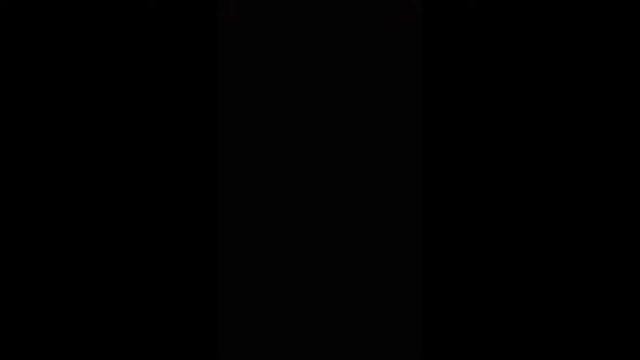 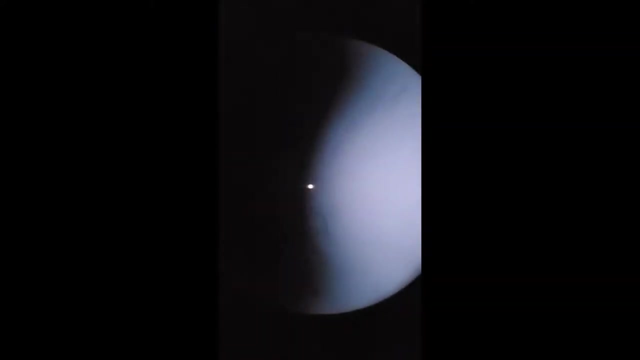 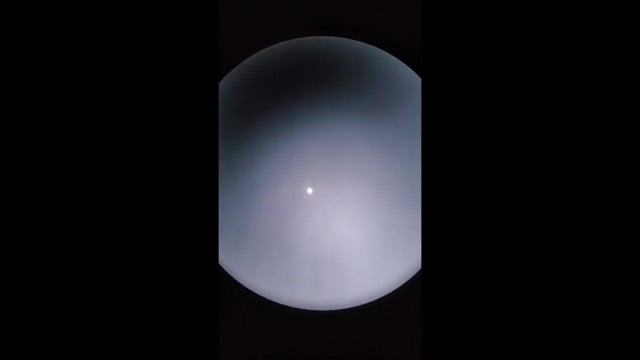 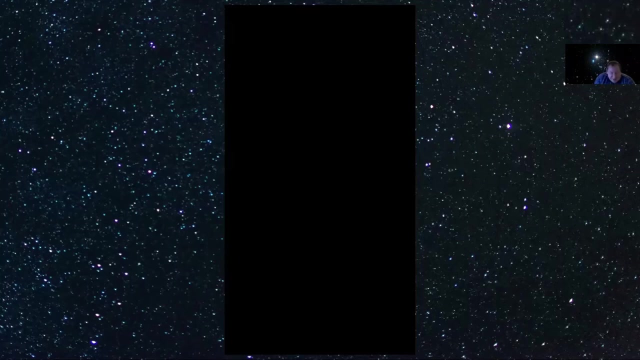 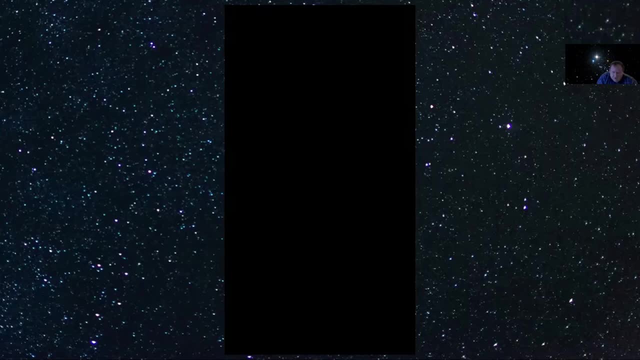 to adjust though that finder. he'll show you that, that stuff. there's a couple little knobs on these finders that will move that little red dot left, a right or upper up and down to to get that aligned with your telescope. um, when you have a Facebook question, Joseph asked. 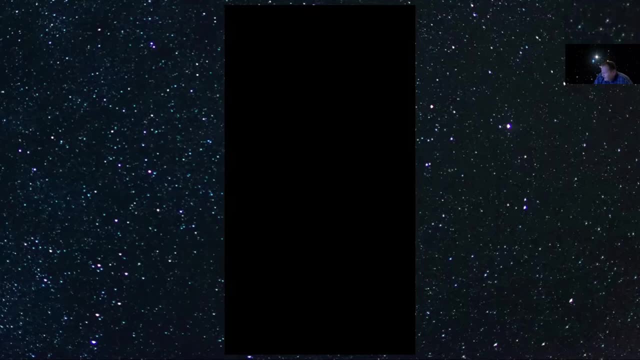 when aligning your finder scope and are looking at a distant object. should you use a hot stick, high or low power eyepiece in your main scope, or does it matter? personally, i don't really think it matters that much. probably if you were using a higher magnification, your your finder would be a. 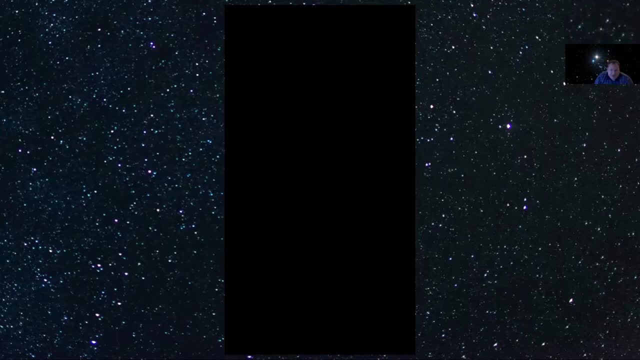 little more accurate, but, um, it's i. i don't find that it matters if you, if you can get, because you're kind of eyeballing everything anyway. so if you can get the top of that uh cell tower in the in the eyepiece and if you get your finder looking at it, uh, when you're trying to find. 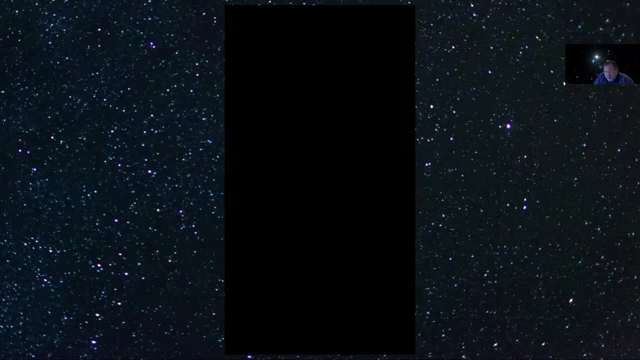 something in the sky. you're going to be pretty close anyway, so personally i don't think it matters. um, probably some people would argue that that it does, but i, i, uh, i just kind of wing it on most stuff and, and usually that my alignments are are fairly accurate, um, i don't see any other. 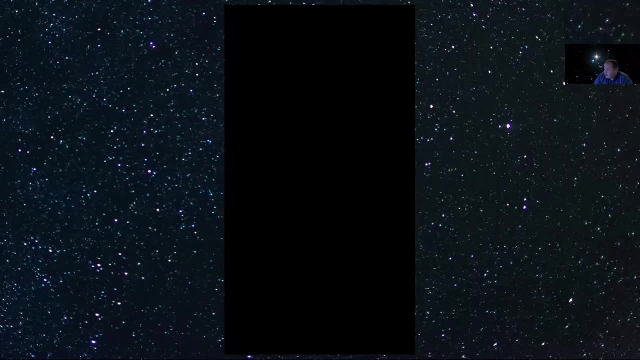 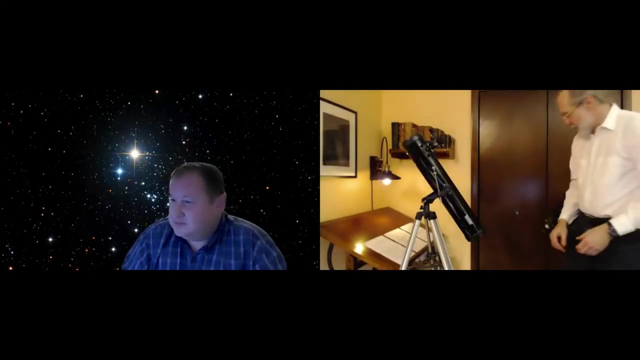 questions. if you, if you do have more questions on the celestron, uh, we can answer those later. um, i think drew is going to take over now, so i'm going to stop sharing and drew, you can? uh, you want to spotlight me? i'm not going to share, i'm just going to be. 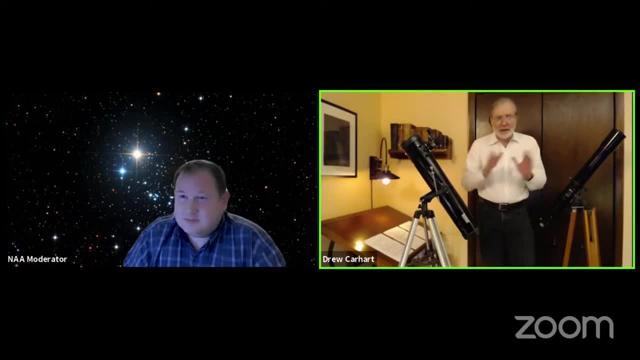 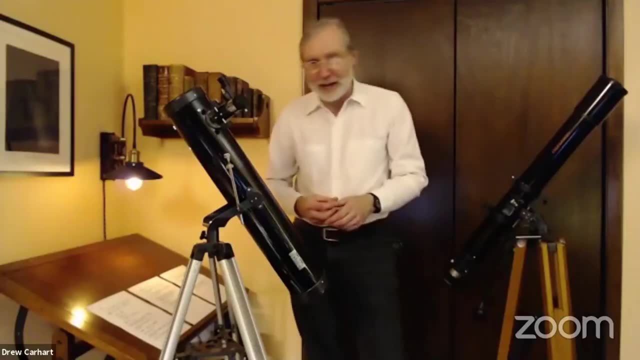 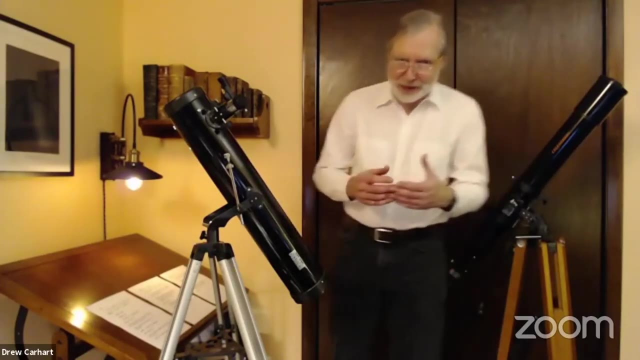 on screen here. so uh, hi everybody. um, i joined jim and welcoming you and uh, i'd like to add, gee, if you uh have your first telescope in hand now you're just learning to use uh. congratulations and uh. welcome to the world of telescope users. um, jim kind of started out with a little more complicated. 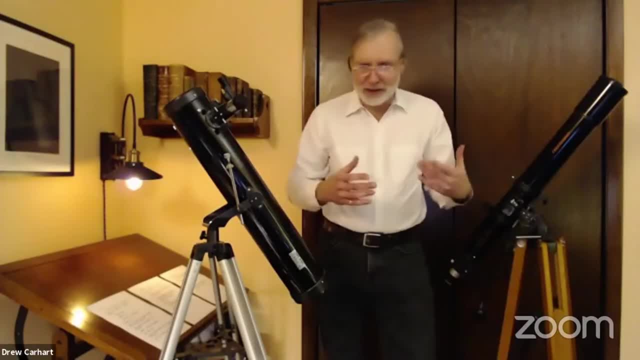 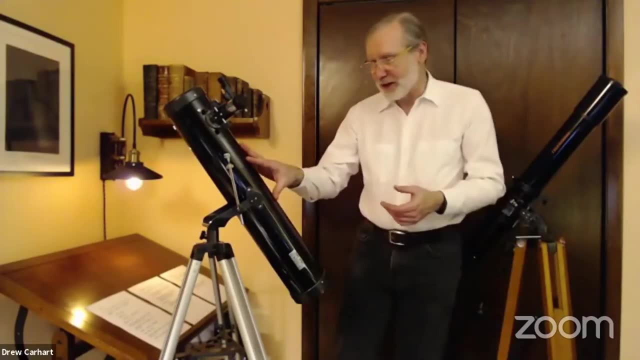 telescope. i'm going to kind of back up and talk about a little simpler stuff and um mainly going to use this fella sitting here as a demonstration piece. this is a uh fairly inexpensive um telescope, like a lot of people might end up with as starting things. um the uh it's. 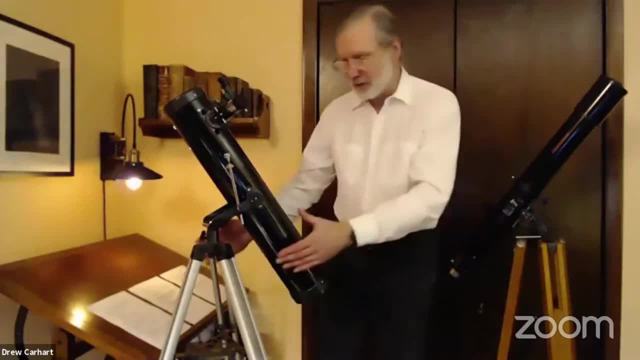 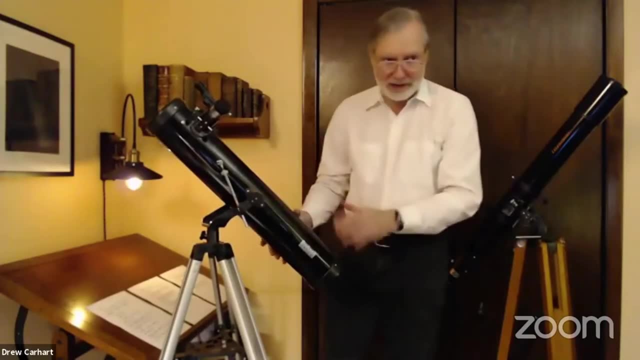 a reflecting telescope. it's on a very simple mount, we're calling altazimuth mount, that just goes up and down and around in a circle. ah, there's no motors on it, there's no computers on it or anything. so it's good for just demonstrating basically telescope things. uh, i think i'd start. 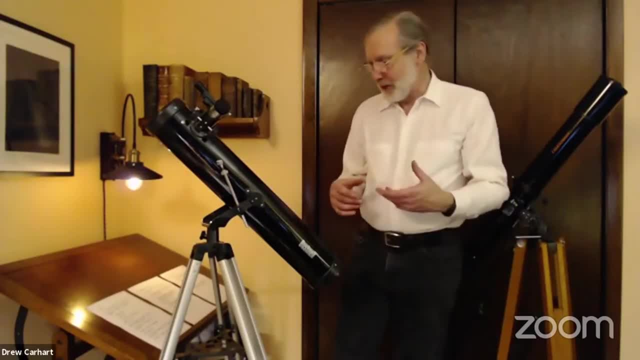 out really uh, enthusiastically if you didn't do a lot of sort of propellant and um i just What Jim said at the beginning of his section was: don't try to learn your new telescope out in the dark in the backyard the first time. Set it up in the house at first. Set it up, Follow the instructions, Learn what the different parts are and what they do. 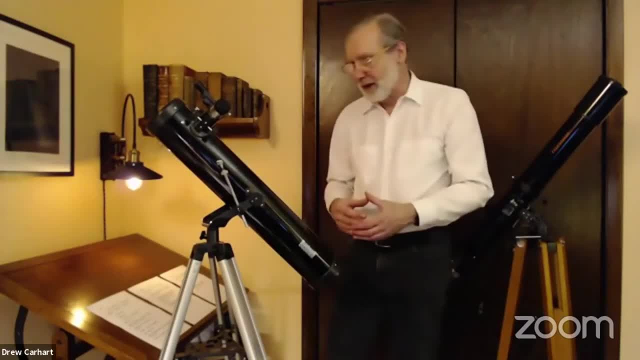 Hopefully you got instructions with your telescope. If not, look them up here, Look them up on YouTube or something, or rather just to figure out what it is and how it goes together. Don't try to fumble, assembling it and using it, pushing it around and stuff the first time in the dark. 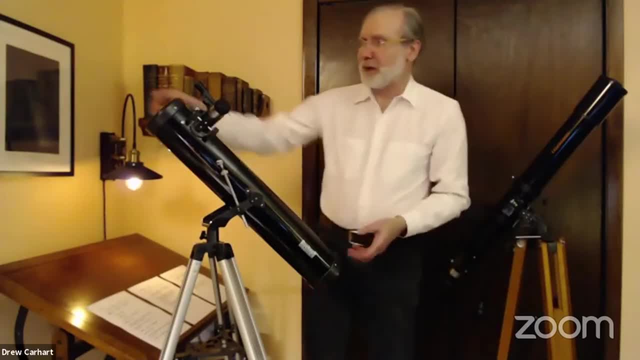 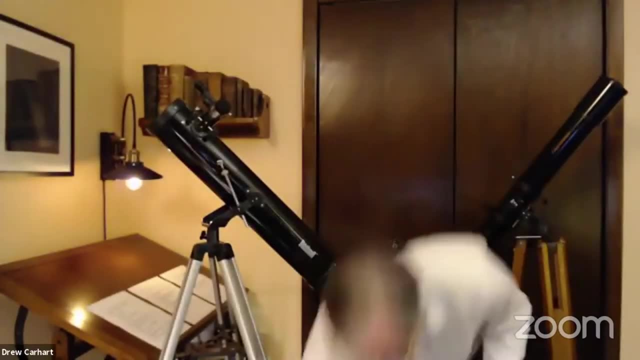 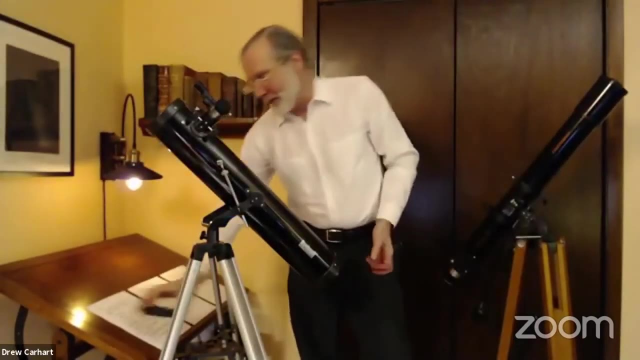 Second thing that's really important. Well, I guess part B is Jim's note that there's a cover on the front of your telescope. I just dropped half of it. Important thing: Save the cover. You need to keep your telescope clean, But when you go to observe remember to take it off. 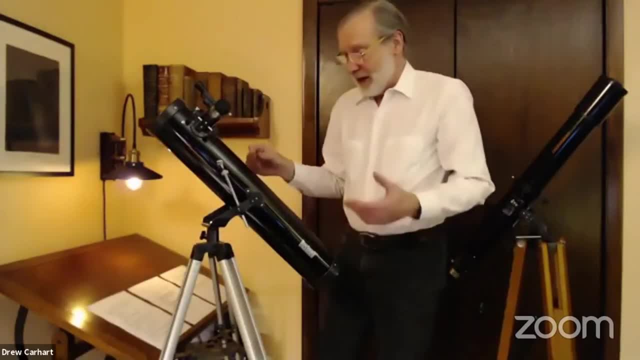 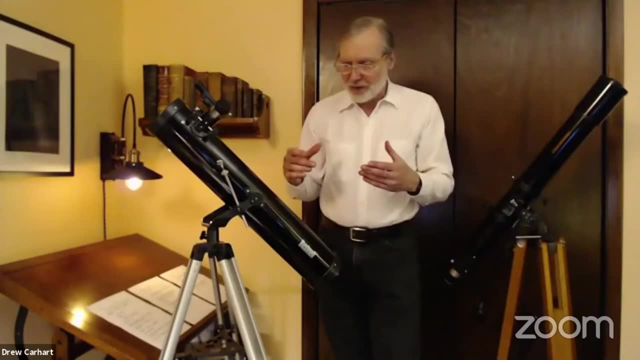 It doesn't help things at all. Have cover on it In inexpensive telescopes especially, but it can be true in any telescope. One of the big failures or semi failures or problems that people have is with the sturdiness of the mountings. 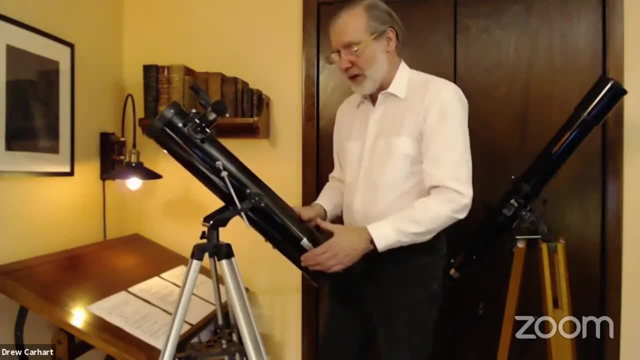 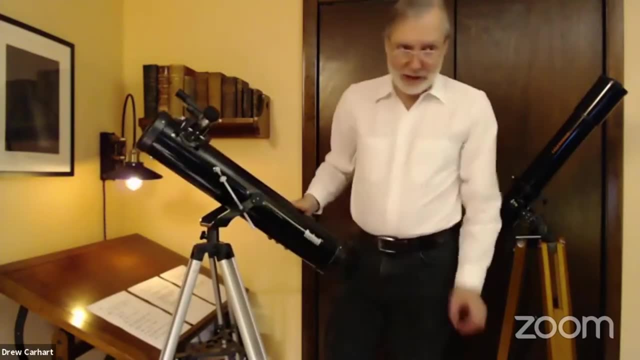 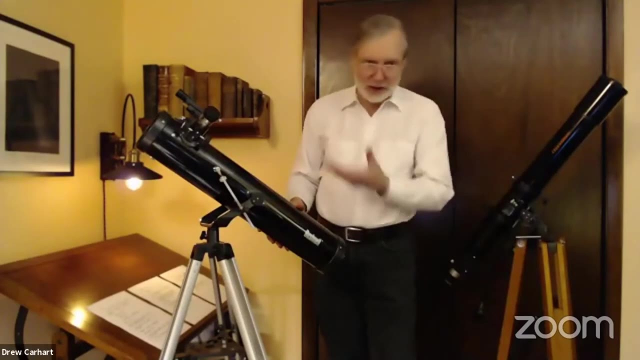 And if you set up your telescope and you find that it's really wobbly and shaky and clunky, that's not good. That's going to bother you every minute that you're trying to use it to actually stargaze with it. 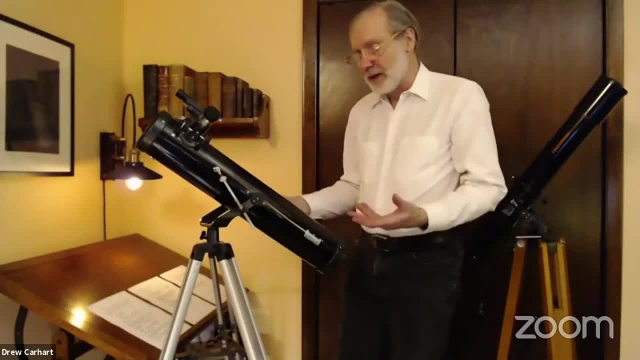 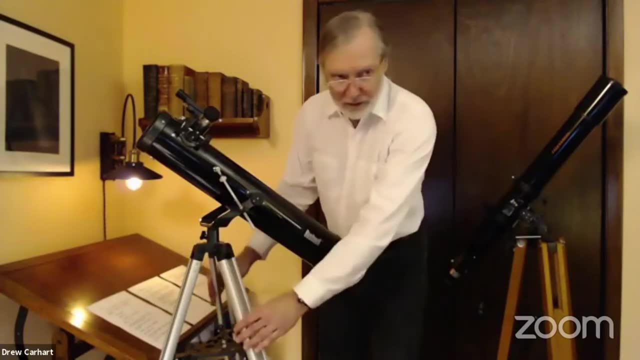 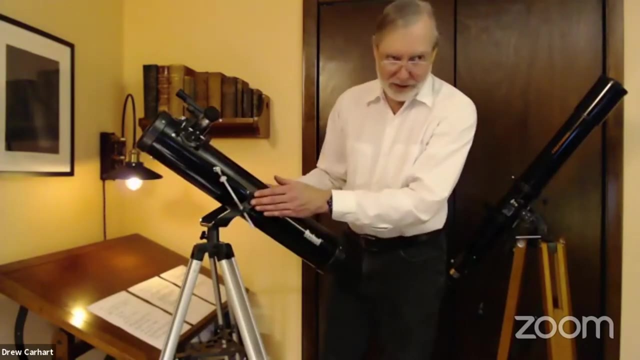 So there's a few things in setting up a telescope that you can do to address this. First off, all of the parts here like this: the tripod assembly and even the mounting. on something like this There are various screws and nuts and bolts and knobs and things. 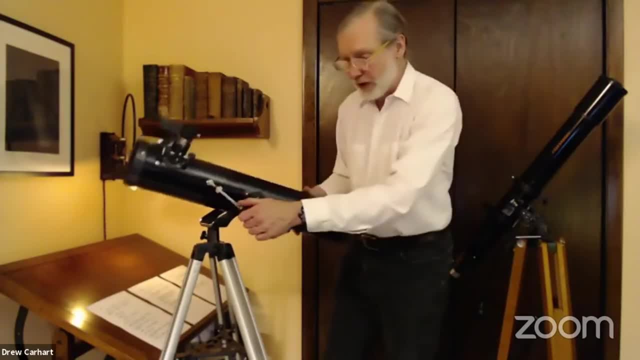 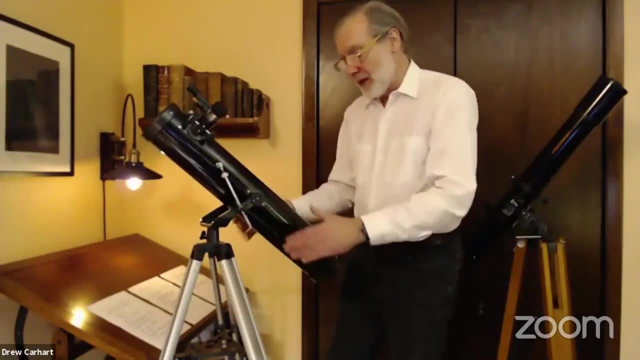 Make sure things are tight. You need to be able to move stuff. But if it's rattly and loose, try to figure out why. If the tripod, which is oftentimes again sort of the weak point in inexpensive telescopes, 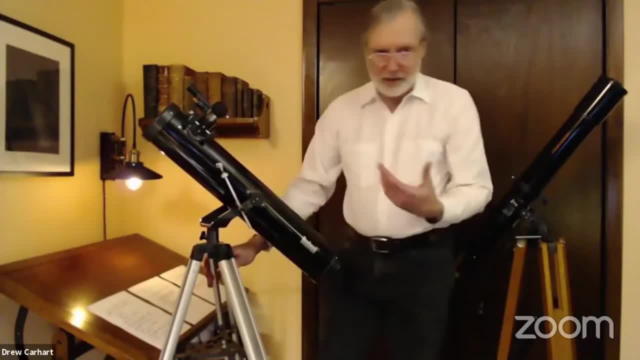 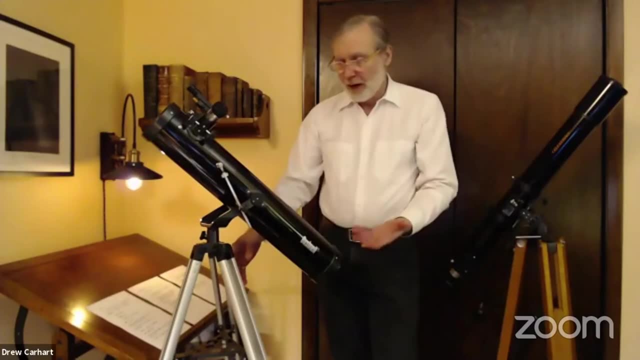 If the tripod is wobbly, there's a couple of things you can do to improve it. First off, Jim showed you that most tripods are adjustable in height. Generally, the taller you've got the tripod set, the more wobbly it might be. 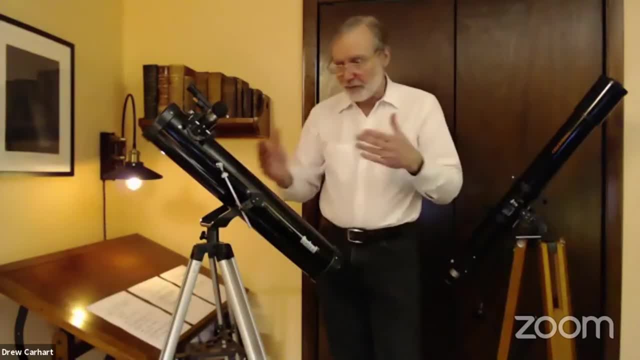 So you might take some of the shakiness out of it by just lowering the legs some, Even if it means you need to sit down or something to observe, or sit on a stool or whatever or crouch over. that might make it steadier. 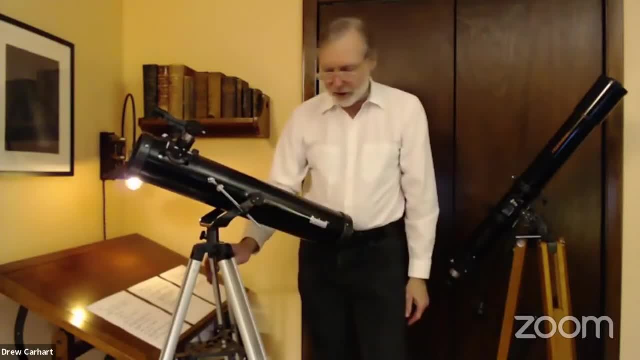 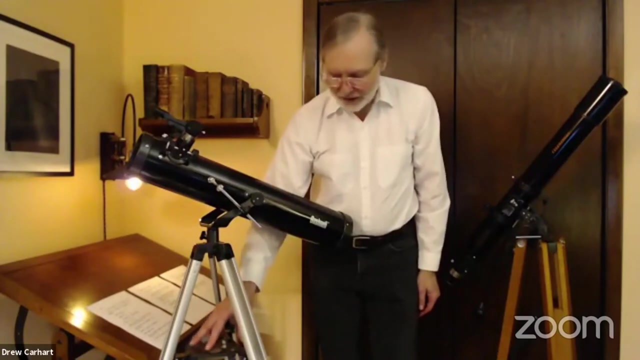 Another handy trick on lighter weight tripods especially is most of them have this spreader plate between the three legs. Jim's telescope have that as a loose plate, Loose plate that bolted up A lot of. again, lighter weight tripods will have a panel in here that stays in place. 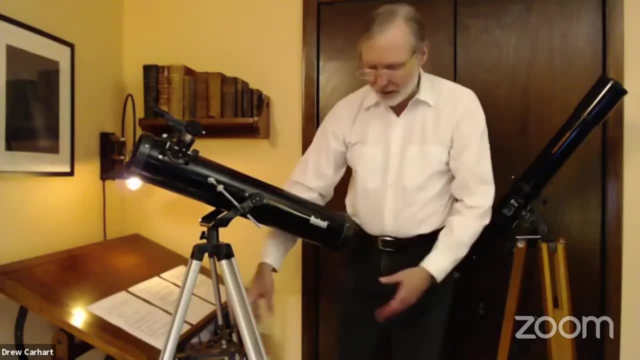 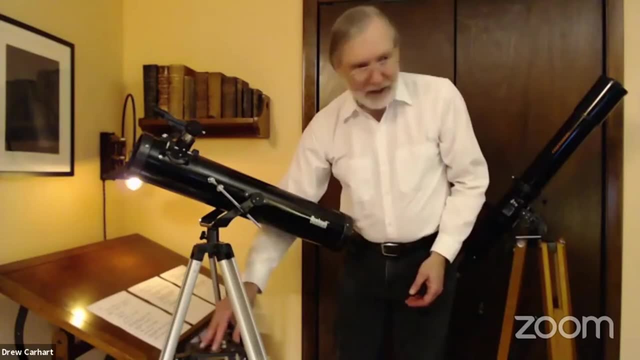 or it's made so you can swing it down onto one leg, so you can fold the tripod up. But tightening that up is good. Adding weight there can make a big difference too If you have a somewhat shaky tripod, if you hang a weight from the middle of it. 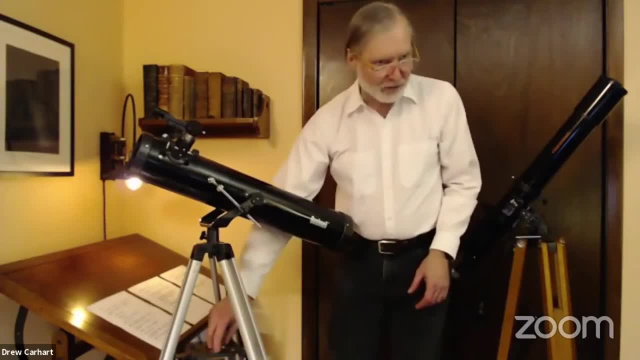 it's a handy place to put things. They always put these holes in them for putting your eyepieces in And I really, in my many years of observing, have seen many experienced observers who end up actually lining their eyepieces up there. 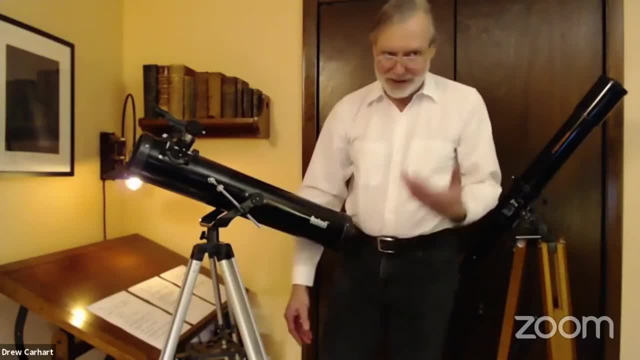 because what happens is they get dew on them or they get dirt on them. Then it doesn't end up sitting out there in space in the open air when you're outside observing. It's not generally a good place for your eyepieces, But you can use that panel to place weight on or even taking 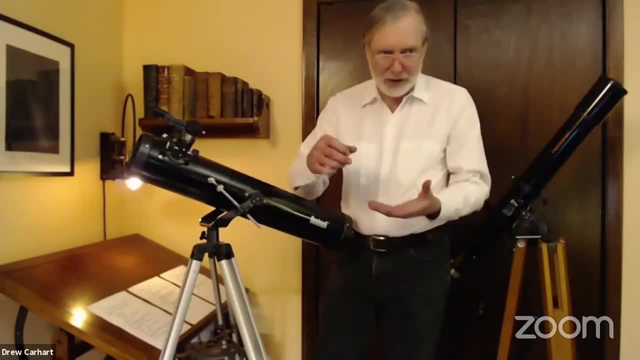 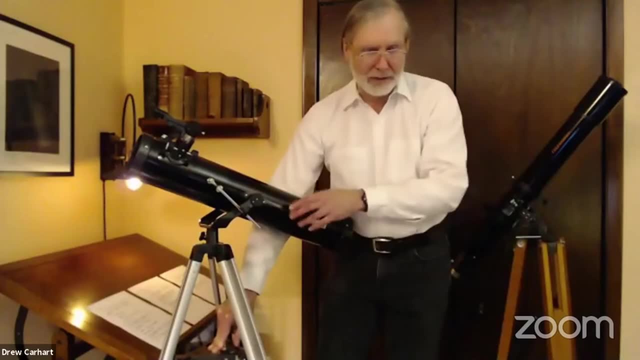 I've seen people take like a gallon milk jug or water jug and put water or sand in it and hang that from here. Adding extra weight there can really stabilize your tripod quite a bit, So that's a trick too. So stability is really important. 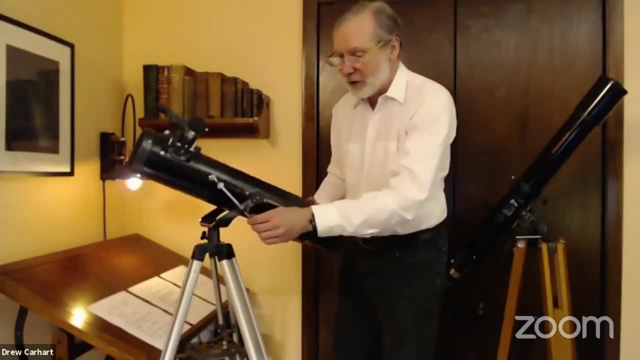 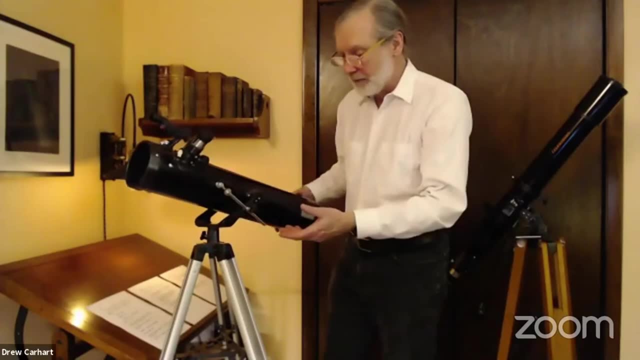 And again, that's something you need to play with. You might find when you're actually out using that- oh, I've noticed that there's something seems loose in here and you need to look at that in the daytime. But working with that first. 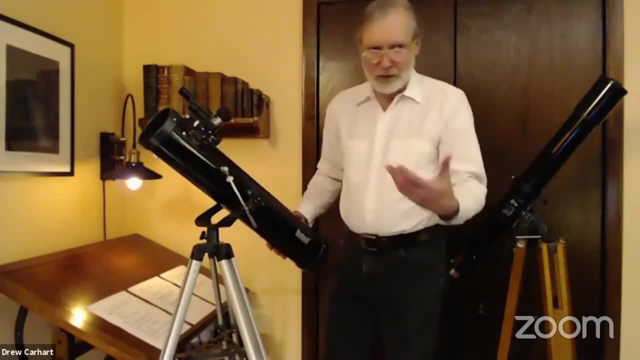 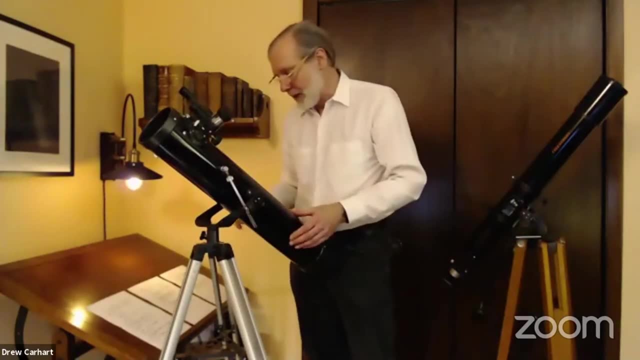 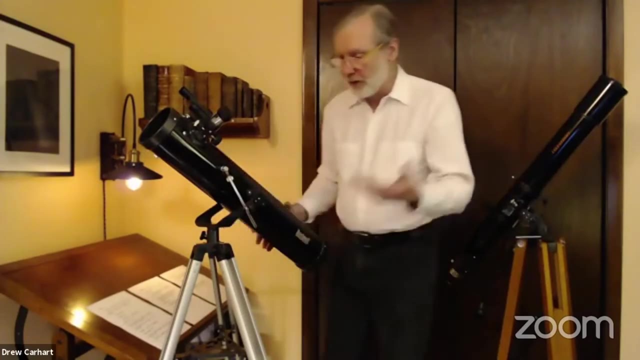 before you again are out in the dark doing your first nights of trying to observe things and point at things again. take care of that in the daytime beforehand. You need to learn the motions of your telescope and your mounting and how it turns. 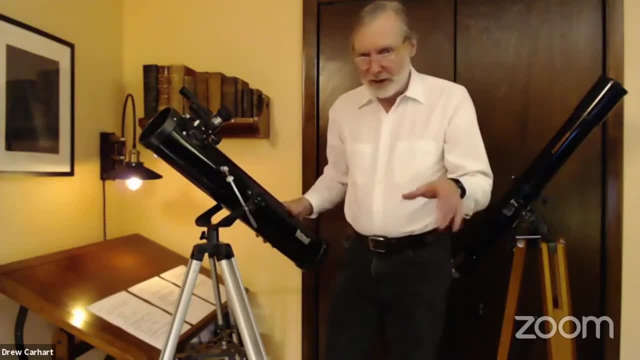 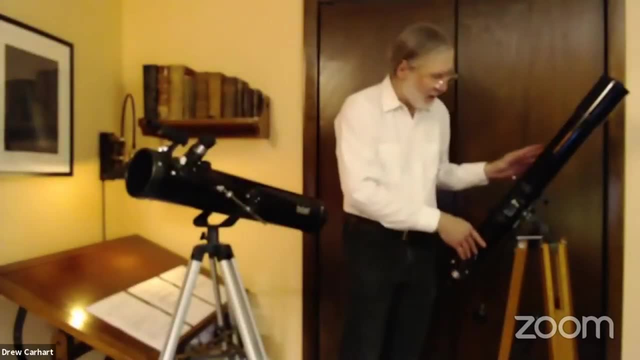 Jim's telescope again had motors on it that are steering it around the sky. This is a totally manual telescope. This is another one back here that's on a manual mount. It's used to the idea of that. this goes up and down and around. 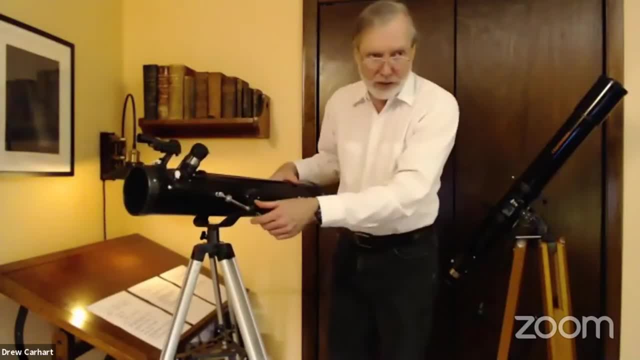 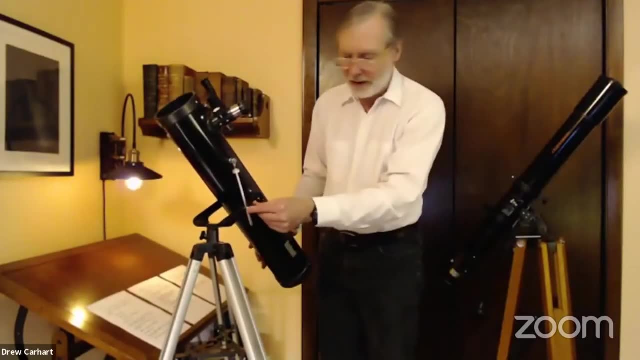 and so you can point at any part of the sky and what you need to do to make those motions go. It's used to the idea that on this telescope, once you put it at the right elevation, you really need to tighten down this knob on the side lightly to hold it in place. 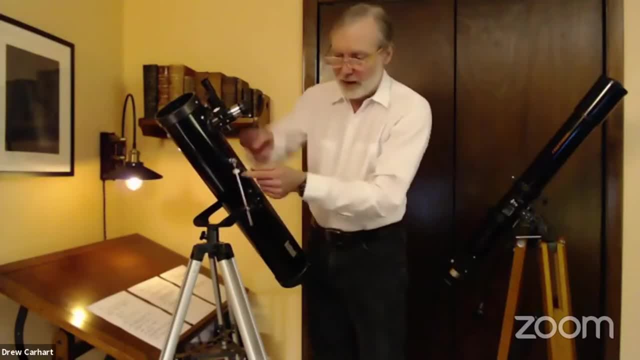 And then when you do that, this one has this feature on it where I can turn this little knob here on this shaft and it makes a fine adjustment of the elevation, So say, I've got Jupiter in the sky, I've got Jupiter in there. 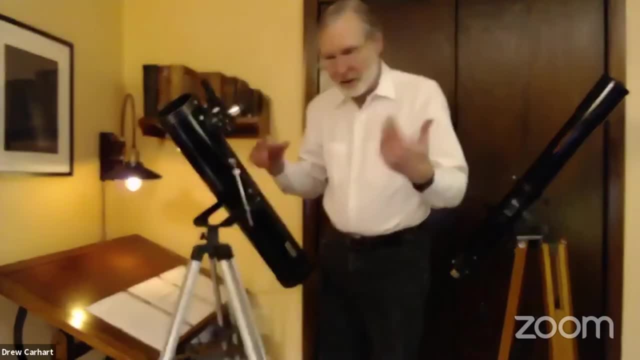 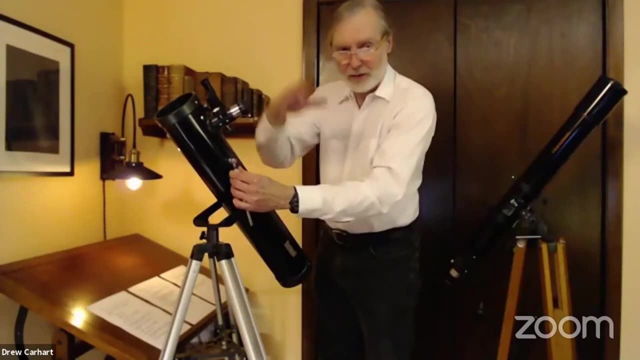 And it's starting to move out of my field of view because of the Earth's rotation. I might be able to just turn this a little bit without loosening things, and slide it back into the field of view without shaking it around and stuff. So that's a handy little thing. 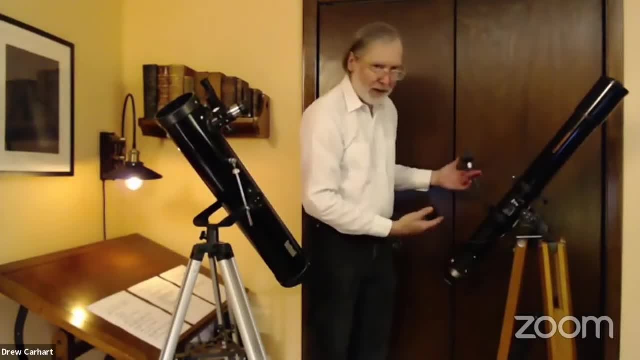 This mount back here is a little better quality one. It has two flexible cables that do the same thing. I can turn a knob to move the telescope up and down. I can turn a knob to move the telescope up and down. I can turn it back and forth. 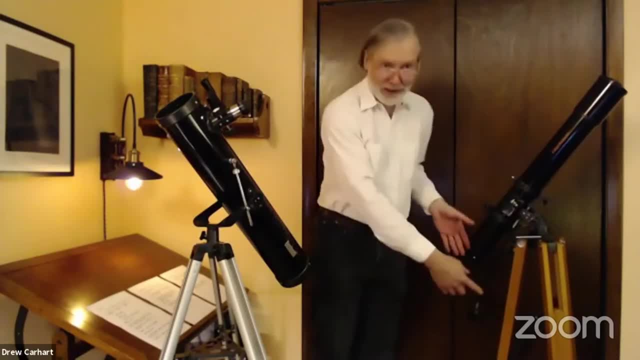 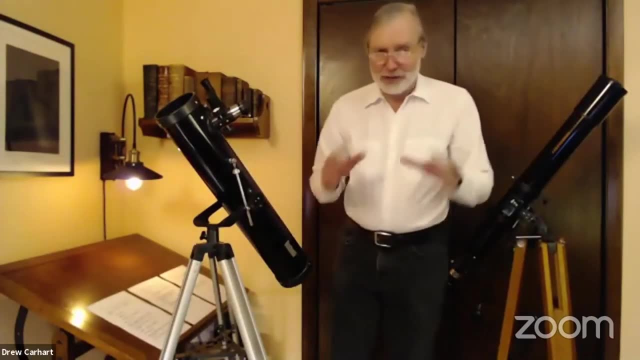 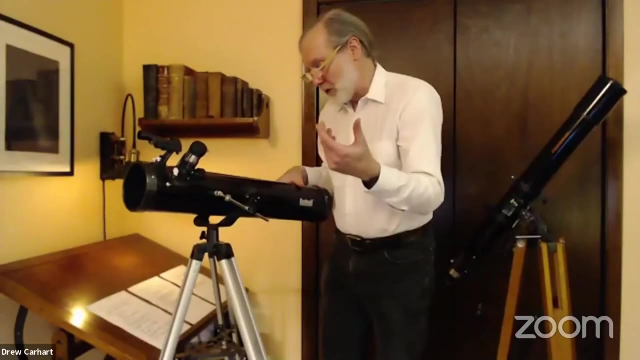 And this one is shaking because it's sitting on carpeting and I do not have the tripod deployed properly at all, But anyway. so these are things you need to learn about your telescope that will be specific to it, So you want to again be able to do this in the dark. 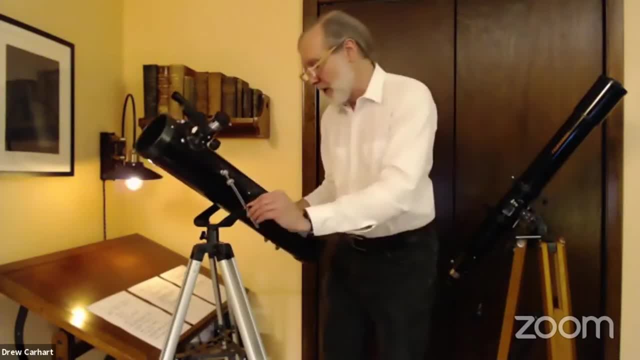 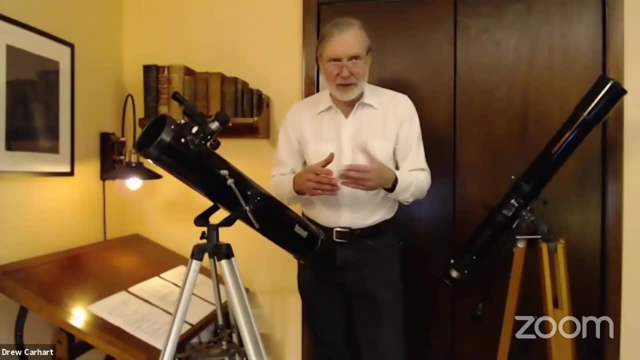 without wondering about it. without thinking about it, Jim already covered eyepieces. I will repeat also that, how important it is to – if this telescope came with two eyepieces – here's a simple summary, a 20-second summary. 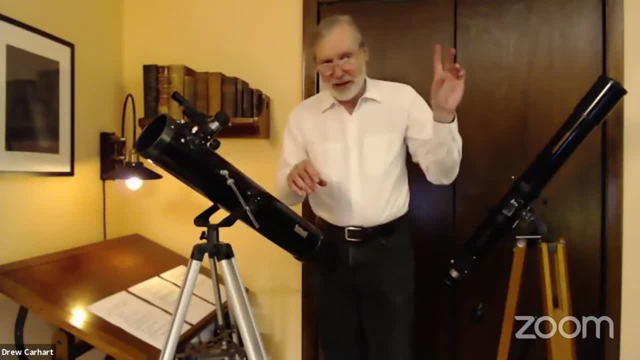 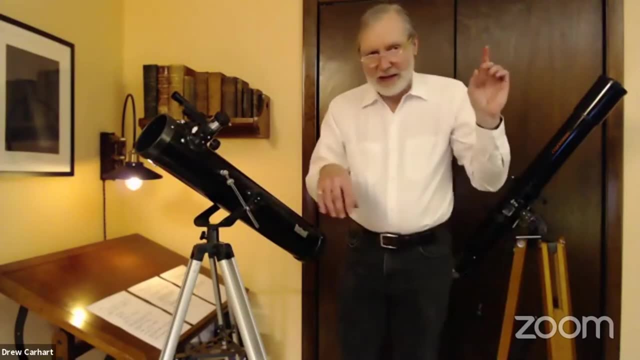 If it came with two eyepieces, there's going to be one with a higher number- say the 25 on it- and there's going to be one with a lower number. that might be like 10 or 12 or something. You always use the one with the higher number. 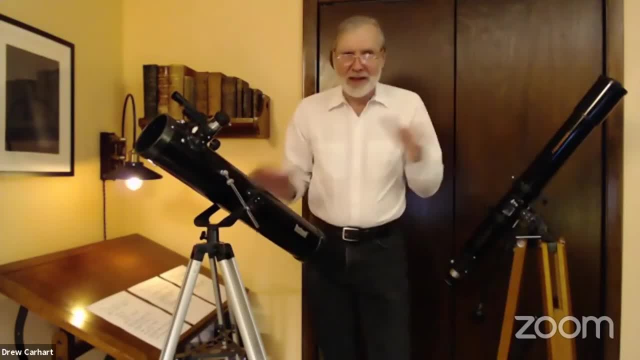 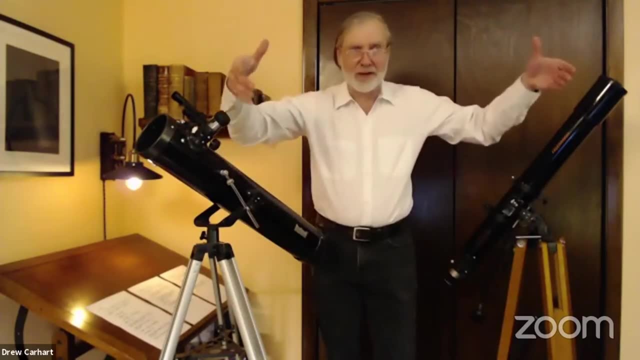 That's going to be your lower number. If it comes with a higher magnification, that gives you a wider field, a much wider field of sky than the higher magnification was, So it's going to be easier to get something into that field of view. 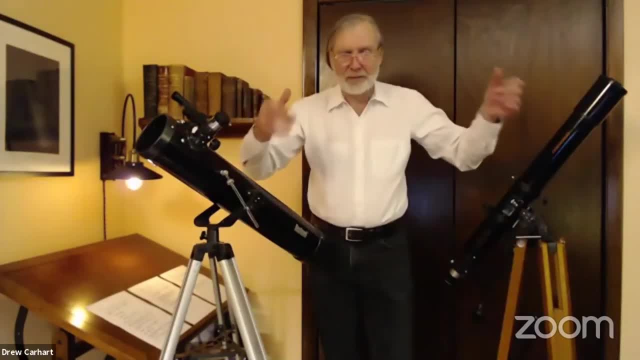 So when you're first trying to use your telescope, what most people find the most frustrating thing is getting things into the field of view first, And if you're trying to do it with looking through a straw or a high-power eyepiece, that's going to be a lot harder. 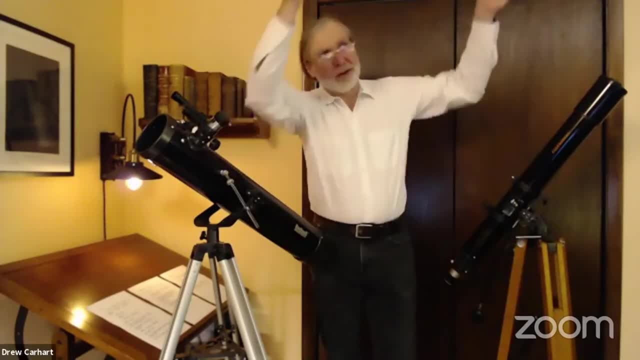 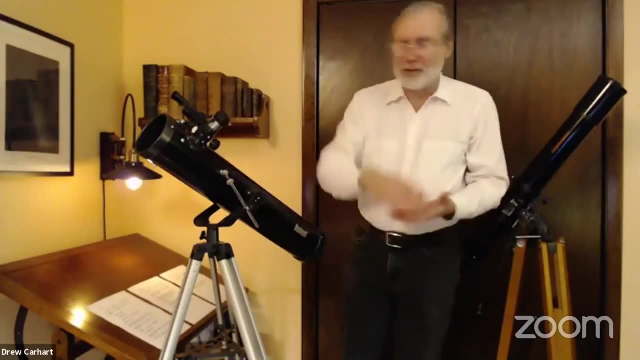 than looking through, you know, a hula hoop and seeing a wider area of sky, which is what the lower eyepiece would be, So that bigger number always starts there When you start getting good at finding things and centering things. 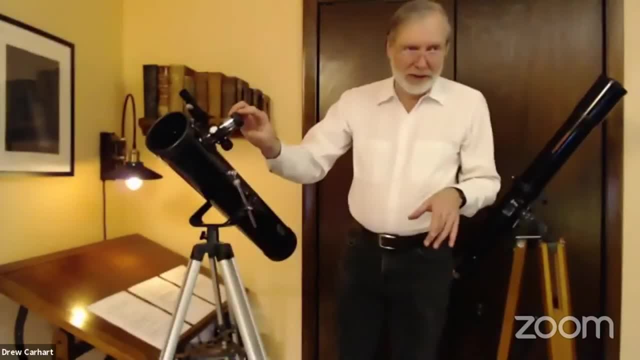 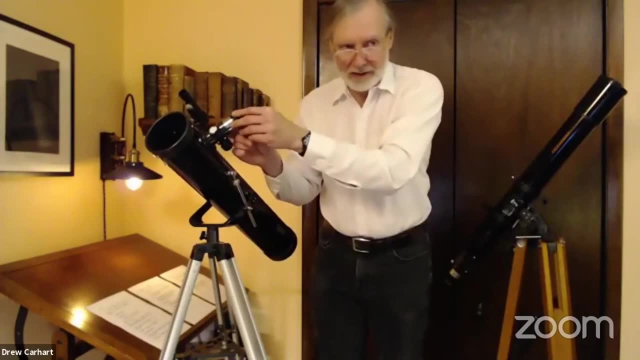 you might say: well, I've got Jupiter in here now centered, and I'm going to switch out this eyepiece and put in my higher-power eyepiece and see if I can still have Jupiter in there or if I can just center it again on that. 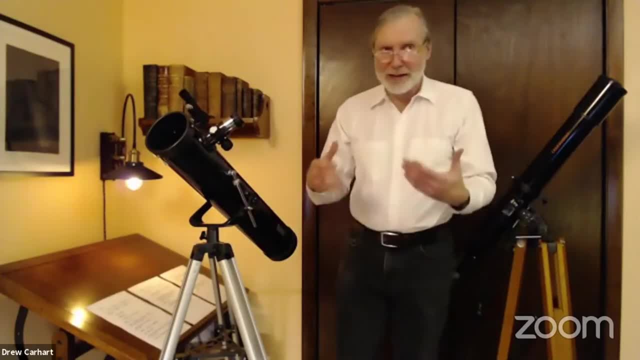 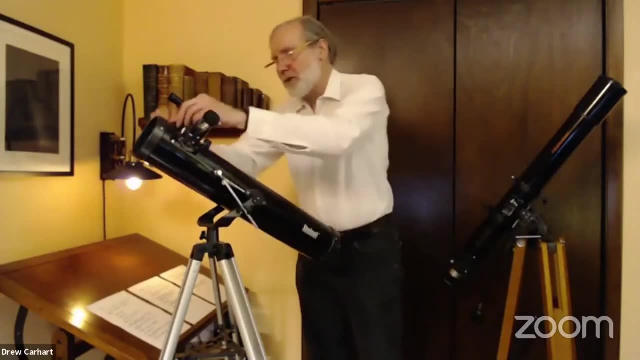 That's how you get to the higher magnification. Don't try to find things at higher magnification. It's just frustrating. Talking about finders, so I'm going to actually pull the red dot finder off of this telescope and switch cameras. 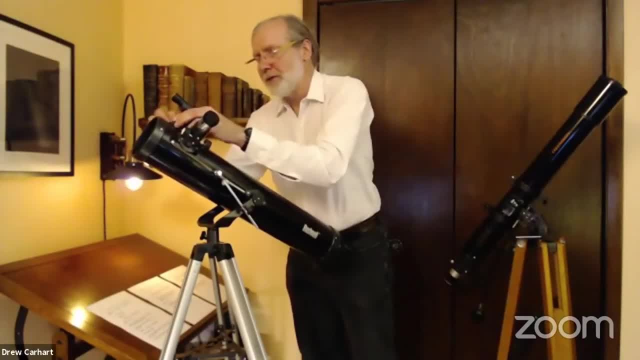 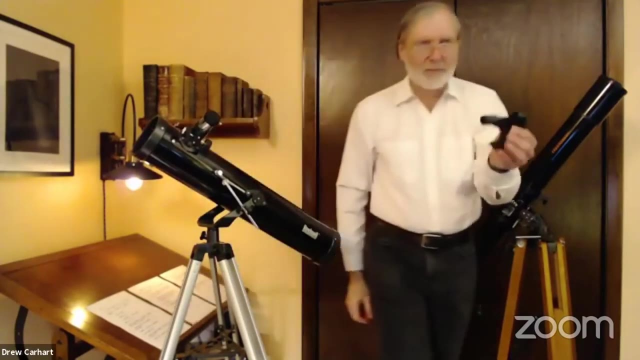 There's two little knobs on the front here that are two little nuts little knobs that hold this on, So I can show it to you a little closer up. So there's, the whole point of a finder telescope or of a finder of any sort, is that the telescope looks at a very small area. 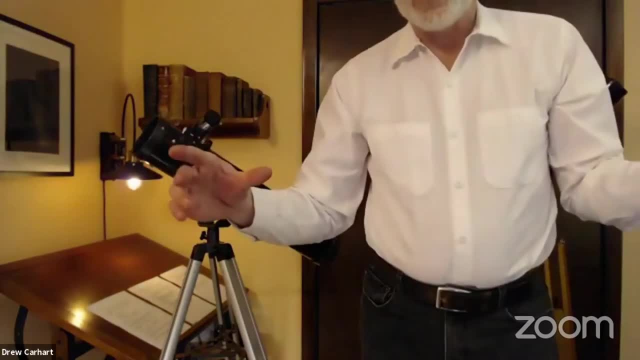 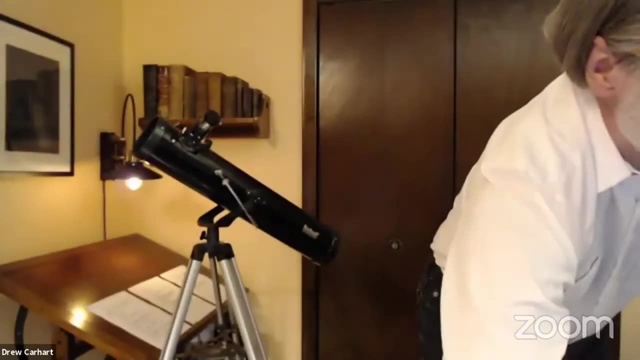 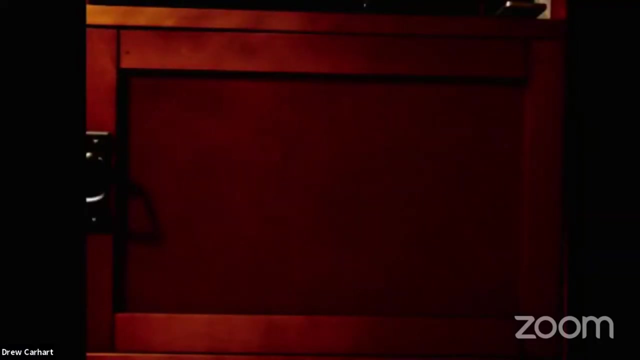 of the sky. The finder looks at a big area of the sky And if, as Jim noted, you center the objects in finder, so they're in the telescope or whichever way you want to look at that, you can use the finder to aim the big telescope. 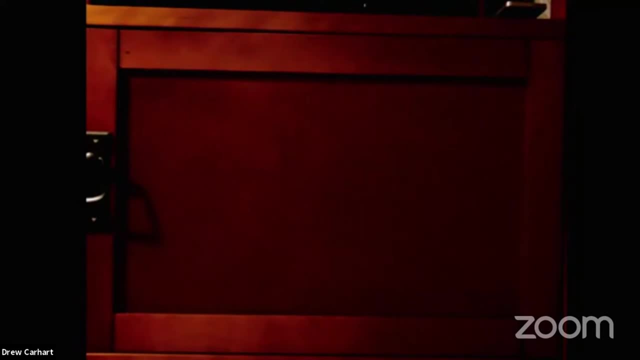 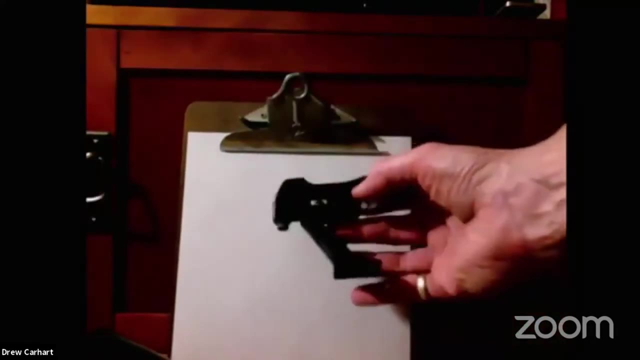 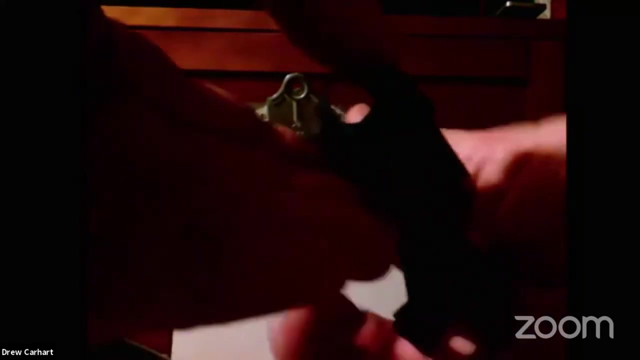 And it's again as Jim emphasized, it's a really important thing. So here's this red dot finder. Let me set this light background up here so you can see it. This does not magnify the view at all, It just has a little window in it that, if I, let's see if I can get this right. 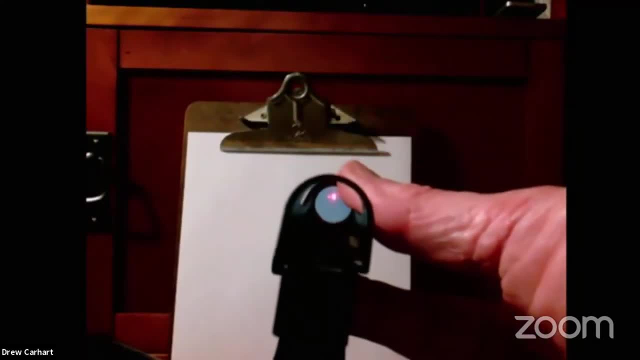 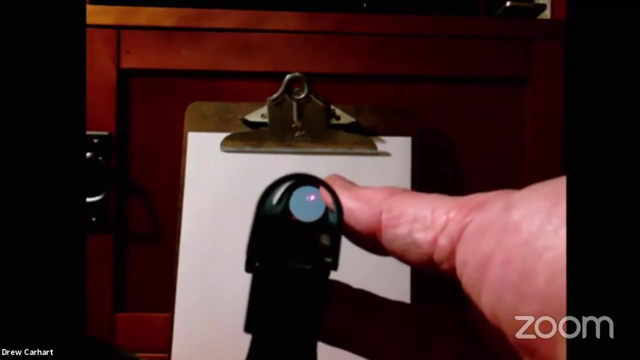 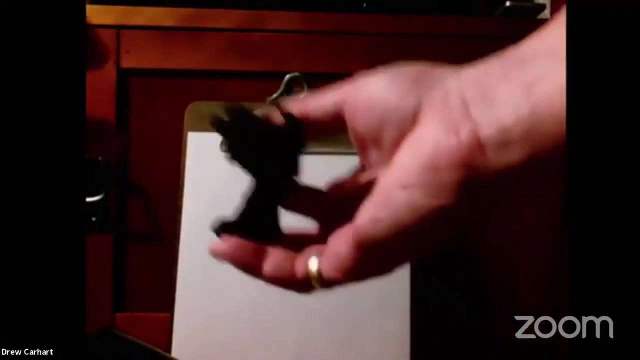 if I hold it up there, it makes a virtual dot on the little window That, in effect, to the viewer makes it look like it's projected on the sky. It's not a laser beam, It's not projecting anything on the sky, But looking through that little window I see where the telescope is pointed. 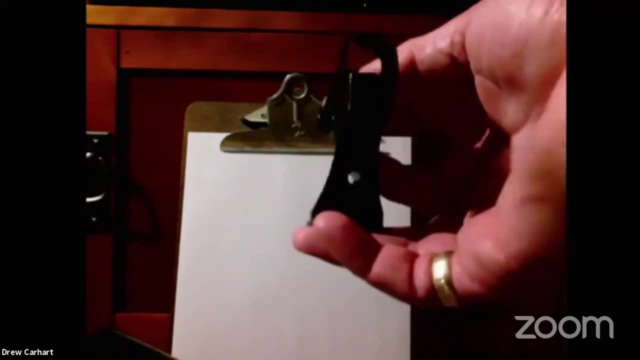 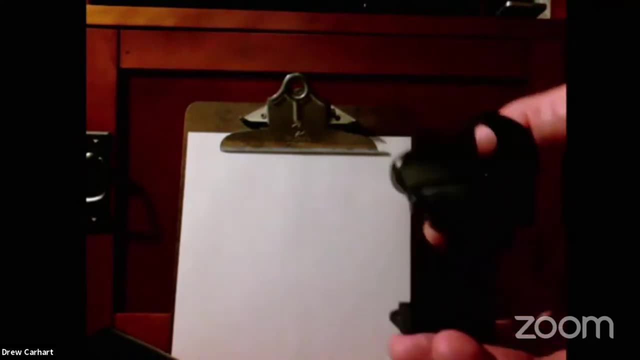 Now, when this is mounted on the telescope, as Jim said, you aim the telescope at something on the Earth: the top of a water tower, the top of a cell tower, power line, something like that that you can recognize. And again, this is something to do at dusk or even do during the daytime. 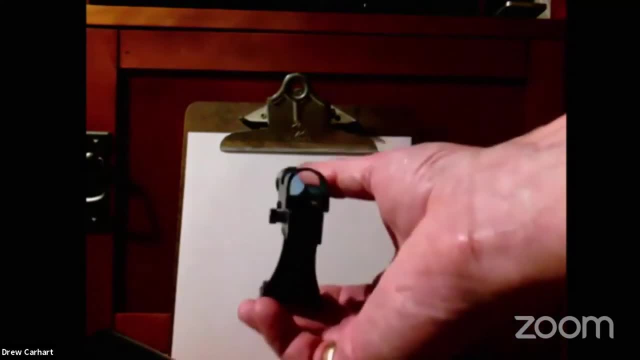 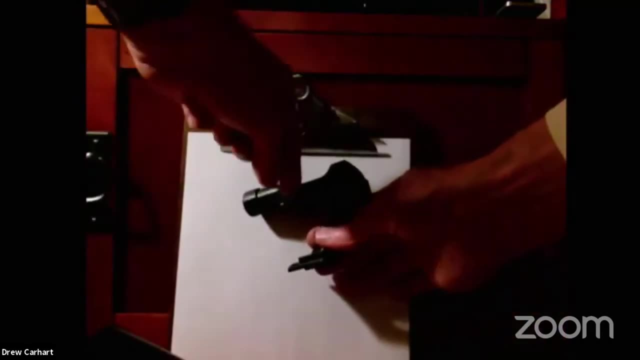 or when you're just setting up the telescope And then you look through the finder and if that dot isn't right on the thing, this kind of finder has a knob on the side that moves it back and forth and a knob on the bottom back that moves it up and down. 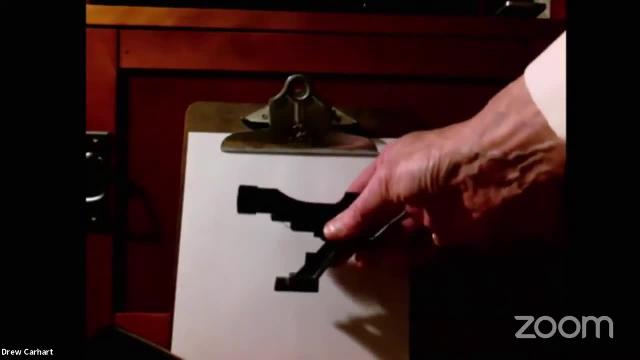 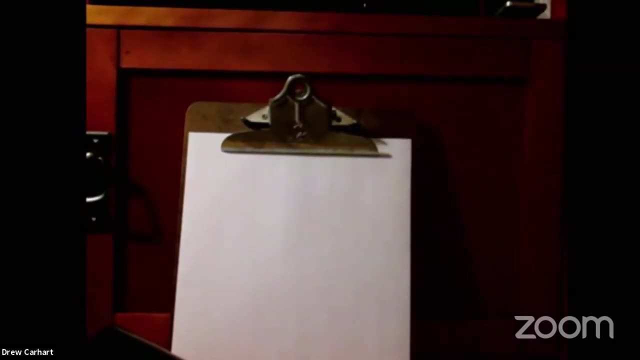 So I can swivel this little finder back and forth and up and down to get it to match the view through the telescope. And that's something that, after the first time you set up the telescope, probably when you use it in the future, even if you take it off. 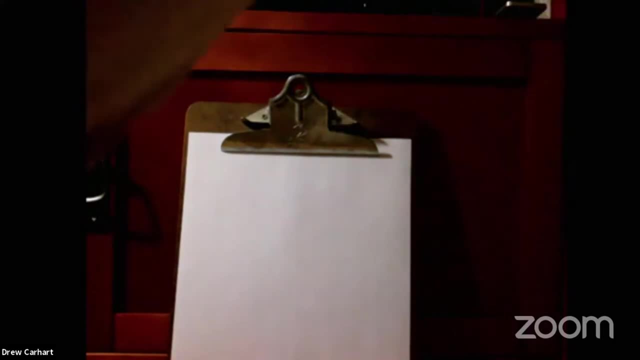 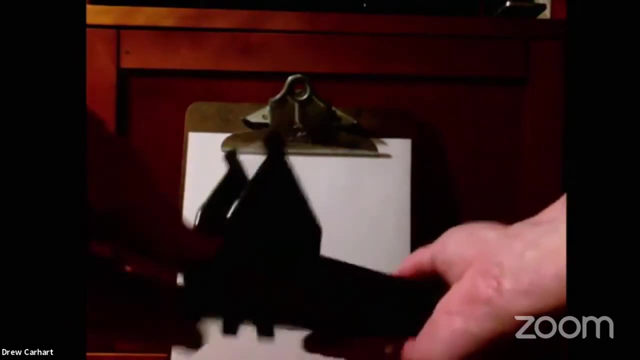 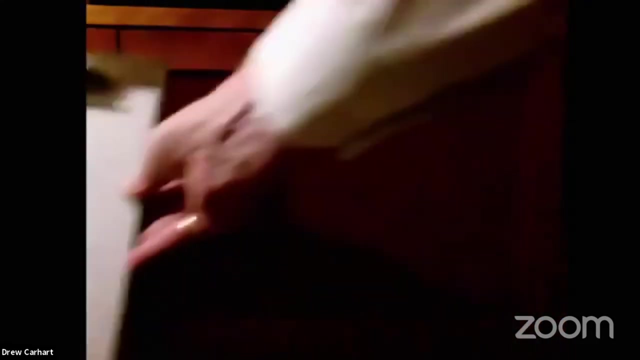 it'll probably be close. But every time you set up the telescope you reset it. This guy is another non-magnifying finder. It's bigger, so you can see this angled piece of glass that you're actually looking at when you look through it. 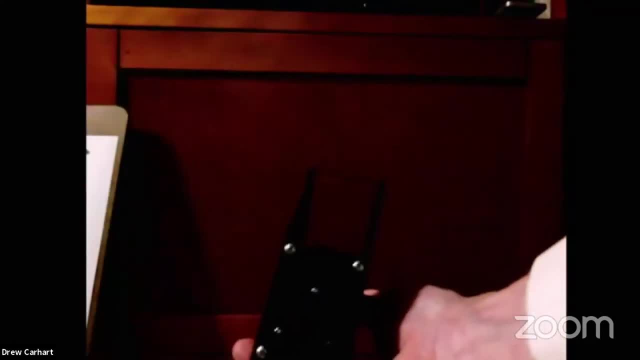 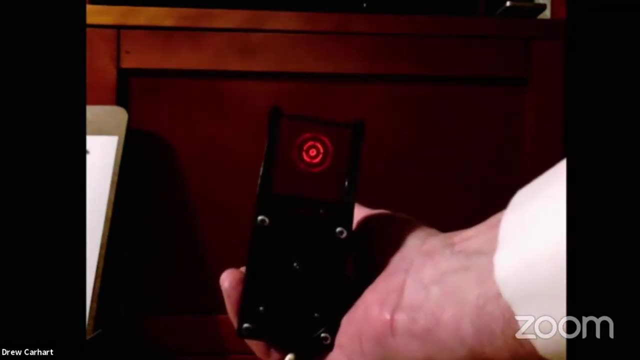 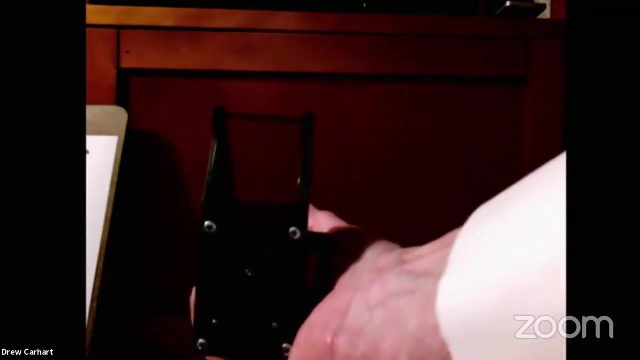 But the TELRAD, instead of having a red dot in it, it puts a bull's eye on the sky for you. So I wasn't leaning over and shaking here. I could do that there, But that's what you see. It's kind of a handy thing. 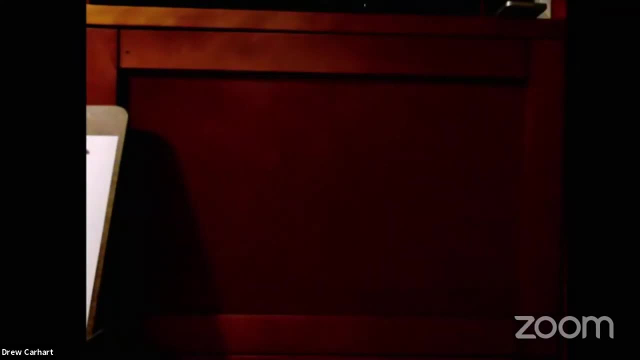 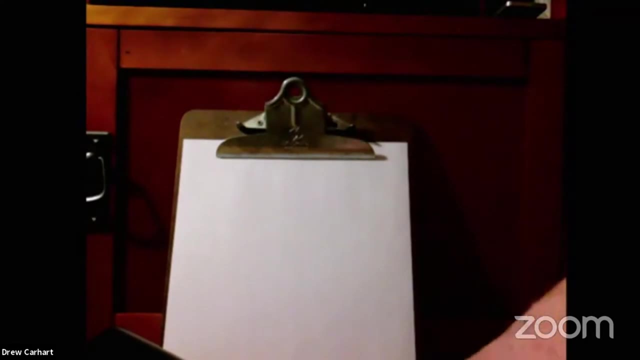 It's a much bigger finder. It's kind of handy because you can actually measure the sky with it because the rings are different sizes. It has a half-inch center ring and a 2-degree and 4-degree circle on it. This is a classic finder telescope. 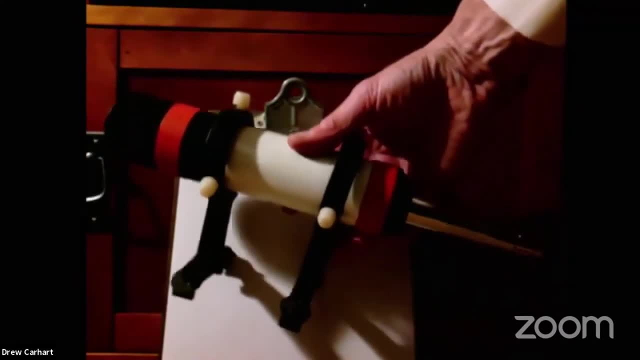 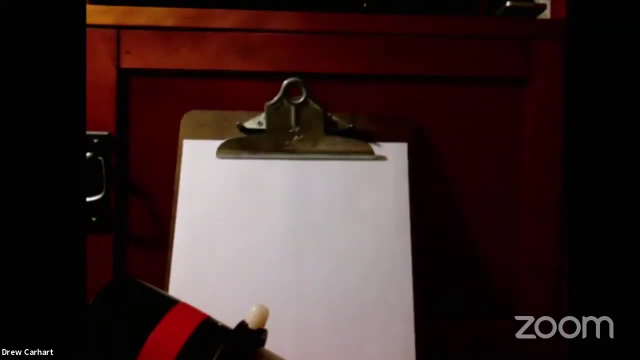 So it's actually a small telescope. If you got started in this hobby when I did, before there were these wonderful non-magnifying red dot or bull's eye finders. telescopes always have a little telescope on the side of them. Same thing. 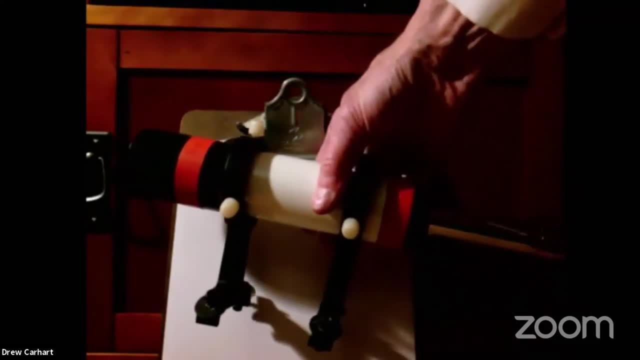 It's just looking at – it's at much lower magnification than your main telescope. This is usually five times about magnification, or six or eight or ten, And so it looks at a wider view of the sky When you look through it, if I can hold that right. 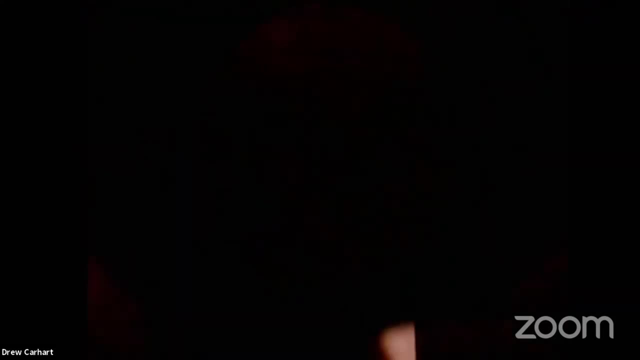 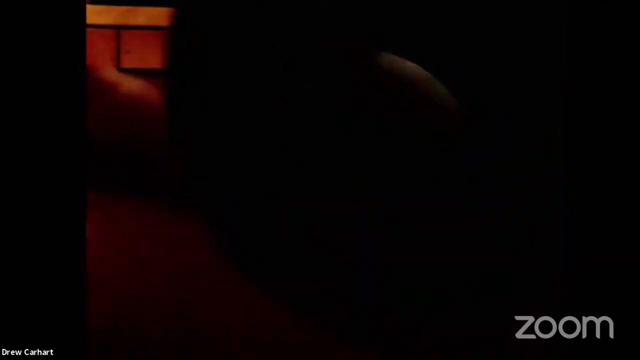 you will see the crosshairs in it. So the red dot is actually a reflection of something or other, But anyway, you can see the crosshairs as I wave it around there. So you're going to be seeing that water tower through this telescope. 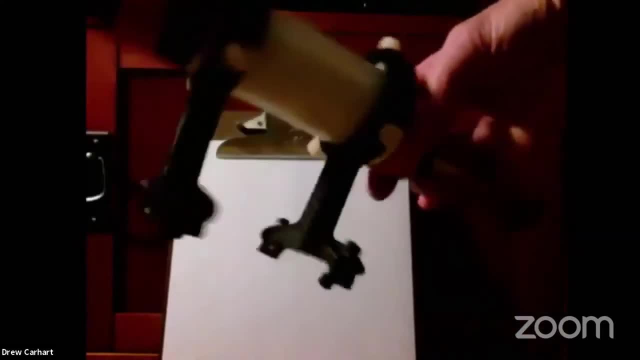 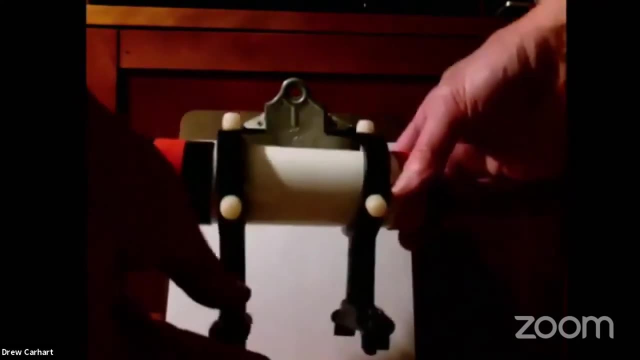 And this kind of arrangement is mounted on these rings. You just adjust these screws by tightening the one side and loosening the other to tilt it up and down or back and forth, or around to get it to aim with the main telescope. But those are finders. 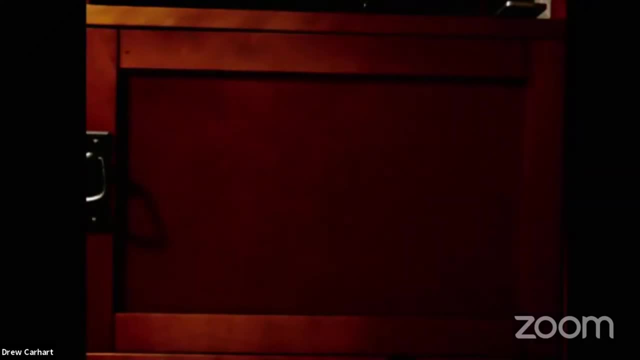 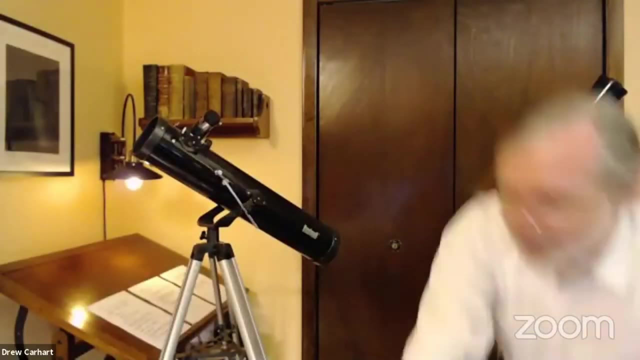 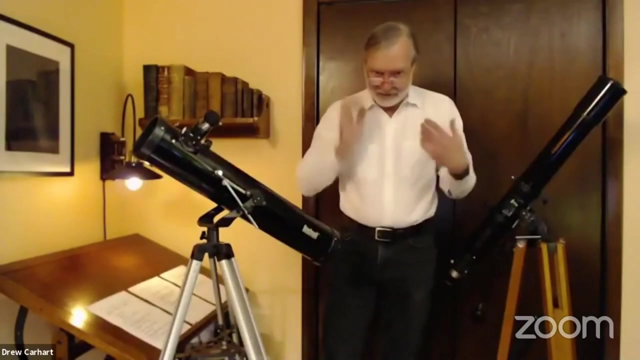 We just call them loosely. And even if you have a go-to telescope, you need a finder. So let me get back up off the floor. And really important, And I think most good visual observers will tell you that whenever they set up their telescope, 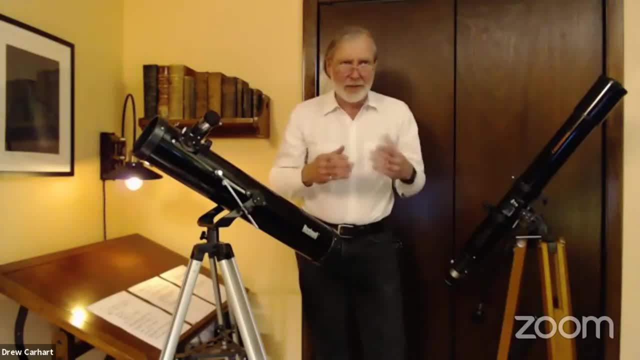 you know it's getting dark out or whatever, one of the first things you do is make sure the finder is on And maybe it'll be smack on. you know from the last time you used it, But you always check it to make sure and you adjust it if you need to. 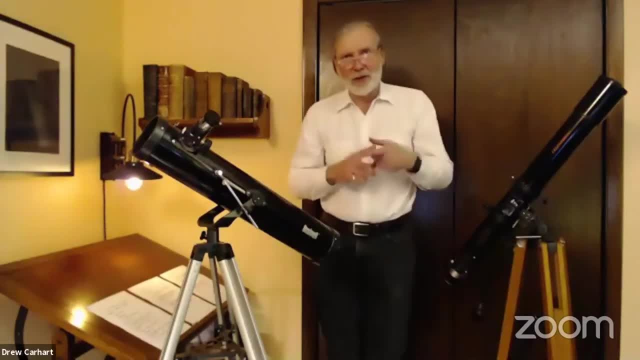 because it not only doesn't do its job, it just frustrates you for the rest of the evening if, when you put the crosshairs or the dot of the finder on the object, it's not in the telescope or it's way off at the edge. 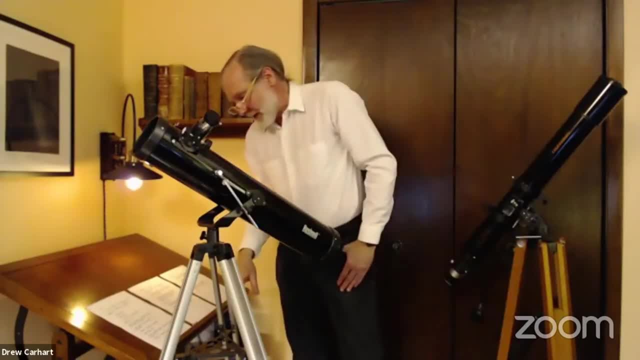 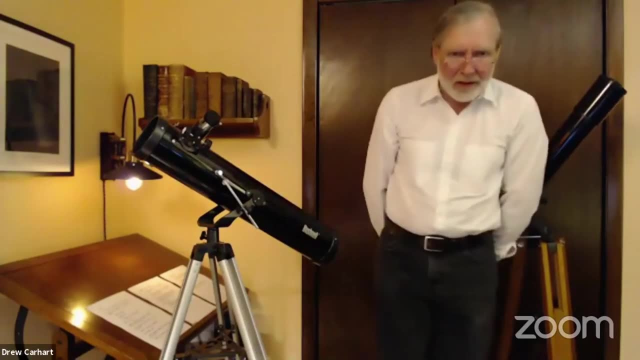 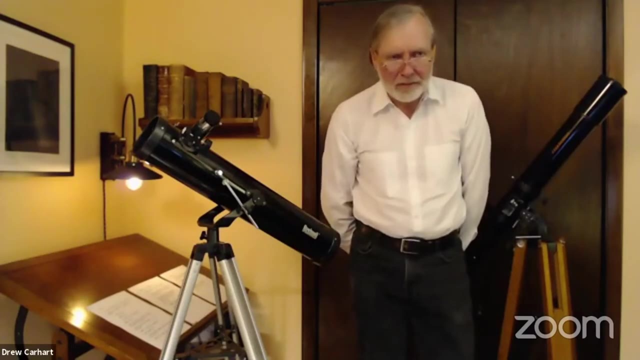 because you didn't adjust it right. Okay, Drew, we got some questions, some Facebook questions that are backing up. Maybe we can address a couple of those. So Craig says he's researching buying his first telescope and he's kind of wondering the difference between an 8-inch Dobsonian. 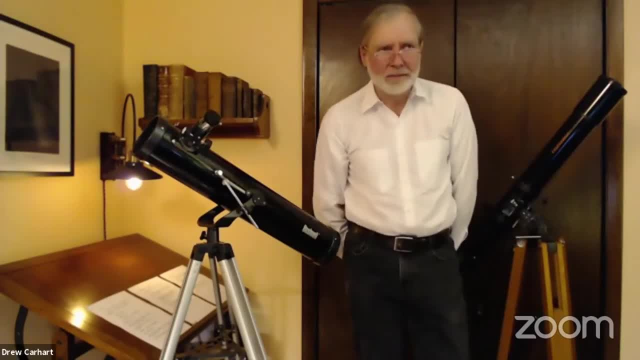 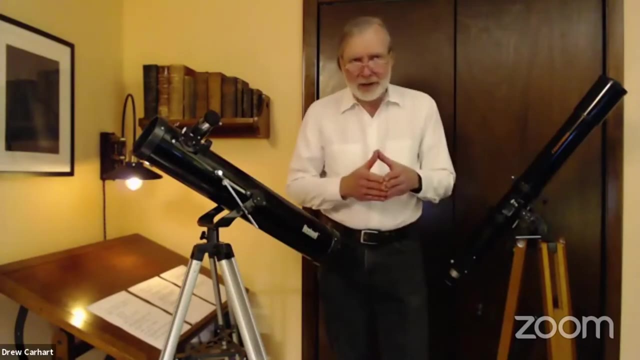 and a 10-inch Dobsonian. Can you kind of speak to that? Can you speak to why one would be better than the other or if there would be a noticeable difference? I can do that pretty rapidly. So traditionally telescopes had come in a certain range of objective sizes. 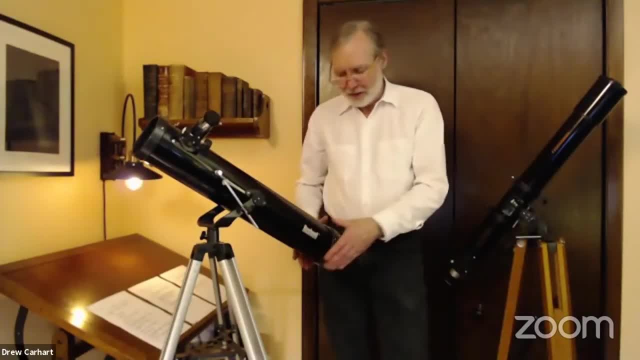 especially once you got into mirror telescopes which came in 3-inch and 4-1⁄4-inch and then 6-inch and 8-inch and 10-inch and then 12-1⁄2-inch and then 16-inch. 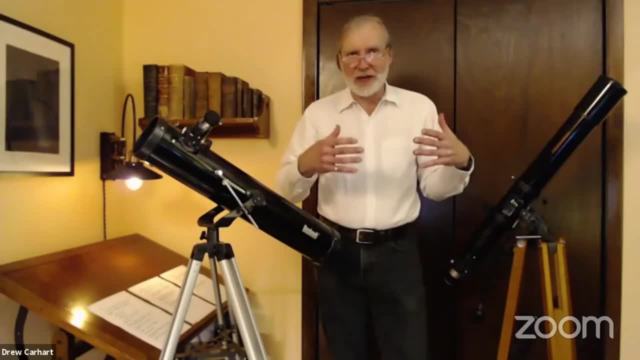 And those sizes are actually kind of based on the geometric progression of light gathering. Theoretically, if you go from one size to the next, you're going to gain a half of a magnitude of what you can observe through it, And that may not sound like a lot. 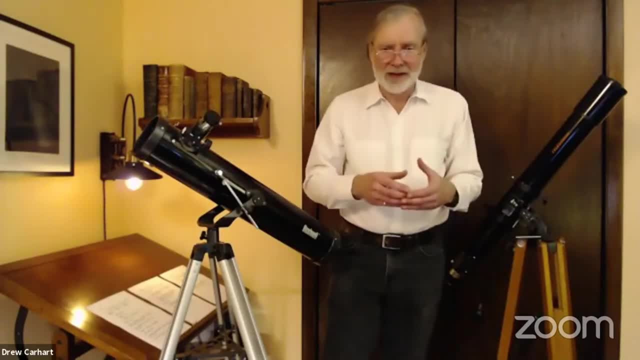 In reality, in practice, most people will find in casual observing that there's not a tremendous amount of difference in one step between, say, a 6-inch and an 8-inch telescope, or between an 8-inch and a 10-inch telescope. 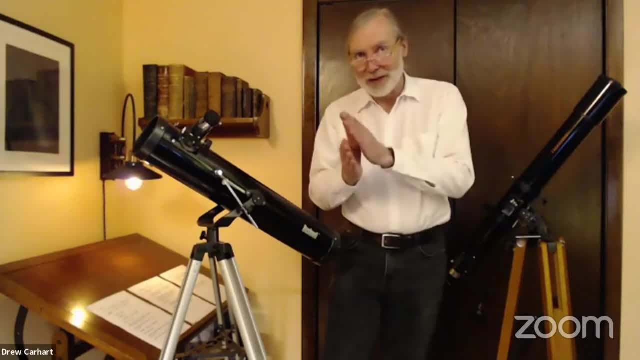 But the difference when you skip a step from a 6-inch to a 10-inch is going to be immediately obvious on a lot of objects. So that's kind of a subjective thing. That's not a really scientific way of looking at it. 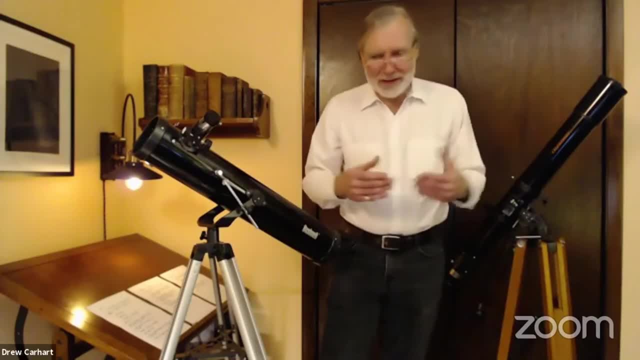 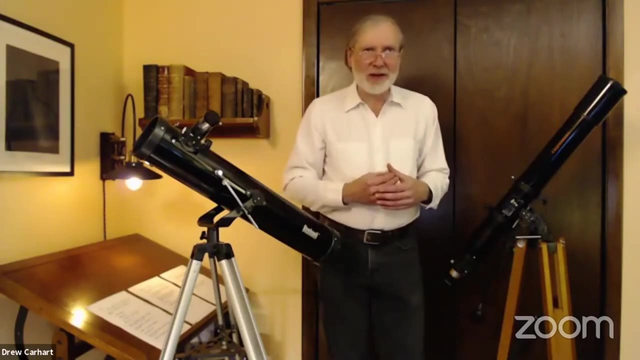 But at least back in the old days. I don't know what the current chatter is on things, but back in the old days it would be gosh. if you have a 6-inch telescope and you want to upsize, you're not going to notice a world of difference going to an 8-inch. 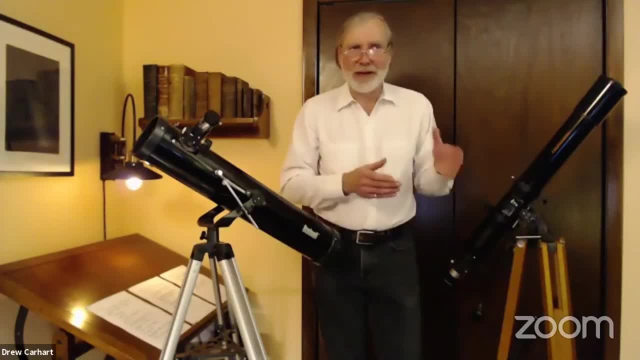 so you'd probably go to a 10.. Same thing with going to an 8 to a 10. You'd go from an 8 to a 12-1⁄2. To gain a whole magnitude of capture of what you can add. 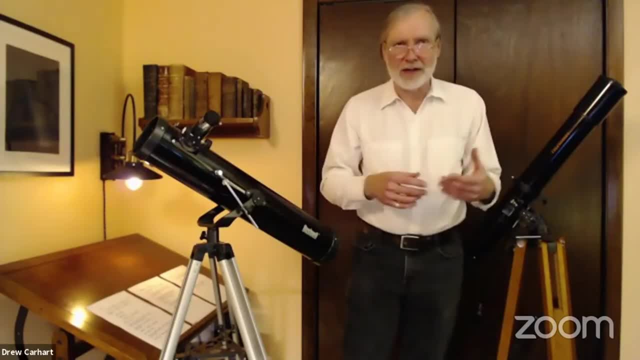 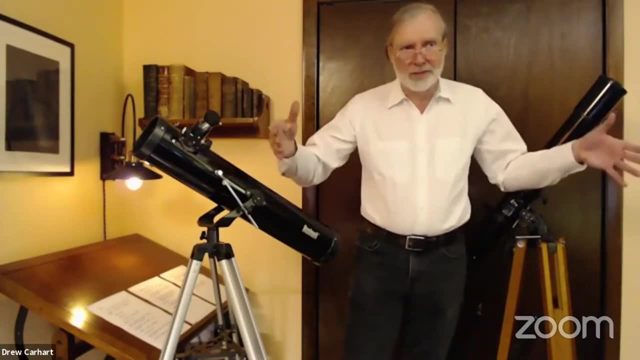 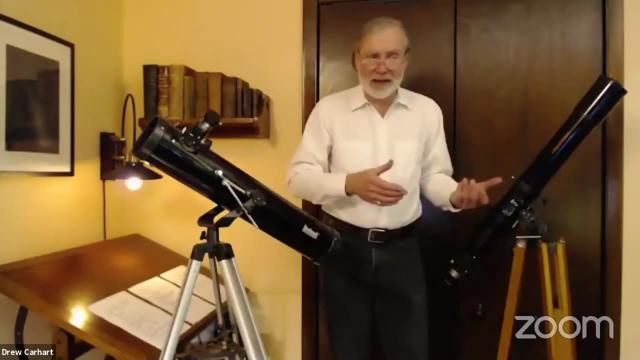 So what the difference comes in? there is the size difference, And if both of those dobs are solid tubes, not truss tubes that come apart, do they both fit in your car? Can you fit the one and not the other? Thinking of the base too, because the base is going to be. 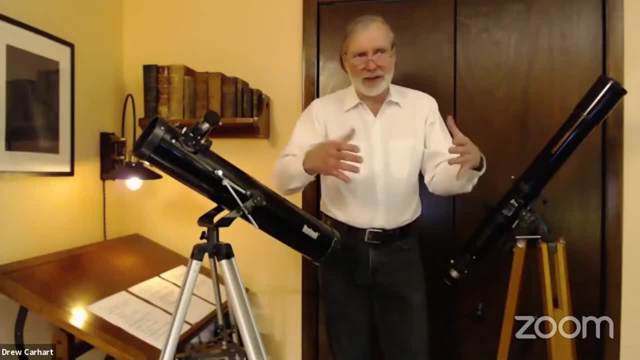 the biggest difference. actually, The base size between an 8-inch and a 10-inch dob will be quite a bit bigger. So from my point of view it comes kind of down to that You could be very satisfied with an 8. 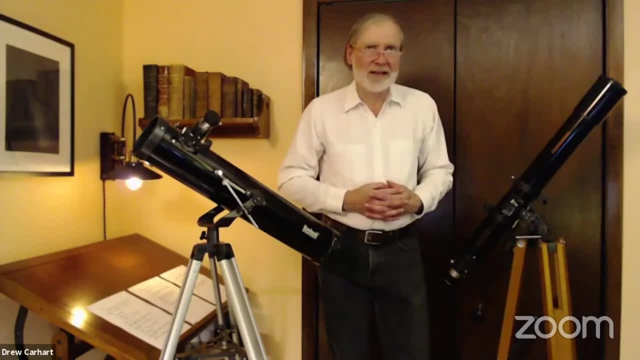 and a little bit more satisfied with a 10, but it's not a huge world of difference. On the other hand, if you've got the money for either and it's just as easy for you to handle the 10 as the 8,. 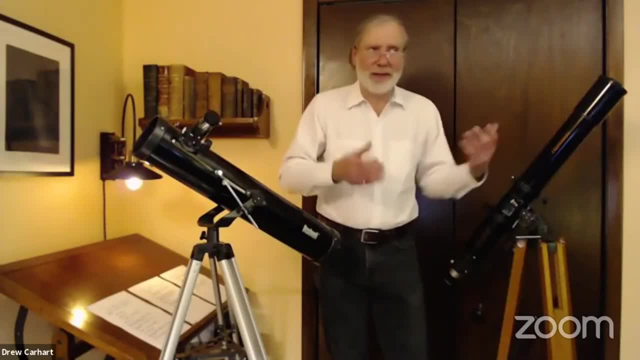 I guess I'd say get the 10, because you do get half a magnitude more of faintness. you can see out there a little fainter galaxy or a little fainter star cluster or something like that. But that's a brief take on that. 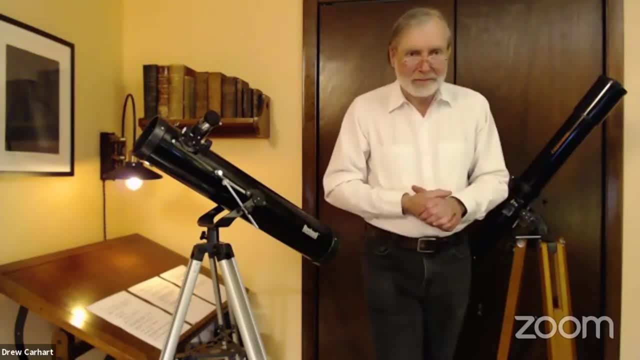 And again, it's sort of a subjective opinion thing And that really only applies to stars, because planets are bright enough anyway that you're- yeah, Your 4 and a quarter is going. I mean, this is an 80-millimeter telescope. 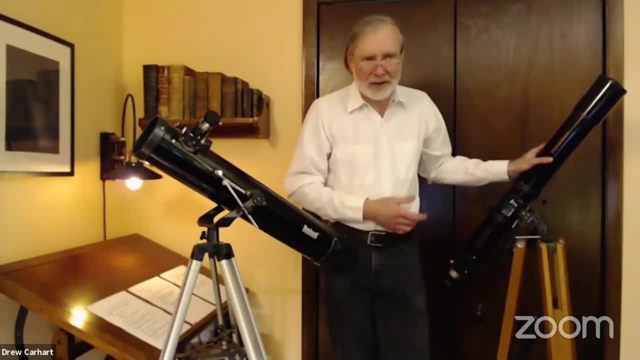 and boy, the plants are great in that you know, for the magnification, So you don't need more than that 3-point-something or other inches. that that is for gathering the planets. But yeah, it's the difference between the 8 and 10. 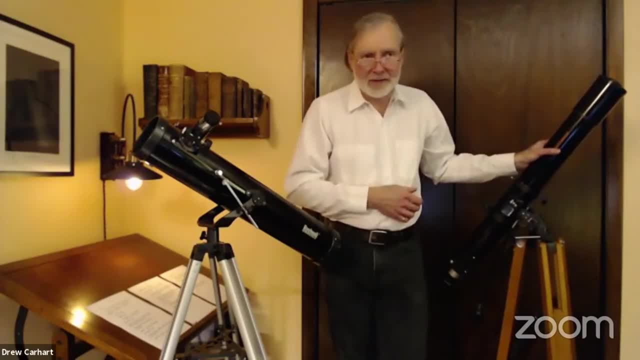 would show up in looking at the galaxies and not in the planets. And just one note, I'll chime in because I used to have a 10-inch DAB. A 10-inch DAB is pretty much the largest that you could fit in the back seat. 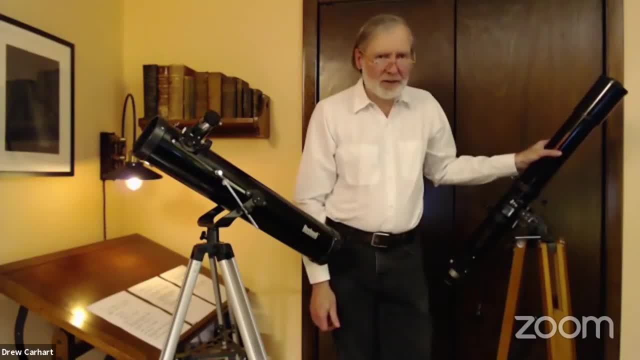 of probably your average car. Once you go to a 12-inch, you need to fold seats down and, you know, get a little more creative in how you would travel with that. You should actually get out your tape measure and see, like I say, will this fit in my car? 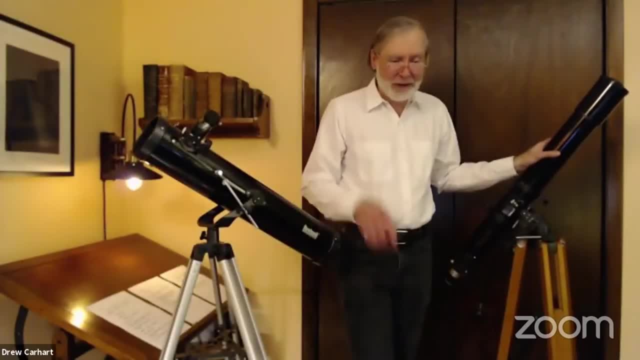 Right right, You'll be frustrated if you get a new telescope and then you find you have to get a new vehicle too. That adds a lot to the cost, Okay, So, Craig, I hope we answered your questions. If not, chime back in and we'll answer them again. 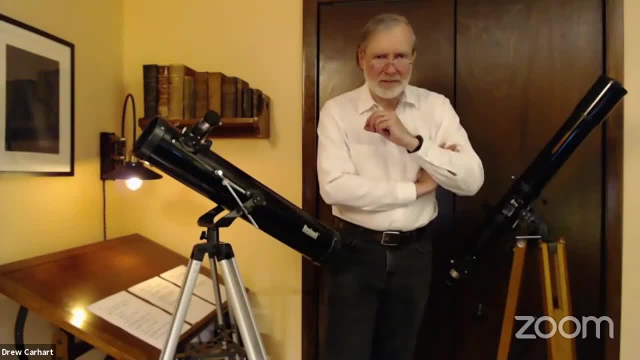 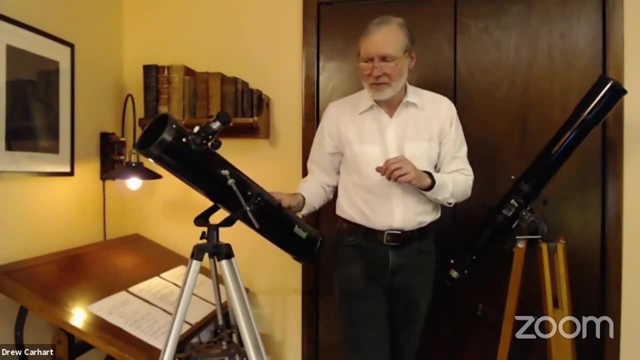 And then you don't have a DAB there but maybe you could kind of show on the Newtonian. So Greg was asking: are there kind of any tricks for using a Dobsonian? You know, can you kind of show how you would move a Dobsonian around? 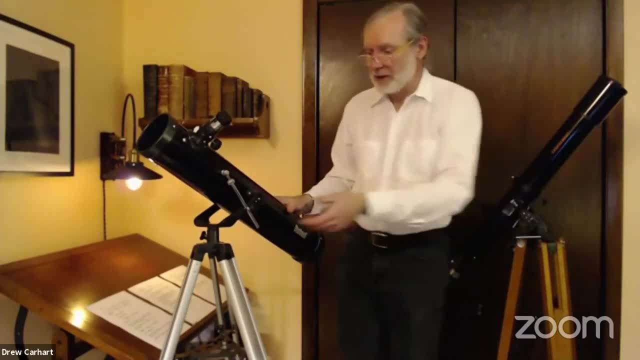 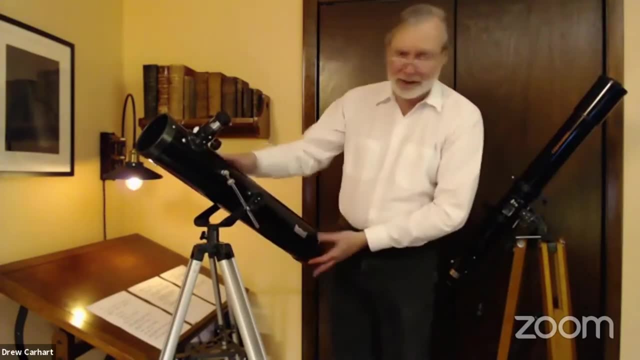 Absolutely Yeah. So the Dobsonian is pretty much the same telescope, except instead of being on a tripod- well, they're both Newtonian-reflecting telescopes, so they have a meter in the bottom. The Dobsonian is just the mounting port. 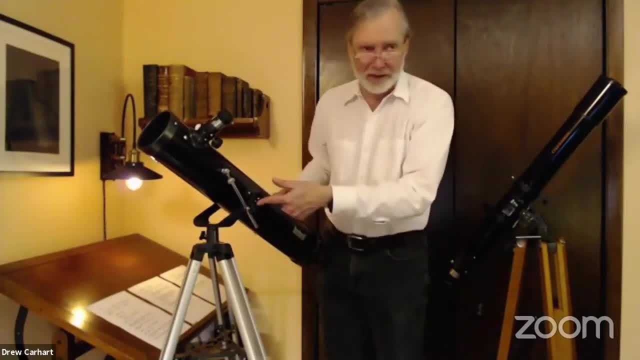 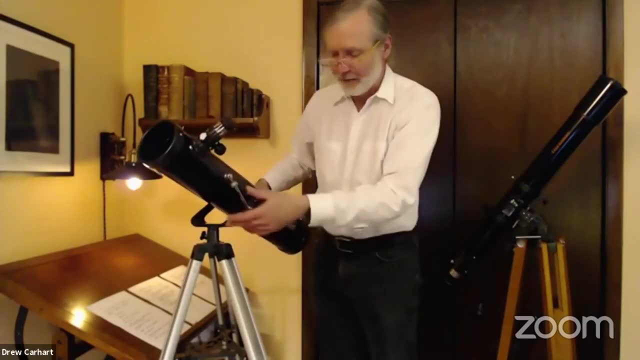 and it is basically this mount. It's a central pivot that the tube turns up and down on and then a base that it rotates on And in this case all of that is up here on a tripod In a Dobsonian that sits on the ground. 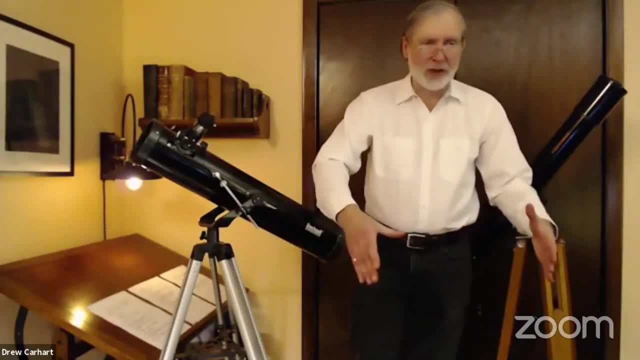 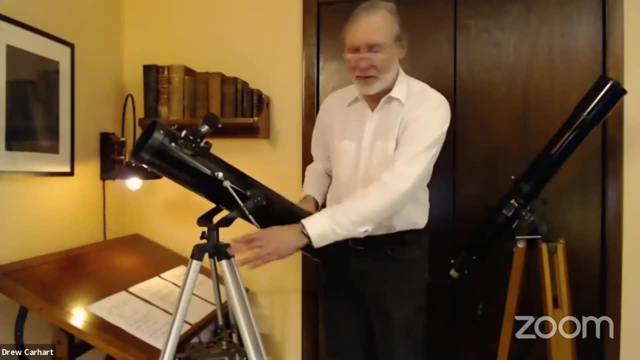 the base is up here. It's a sort of box generally that does this same thing. It has side pivots with the telescope tube and a base that swivels up and down. This is part of learning your you know. 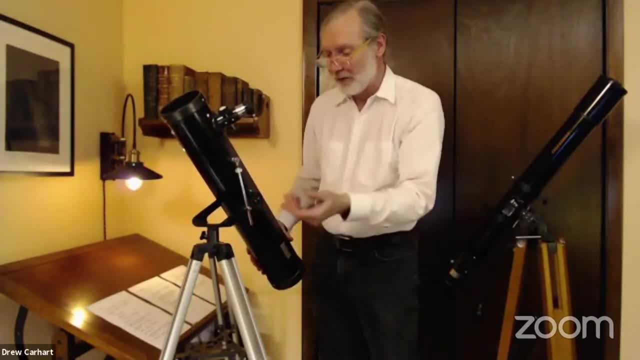 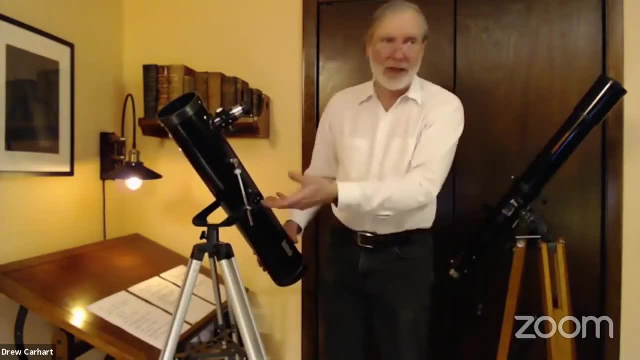 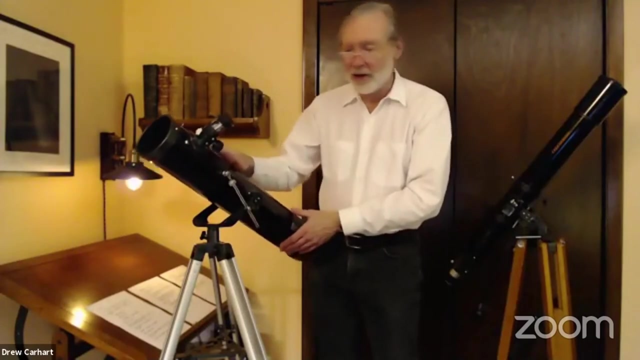 way of using the telescope period You don't have in the basic telescope. you don't have any sort of readout of where it's pointing or something You're using your finder telescope and your maps of the sky that I'll get to. 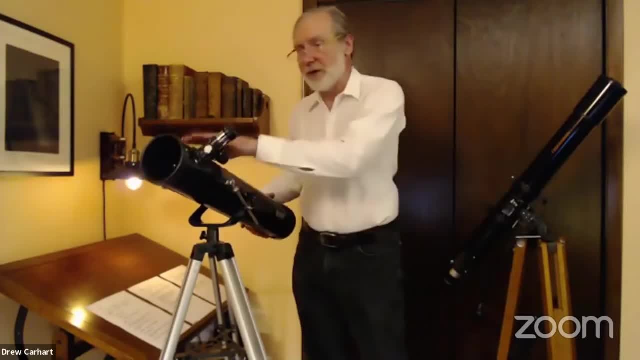 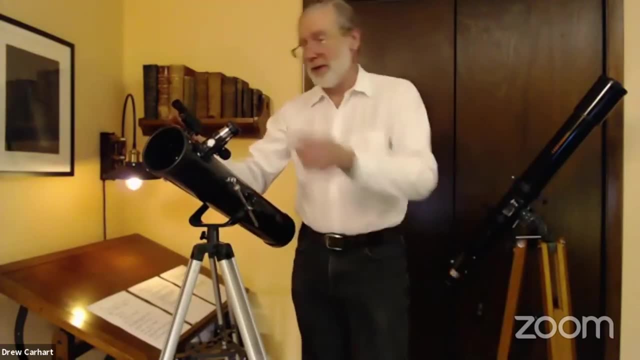 And saying, basically, that's really simple. If I see where the moon is over there, I use my finder, which I stole off this one, and I point the telescope at the moon, And that's simple enough. Or if it's Jupiter or whatever, that's simple enough. 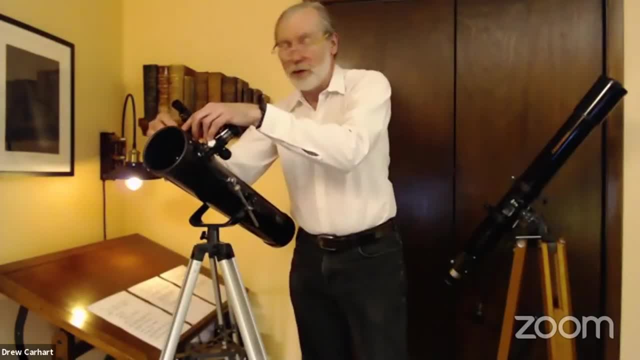 When it comes to other things, you have to learn your methodology for figuring out where those things are. Um, And that applies pretty much to any manual telescope. This one back here is the same thing. This is on a altism, It's not also. 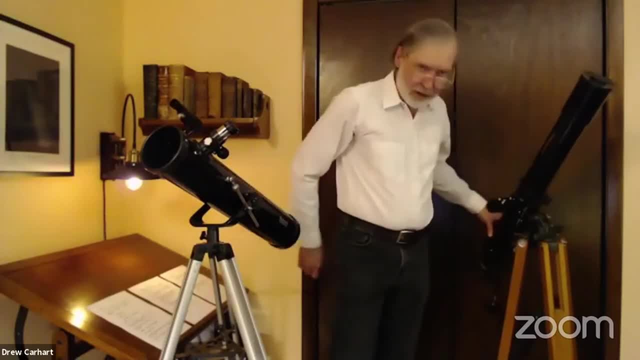 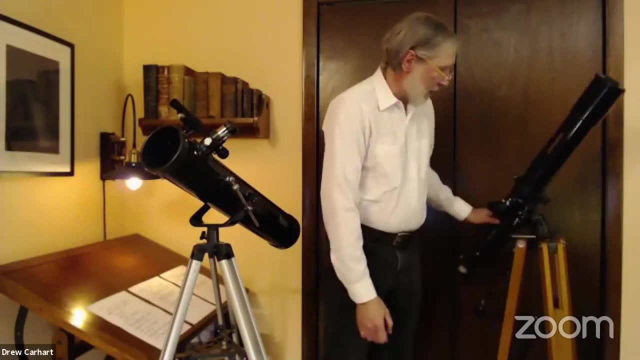 And the finder on this telescope is actually not going to see it well, against the closet here. It's actually mounted down the side of it here, But this is a red dot finder here And we use this by turning on that finder taking out our star charts. 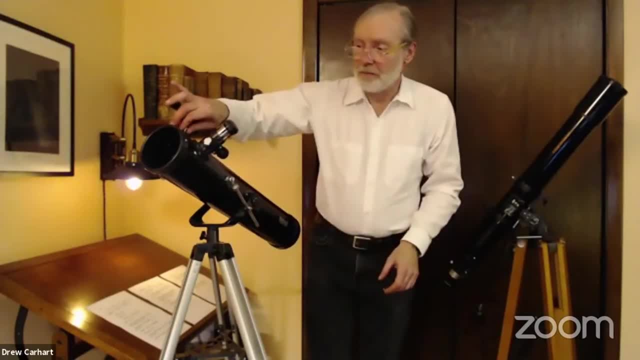 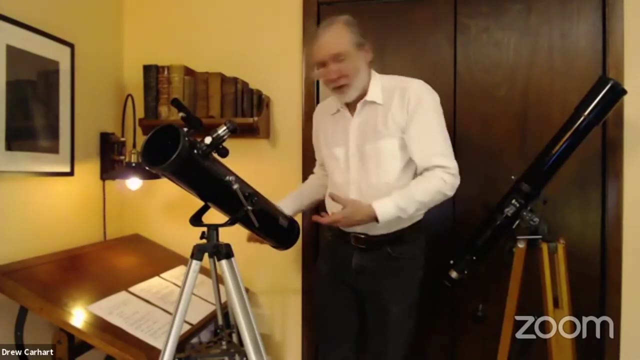 and uh, aiming that dot in here onto the point in the sky where we think the galaxy is or the star cluster is, And that's just based by looking at a chart. The chart can be a book with a map. It can be on your phone. 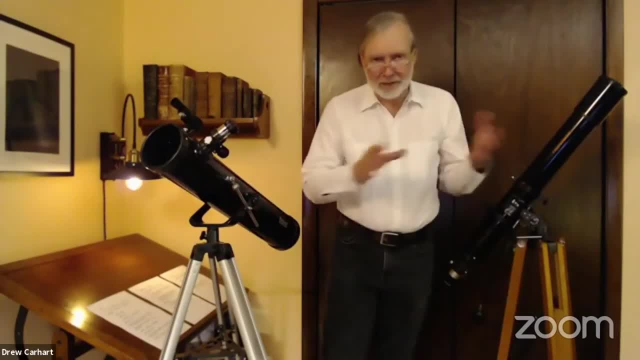 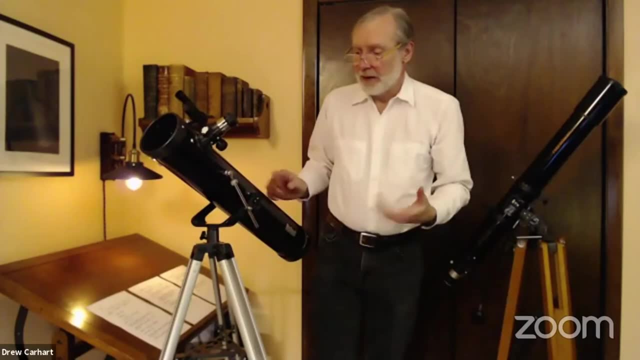 if you're using, you know, a phone app that you can zoom in on and see the locations of things in the sky. Um, But again, it's this basic back and forth and up and down. The trick is, once we've got something in here. 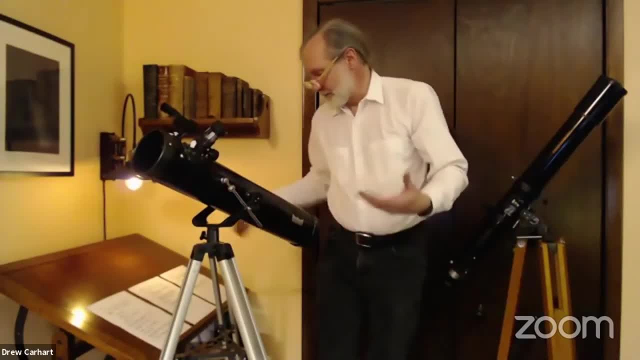 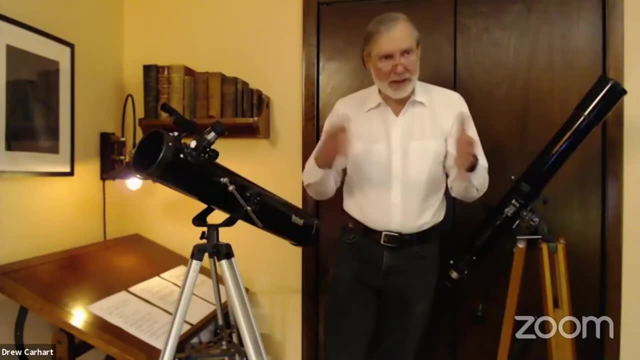 I'm just going to talk about. talk about mounts a little bit more Again. Jim's telescope that he was demonstrating on has a motor that's tracking the sky- Actually a few motors that are tracking the sky And that one it's turning it sideways. 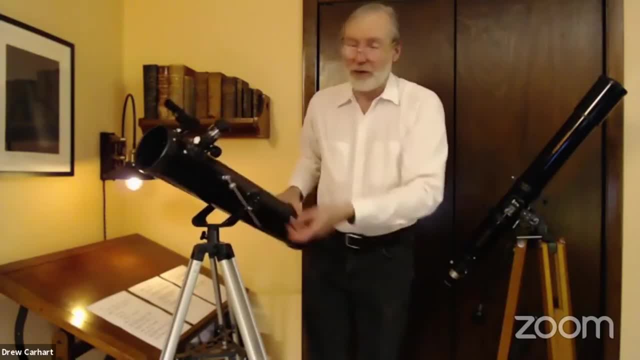 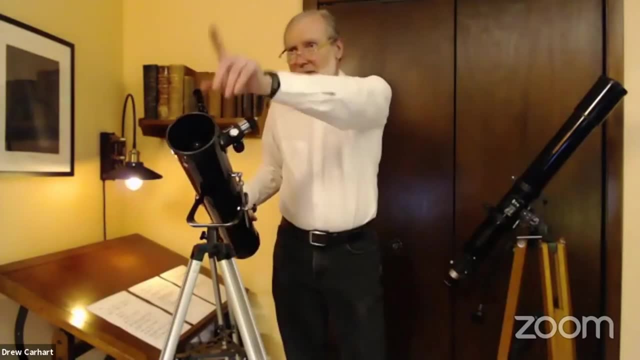 and up and down at the same time to follow things across. You have to do that manually with a manual telescope. If something is, If I'm facing south here, which I am, and something If the moon's up here through the evening, 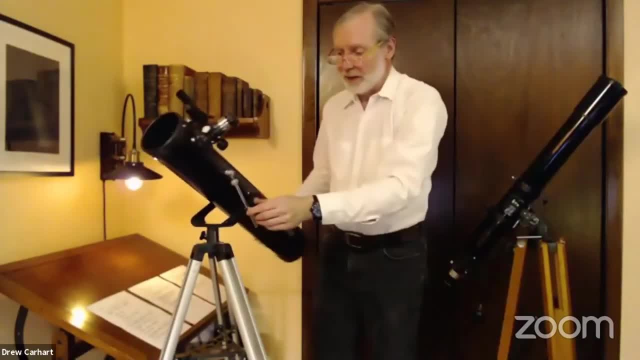 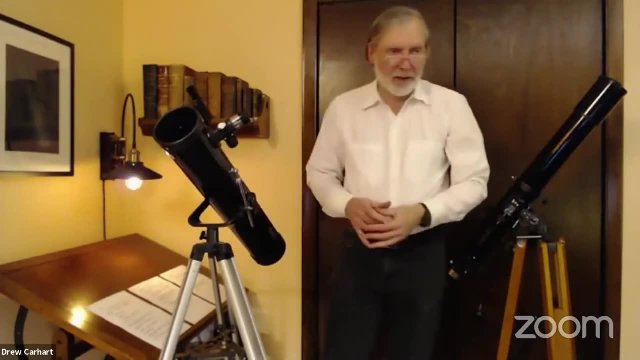 it's going to head west and downwards, so I have to constantly be adjusting this over to the side and downward as it goes down the sky. It's just something you practice at doing, Um And moving, So I don't know if it. 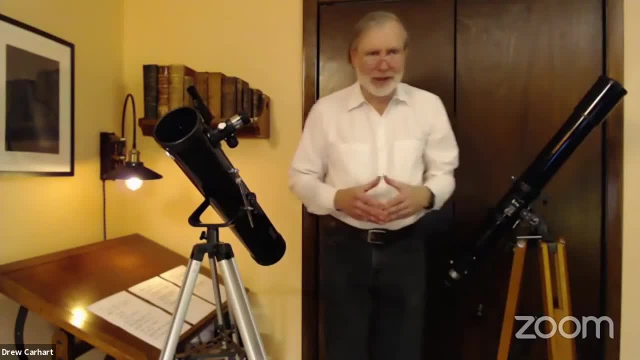 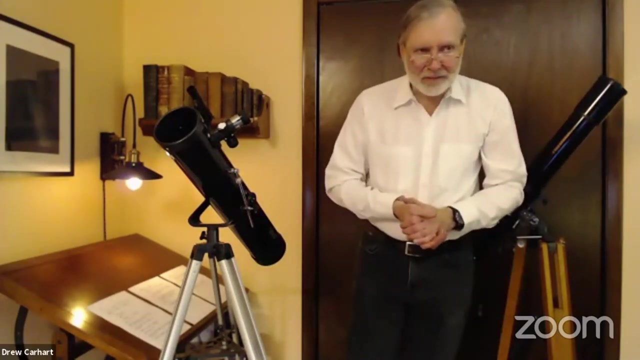 That isn't a whole class in Dobsonian use, but um, It's really basic, fairly straightforward, but it does take practice. I don't know if I don't know if I answered the question well or Yeah, Greg, if you have any more questions. 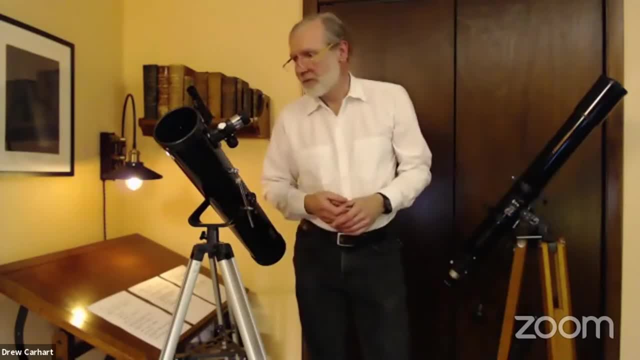 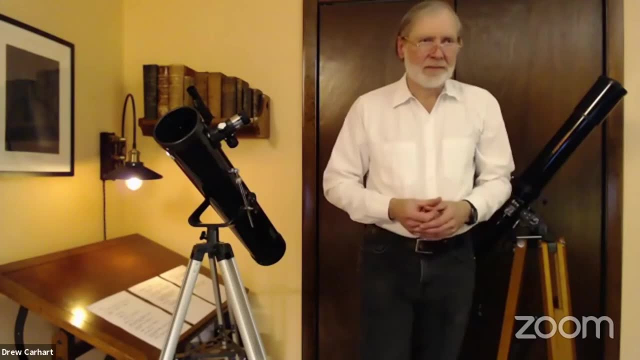 we can kind of chime in One thing. I just There's a little bit of a discussion on telescopes happening on Facebook and I think one thing to chime in, there's kind of no perfect telescope. That's why there. 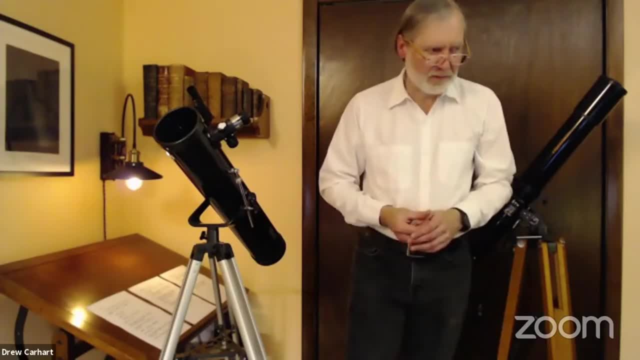 If there was a perfect telescope, that would be. They would only make that one telescope. There's Newtonians and there's refractors, and then there's kind of the Smet Cascarines, which are the combination of the two. 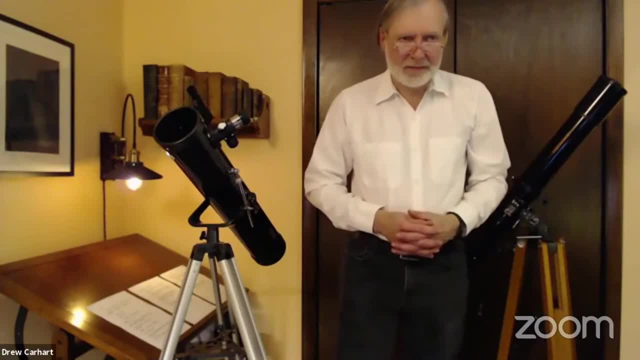 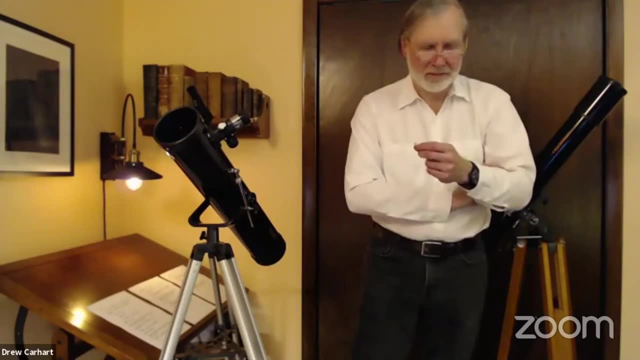 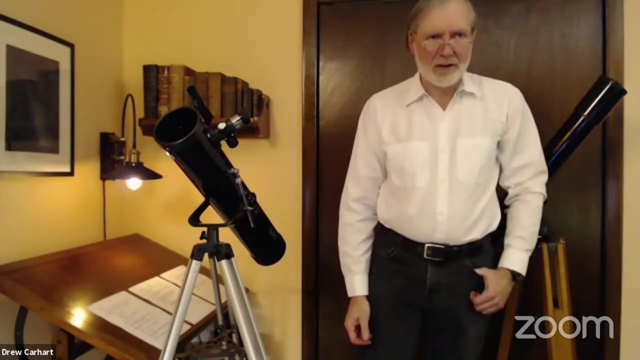 and each one kind of shows the sky a little bit differently, and some are more compact than others and some are, you know, bigger than others, and it's really kind of a matter of personal preference when it comes down to it. If you're watching us on Facebook, 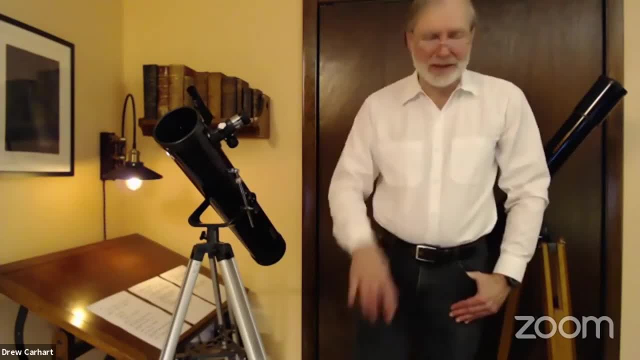 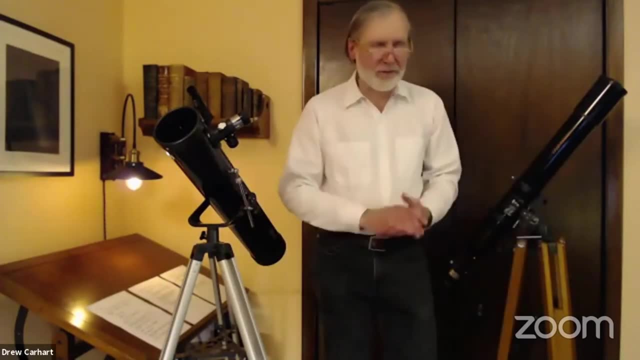 our old videos are on Facebook, but I would recommend instead going to our YouTube channel. I think it was our October fundamentals presentation. October of this last fall was on choosing a telescope and I went in depth on those differences between the different telescopes on that. 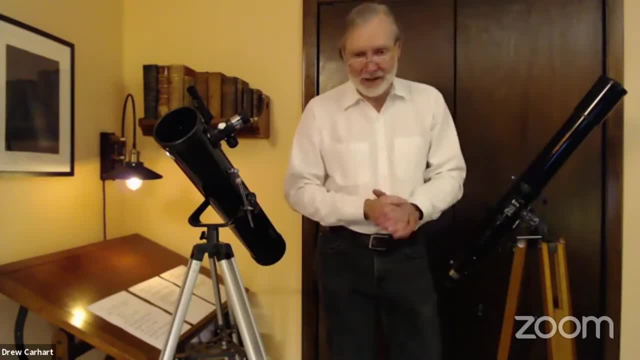 so I refer people back to that, because I covered those points and that point exactly that there isn't one best telescope, that we really need to pick telescopes that match our ways of wanting to do things and our interest in what we want to see in the sky. 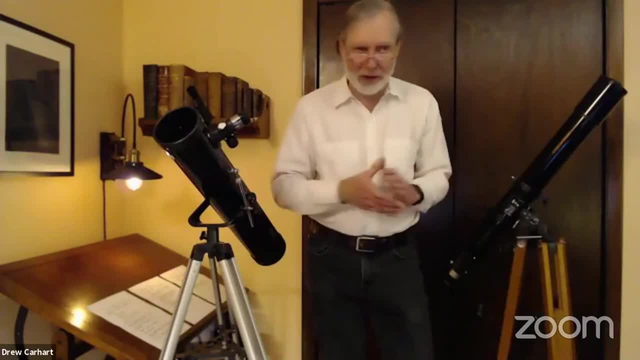 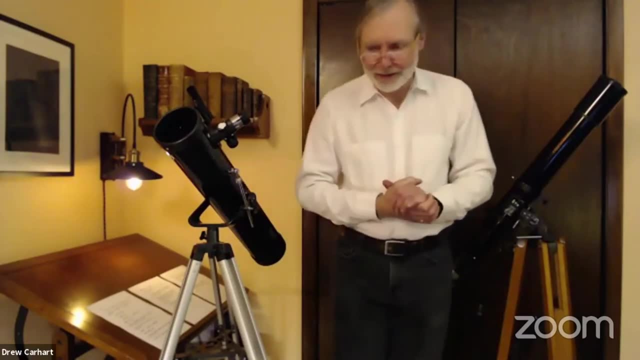 you know what clicks for us as far as we want a computer or we don't want a computer and things like that. So there's a good hour plus on just that specific topic in our October fundamentals program which is available for you. 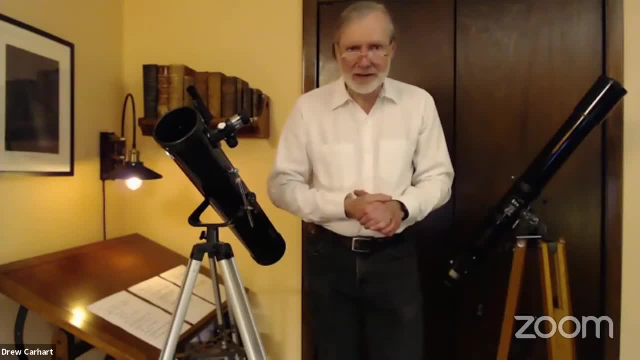 Anything else that I should touch on here. One more thing Again. they're kind of discussing buying a 10-inch Dobsonian or an 8-inch, and I think they're talking about a Smith-Cassegrain. The big difference there. 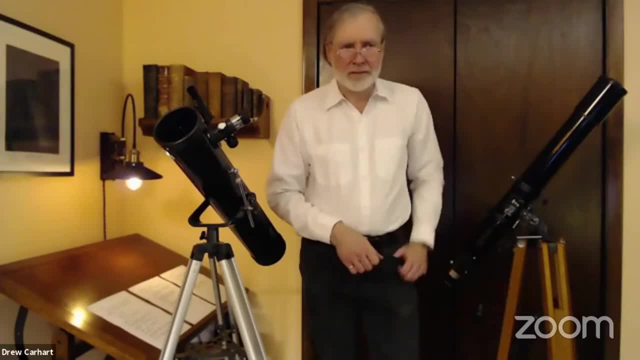 probably more than the aperture is the cost that would be associated with it. and when you talk about like a Celestron 8SE, the bulk of what you're paying for is the gears and motors that drive that telescope around. If you're willing to do everything manually, 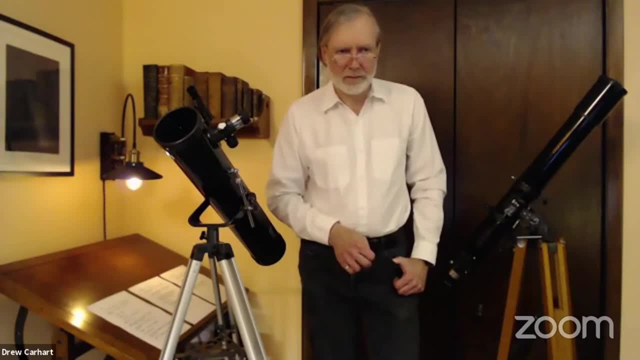 a 10-inch Dobsonian can look at the same stuff in the sky. It's just if you're, You have to find it yourself, You have to drive the telescope yourself. So again, it's kind of personal preference, but if 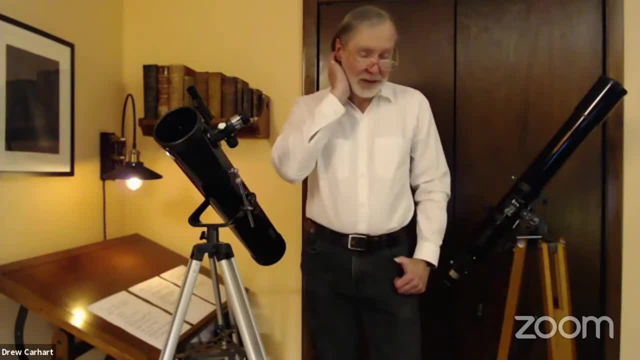 It's entirely personal preference. It's entirely what works for you. As I pointed out more than once during the presentation, in the fall on choosing a telescope, there isn't one best telescope. There's a lot of different telescopes for a reason: because they all have different features. 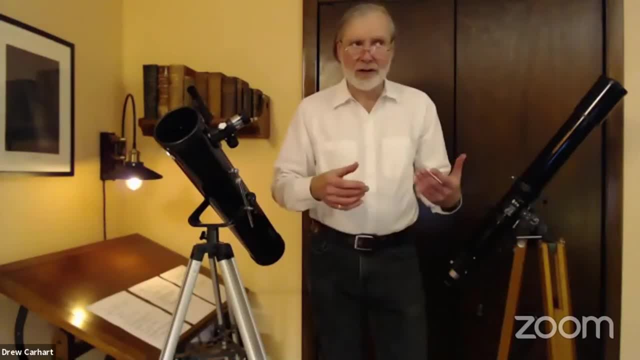 including different mountings, and they're all better for one person or another, or one thing or another, one use or another and in the end, the bottom line is: the best telescope for you is the one that you'll actually use. If you get a telescope. 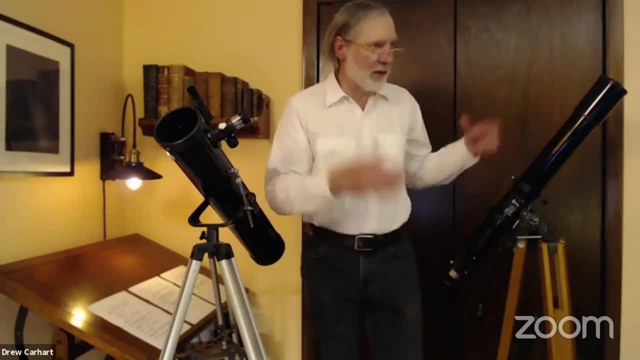 that has no computer on it and you're like: I don't know how to run things that don't have computers on it, then that was a mistake If you get one that has a computer on it and it does nothing but frustrate you. 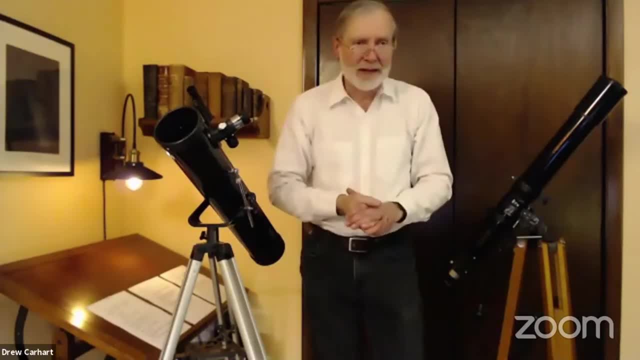 when all you really want to do is point that thing at the sky over there, then that was the wrong telescope for you. So again, it's a matter of what clicks for you, what gives you the most pleasure and what gets you out. 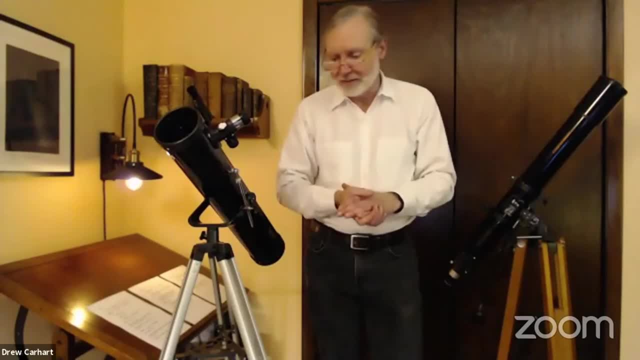 actually observing the most. Again, there's the classic thing of people buying too big a telescope because big sounds really good, but if you never take it out because it's too much of a hassle, you take a big telescope out and lug it around. 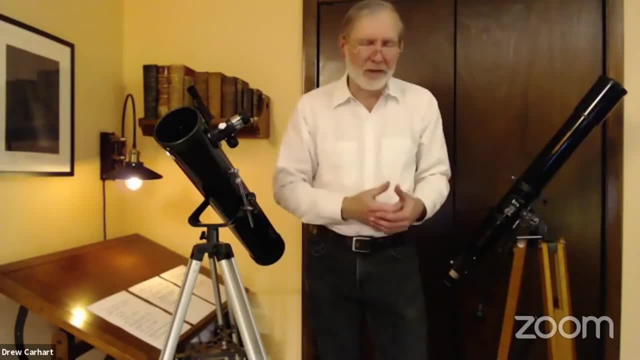 and assemble it all just to look at something for 20 minutes tonight, then that's not a good telescope because you didn't actually use it, whereas a smaller one that this you can leave set up in your living room or your den or something or other. 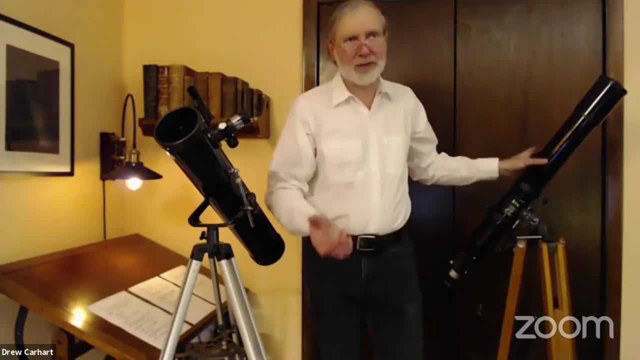 and pop outside and pretty much assemble and be observing in less than two minutes probably- and maybe you'll use that more- and all of a sudden this became better than a 20-inch telescope. If you use it, you'll use this one and you wouldn't use. 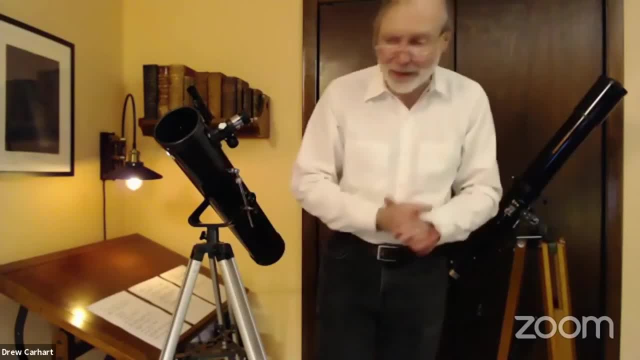 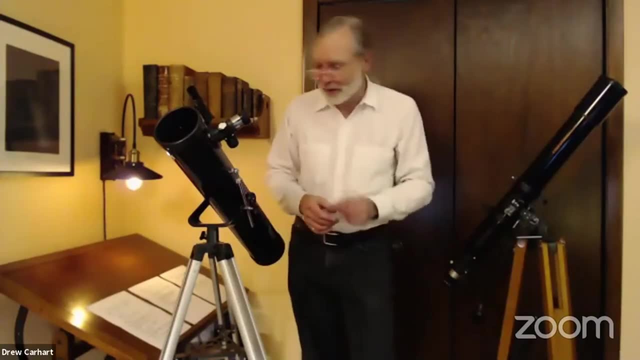 the 20-inch telescope. So yeah, again, that's a different program on going back a step and picking the telescope. I do recommend the October program, not just because I gave it, but it covers a lot of these points really in a little bit more detail. 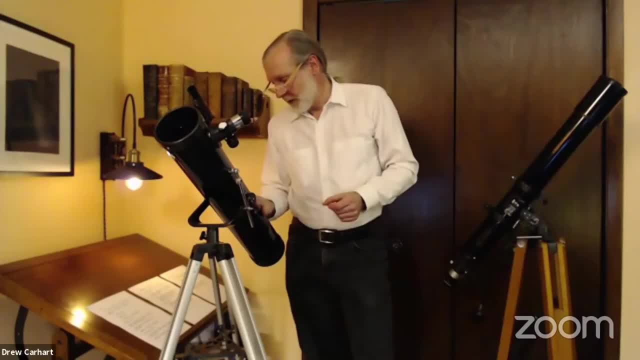 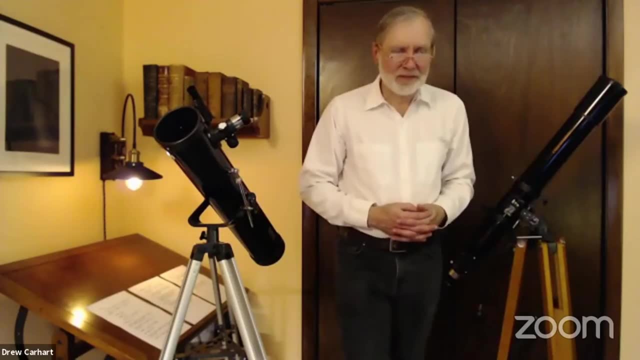 Okay, One more question and I'll let you get back to your program. We got a lot of questions tonight. This is great. I don't think we've ever had this many questions. So Joseph asks any hints on swapping eyepieces during an observation. 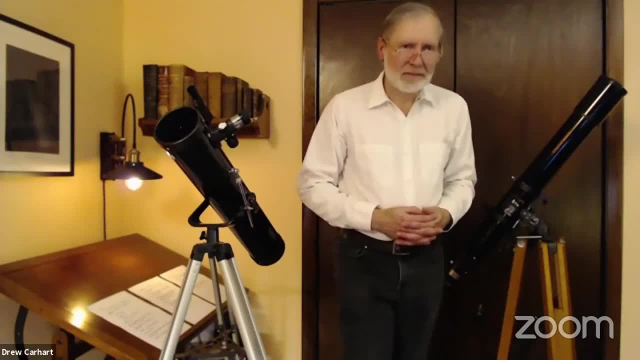 I usually knock it out of view and the focus also changes. And he says: stupid question: do you ever grease the inside of the eyepiece holder? Starting out with the no question, stupid, I would never grease the inside of an eyepiece holder. 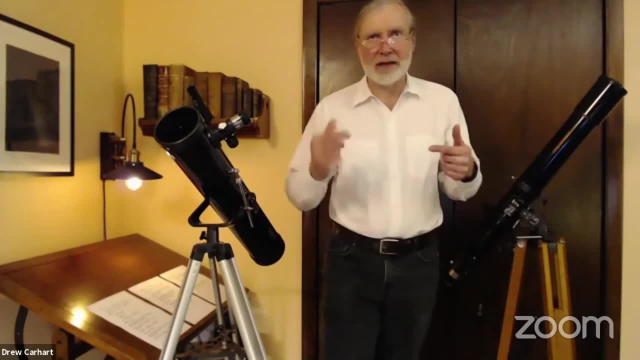 because you certainly don't want to take any of this and getting into the eyepiece and any lubricant really. So addressing that particularly, yeah, that's an issue. It's going to vary from telescope to telescope with how much problem you have. 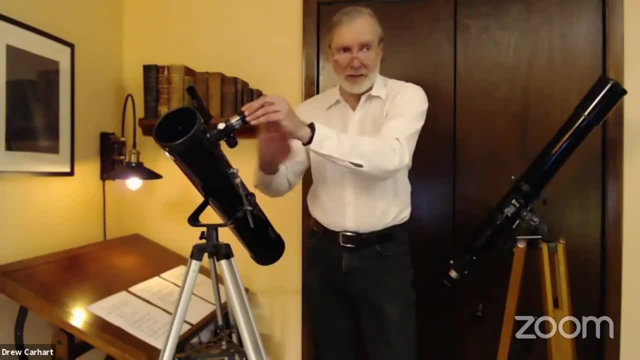 getting an eyepiece out and putting another one in without something moving around a lot. That initial thing I said about tightening up your mount is very applicable there, but also quite a few different kinds of mounts. Again, there's a lot of different mounts. 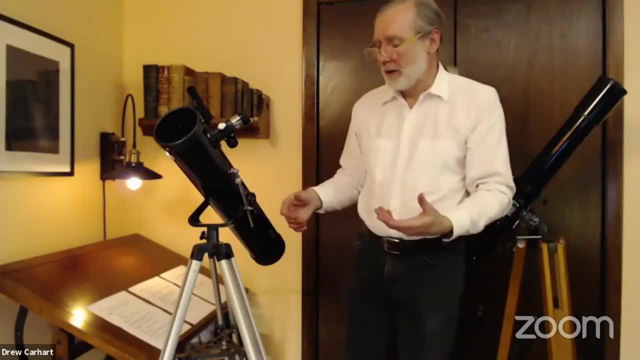 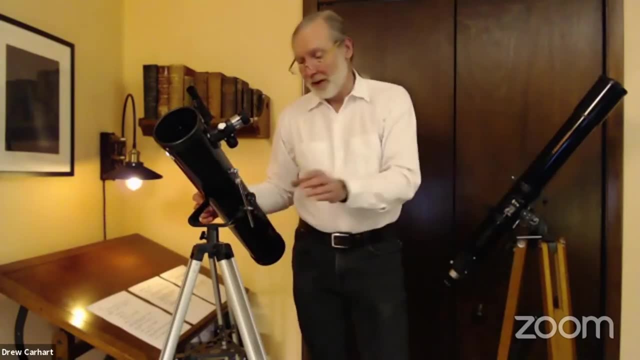 that have been made over the years and are still being made now, And they're all designed a little bit differently, but quite a few of them have some sort of lock on it or another. The exception now to that would be a lot of the go-to telescopes. 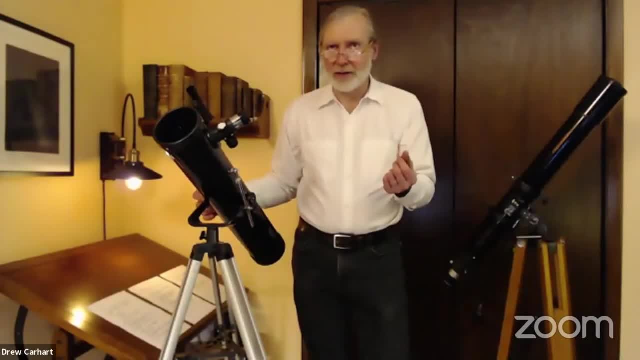 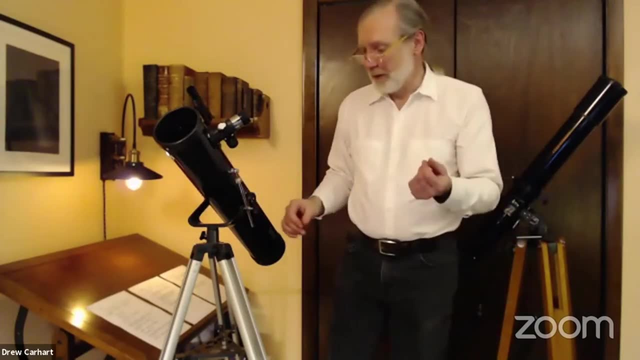 because I remember that when Celestron- no, it was NEAD first- NEAD came out with a go-to telescope well before Celestron did, but they left their mount kind of the same and they left the locks on for the Xs. 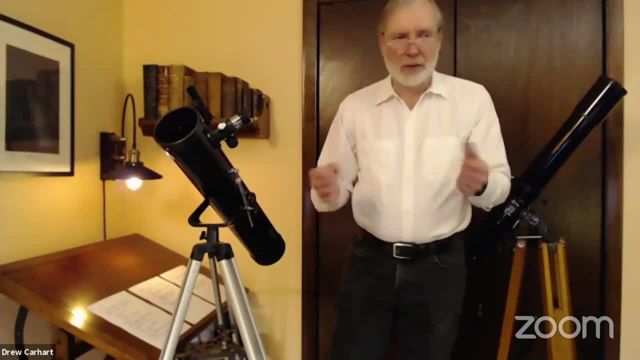 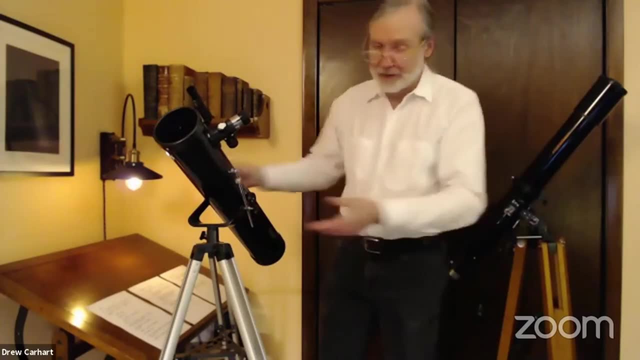 so that people make it, so they wouldn't turn. But but then people were destroying their motors because they were trying to go to and it would get locked or something. So a lot of cases they're designed now without locks on them. But if your telescope 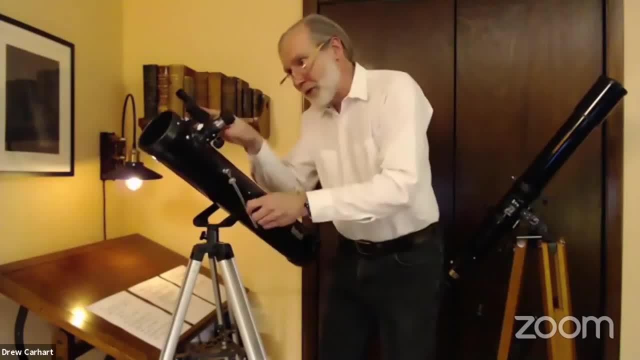 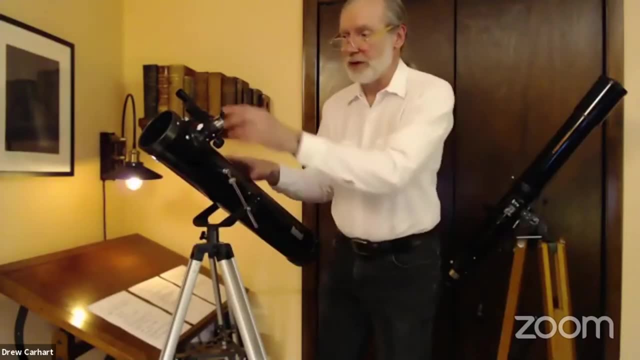 does have locks on them. the thing to do is to get Jupiter centered in here and lock the mounting. So you know, turn this knob and that knob so it doesn't turn easily when you go to change your IPs. That's the best you can do there. 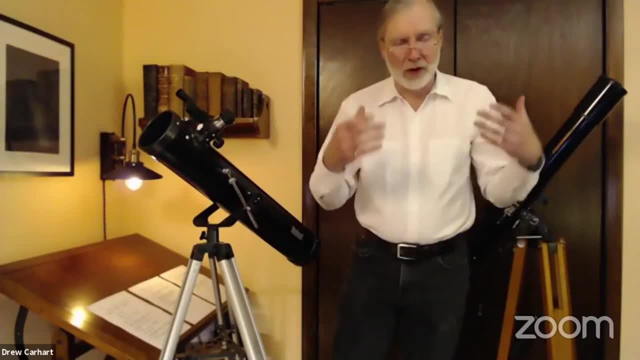 A lot of the the go-to telescopes should either be always locked on their gears, so you can't push them manually, or they should be on a clutch that should be adjusted to be fairly firm. So it's a matter of practicing If you're. 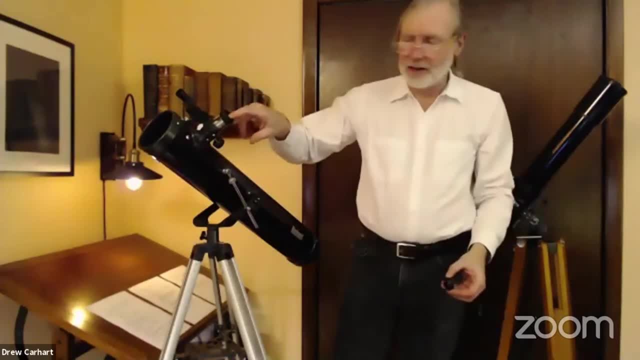 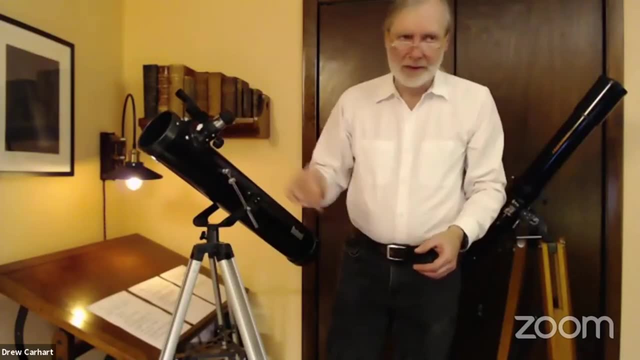 you perennially have problems with it being hard to get IPs in and out of your finder. I would look at the finder and see if there's some way that it could be slightly modified. This finder has a plastic ring at the top of it. 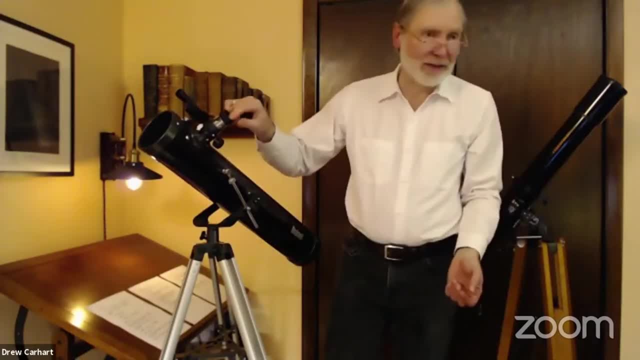 It's a cheap telescope so it's plastic at the top. You could sand the inside of that out if there was an issue. Make sure if you have a locking screw that it's backing all the way out before you go to pull the IPs in and out. 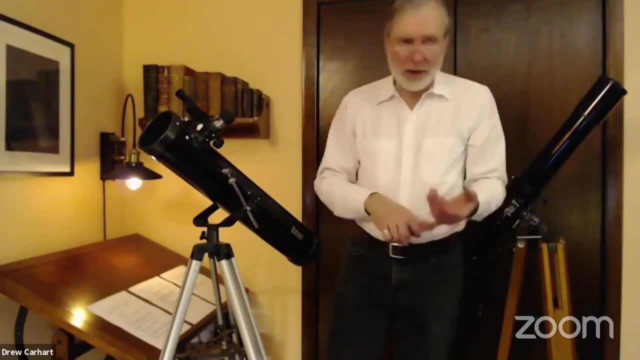 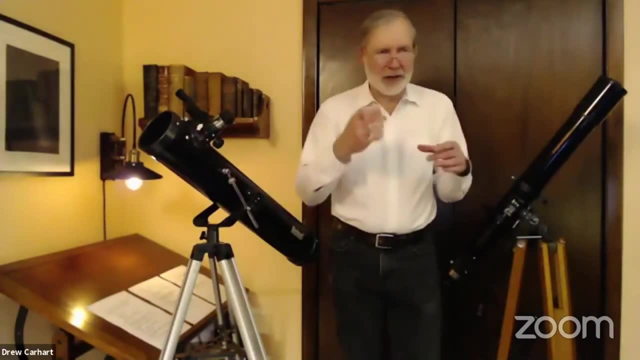 But again, it's a matter of practice Focusing. the default would be, say, every time you change IPs, the new one is going to need to be refocused from the old If you get two IPs that focus at the exact same place. 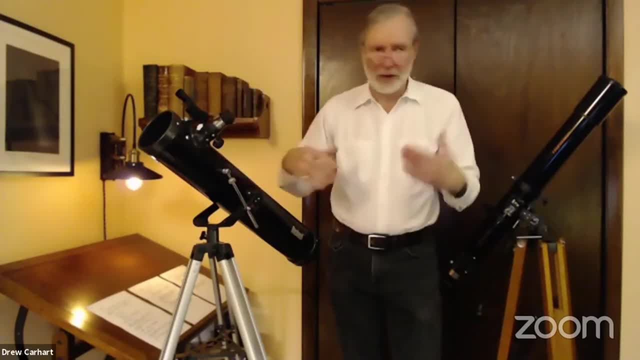 when you're setting into the IPs holder. that's called parfocal. Some sets of IPs by a certain manufacturer sometimes will be made to be parfocal, so you can take out the 20-millimeter IPs and put in the 10-millimeter IPs. 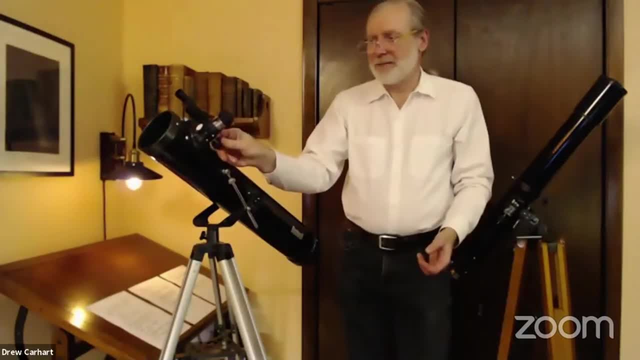 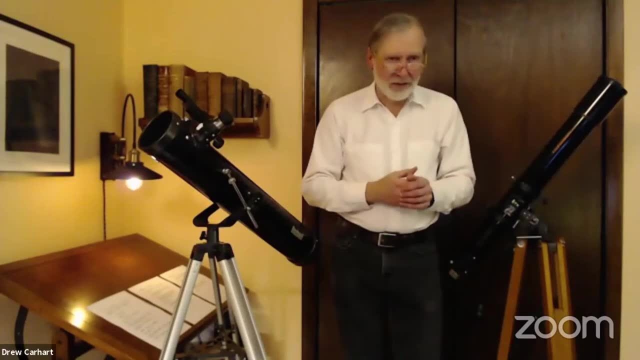 and not have to refocus the telescope. But focusing should get to be such second nature for us that it really isn't that hard to do because, as Jim pointed out, in focusing my eye will focus different than the person standing behind me will- at least a little bit probably. 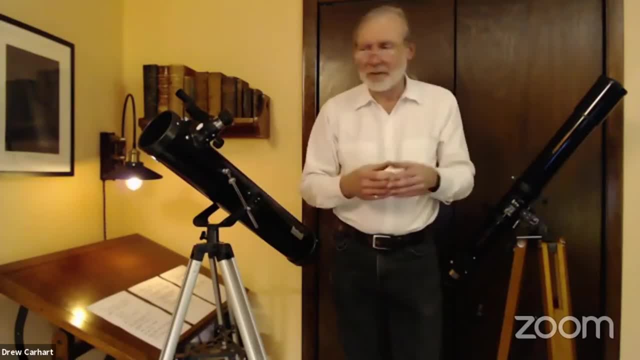 So we're always looking for the telescope and taking focus a little bit, So that shouldn't be a limiting factor, But expect that when you change IPs- But again, for it to not wiggle when you're changing it- lock the telescope as much as you can in place. 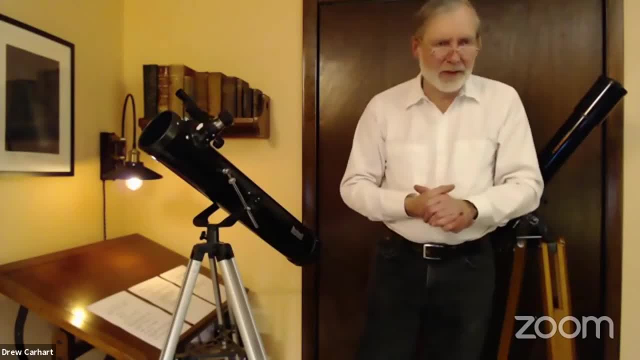 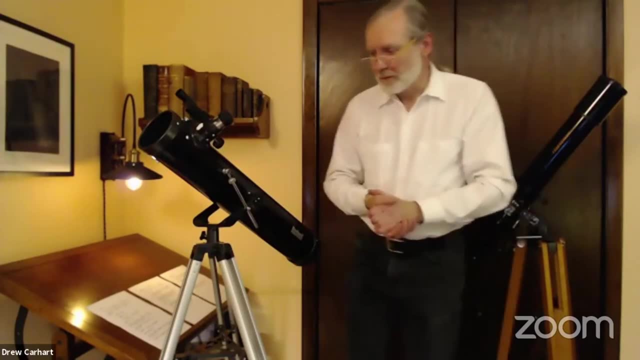 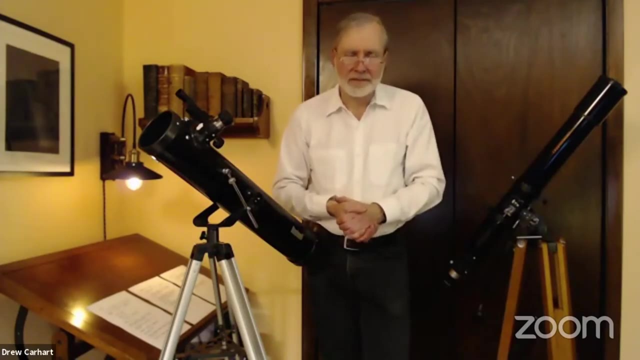 is the number one pointer. Something else I'll chime in and say: sometimes on a manual telescope I'll cheat a little bit. If I see what direction the sky is moving, I'll maybe put that object to the opposite side. So as I move away, 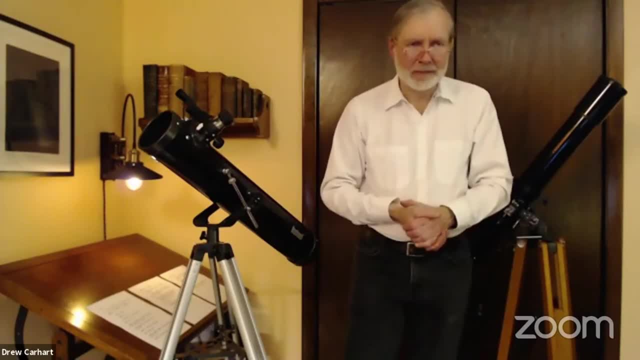 from the telescope to let another person look at it or to change IPs. by the time I'm done, it's maybe drifted into the center where, if it was at the edge when you start adjusting the IPs, then now the object's out of the IPs. 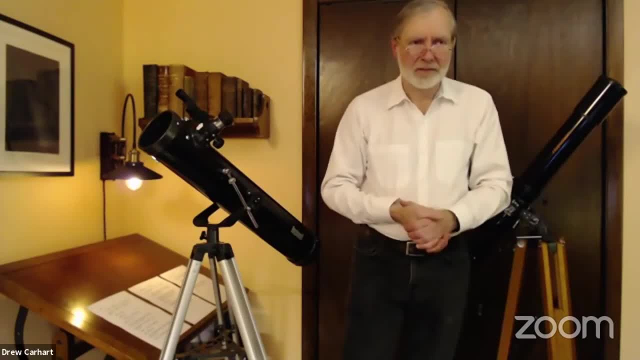 especially when you're going from a low magnification to a high magnification, that object's going to be moving faster through that IP. So if you cheat a little bit, you can maybe swap your IPs in time. And one other thing, and then I promise: 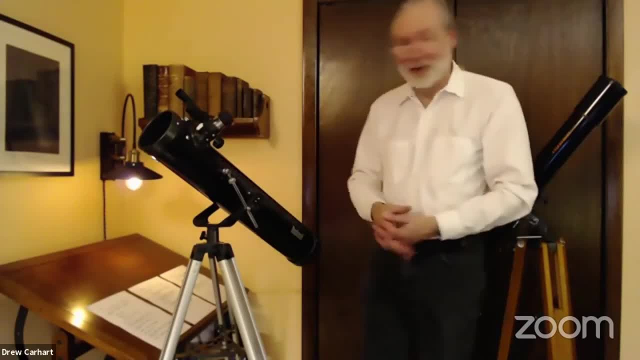 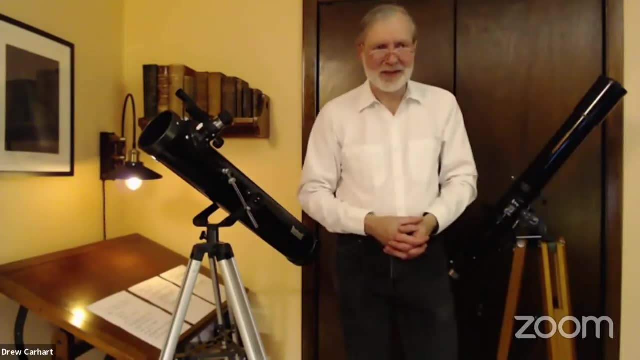 I'm going to let you continue your presentation. Go ahead. We want to say hi to Owen. Owen's five years old and it sounds like he got a a six-inch daub for Christmas. Oh, congratulations, I've met Owen. 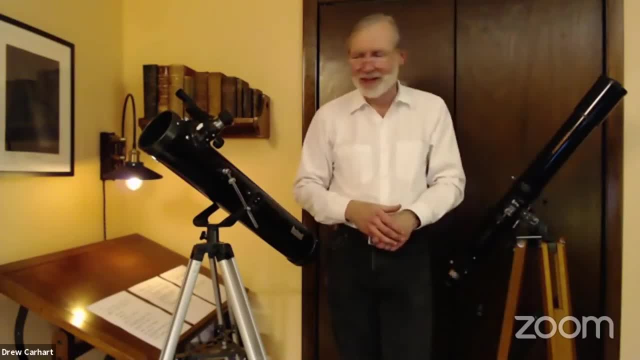 So congratulations, Owen. That's great, That's cool, So that will be a wonderful telescope for the whole rest of your life, So that's a great thing. So well, Okay, You can continue. All right, Where was I? 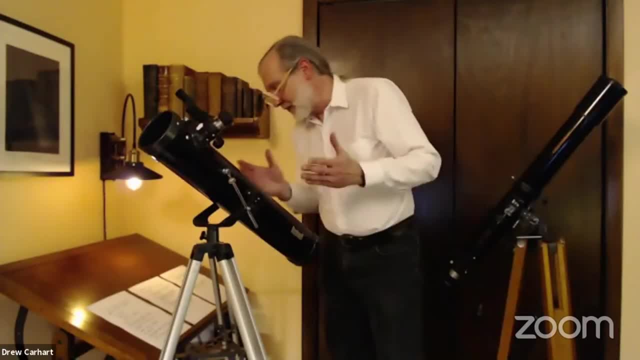 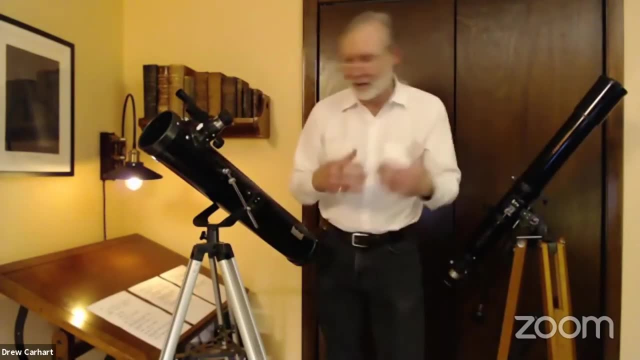 Looking at my notes Over here. Okay, So we're tracking. All I wanted to touch on a little bit briefly was again for the beginner point of view, and I kind of sidetracked it already is choosing what to observe. 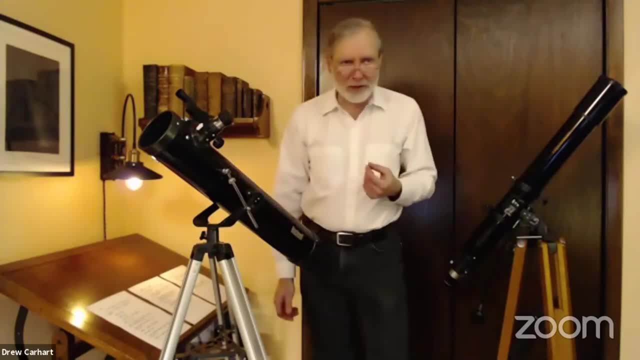 You get a new telescope and you take it outside and the moon is up. and you look at the moon and you say I think that's Jupiter over there. And you look at Jupiter and then you're kind of like, well, now what? 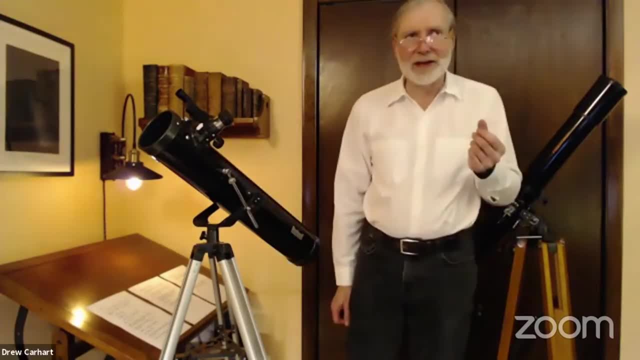 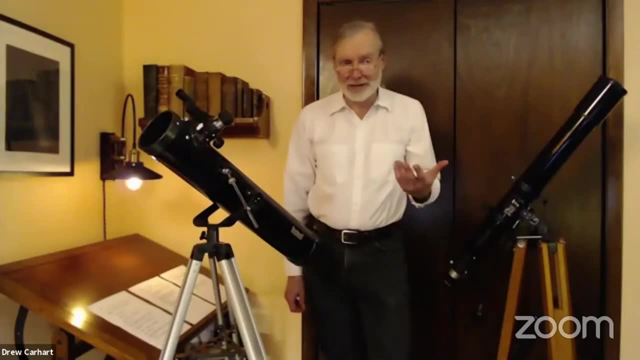 If you have a go-to telescope, it might help you a little bit figuring out what to look at next. But, as Jim already noted, if this was a on a computer, it might help you a little bit figuring out what to look at next. 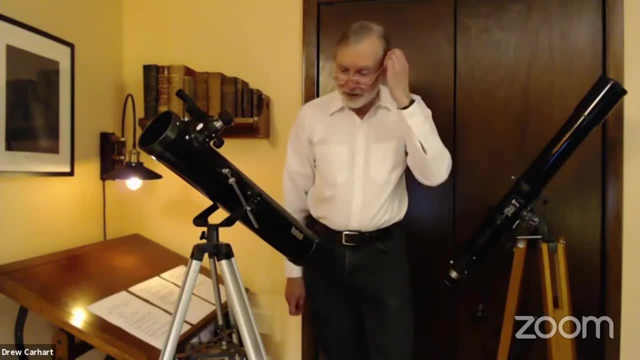 But, as Jim already noted, if this was a on a computer, it might help you a little bit figuring out what to look at next. But, as Jim already noted, if this was a on a go-to mount, this three-inch telescope. 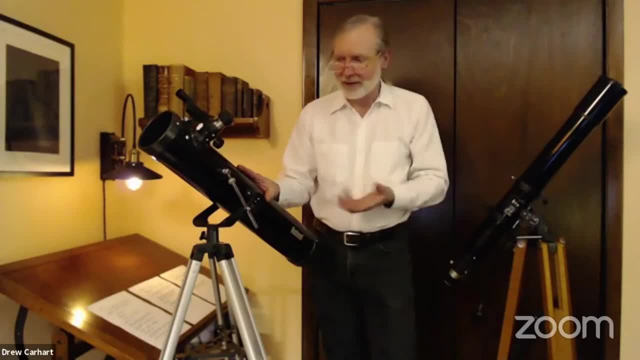 was on a go-to mount, it would have the same, exact same control that this company's 16-inch telescope would have on it. So the go-to catalog would be all three, 2,000 objects or something, 20,000 of which. 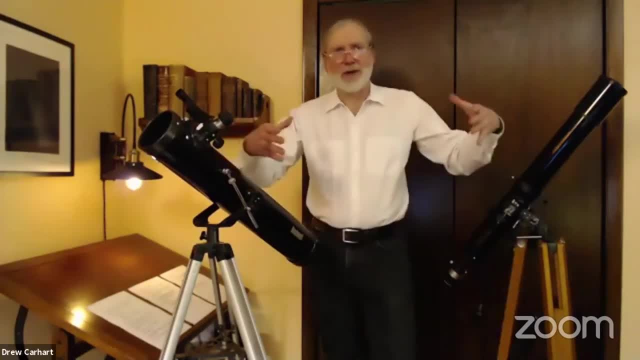 you can't see through this telescope, which you need, you know, a 12-inch or a 14- or 16-inch telescope on a mountaintop in the desert to see, you know, visually through the telescope. So you still need. 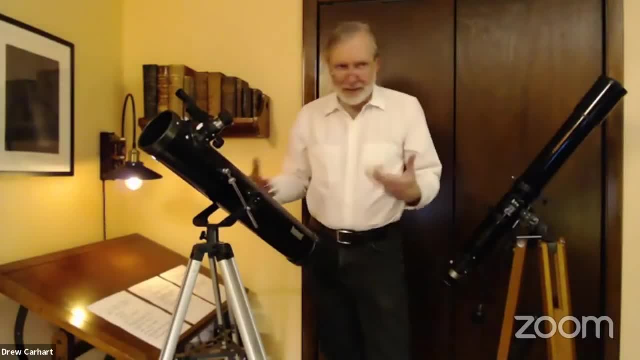 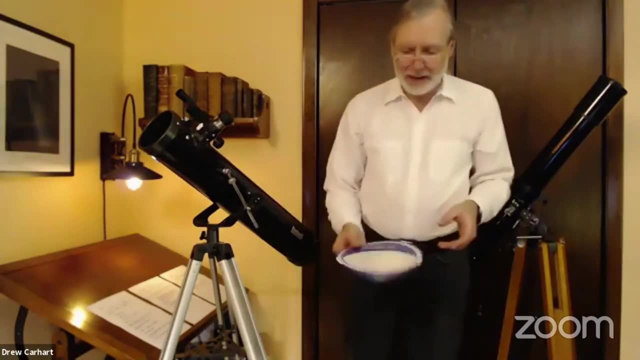 some kind of um guidance about what to look for in your telescope. Even if you have a go-to telescope, you need to learn your way around the sky some, And there's no better way than starting out than with a planisphere. 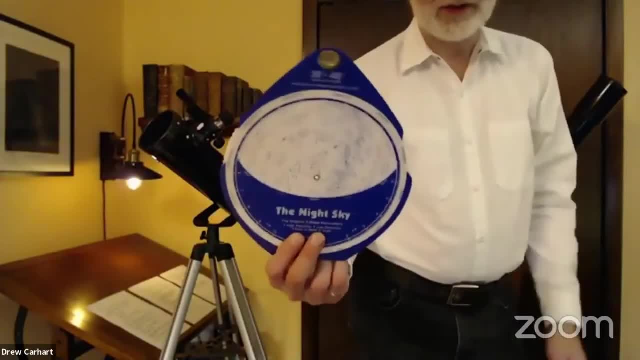 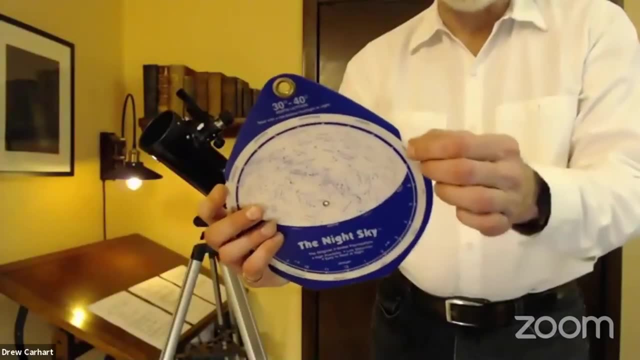 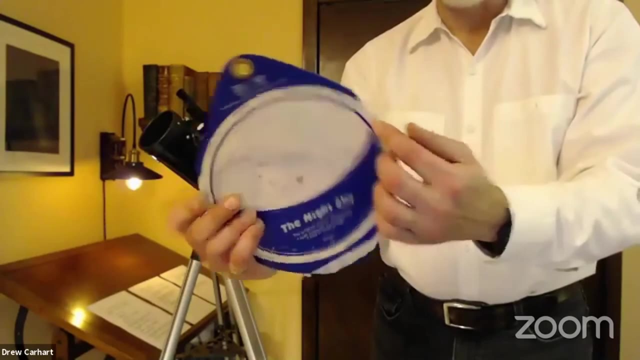 So this is a really inexpensive little accessory for observing. It's a wheel inside a holder and it's got the the days of the year on one scale and the hours of the night on the other scale, So you can use this date with the hour. 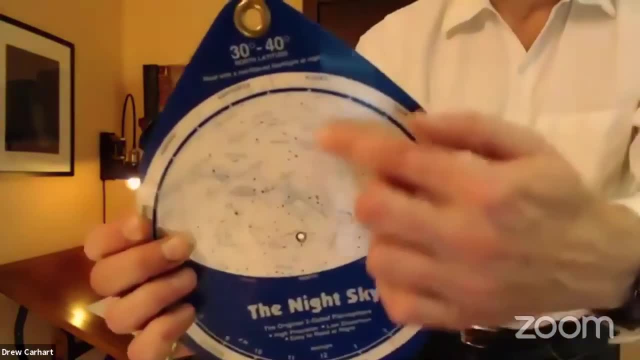 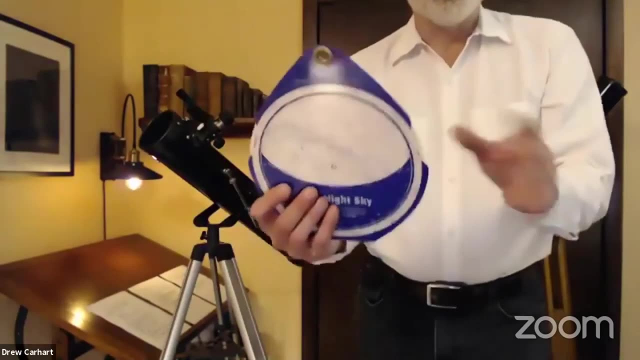 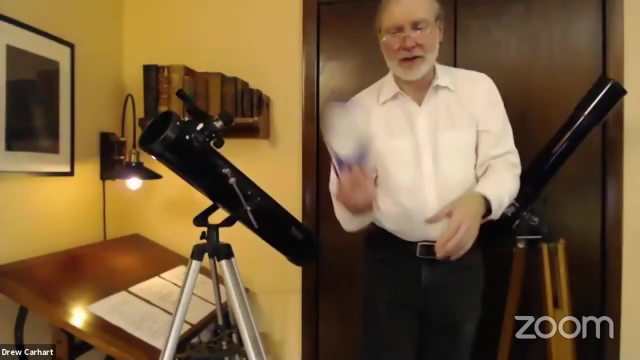 you're observing and it shows you what the sky is and it shows you the bright stars and the basic constellations And you can take this outside, wherever you are- in your suburban yard or in a really dark place- and figure out what those stars are that I'm seeing. 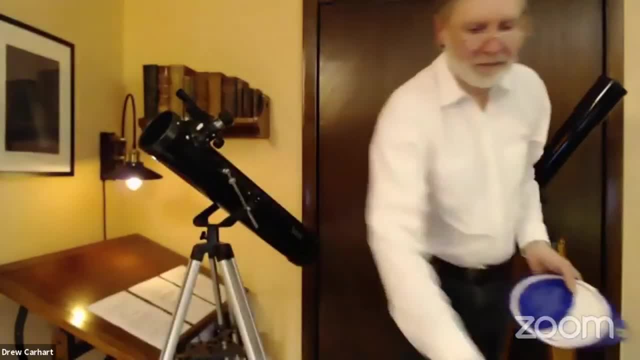 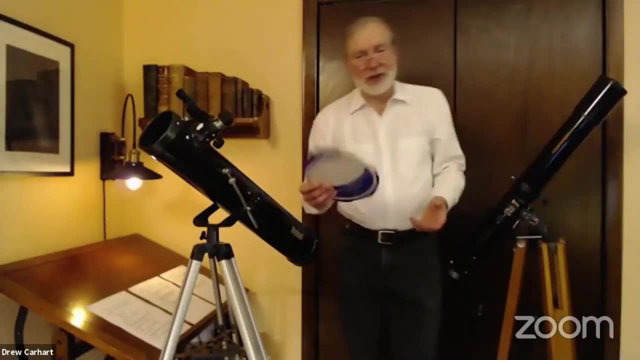 up over in the sky there. So the planisphere is a great thing. You can use your phone app- Hang on, It's going right now- but to show you the sky. I still think this is better. I think the phone apps. 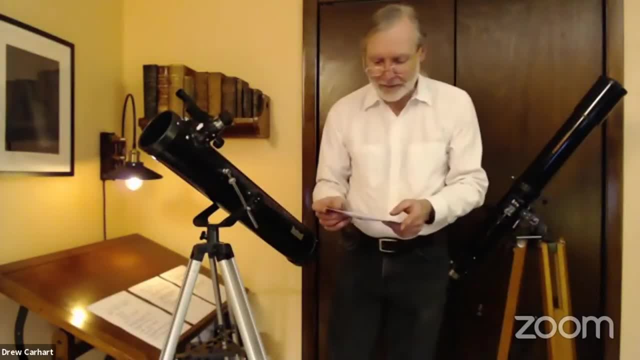 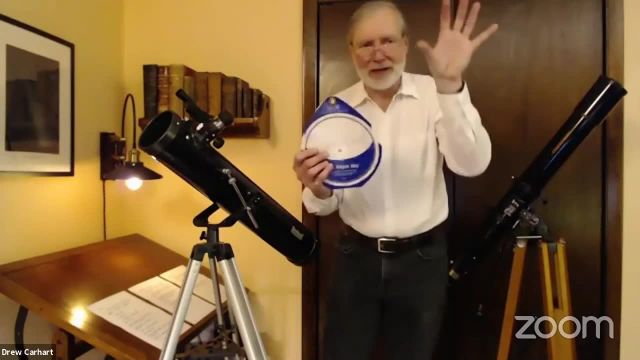 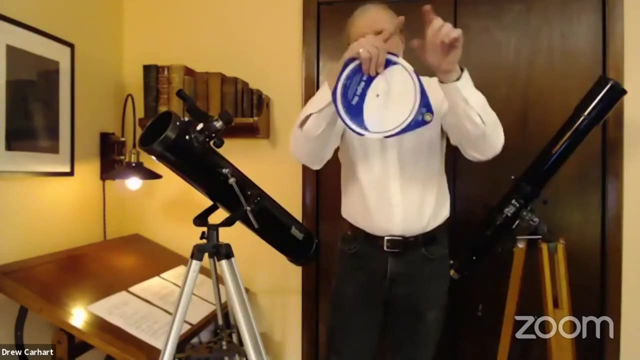 are kind of clumsy. I know that sounds very Luddite to say that, but they don't. this doesn't have problems with trying to decide where you're looking and shifting back and forth on you and not showing you what the proper scale is, because you can. 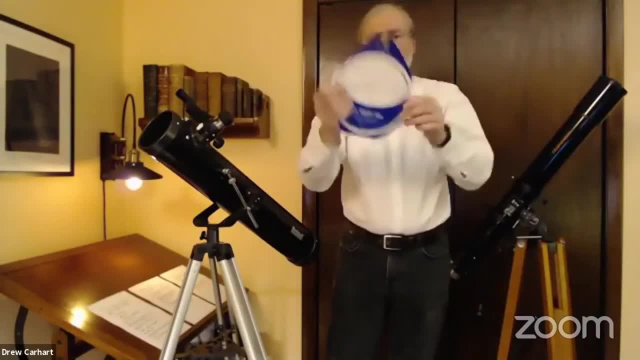 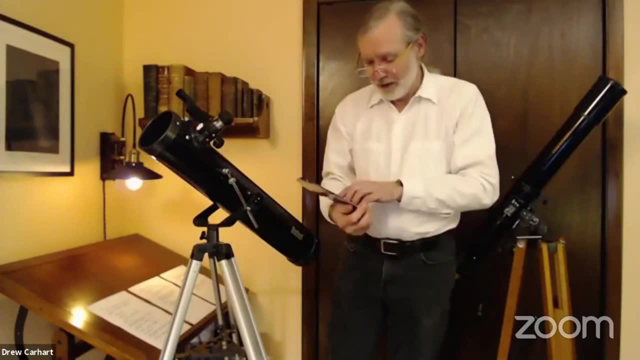 zoom in on the phone app or zoom out and it's like, well, this is always just kind of fixed there. It's a handy. you can study this during the daytime, set it for tonight and look at it and say, oh. 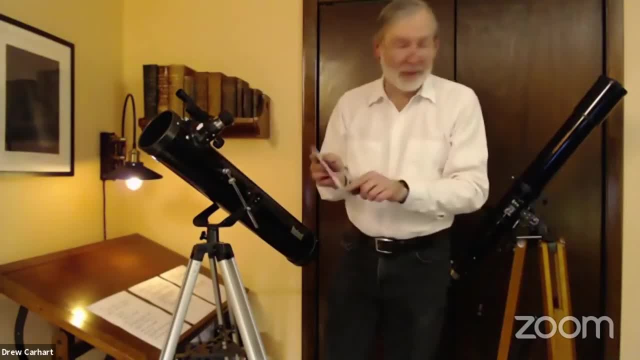 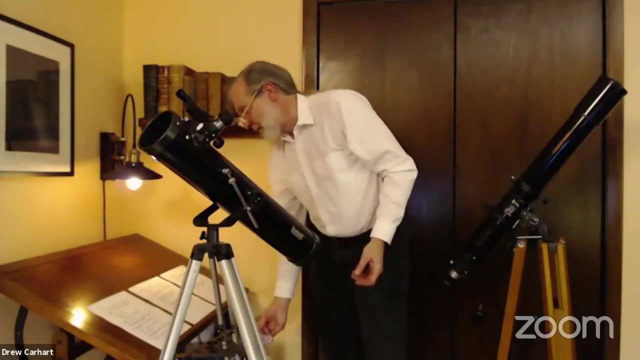 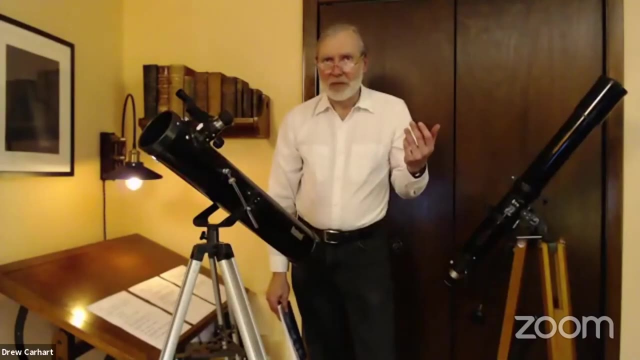 well, that'll be Vega setting over in the west, as I you know, as I go out tonight, so I'll look for that and great resource. Then you need to learn what to expect to see in your telescope again, And some of that. 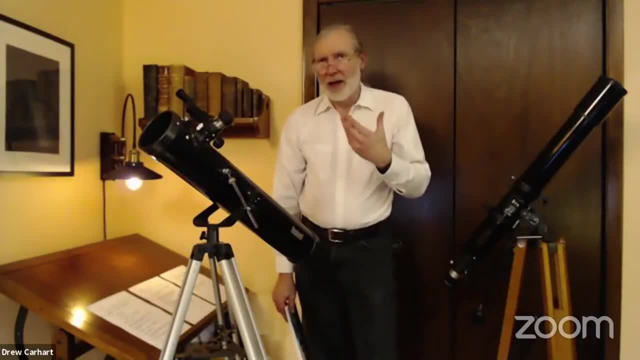 will come by practice. Say well, I saw in this list that there is a sixth magnitude or say a 10th magnitude galaxy and I looked there and I looked for it all night and I didn't see it. So I kind of wonder. 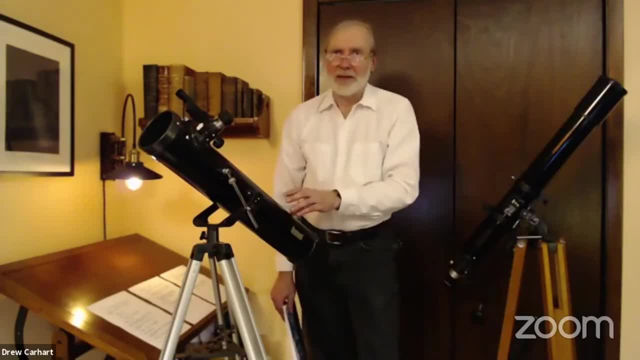 whether I can see 10th magnitude galaxies in this telescope. or it might be an eighth magnitude galaxy and you say, oh, I got it, So I know I can see that in this telescope. So learning that is important and that's going to depend on. 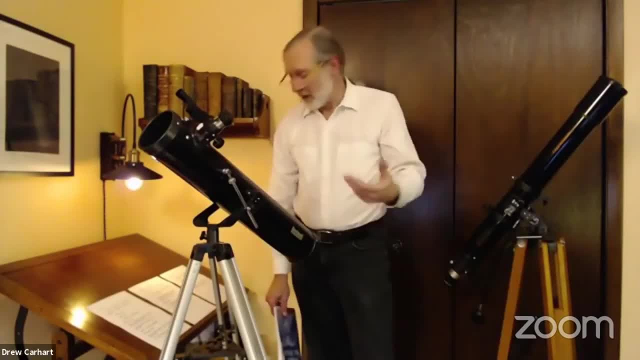 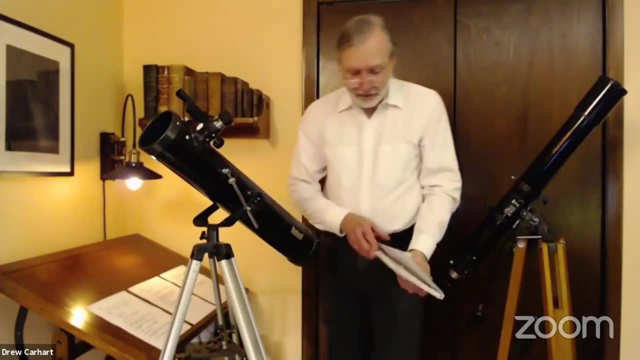 what your telescope is, how good your eye is, what your observing conditions are like, what you're looking at. But then you need to know your way around the sky. There's sky charts of all sorts. if you're a manual user, that just are maps. 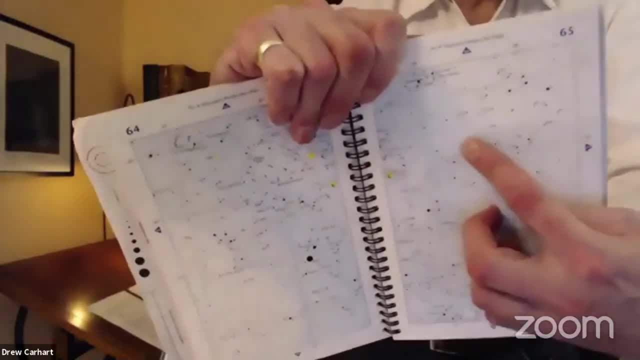 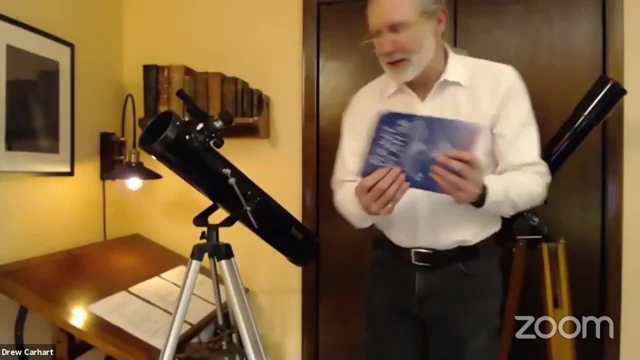 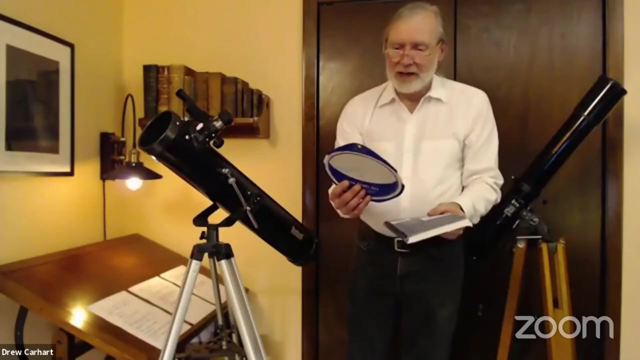 of the sky that show you the stars and then show you where various objects are that you might want to look at with your telescope. It's kind of an essential thing. The planisphere is going to show you where the constellations are. Some of them: 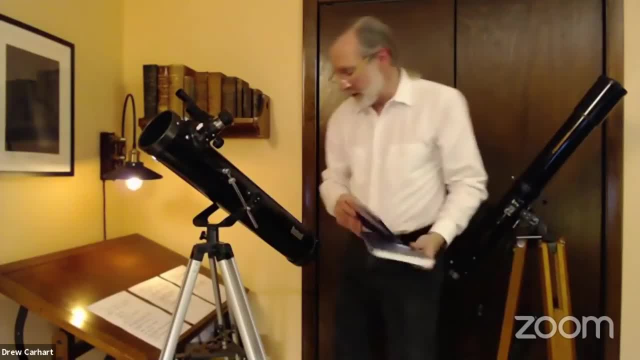 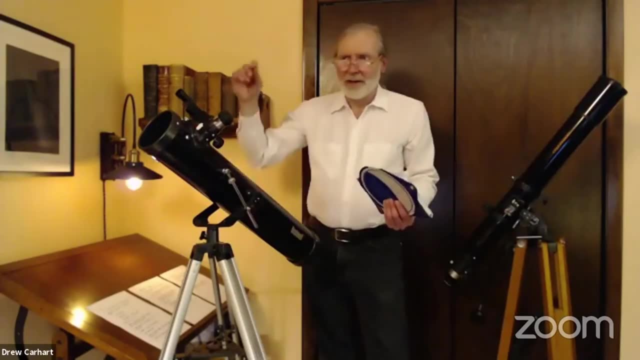 have actually the navigational stars listed on them. So Jim mentioned that when you use your- so you set up your go-to telescope- you might end up having to look at the star Mirafak or something or other, because it says: I'm looking at Mirafak. 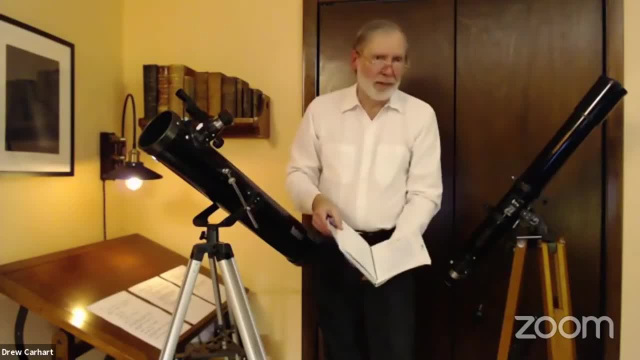 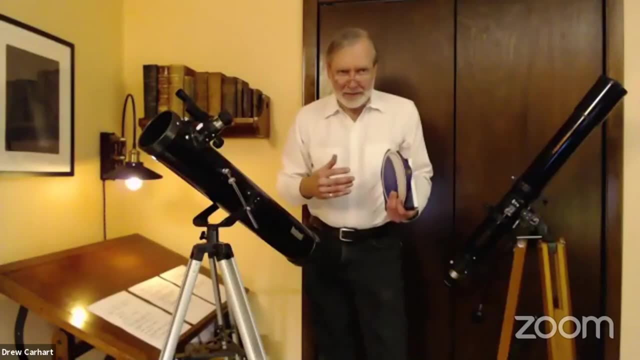 and you're like: well, what's the star Mirafak? But a chart would maybe tell you that. Maybe your phone app will tell you that, or your planetarium software on your computer would tell you things like that around the sky more. 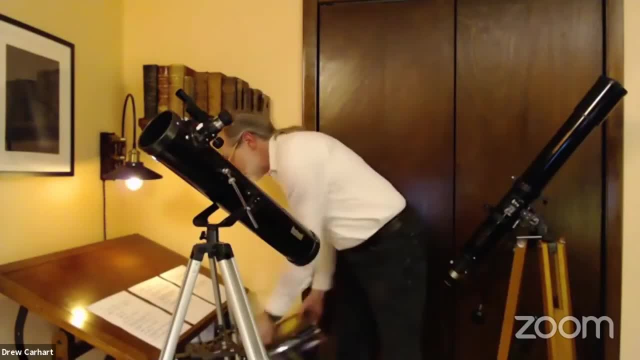 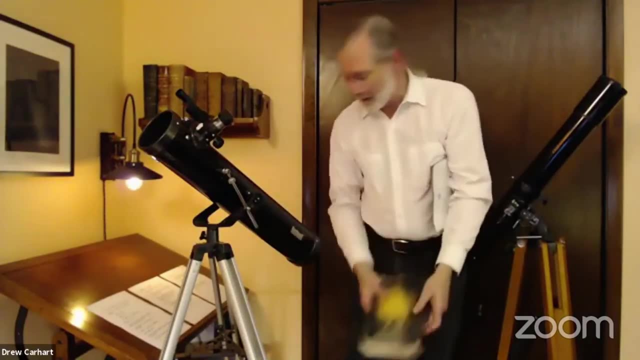 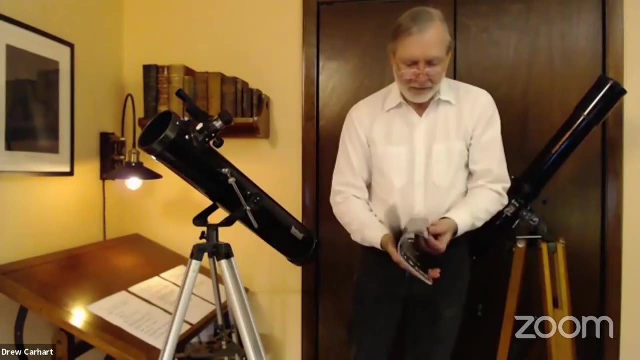 And then there are all sorts of lists of objects. There are whole books on things to observe in the sky. There are articles in magazines like Astronomy or Sky & Telescope every month about this star cluster to look at or this group of galaxies to look at. 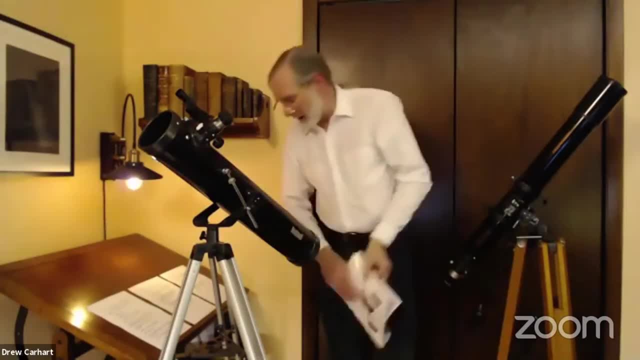 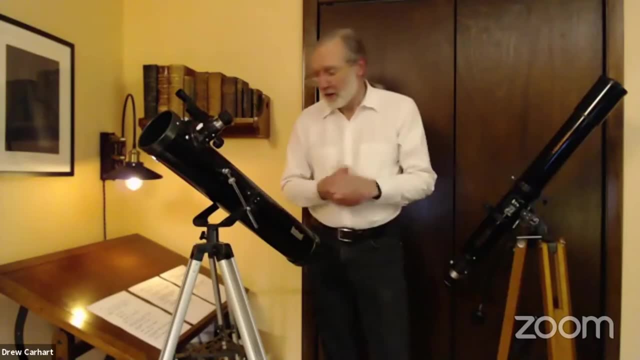 or something like that, And so there are resources like that. The internet, the web, is full of resources on objects to look at and stuff. So you need to know what the capability of your telescope is and know basically how to find things with whatever your telescope. 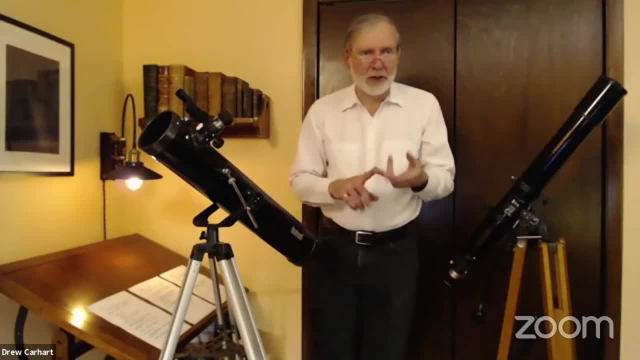 setup is, And then you can start making lists of I'm going to go out tonight and I'm going to find these two or three things that I've never seen before, And you can spend your whole life doing that, because there's thousands of things to look at. 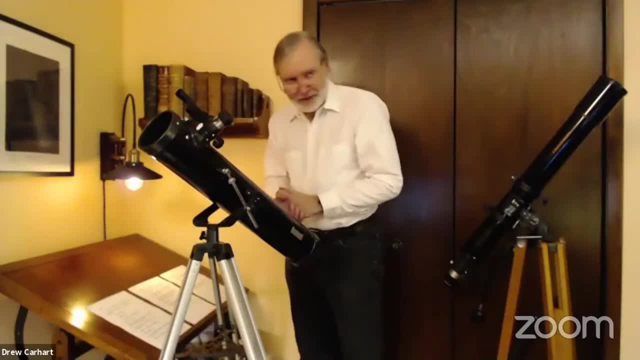 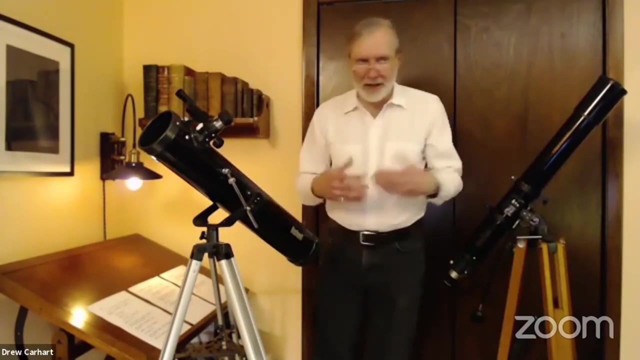 in a telescope. So keep on exploring that way. The last thing I had down was we were asked to give a brief thing about telescope care. we suggested we do. I know that's something that we've done- whole presentations on cleaning and caring for telescopes. 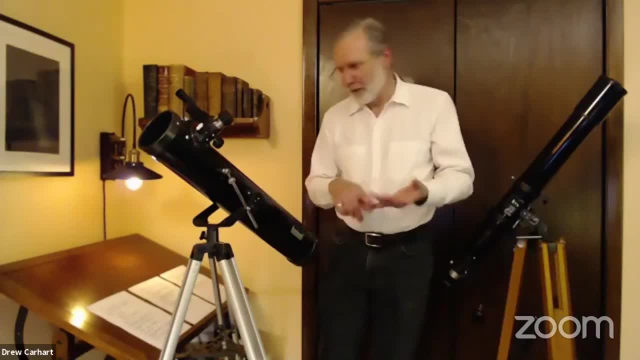 And so there's a lot of details to go into, but I'll hit just a couple of points now. First off, clean and dry Both the optics, especially the optics, but then also the mechanical points parts and certainly the electronic parts if you have a telescope. 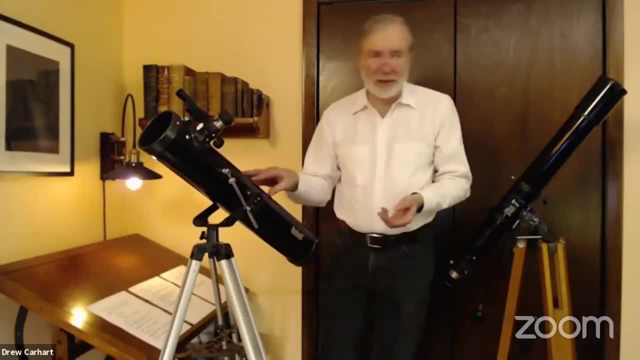 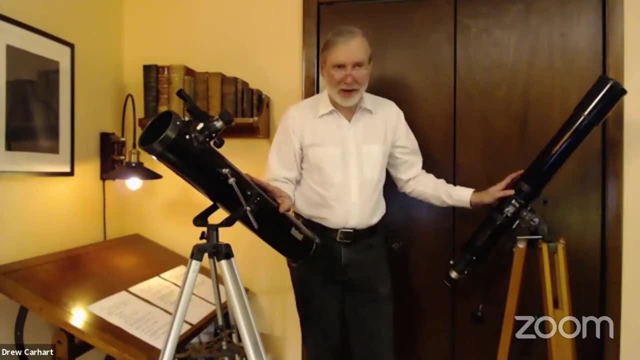 with electronics in it, clean and dry are the key. You're going to use this outside and when you bring these in they might not be clean and dry anymore. They certainly might not be dry In any time of year. we can get dew on telescopes. 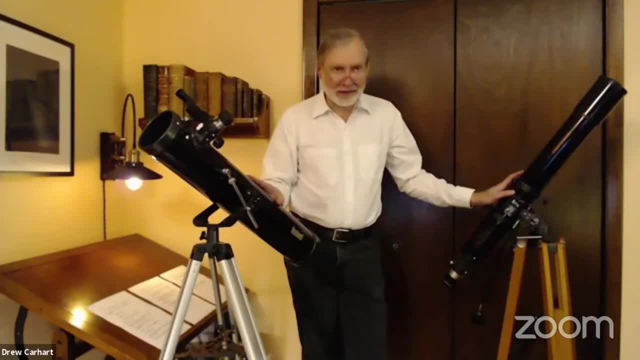 it'll be frost at this time of year. if you're out in January, you can get frost on the telescope. In the summertime it might just be dew. it's condensing through the night as the air temperature drops. You don't want to leave. 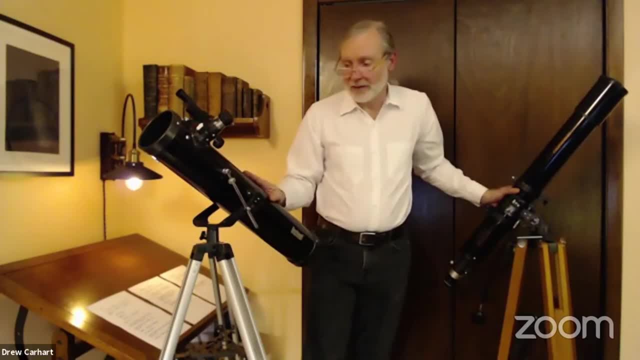 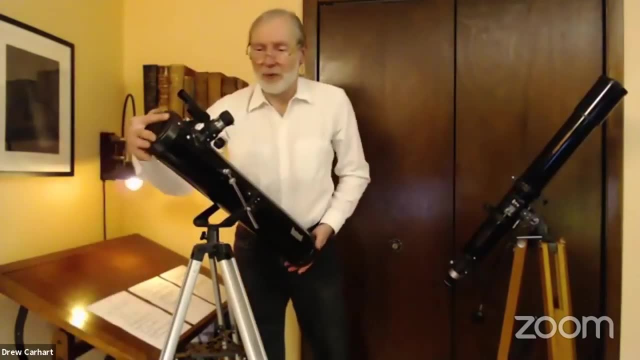 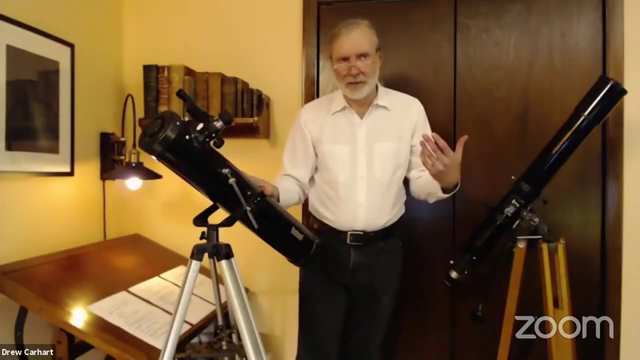 that on the telescopes. So the key for clean and dry? it may seem counterintuitive: put the caps back on, put the eyepieces away, cover the telescope before you bring it back inside and that'll help keep the interior humidity in the warmer area inside. 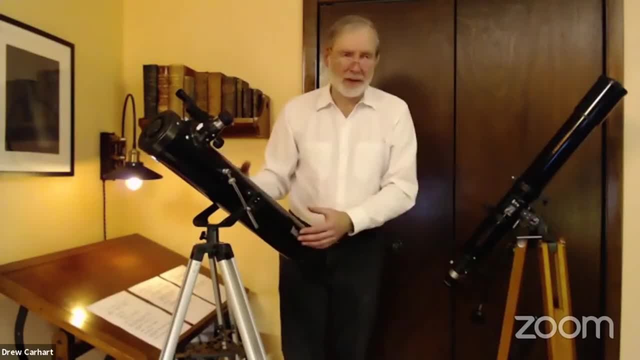 from condensing on the telescope or in the telescope while the telescope warms back up. After it's warmed back up, maybe the next morning when it's in house temperature, take the covers off and make sure any moisture on the inside is gone. Same thing. 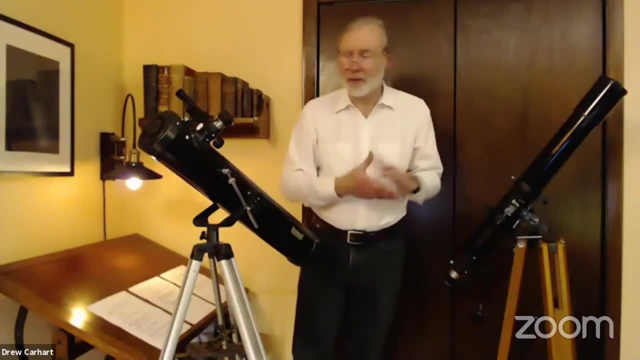 with eyepieces, it's better to put them in a case than any other part of the telescope- The clean part. we try to keep things clean as we use them. We learn to be careful when we're handling our eyepieces to not touch the lenses. 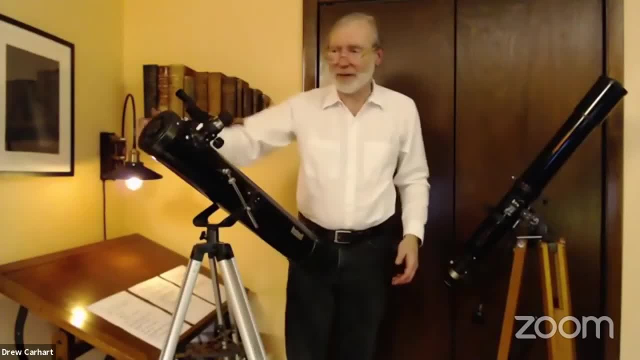 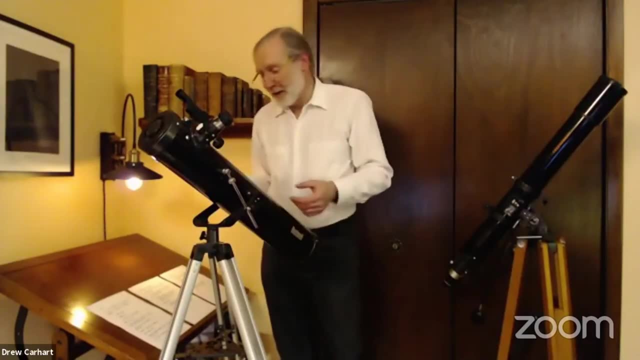 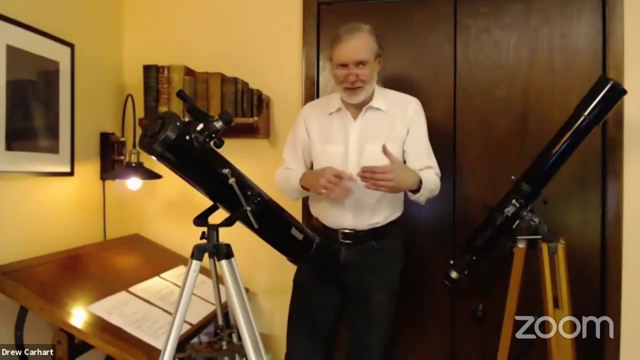 We certainly. if you have a lens in the front of the telescope or a corrector plate in the front of the telescope, you don't touch that really anytime. I'm not a fan of keeping telescopes in garages. You get broad swings of temperature and humidity. 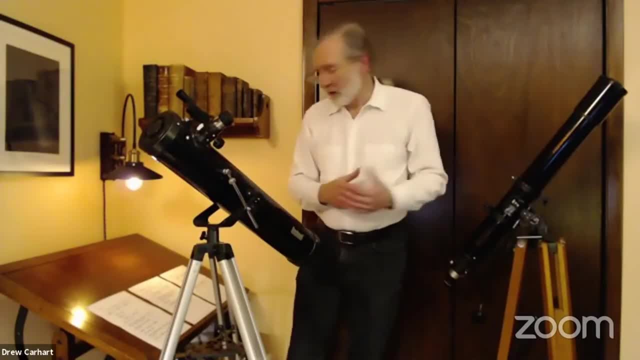 even if your garage is really clean, it's probably not as clean as somewhere in your house would be. So keeping it clean in the first place for again, all those parts for the optics, for the mechanics and for electronics- I'm sure we'll be doing programs again. 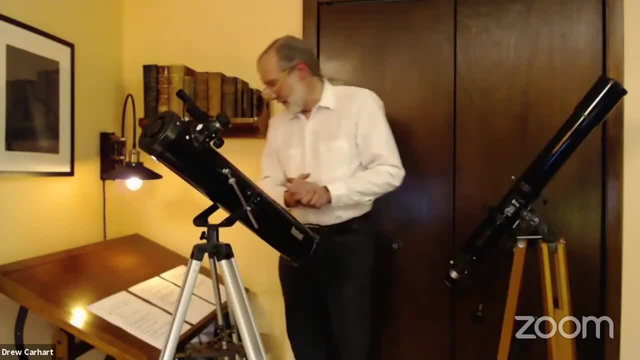 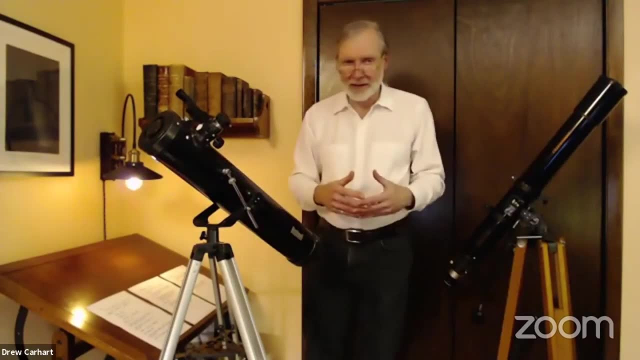 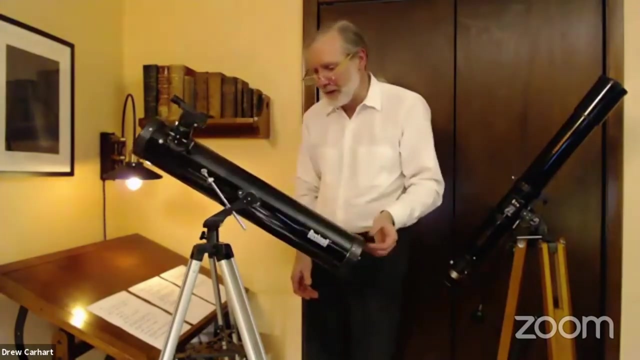 every couple of years we do a program on cleaning optics which can fill an evening, so we'll do that again before long. but there are ways of safely cleaning optics and it's actually better if your lenses- especially they- get dirty. it's better to clean them than to leave. 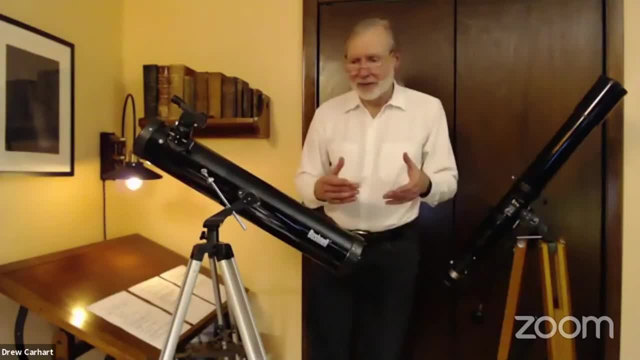 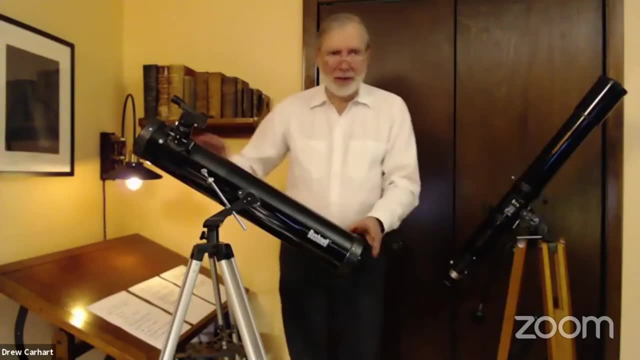 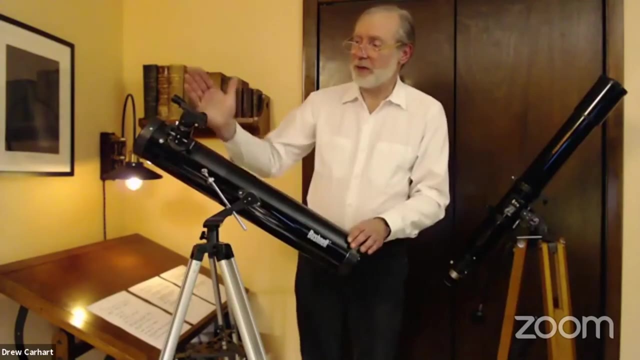 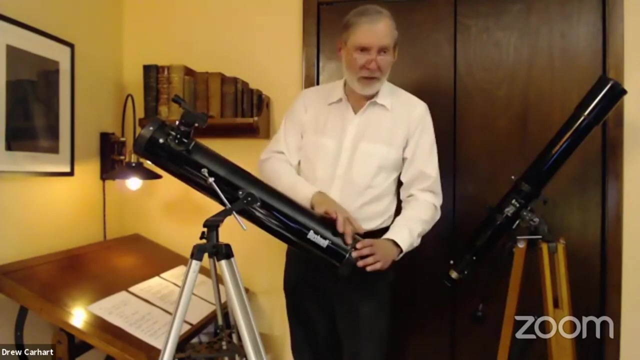 them dirty, and it's a simple, very simple principle that you really should know basically what it means for your telescope. so there are a lot of optical parts in a telescope. this one, for instance, has a mirror down the bottom that's gathering and focusing the light. it has a 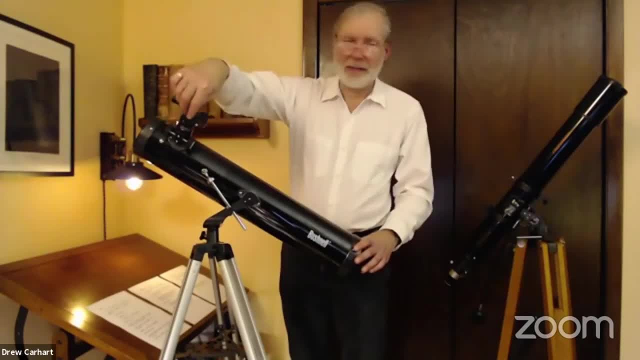 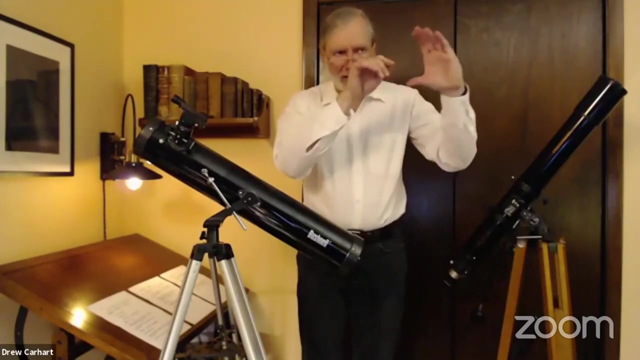 second mirror up at the top, an eyepiece in it. so these are all parts of things in the optical path of the telescope and each one of those things, the mirror here, the mirror up here, this finder or the focus around- excuse me here- and the eyepiece. 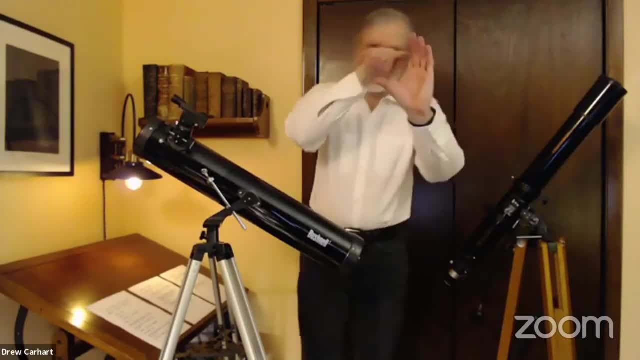 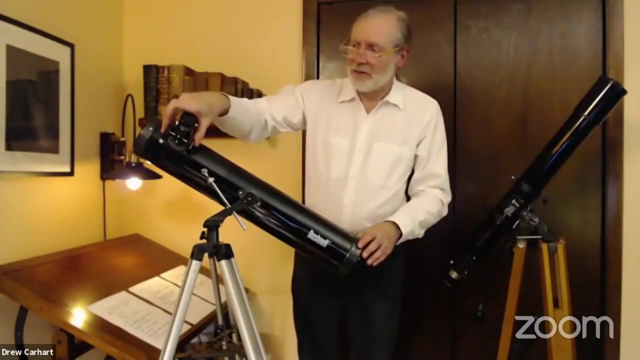 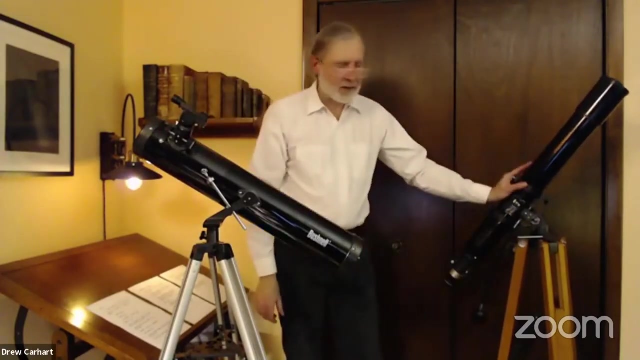 that goes in. it each have kind of a little bit straight at it. collimation means adjusting the angles and positions of all the different components in your telescope. so they're all of those lines are the same line. so the light comes neatly through and hits the sweet. 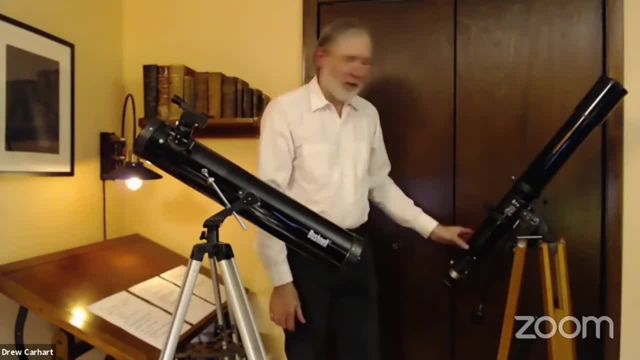 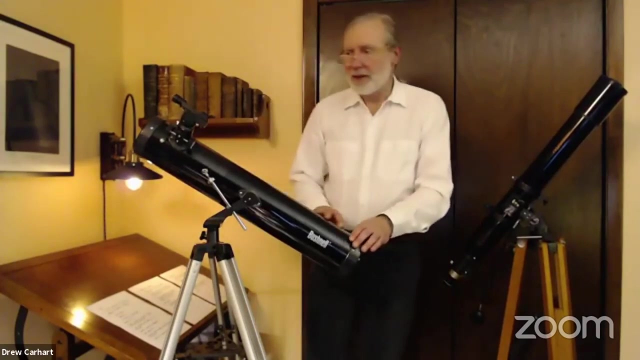 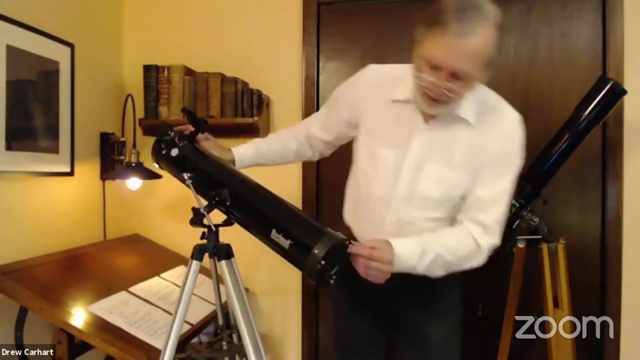 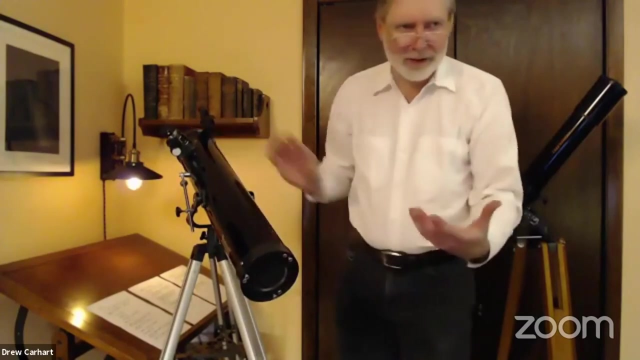 spot of the telescope. everything is anchored in place here well and it doesn't get out of adjustment and you can have a telescope. I just looked through telescopes this sort of design that were 100 years old. they were still in perfectly good alignment, ones optical adjustments. 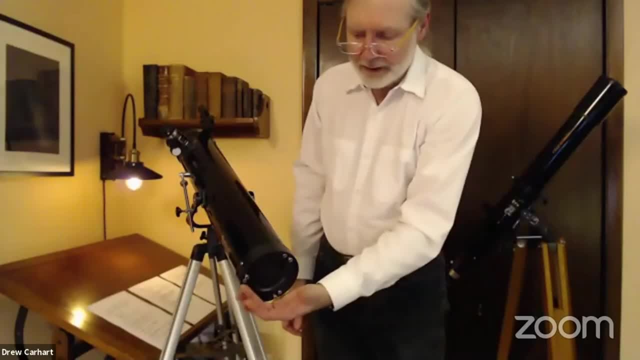 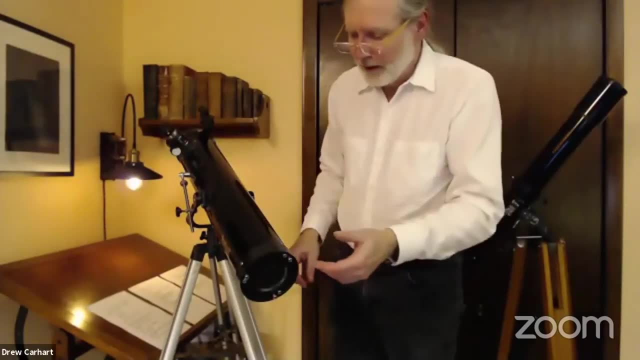 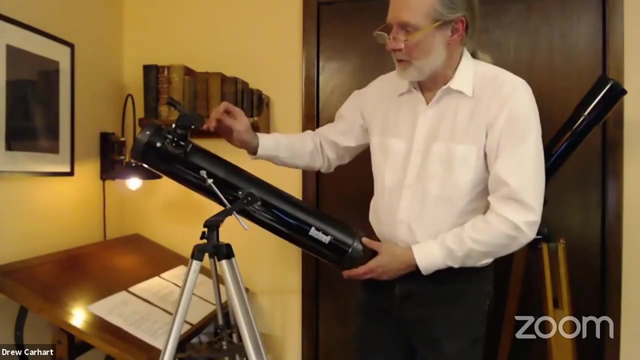 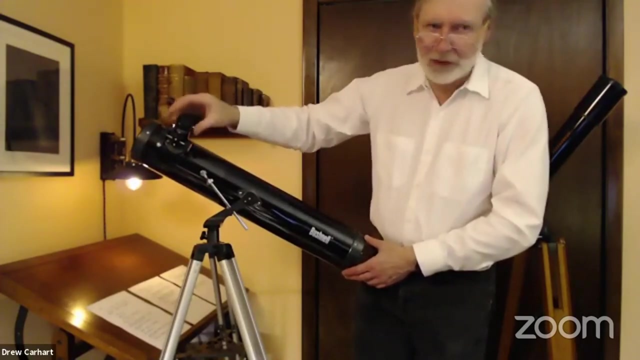 come in a triangle, they come in threes, so you can tilt something by moving one of the corners of the triangle in and out, or two of the corners in and out. so collimating means lining up this mirror to that mirror, potentially the second mirror to the. 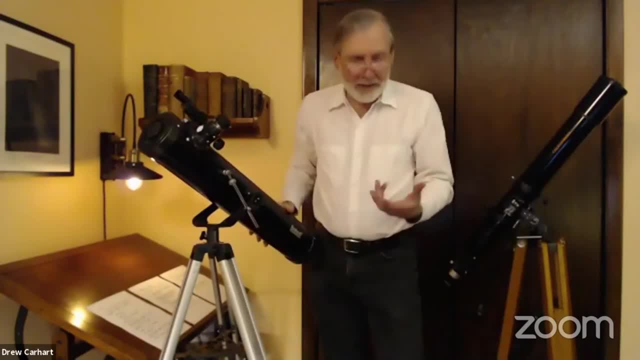 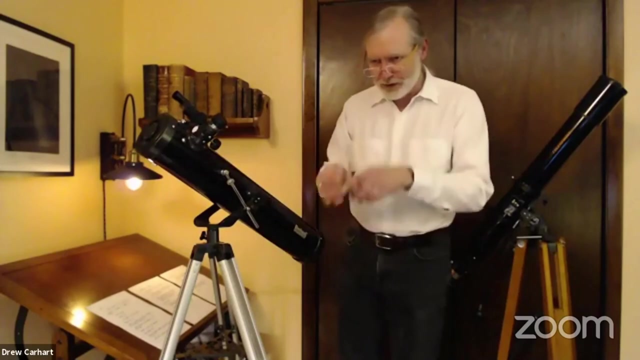 eyepiece. so it really depends on your telescope what the need for checking collimation is. again, if it's a well-made refractor, it's probably something you'll never gonna have to worry about. if it's a reflecting telescope like this, that's like one that's 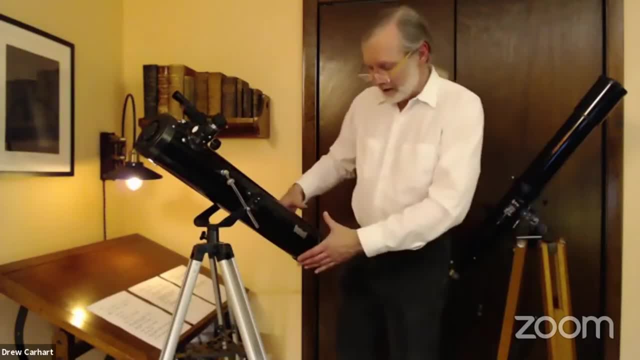 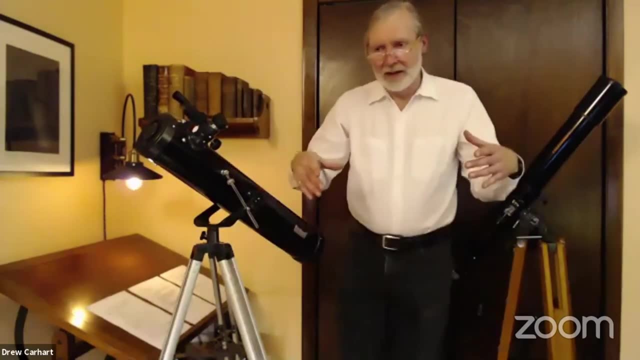 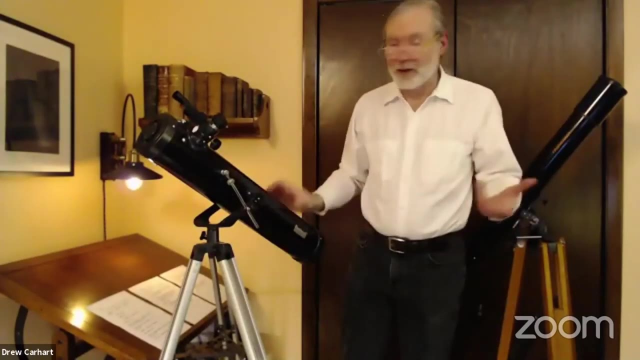 sitting over the corner over here that the base is reassembled to the uprights on it that hold the top of it on it where they have the second mirror in it. I have to check the collimation to make sure it's all in good alignment. 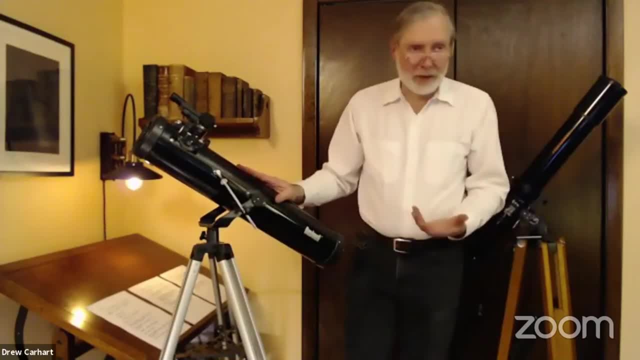 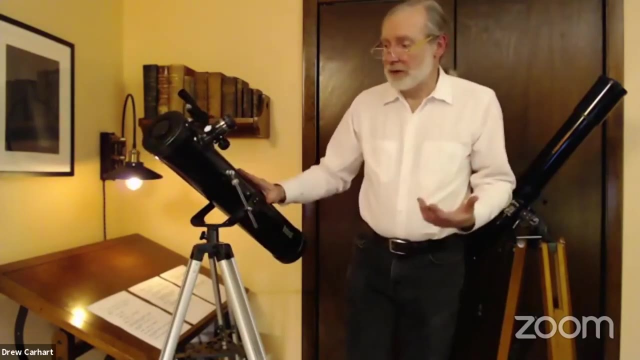 it's actually a well-made thing and I can reassemble it all from its many parts, and oftentimes it's still smack bouncing around or whatever, so depends on your telescope. if you have a reflecting, especially Newtonian reflector, you should get used to finding out. 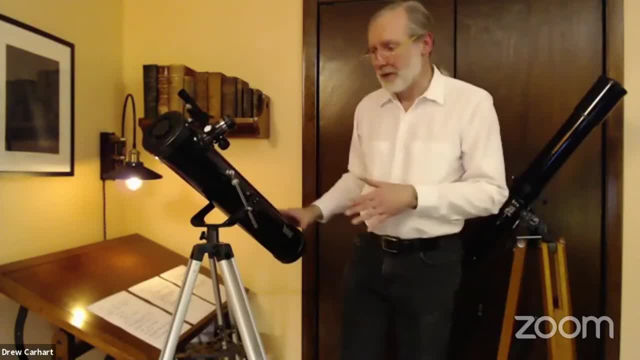 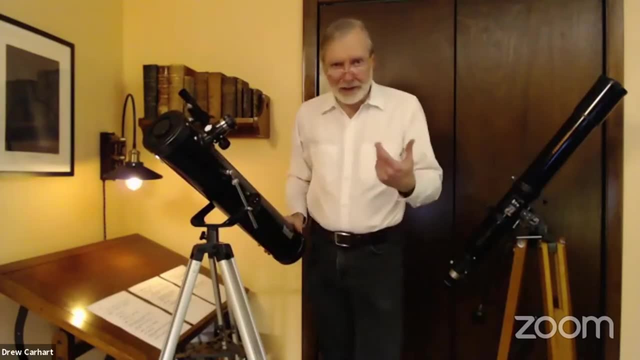 and learn how to do it and get used to checking the collimation to see how, whether it's good or not, and whether it needs adjustment again. you may hardly ever have to do it, but you need to do it, and so that's really the most important. 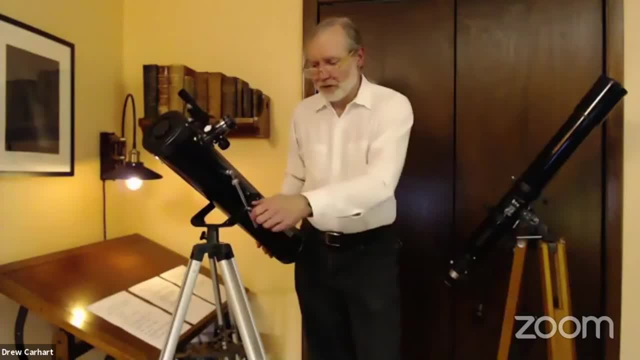 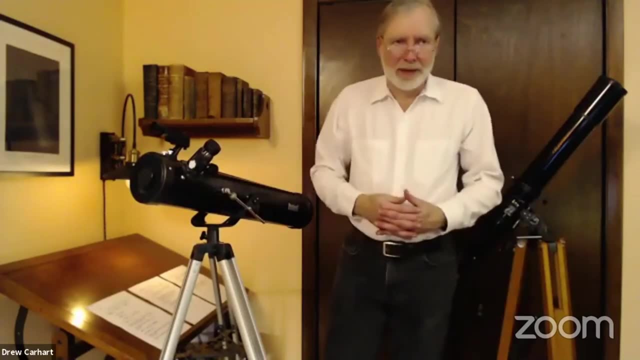 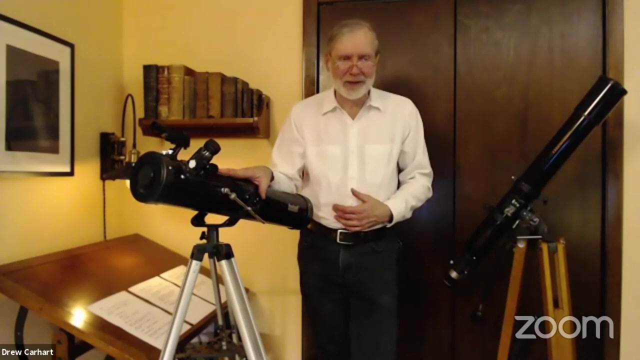 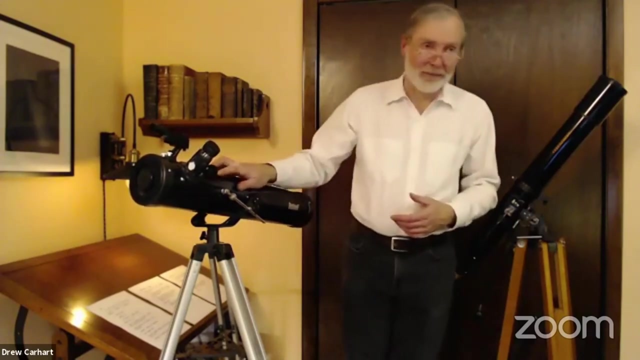 thing that I think is really important to you all in your telescope, and it's really important to look at what you that they shouldn't have turned, or not understanding what exactly they're trying to do. so again, that's almost a different, but it is another whole program on really how to address. 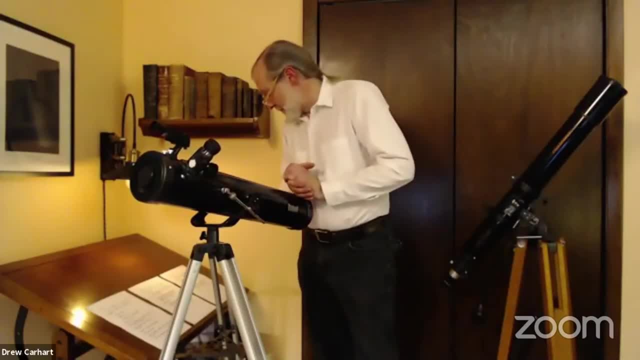 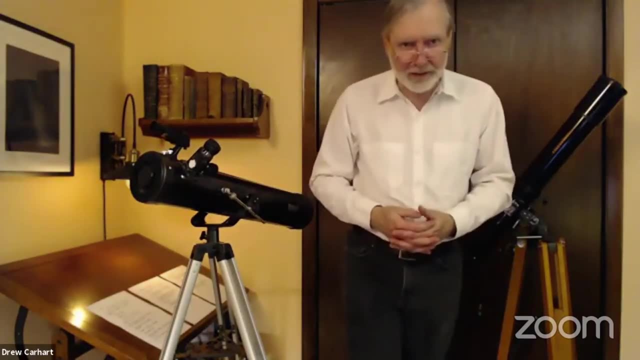 that effectively. um, that's the things on my notes down here that we're in my turn to cover. so, uh, is there anything else, jim, that we're. well, i'll just comment on on collimating, uh, on a smit casagrain, unless you have an obvious issue that you can see that a star is totally. 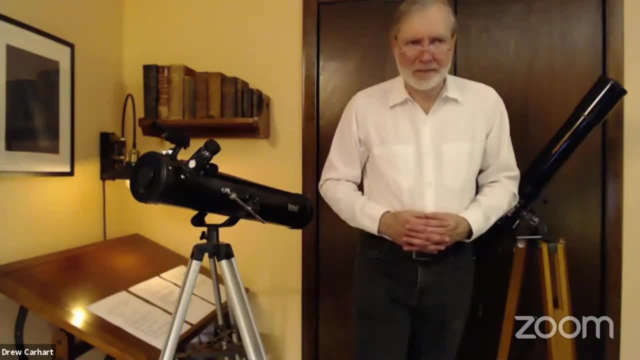 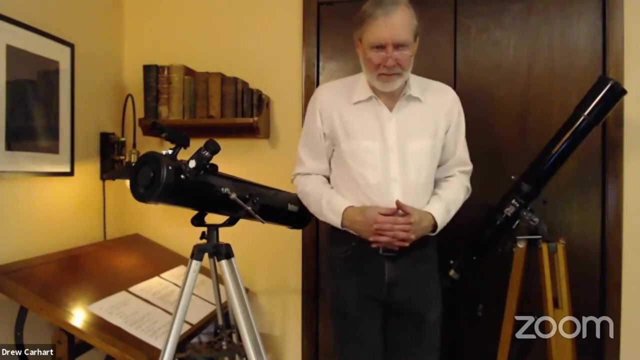 not aligned. i would say: try not to touch it, because it probably shows up manufactured in a way that that it's good enough. um, if you accidentally dropped it a little and something shifted and and then it's not working right, then then i would say, yeah, collimate it. but 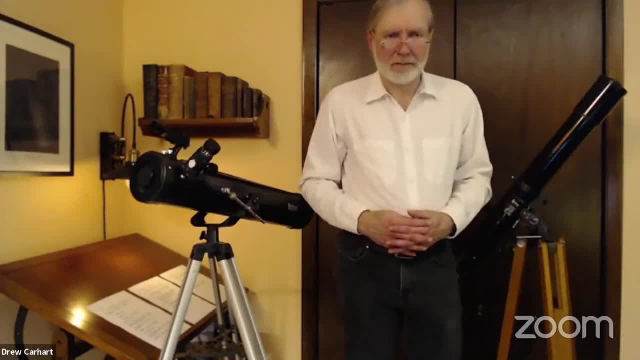 if you, if you were focusing one night and you go boy, that star is just not as sharp as i think it should be. i don't think collimating's it's gonna. it's gonna cause you more frustration than, uh, than the improving your, your views, probably for the most part. 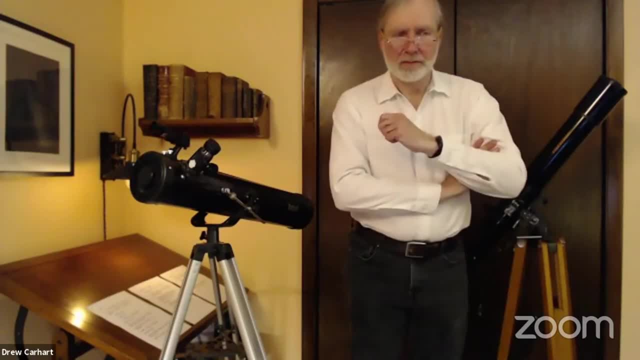 and then also i'd say that i think probably the smaller the the reflector, probably the less collimating you need to do so. a six inch, you probably collimate it one time and maybe never really touch it again. if you have a 12 inch, um, you know that bigger mirror, just gravity alone is making that shift a little more, as 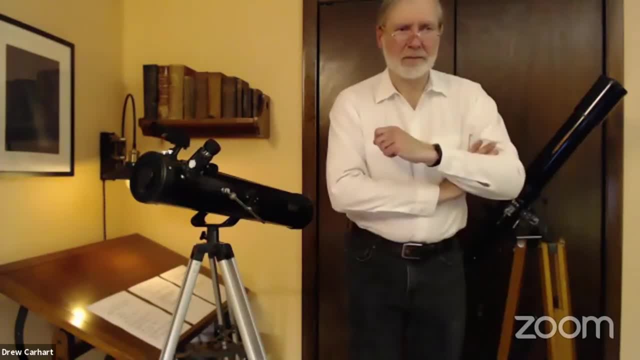 you're driving around in your car, so that that probably needs to be collimated more often than a smaller- uh, smaller- scope- i think it's something you can learn fairly easily- is how to check it out. so, if you're a big car and you're going to go to, the most important thing, by the way, is 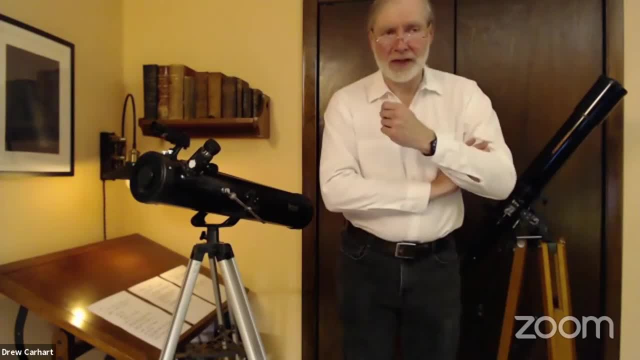 that you can check your collimation of your telescope by looking at a star and um, in 30 seconds i can tell whether the issue somebody's having with the telescope is collimation or not, just by observing a star. so that's a technique. that's what you want to do. 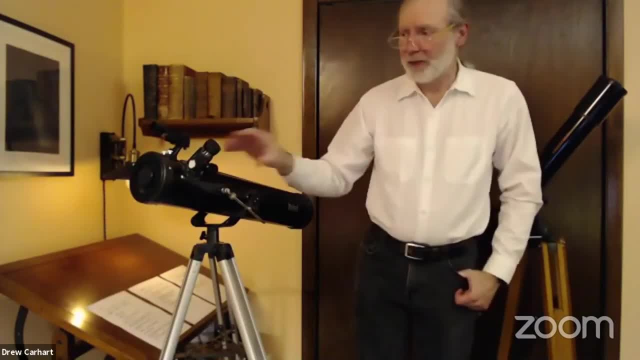 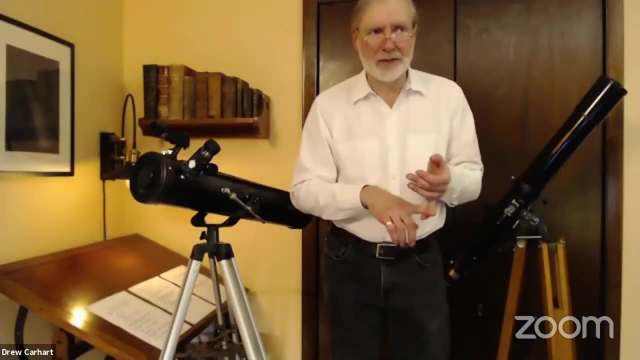 well with the. so with my 12 and a half inch over here when i set it up, i eyeball it and i can, i'm alignment. um, then i have a couple of simple tools that i look to be. i put in the id folder. i look. 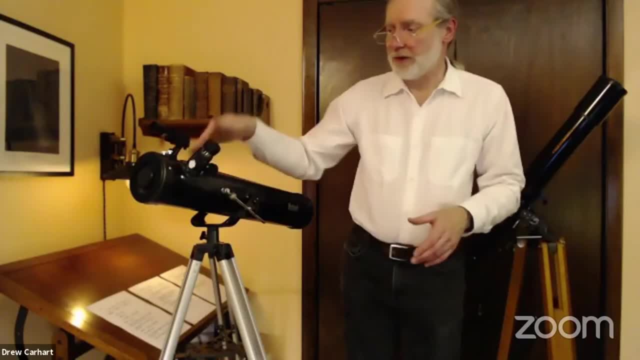 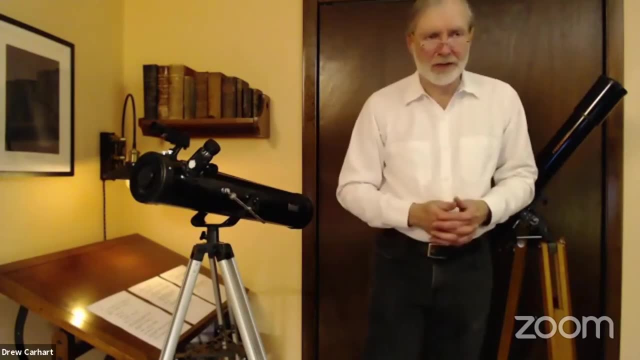 through to make sure. and again, it's a matter of all of these different angles being right, of the different parts. but i've oftentimes assembled that telescope and checked it and it was fine. but it's exactly like the alignment of the finder that it's just something that when 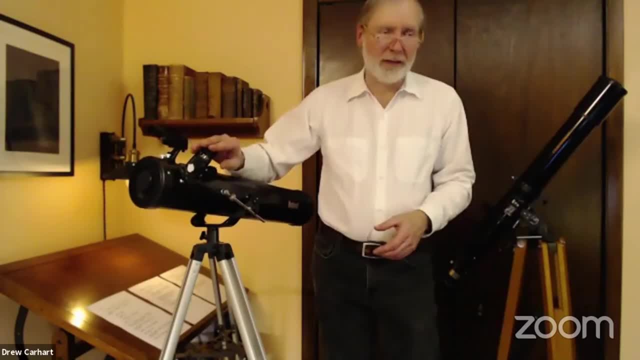 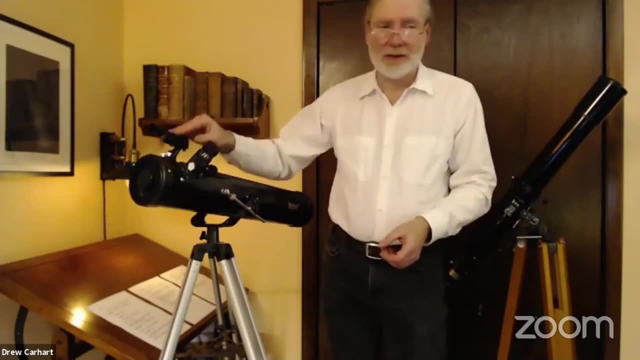 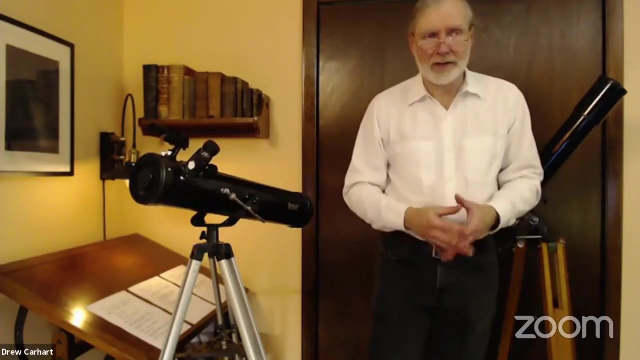 i set up the telescope, it's actually actually check the collimation first, because when you recall it, it's all still. it won't be in alignment with the finder anymore. so, uh, that's first and this is second, and both of those steps it's way less than five minutes to check um either of them. 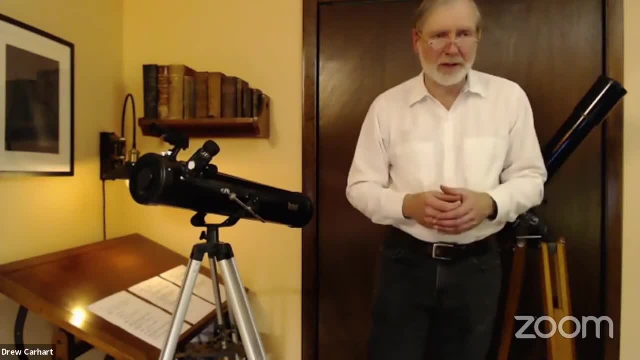 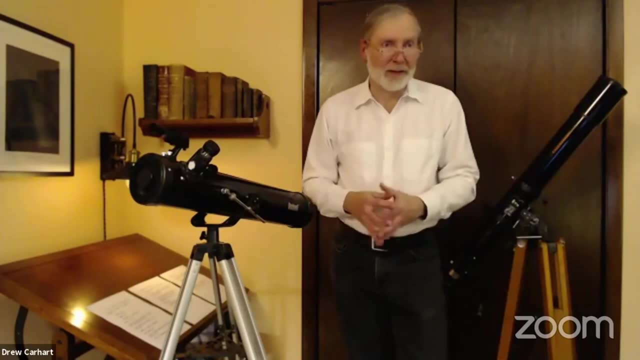 you know, see whether there's any adjustment that's needed, and, uh, and once you learn how to do it, um, neither of the adjustments take more than five minutes either. so, really so, it's not. it's not something that's threatening, but you do want to understand it, and 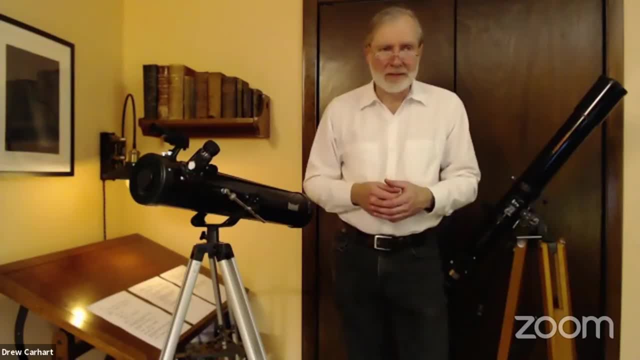 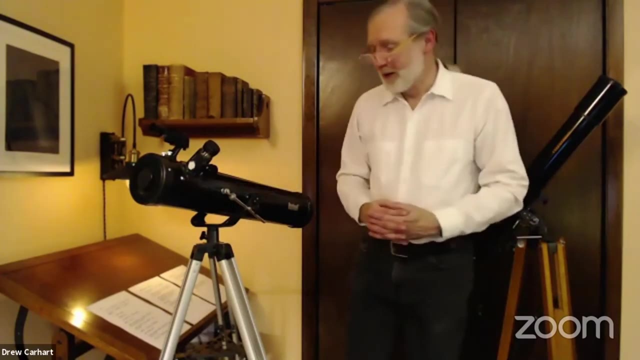 you don't want to dive into it. um, it's like you know, it's like surgery or something. you don't do it if you don't really need to do it. it's a um, because you're just opening yourself up for complication. anything else on the question list? yeah, uh. so joseph asked: are there? 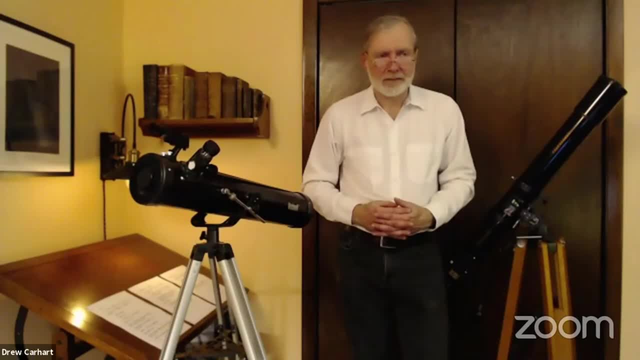 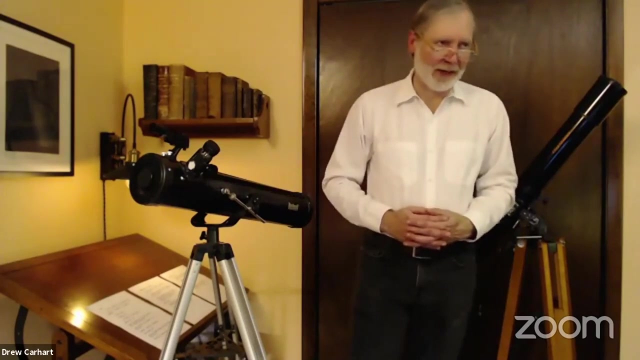 uh, oversized planet planispheres out there. uh, kurt, kurt actually responded and found a 16 inch. do you know, have you seen really big planet spheres? that's? that's as big as- except for ones that were made for, like, putting out exhibit um in publication- i, i think i've got a 16 inch over. 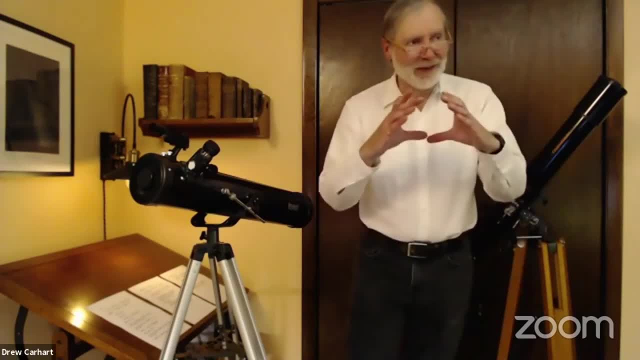 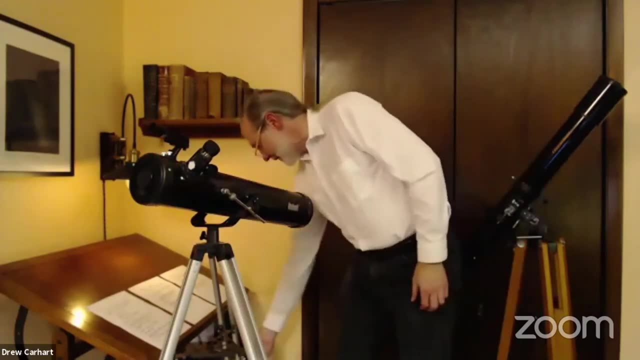 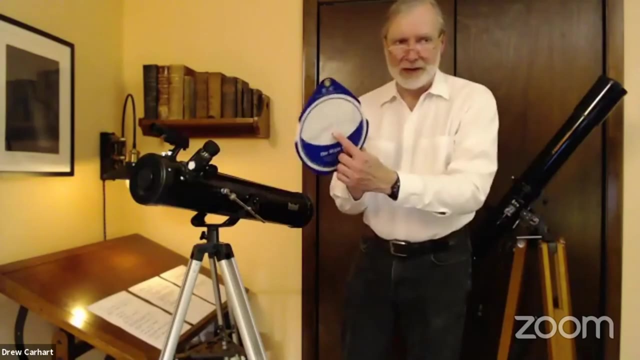 there somewhere. i've got a few of them. i've got a really tiny one that is nice southern sky one that so their planis theory is uh optimized for a certain latitude and uh shows the angle of the sky that you're getting, how high above the horizon. 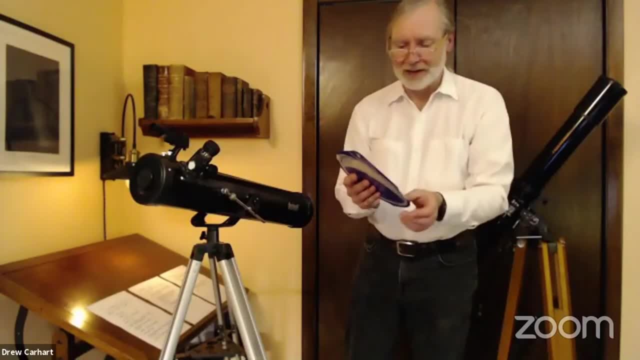 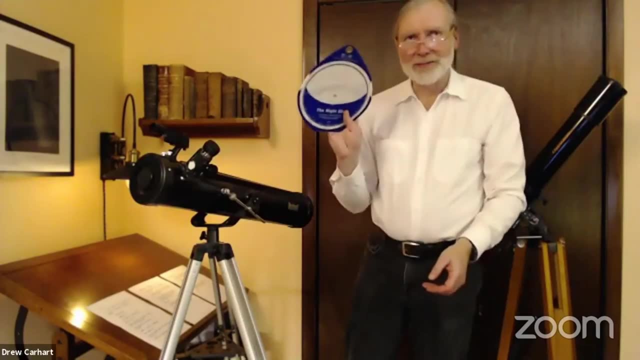 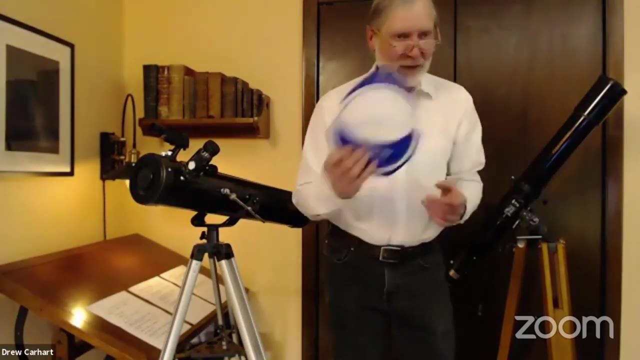 and uh, polaris is going to be actually um, but uh, size wise, yeah, um, but you know, welcome the problem of being middle-aged or older: you can't see small things in the dark. um, if you're going to be using maps outside, uh, i still almost prefer a map to a screen. 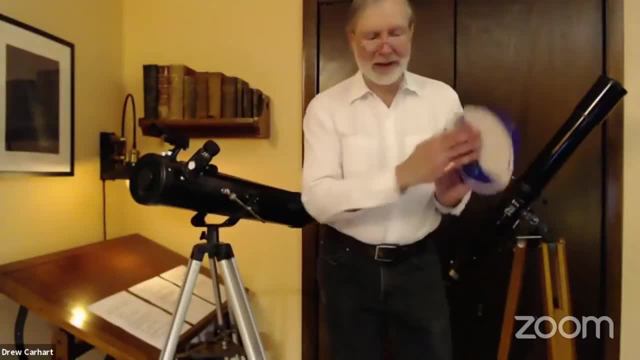 because i have a couple of really good flashlights that i like for lighting up. um, i can really minimize the amount of light reflecting back in my eye and still manage to. so the trouble with being my age and wearing reading glasses- which i only need these for. 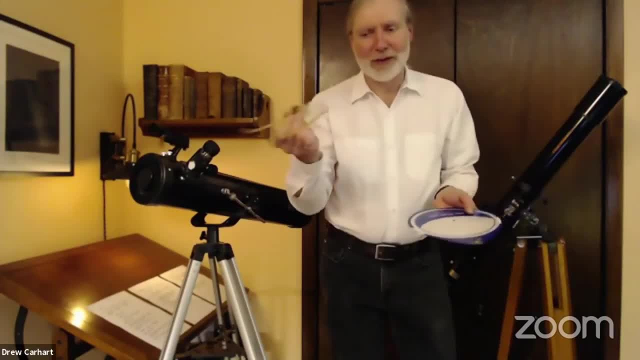 seeing things that are closer than my arm, that can reach um that. i'm constantly taking off my glasses to look up in the sky or look through the night piece and then putting the back on to look at a chart or whatever, but i'm not going to have the same amount of light reflecting back into my eye. 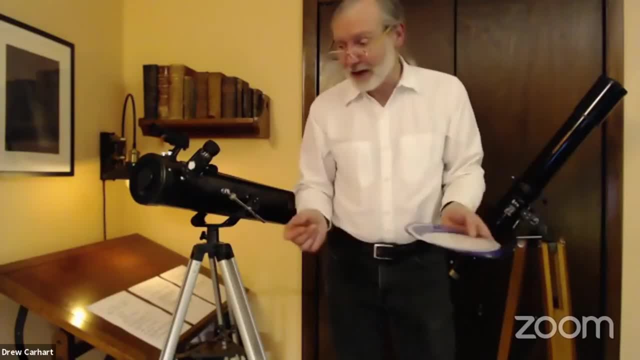 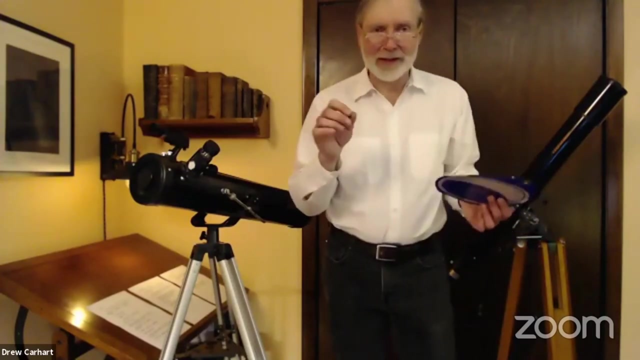 hey, that's life. um, you can. actually i do have. i don't have one with me- having a magnifying glass with a flashlight built into it. i've got one somewhere around that had a little bulb in the back of it. that's back from the incandescent days, but i painted the bulb red. now you could probably. 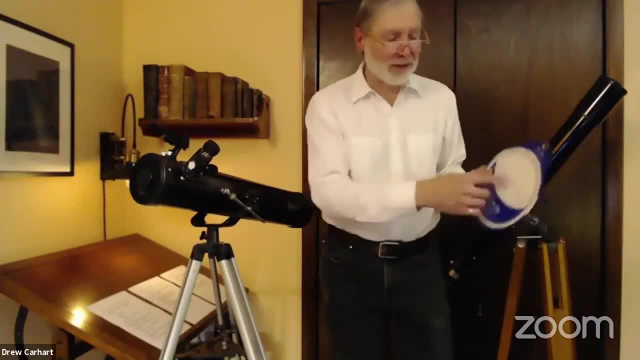 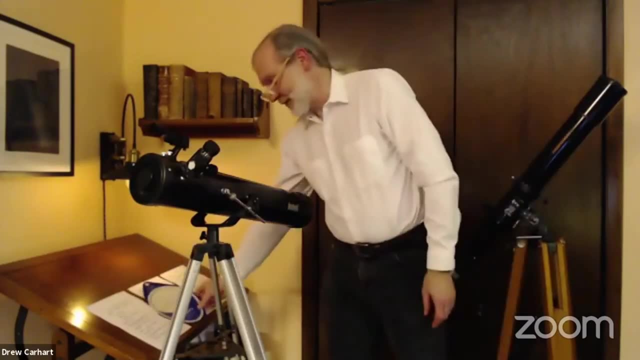 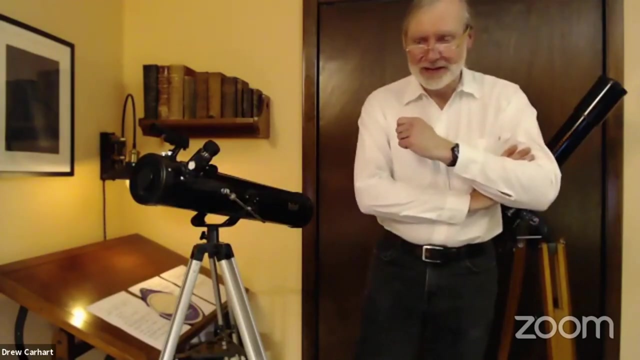 get one with red led in it. that's a handy thing for reading small stuff in the dark. but yeah, that's life is um, it's. it's hard to see little things in the dark when you're older. uh, anything else, yeah. so derek asks: how much observing would you recommend before? 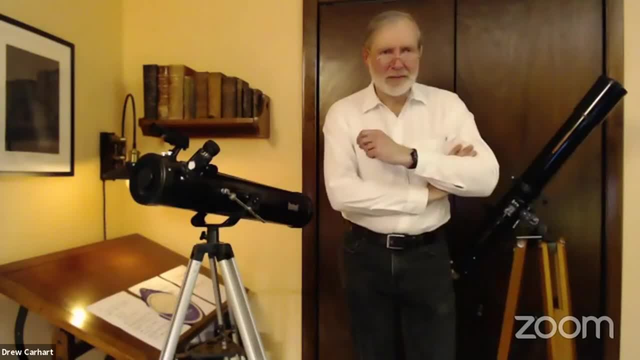 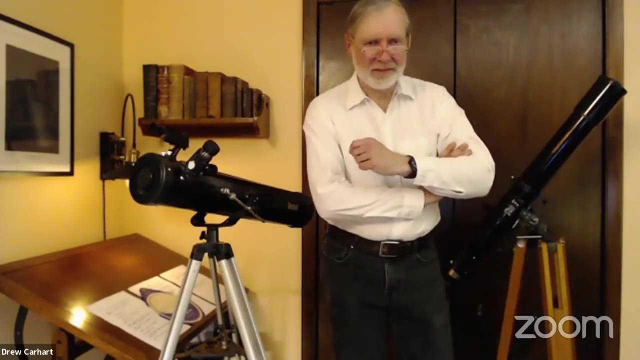 trying astrophotography and would i need a crash course or more in it in photography, to attempt astrophotography? so i'll just chime in real quick and say if you, if you think you're going to do astrophotography, you need to start off with the right type of mount. 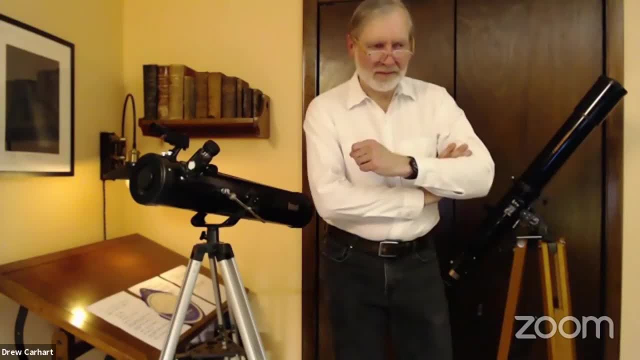 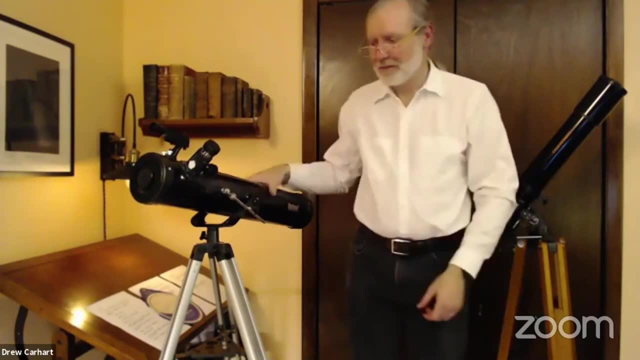 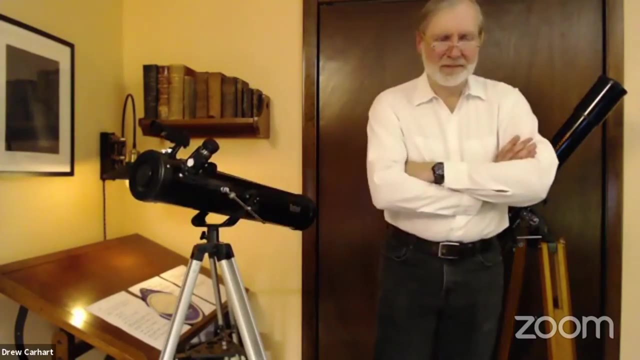 first and foremost. so if you have, uh, as drew is showing earlier, the telescope goes, you know, to left and right and up and down. um, that's, that's bad for astrophotography. you would want an equatorial mount. that's gonna, that's gonna move in the same uh arch that the you know. 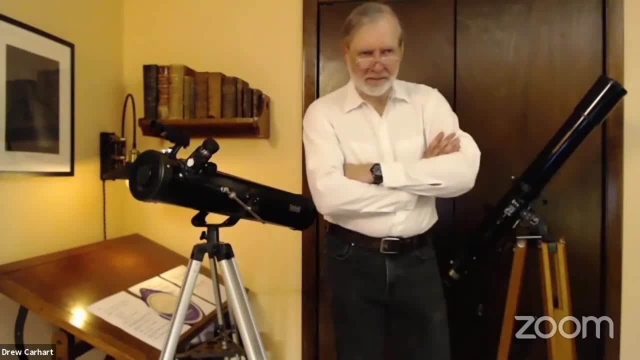 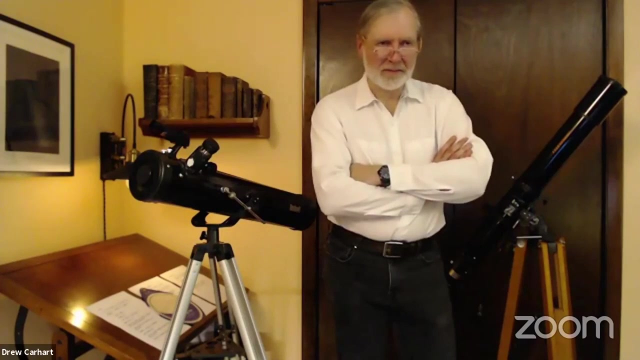 that the sky is rotating in. so it's it's. it's tough to retrofit a old azimuth scope to do astrophotography after the fact. you you end up throwing a lot of money at it to uh, to try to convert that, i guess. um so so i'll say that, just first off, we did a program last month on 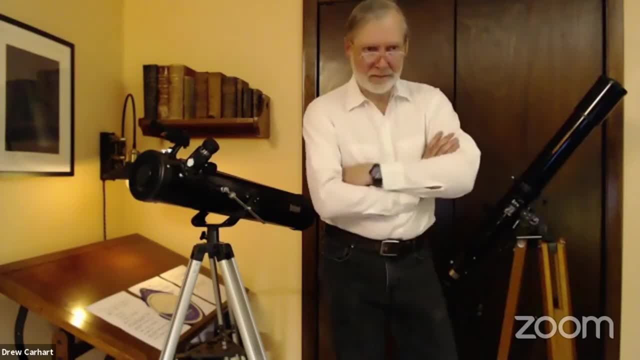 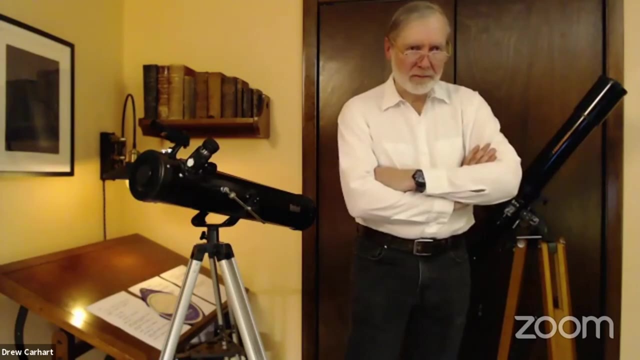 kind of astrophotography for beginners, so that's on our youtube page and, uh, that was basically mainly with a dslr camera, which is, yeah, camera you can use for normal daytime photography too. and then the other thing. so i tried to do astrophotography and i failed at it, so i i'm, i'm, uh, the one of the things that i. 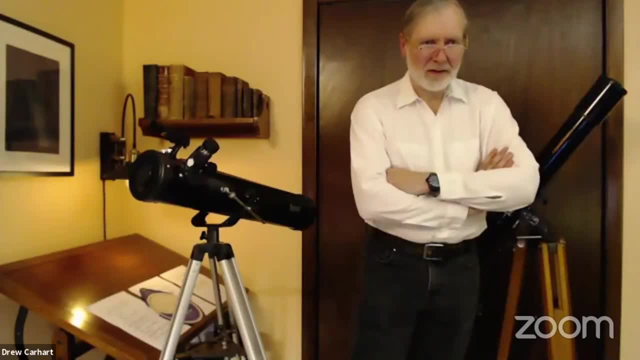 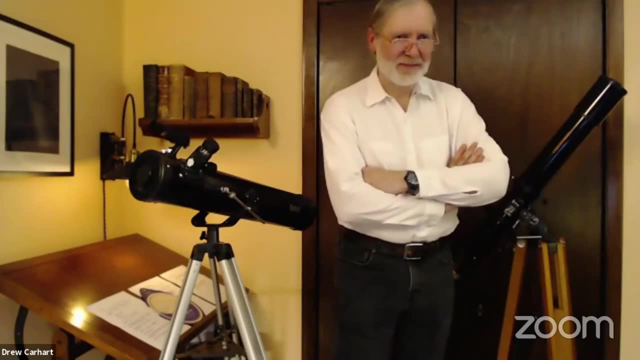 noticed right away is when i was sitting outside trying to do astrophotography. i was bored because now this nice, big, fancy telescope that i have has a camera hooked up to it and then i can't use it anymore. so the first thing i mean, after a week of trying to do astrophotography, i went out and bought a second. 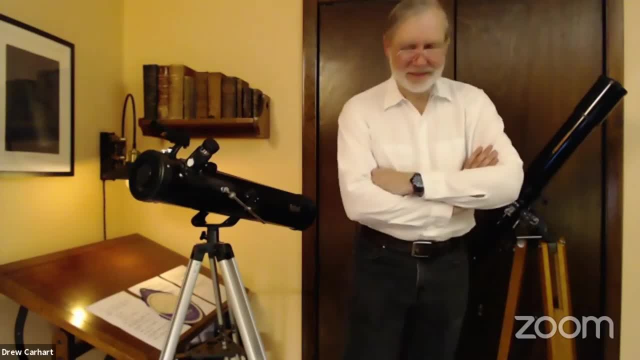 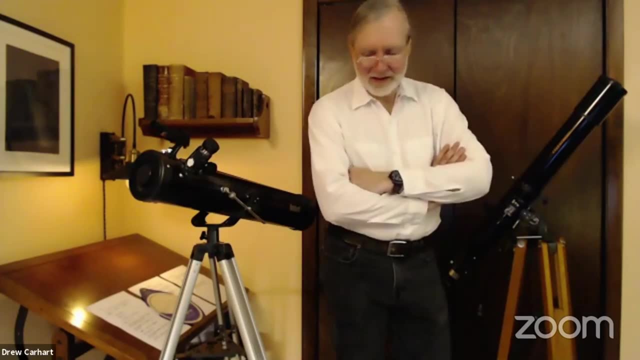 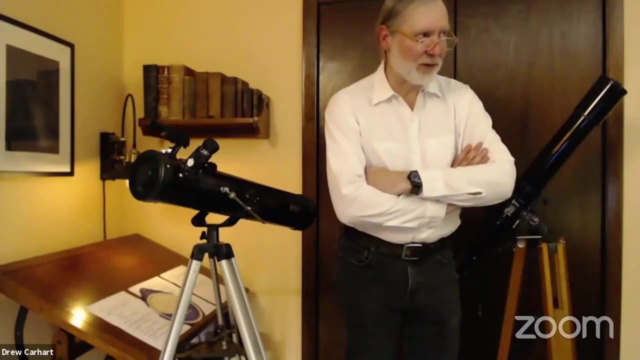 telescope so i could look through one while the other one was taking pictures. so it can be a slippery slope on uh your finances if you uh. well, i, during the the october presentation on uh choosing your first telescope, i said at the beginning of the program that i was going to do. 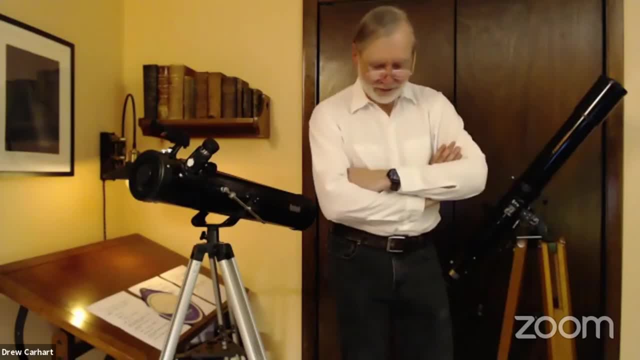 it and i realized a lot of the questions had been already been definitely brought up in the description because i was so tired of it. i was just sitting there thinking about it, so i was asking someone at the beginning of it. i'm talking about telescopes for visual use and i caught. 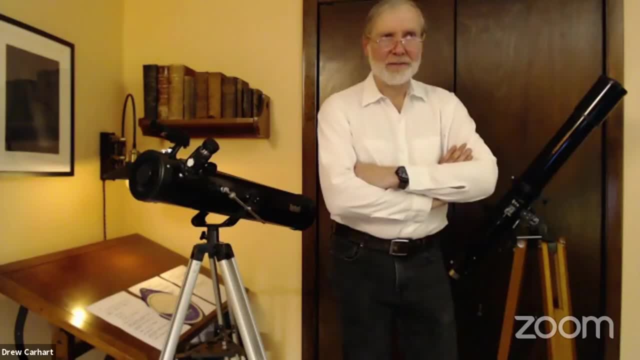 for that from some people because well, it's like, well, i usually use the same telescope for the two. but my friendly advice is that, um, i think both astrophotography and visual observing used to maybe be simpler than they are now. astrophotography certainly is branched from like four ways you can do. 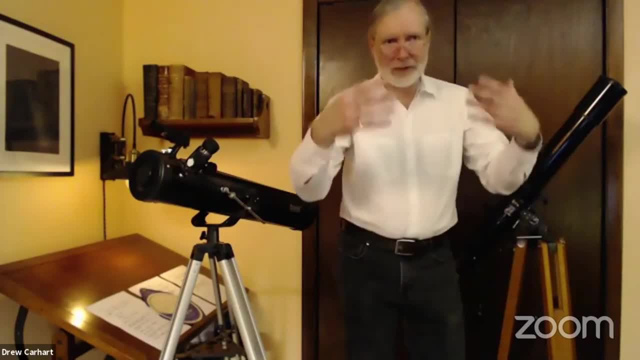 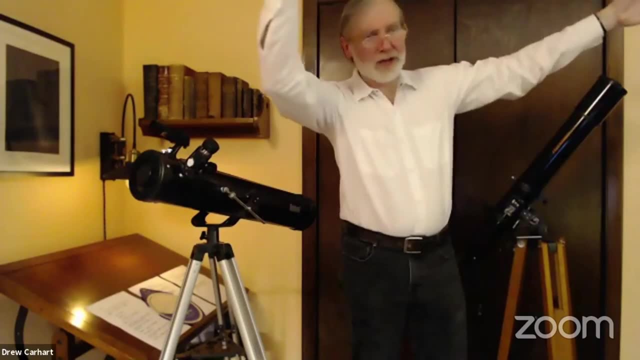 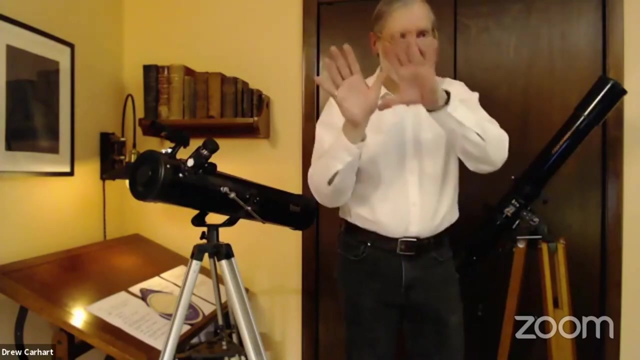 of ways you can do imaging of some sort or another of stuff up in the sky, of celestial things. it's a whole tree that's branched out in many directions and in some cases the stem, some of the stems and the parts are very similar to the tree over here that we visual observers use of. 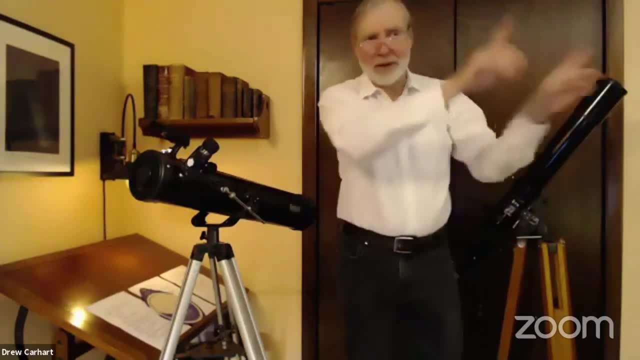 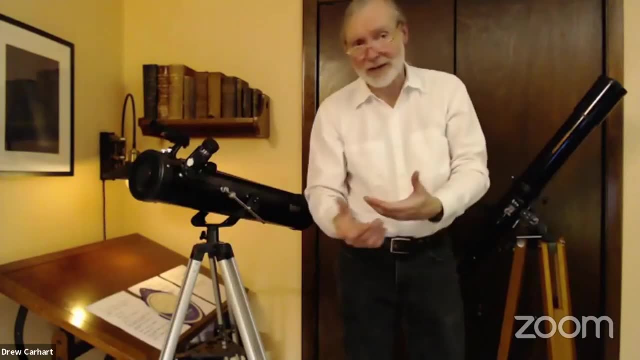 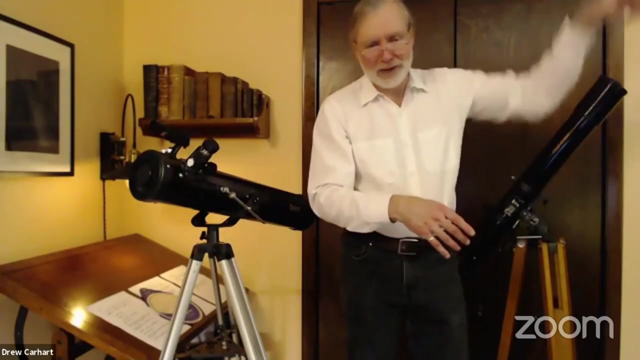 things in other ways. it's gone off, but parts of it aren't the same. you've had the perfect telescope to do one kind of astrophotography. it would not be the right telescope to do a different kind of photography and so it's really a complicated uh branching woods stuff out there. 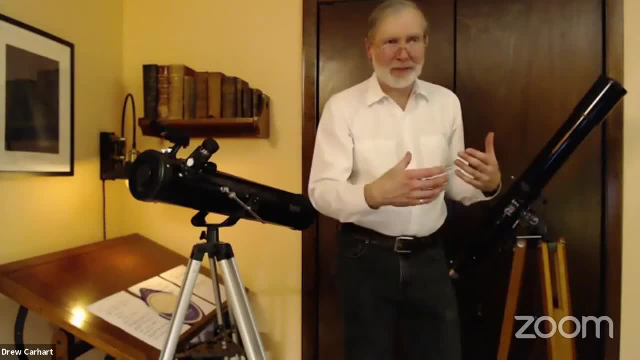 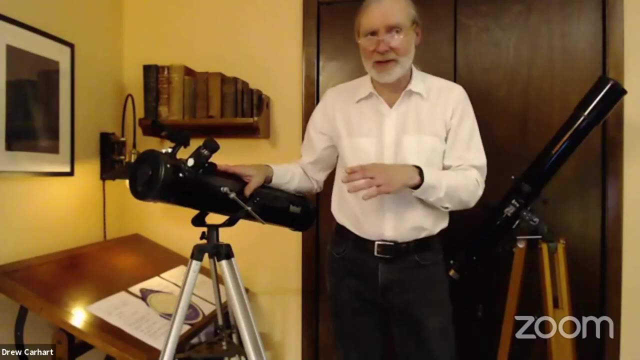 and uh. so it really takes backing up and saying what do i want to accomplish in the end and what do i need to do that? and again, in some cases it might be well i could buy this one telescope and i can both observe fluid with it, because i want to observe pluto with my eye and i can. i can take pictures of galaxies and 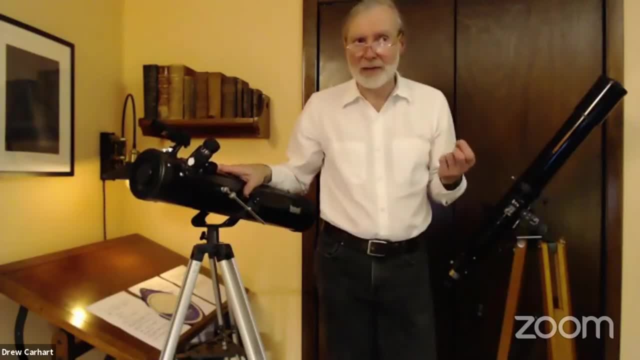 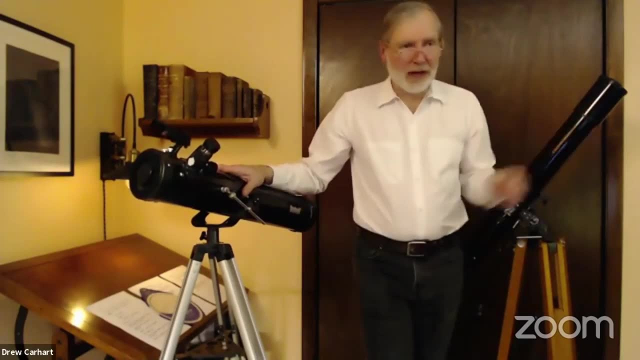 that would be great. but there's going to be a lot of times when it's like, well, this telescope is optimized for taking pictures of galaxies. it's probably going to sit with the camera on it all the time, because i have to dismantle it to put the camera on and this and that, and i'm not really. 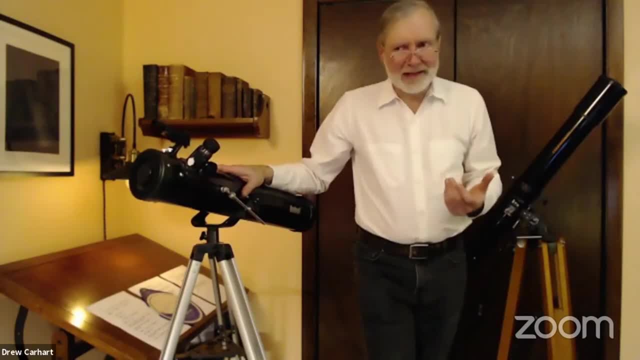 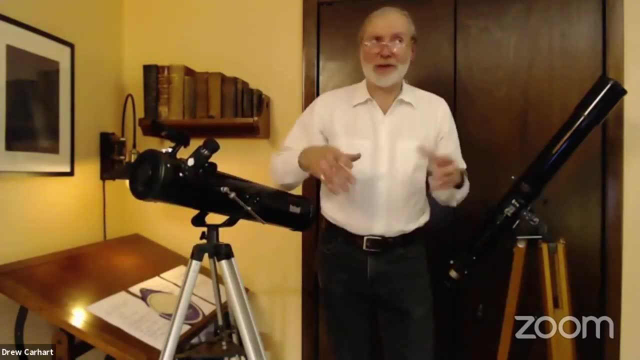 going to be observing with it otherwise. so it takes study. i wish you know, i wish there was a. somebody could even get an hour present tation. that would cover all the bases of it, but it's, it's a complicated thing and i and part of his question was: should he take a crash crash course in photography? 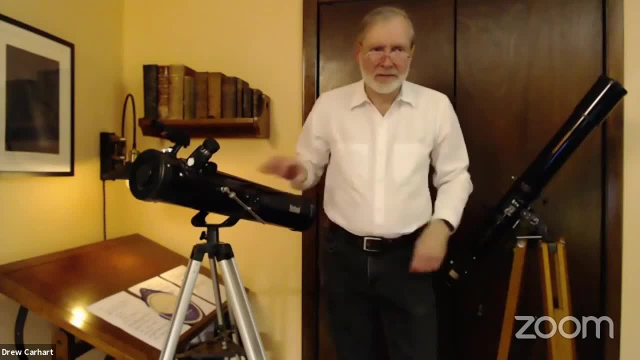 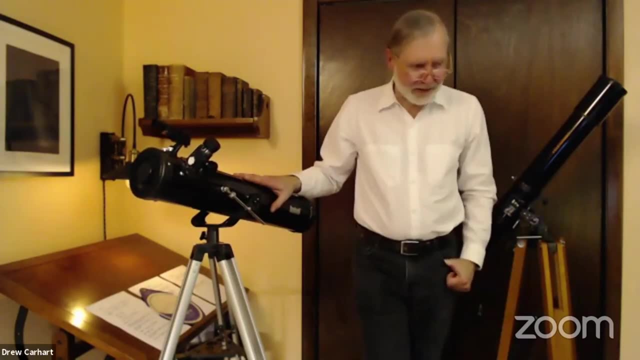 i would almost say you needed more of a crash course in photoshop and how to. uh, we did have one of those um in a monthly meeting back in june. i think um was our presentation on processing digital astrophotos, so that's on our youtube channel. but yeah, that's a whole thing to itself. you not only need 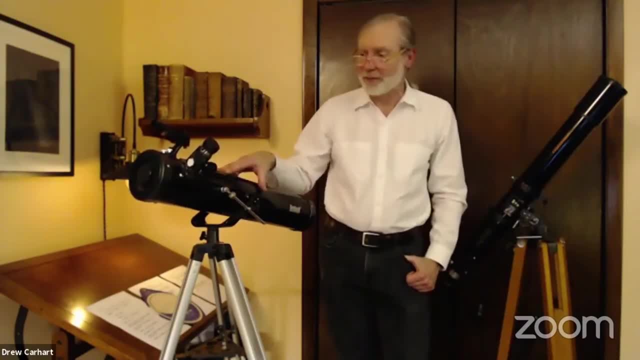 for that type of setup you not only need the telescope and the camera, you need the computer with all the software on it in the wherewithal to use all that to actually come out with a picture to show on the end, because it doesn't come out, like the old polaroid cameras used to, with a